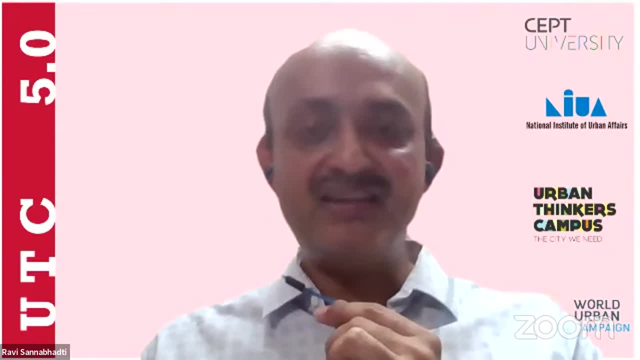 I don't need to actually mention his CV is so long, but he has been associated in a number of urban development, urban governance, urban infrastructure initiatives with the UN, World Bank, USAID. But throughout all his assignments, poverty alleviation has been a kind of key component of all his assignments. And before joining NIUA, he has had certain kind of notable achievements. He was intensely involved in supporting ecosystems to design and roll out urban programs, including localizing SDGs. 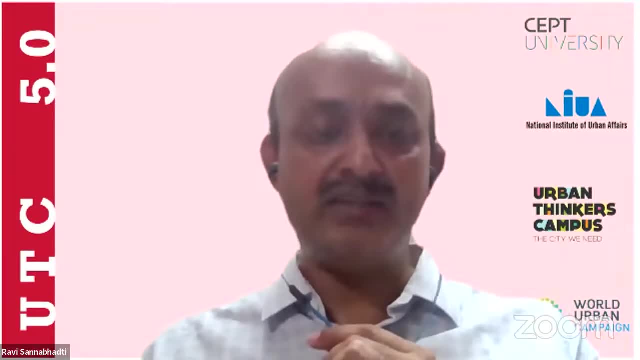 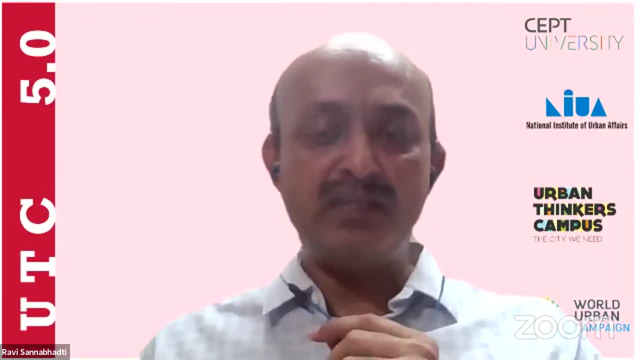 development and planning and specializing in urban management from Institute of Housing and Urban Development Studies that is IHS Rotterdam Netherlands. 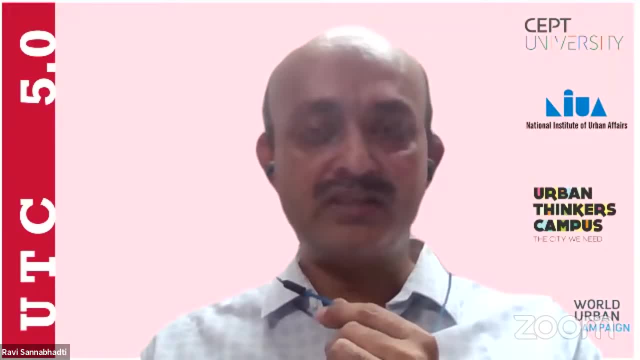 So I would request Mr. Hitesh Vaidya to kind of please chair and moderate this session. 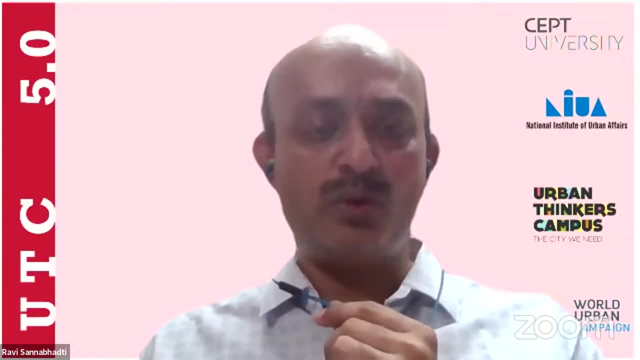 The first speaker for this session is going to be Professor Om Prakash Mathur who is a 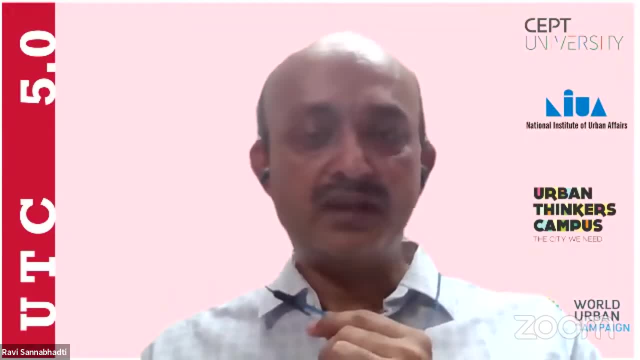 senior fellow and global cities Institute, at the global cities Institute University of Toronto. 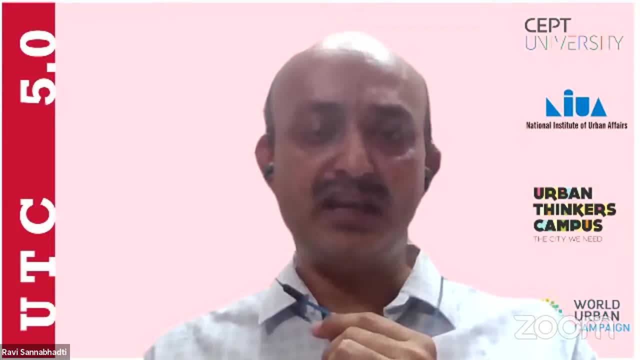 He has served from 2014 to 2019 as a senior fellow and chair Urban Studies at the Institute of Social Sciences New Delhi. 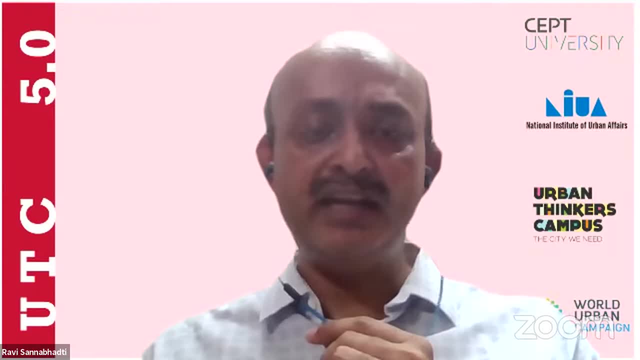 And held this position from 1992 to 2011, the position of IDFC chair professor at the NIPFP New Delhi. And from 2021 to 2020. Okay. 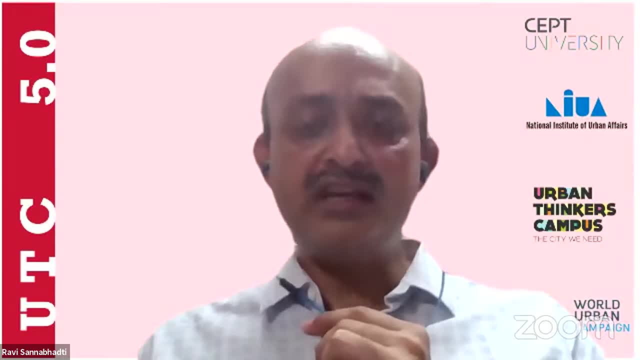 From 1984 to 1992 he was the director of NIU-8 and a distinguished professor from 2011-2014. I can go on and on about Prof. Om Prakash Mathur. 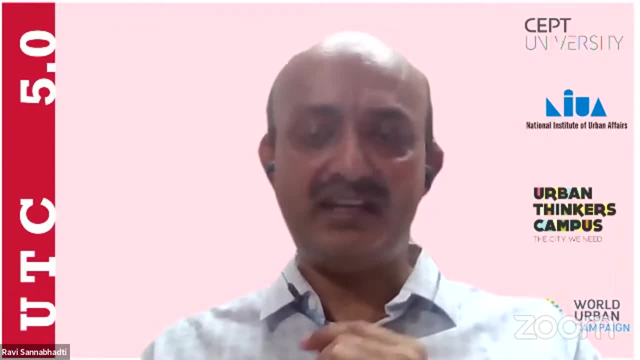 As my colleagues have often mentioned, he has been a teacher to our teachers. So in that sense he has been a master teacher to all of us. 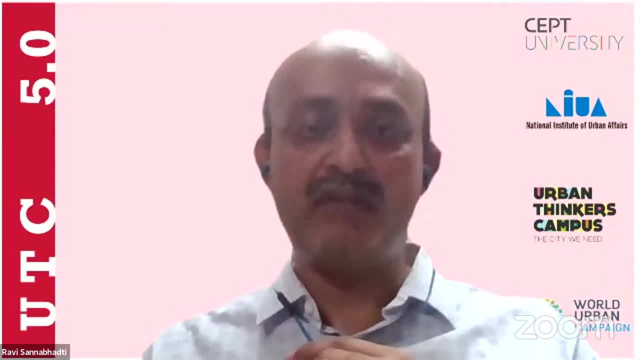 He has served in a number of various committees at the international level of the UNDP, UN Habitat, ADB, GIZ, World Bank, UNICEF, to name just a few. Similarly, he has served in a number of national committees, notable among which was the Jawaharlal National GNURM Mission. 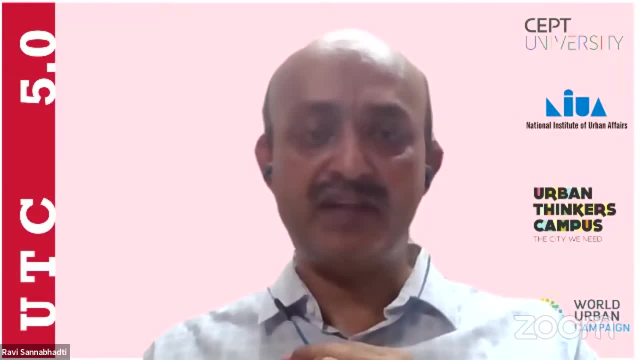 He was also a member of the High-Powered Expert Committee on Urban Infrastructure Requirements 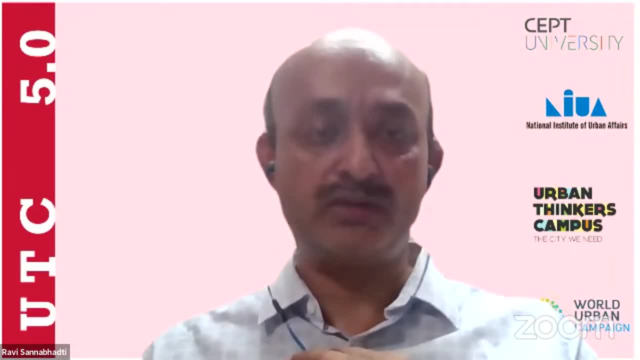 And a member of the advisory panel of McKinsey Global Institute. 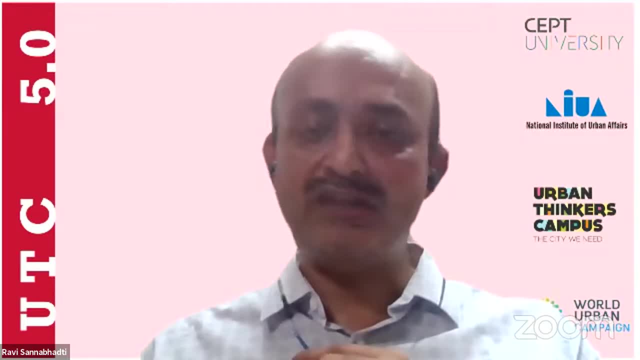 Of course, his list of publications is kind of endless. 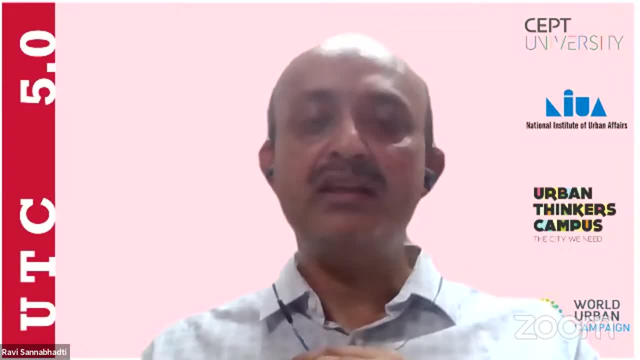 So I will not get into it, but I would just say that he began his education, he began his career with an education or master's degree in economics. 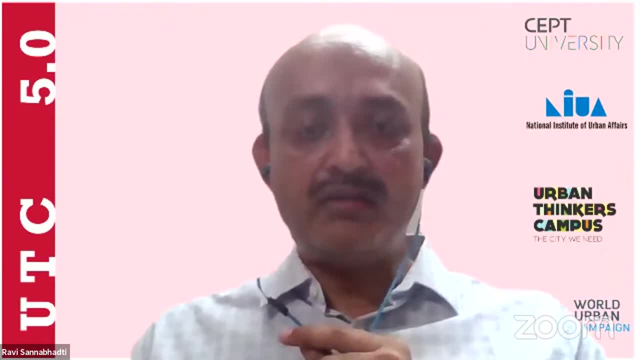 And he has attended graduate courses at MIT and Harvard University, USA. 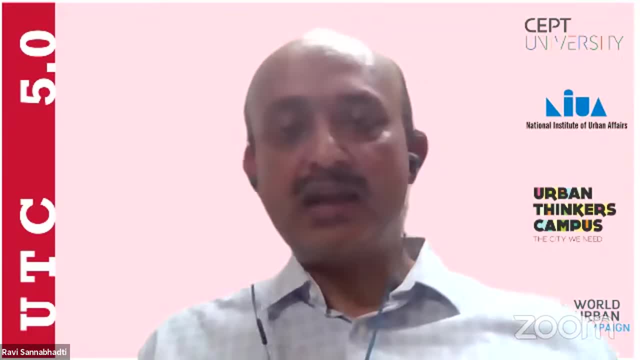 So that is in brief about, I will extend my invitation to Professor Wajid to now chair the session, as well as later invite the first speaker to come in and give his thoughts on this topic of reimagining policies for our cities. 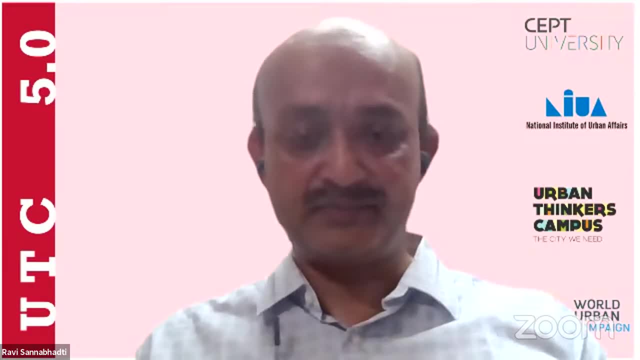 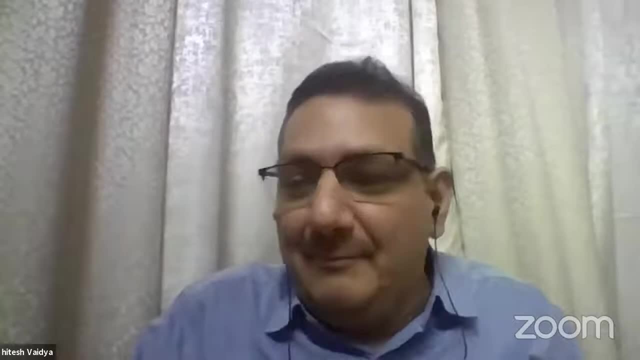 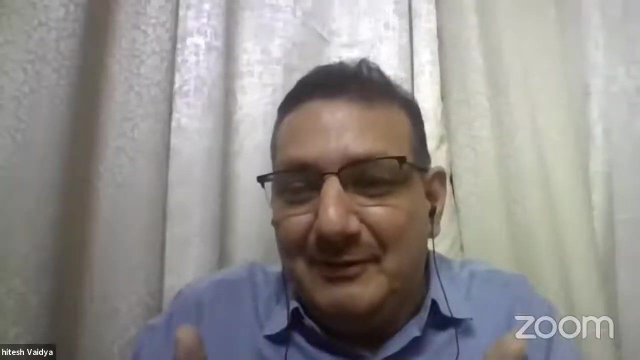 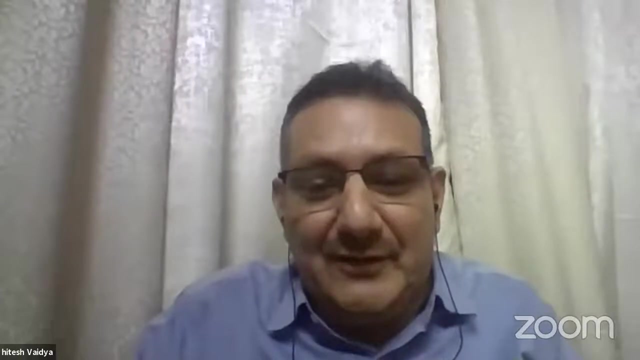 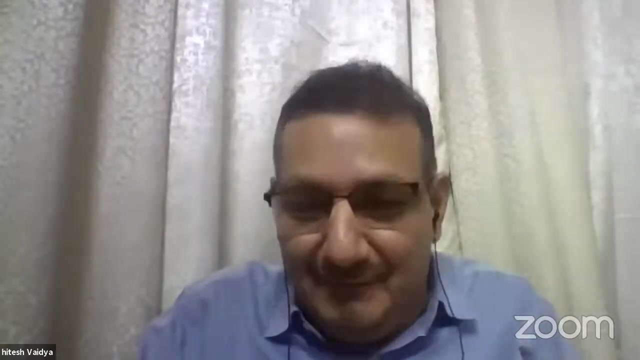 Please, Mr. Wajid, can you please do the honor? First of all, thank you, Ravi. And thank you, SEPT, inviting me. For this session on policy dialogue, need for urban policy change, I think. But before I say that I am chairing, you know, I have learned ABC of planning with the people who are sitting on the panel. So I, you know, with my all gratitude to Professor Mathur, Madam Sheila Patel, Professor Massimo, Professor Ramachandran, who will be joining. Sir, I'm really not. 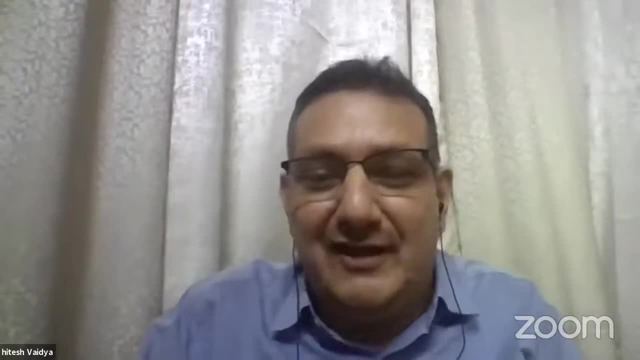 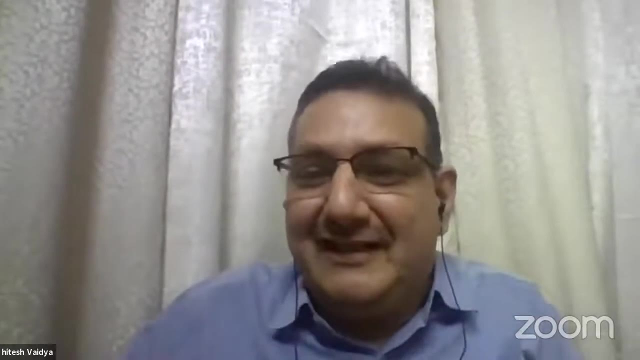 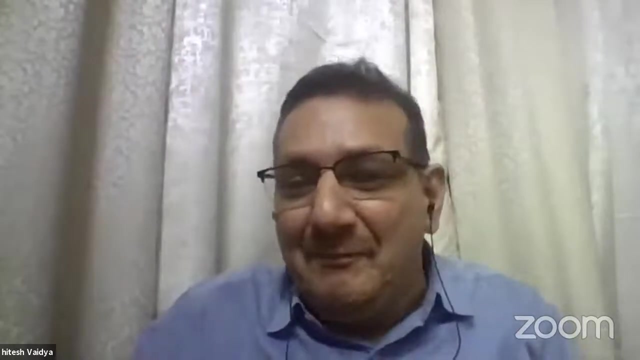 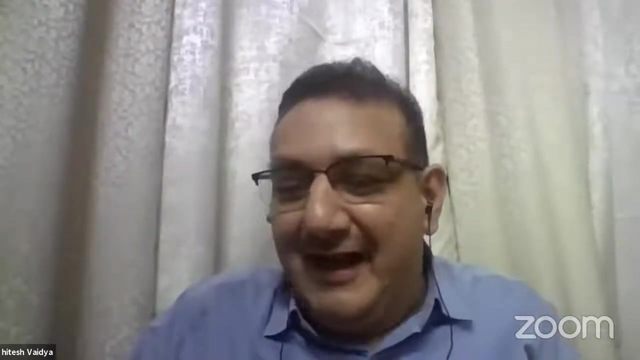 Neither the capacity nor capable to chair a session where you are representing my please apologize me for just because I'm sitting in a chair, I think, but with my all humbleness, I'm really, really sorry that I have to feel. I can't show you but tears are there in my eyes because I'm sitting there just because you are there. 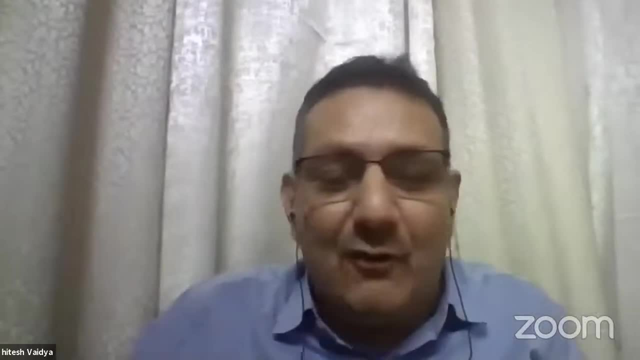 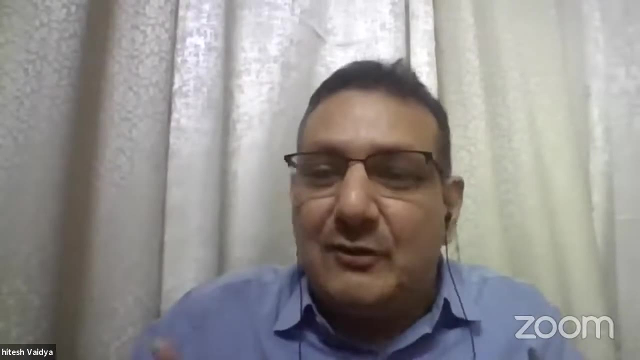 I don't have any words to say so. And with the stalwarts like this. You have taught us who have who have been guide, they are the vision pitamas of the sector and today what we are living in this urban area is the urban which we have inherited from them. 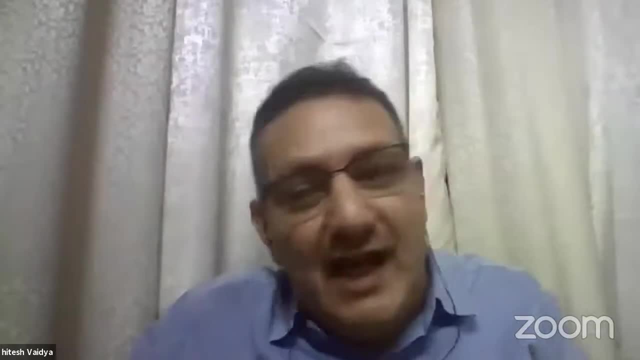 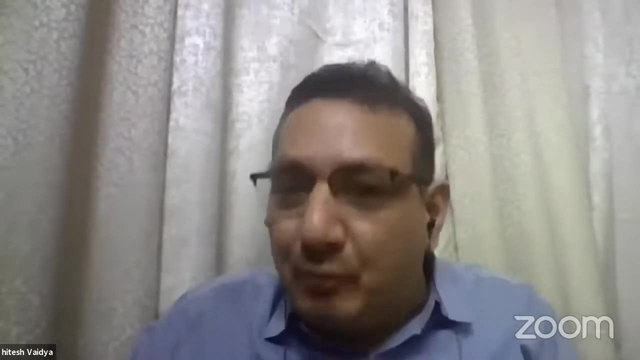 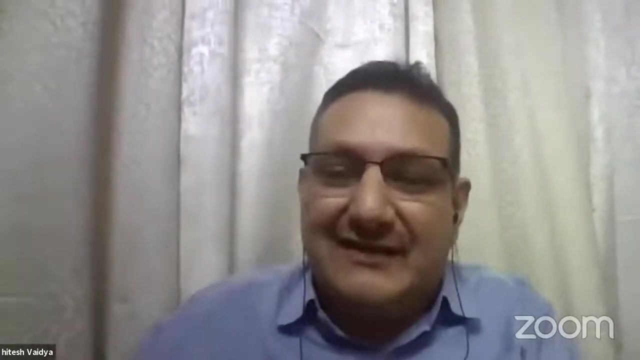 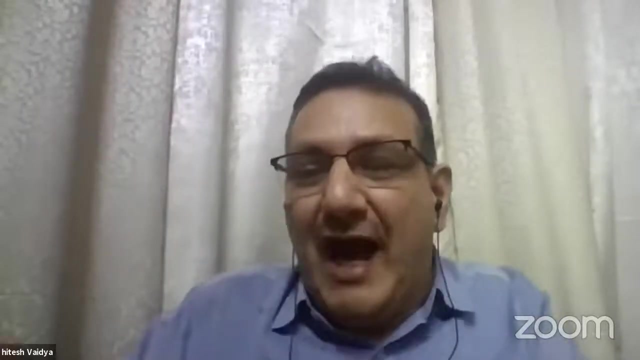 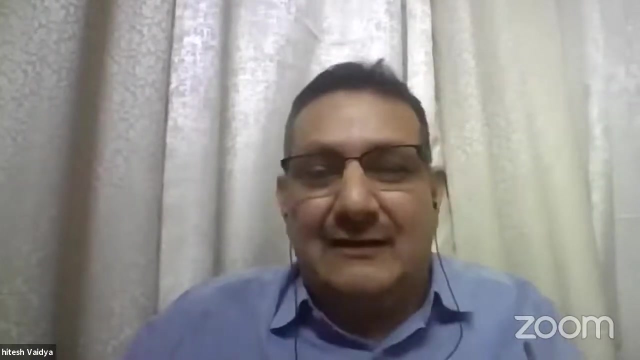 And I'm sorry, I must say the what you gave us, we have not been able to sustain it. It's our our generation has not added it, we have spoiled it. And this beginning today is if tomorrow my son which I was studying. Next. says what type of planet you have given what is that you are leaving us behind i'm i'm ashamed that we have not been able to do that but i i look forward your guidance that at least when i go out of this sector i can hold my head high in front of my son that at least i gave you something which 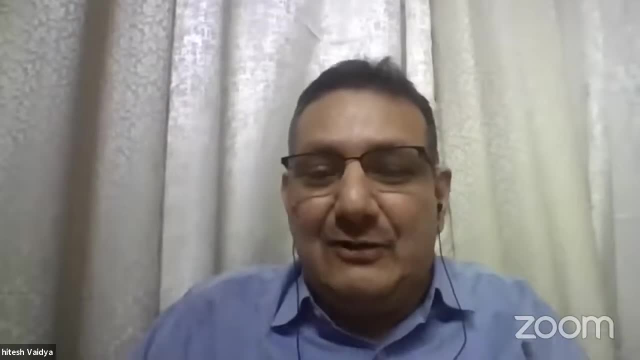 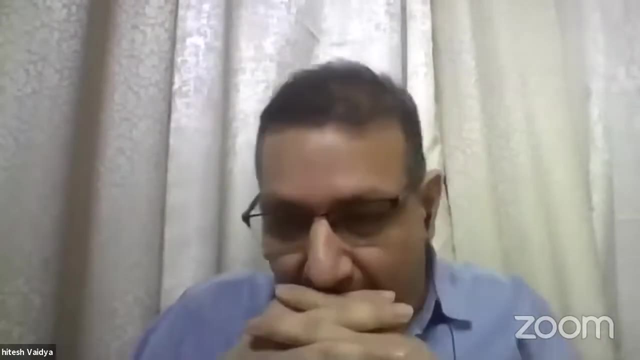 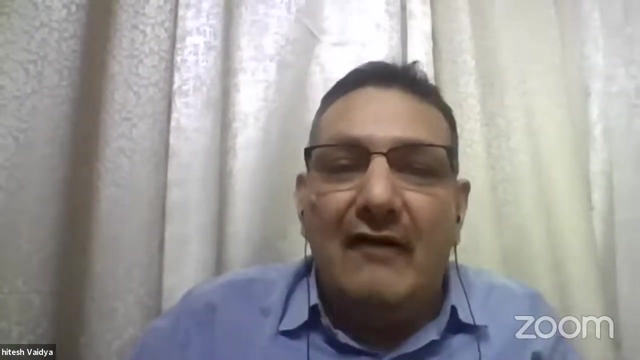 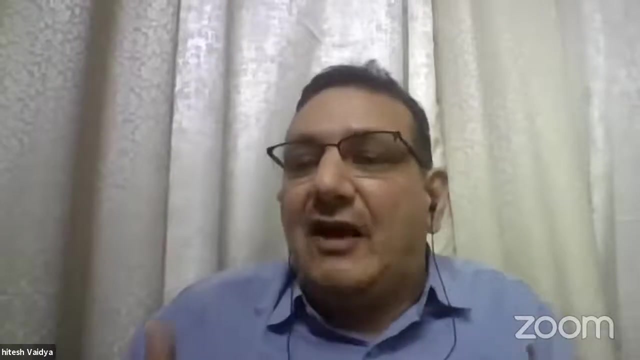 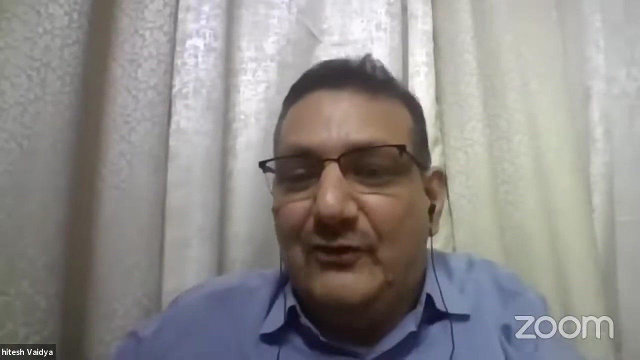 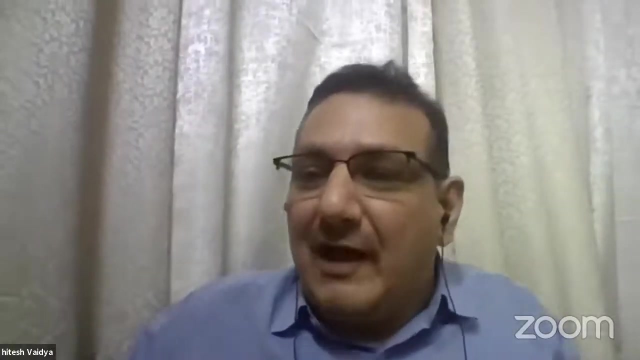 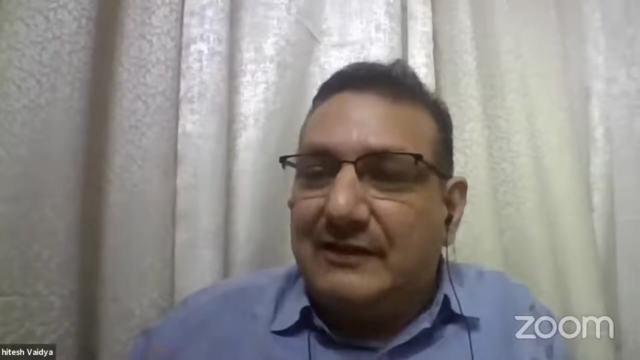 you can build on it so with that uh great uh gratitude sir i'll start beginning please excuse me i don't have any sentences to say but during the post-covid sir as you uh rightly say we have been struggling with this all issues which is are we safe in our own cities how safe our cities are how we are managing this new normal the way we are calling reimagining our new normal the way it's when we were looking at an abnormal era and we were moving towards the normal so what should be this new normal we have been looking at the challenges of mobility now people are scared of coming into a public transport uh you we have seen a huge number of private transport triple the number of vehicles on on 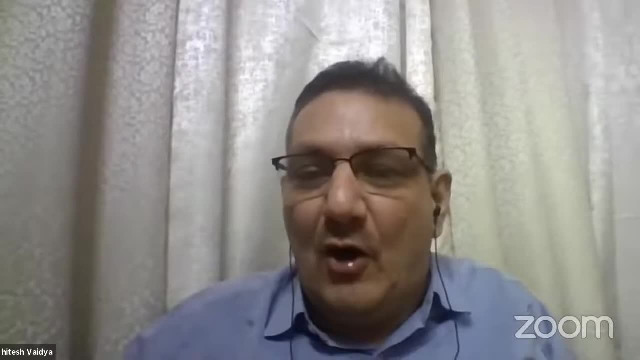 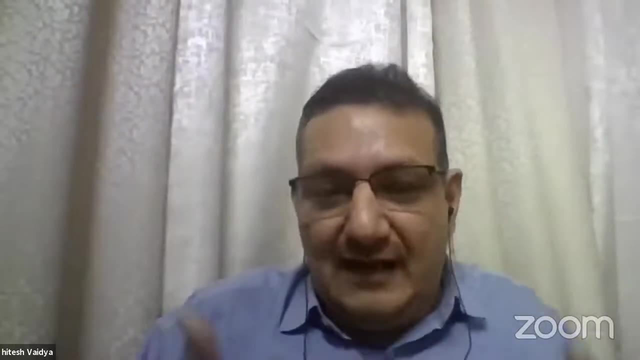 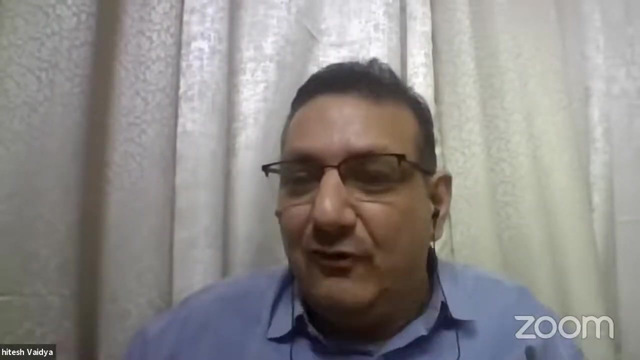 on the road so what should be that new normal in terms of public transport versus private transport we are looking at work from home which was not there and right now with this um meeting which we are having virtually i you know even we say that is a new technology new way of working we are looking at work from home which was not there and right now with this um meeting which we are having virtually i you know even we say that is a new technology new way of working 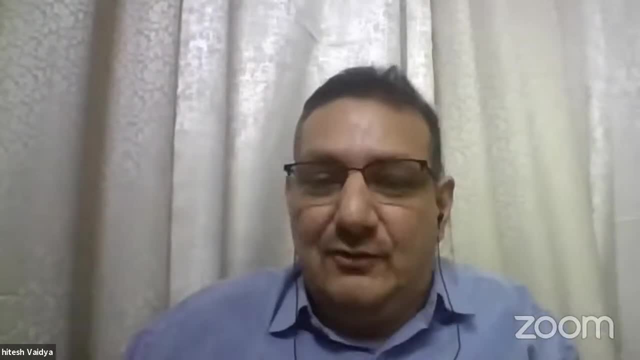 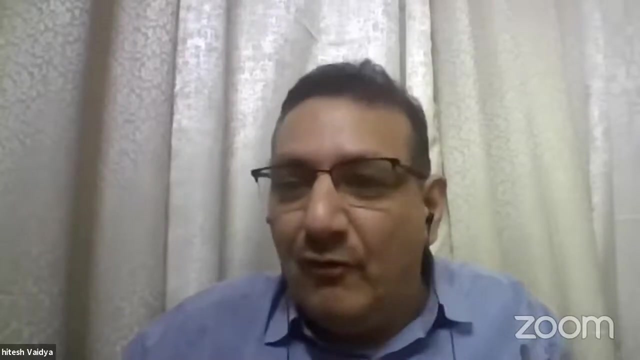 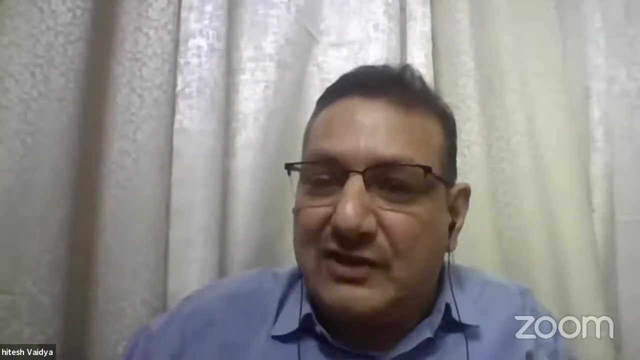 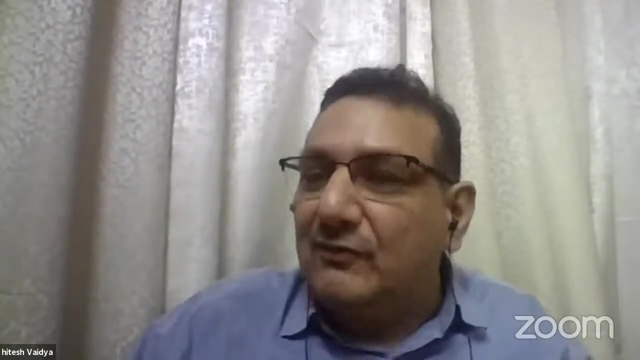 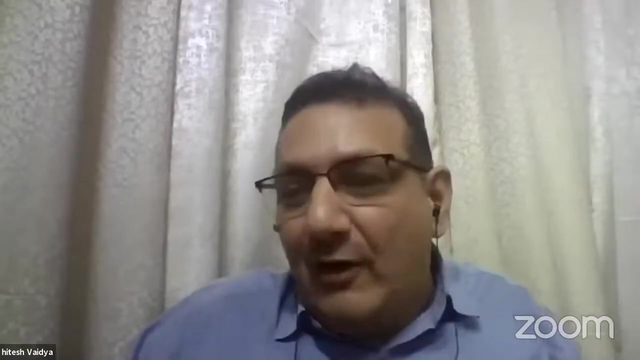 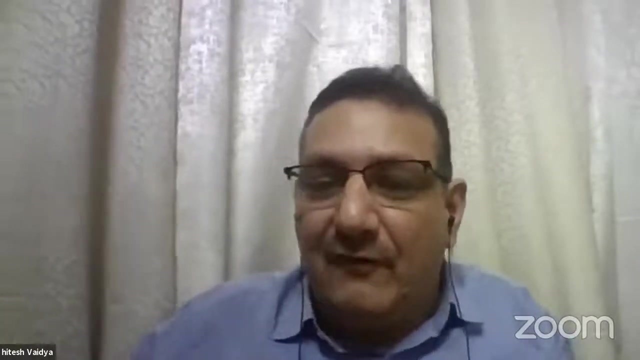 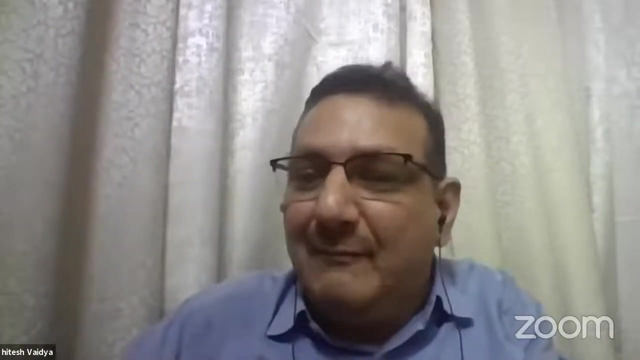 but i think virtual meetings really loses the empathy towards the subject which we have to do it so how do we adjust ourselves to this new normal of office versus work from home because for me as an i think working an organization of a government organization work from home sometimes into no no work at all so how do you really adjust yourself with the systems which we have which are not adhered to the work from home culture and we just jump to the work from home second sir we are also looking at um commerce the whole commerce in the city has changed we have now looking moving from retail shopping to online shopping even though online shopping is becoming good but the people you know in front of your society when you see well numbers of packets and number of people your service lane are choked because of these delivery people who are standing on your thing and is creating even not not only the main road but your service lanes have chocked because of this 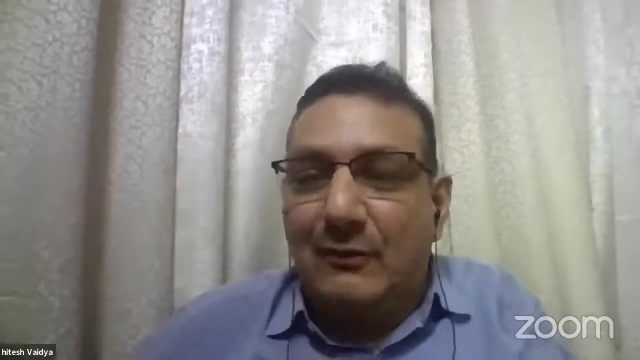 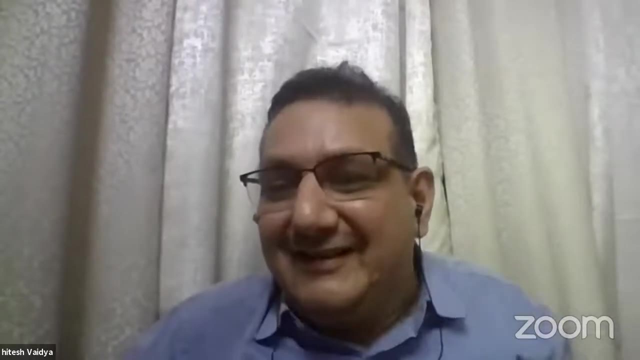 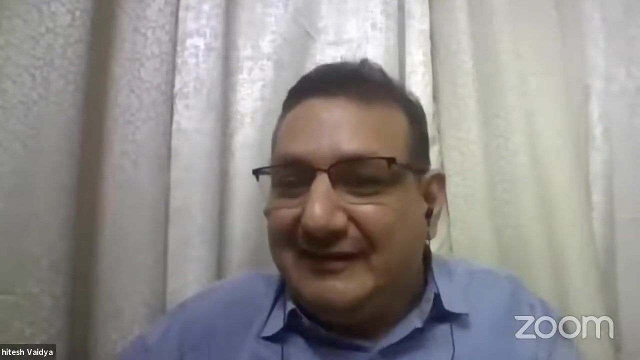 online shopping people who are coming with their vehicles uh to deliver the goods and so on and so on so on and so on so on so on and there is a lot of conversation about sustainable way to deliver things socializing you know and we also studied uh human is the social animal and now we are sitting in our own chambers talking to this screens how social we are and how do we really 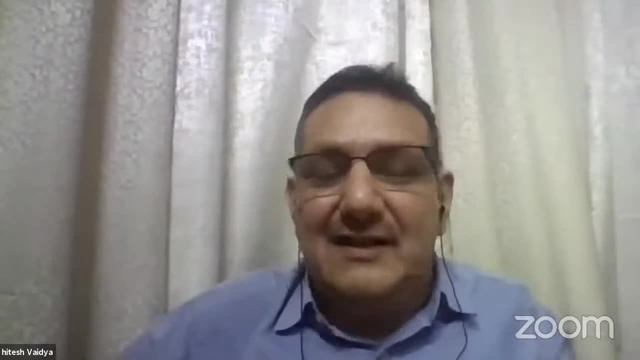 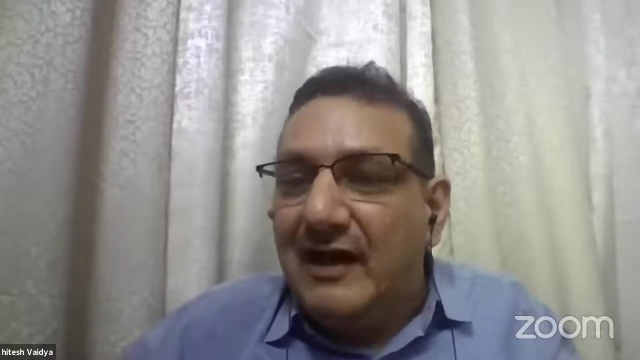 move toward that social norm this is a challenge and if we are talking about planning sir which i see as i told you we have failed as a planner uh to really manage our cities better we are 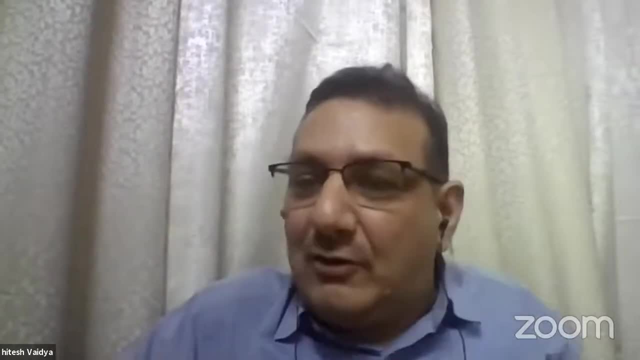 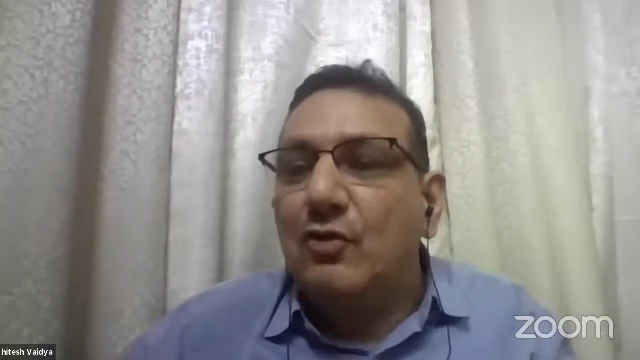 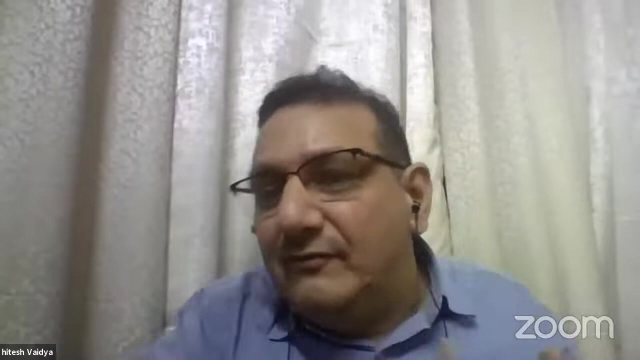 about prosperity, we all talk about inclusivity, we all talk about sustainability, but right now we have these challenges to sustain this and move forward that new norm or new normal we want to do. Sir, I don't have anything further to add but you know listen to your so many years of 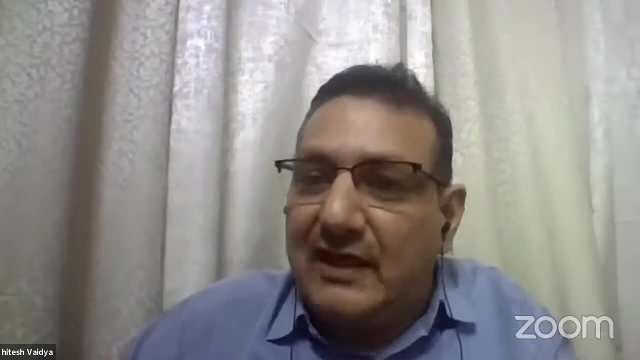 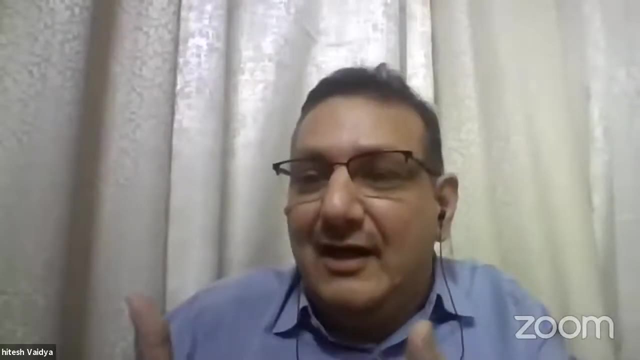 what is the guidance you can give which we can pass on to the next generation or at least start working on those which we have not done. So I will invite with my all humbleness to Professor O.P. Mathur over to you, sir. Thank you very much, sir. 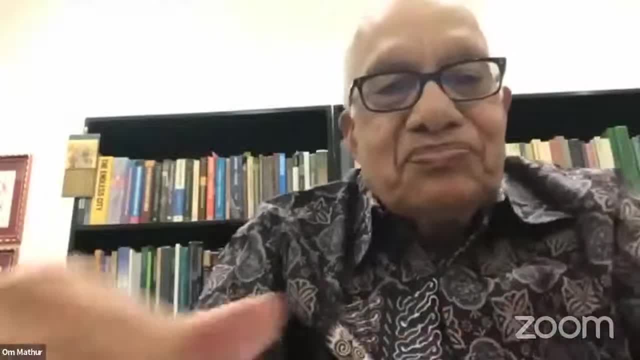 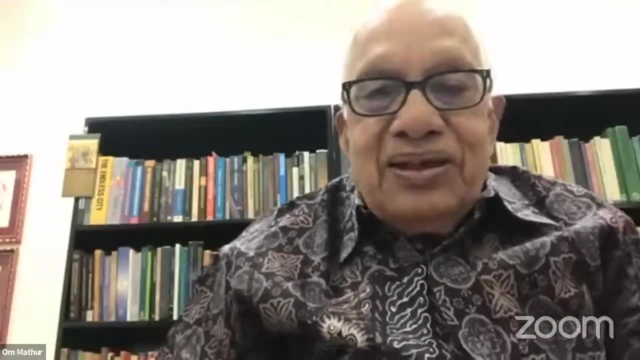 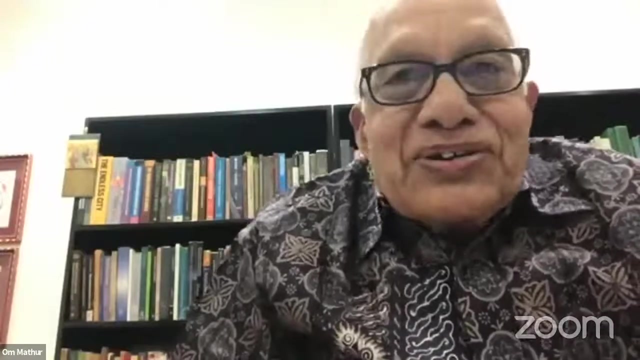 Thank you very much, Hitesh, both for this invitation as well as introduction. I don't know what all you said needed to be said but let me not spend time on that. We can discuss it some other time. 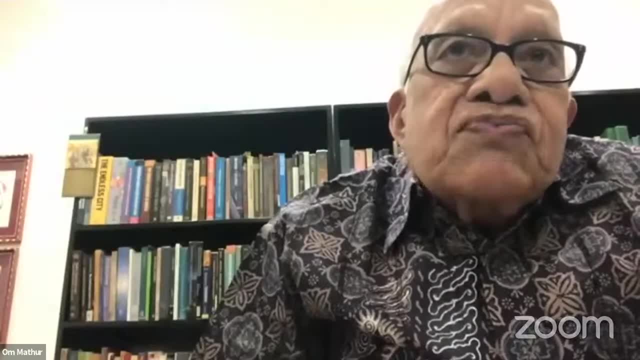 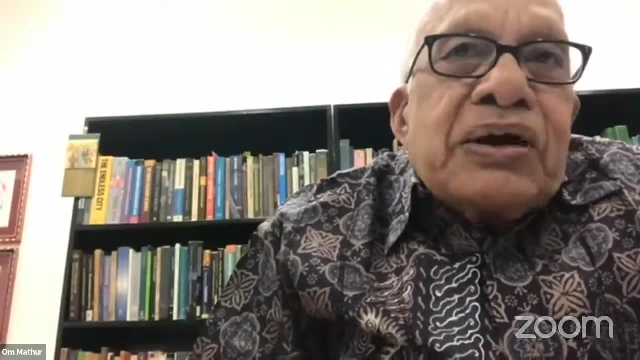 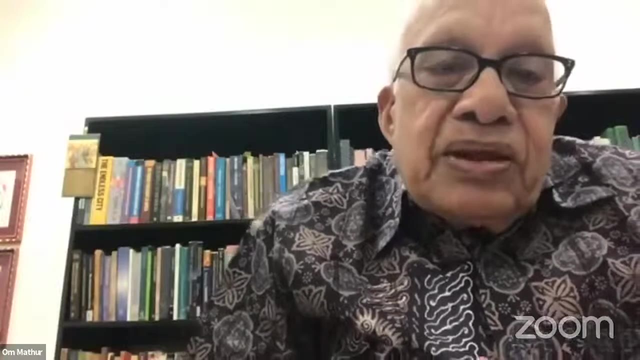 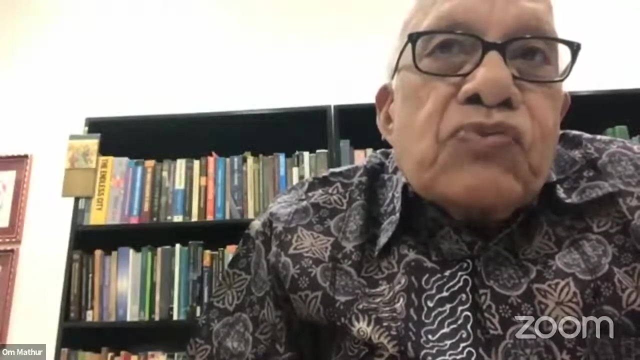 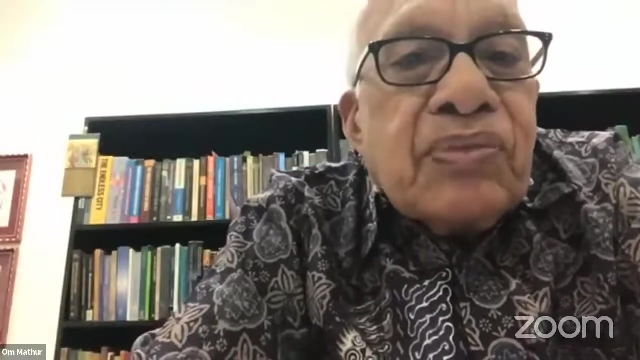 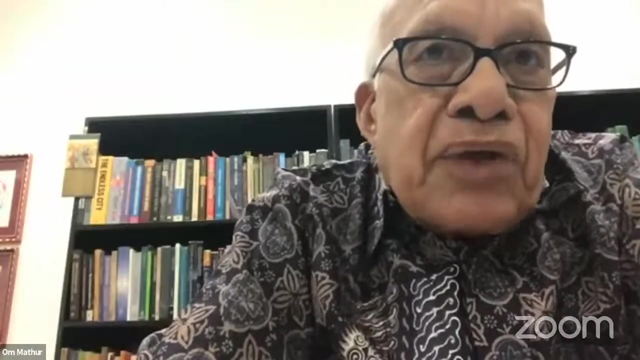 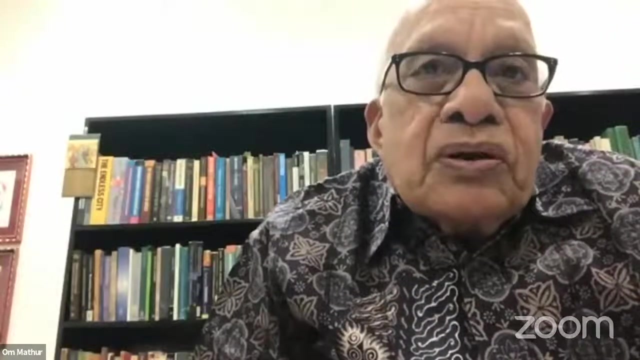 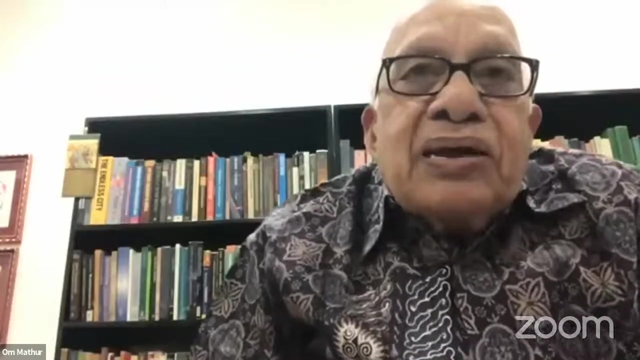 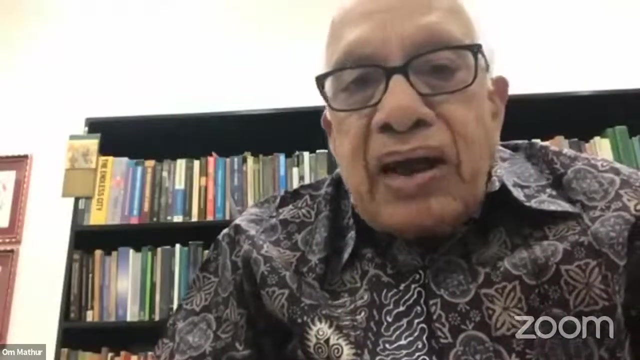 I think that the subject of this evening is particularly important, not for the reason that you mentioned but the fact that you're combining policy, practice and pedagogy in one discourse. This I think is a very novel idea. And normally what we do is that we confine ourselves to these fears of our own interest and specialization but really have the opportunity of discussing it in a framework that combines pedagogy, practice and policy. My remarks would deal with the policy issues with respect to urbanization and I will try not to deal with practices and pedagogy to the extent I can avoid them. Can you see them? I can't see anyone. We can see you. 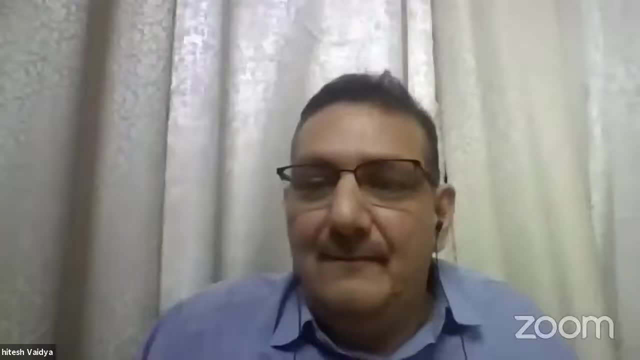 We can see you, sir. We can hear you properly. Sir, we can see you. 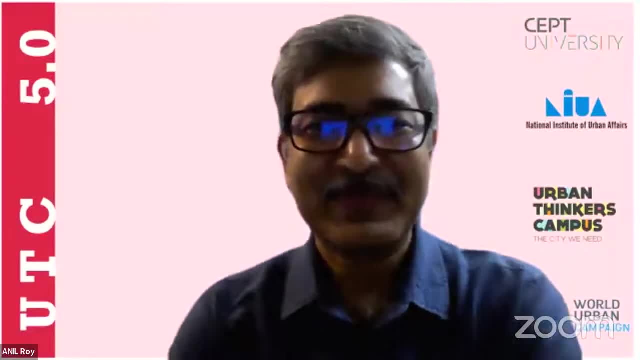 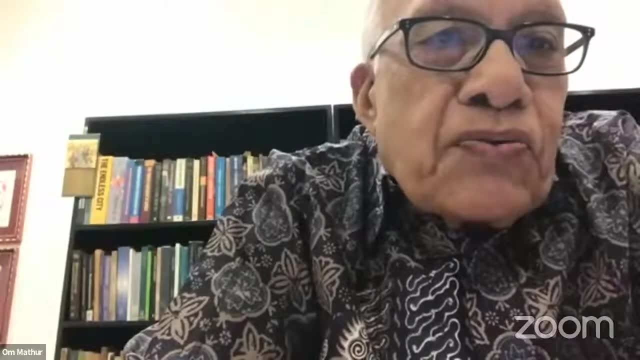 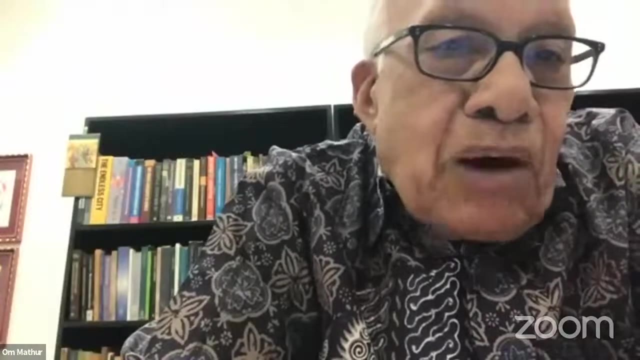 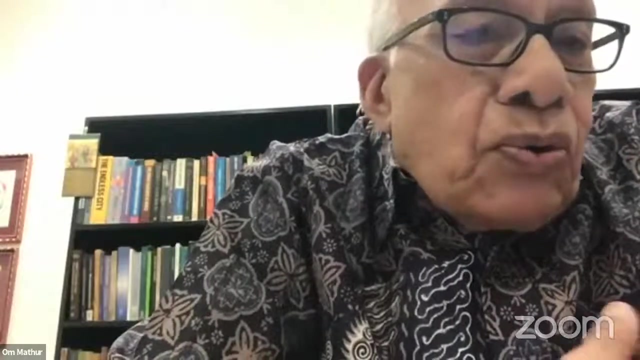 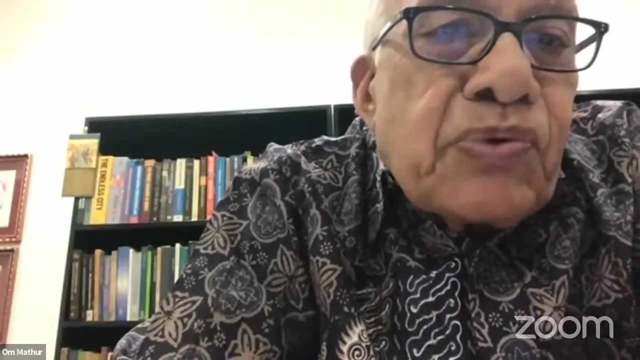 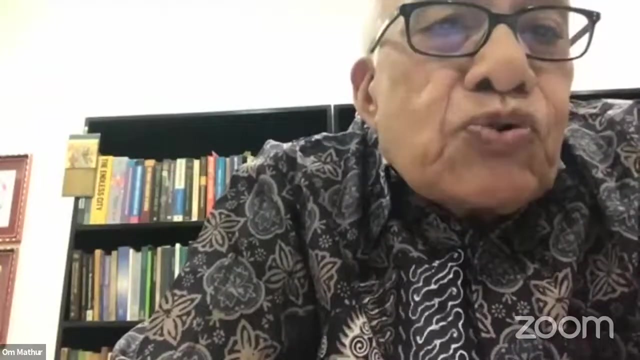 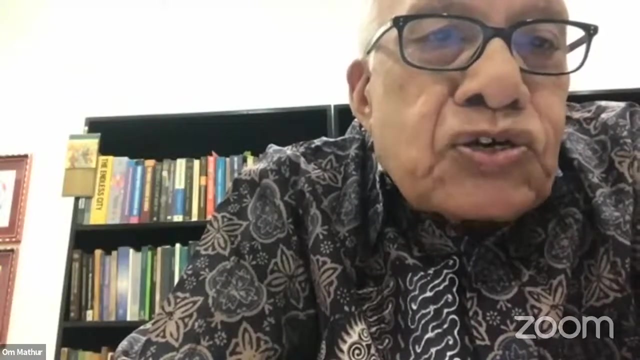 All right. From the concept note that all of you sent, I see that the trigger for the conference is really COVID-19. I see that the trigger for the conference is really COVID-19. I see that the really COVID-19. I see that the trigger for the conference is really COVID-19. I see that the during COVID-19. I see that the trigger for the conference is really COVID-19. I see that the size of the debate that the alphabetizes this language, including that the Money makes for us thinking that we have bona fide having economic power coming through and I see that from an early perspective we have only given off a lownightly 바$ if a million people pass through our 401 Facet goals and Shanghai have hidden private 들어였ъ period näm巧 period tut both infections as well as out-migration form in large cities and the inference that 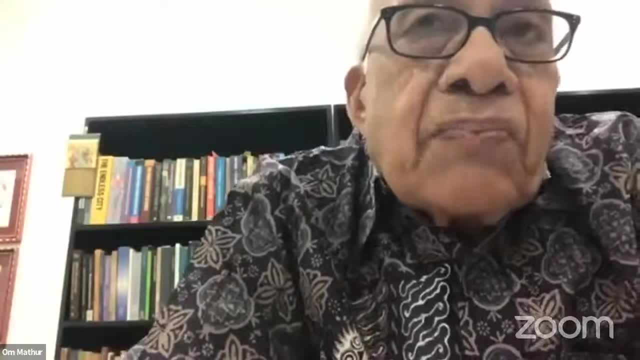 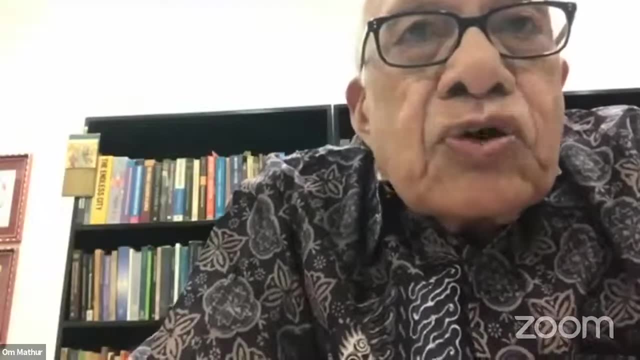 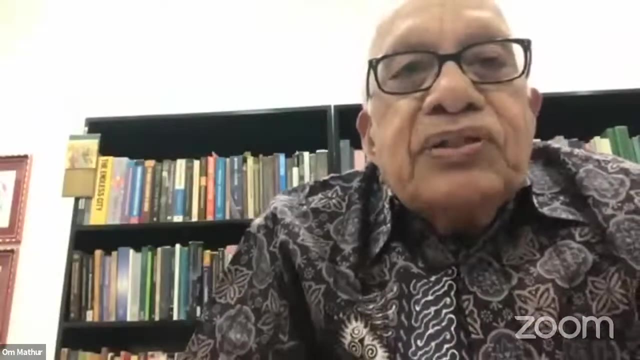 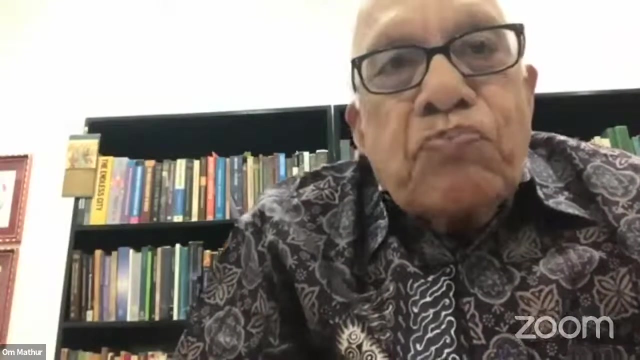 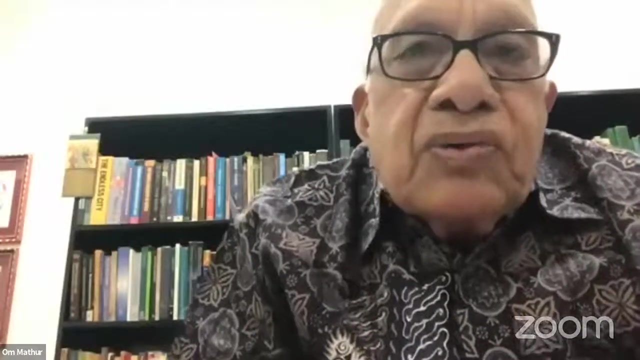 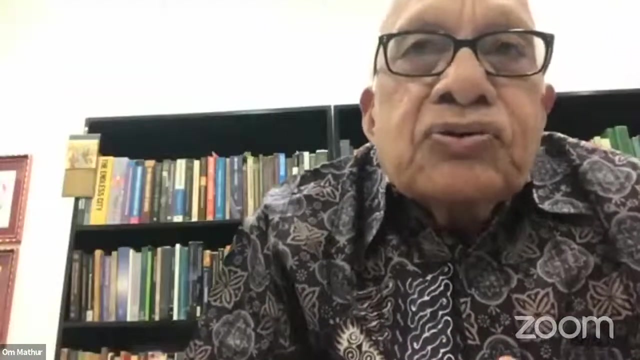 several analysts are trying to sort of draw from this phenomenon both of migration as well as concentration of infections in large cities is that large cities have become far too big and we need to work towards changing the size distribution of cities to a more balanced size distribution. They find that the present size distribution is not conducive to events such as the one that we have just gone through and we are going through, COVID-19 and the mass migration and it needs to be adjusted to the requirements that now confront us. 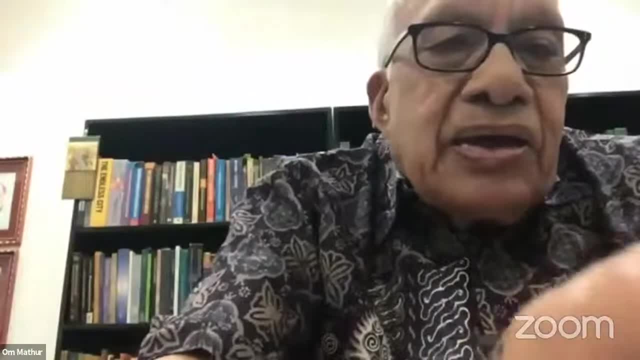 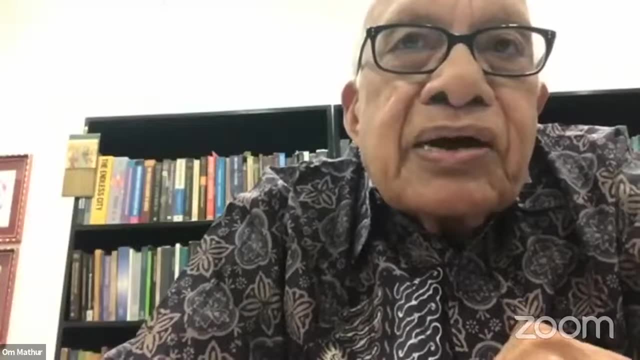 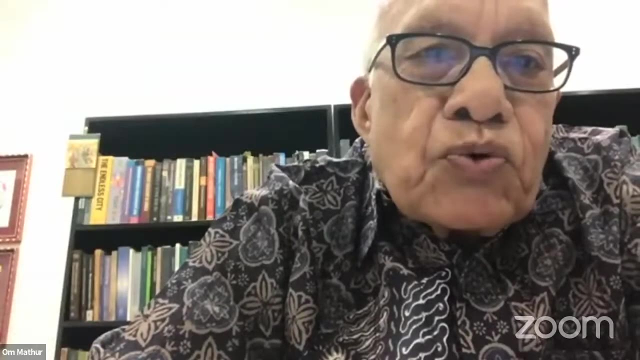 Irrespective of what Hitesh has said, my reading of the whole situation is that this inference that has been drawn that we need to revise the policy simply on account of COVID-19 and the mass migration that we have seen is somewhat misplaced, if not flawed. And I'm saying this for a number of reasons. 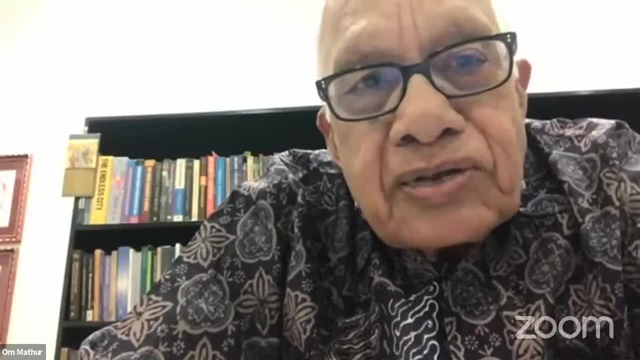 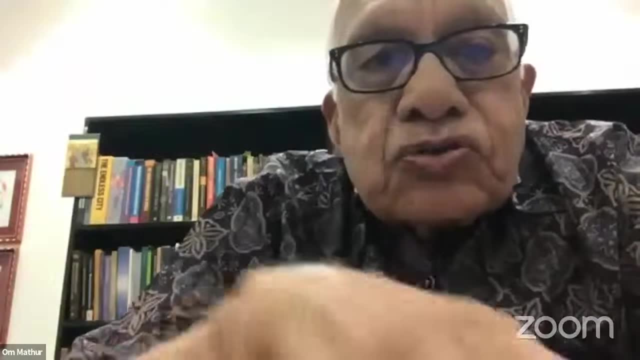 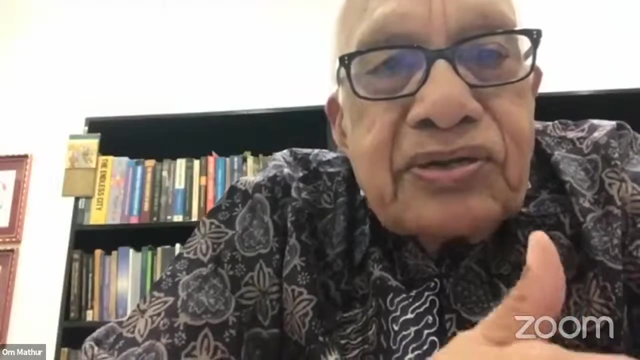 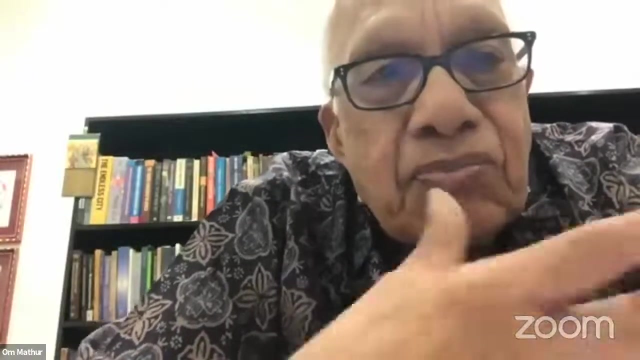 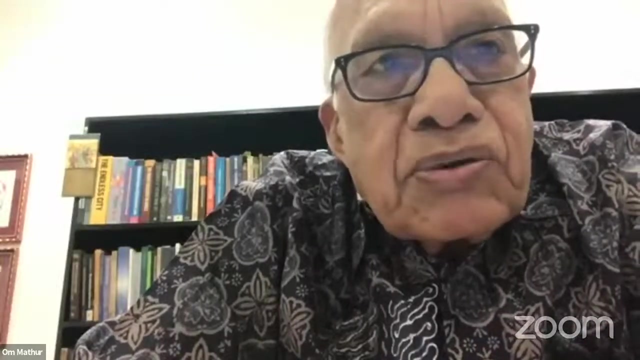 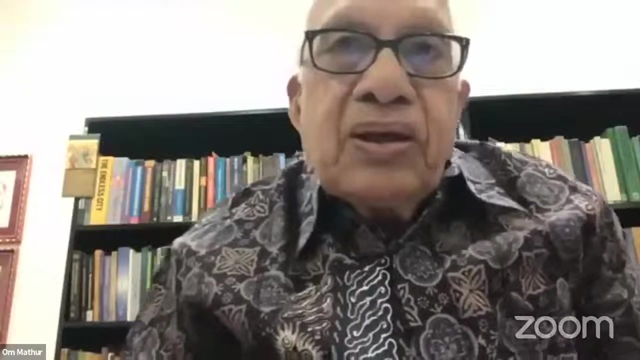 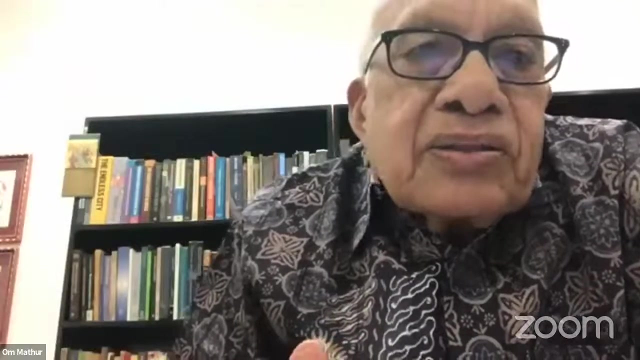 Number one, number one is that the determinants of size class distribution are far too strong to be affected by an event such as COVID-19. If I use a statistical term, COVID-19 and the mass migration are nothing else but one of those stochastic kind of an event, random event that has come in. It is having or people tend to believe that it is leaving very small area. We don't know the size of the event, especially as far as the mass of the event, that we have seen. But you know, it is a large scale impacts and long term effects. But there seems to be thinning out as we see from the limited data that keep coming in, into the print media. 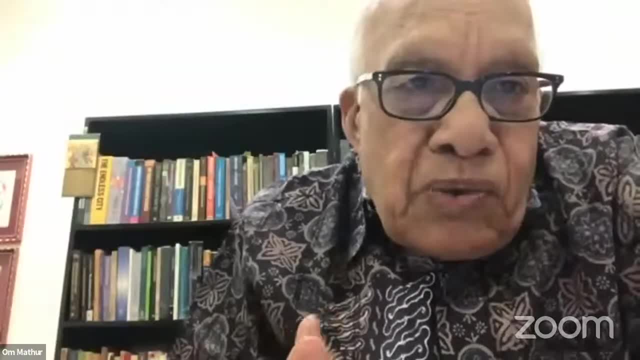 And that that evidence that is coming in, number one, there's a reverse migration already. This doesn't really take place. Number one. 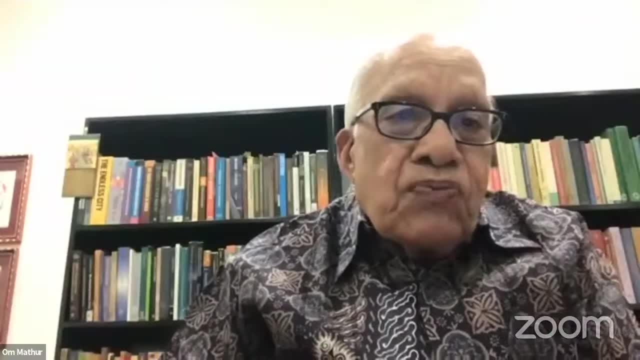 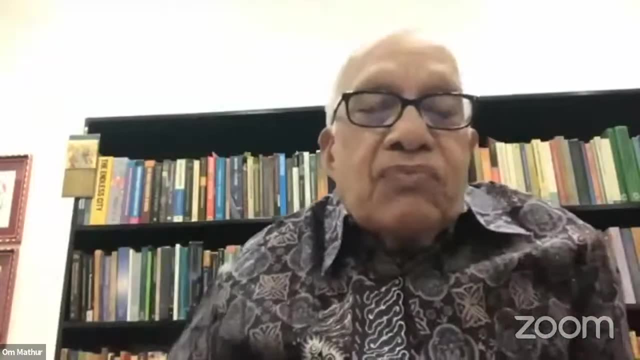 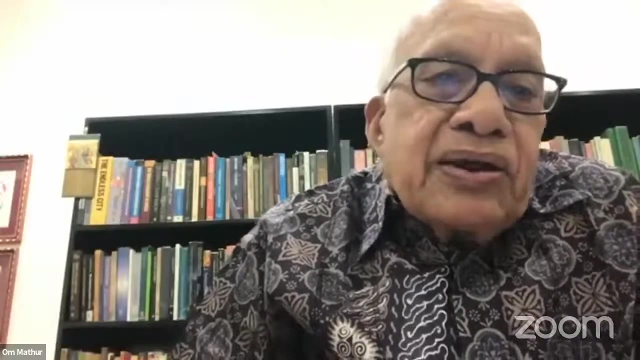 The second one is that there is a trickle down of infection from large cities to the American continent, as I said, not because of the rapid expansion of COVID. large cities to small cities and to their rural areas. So our original virtualization that it was confined to large cities and therefore the large cities should be dealt with and they are really, they need to be thinned out that probably does not hold good. 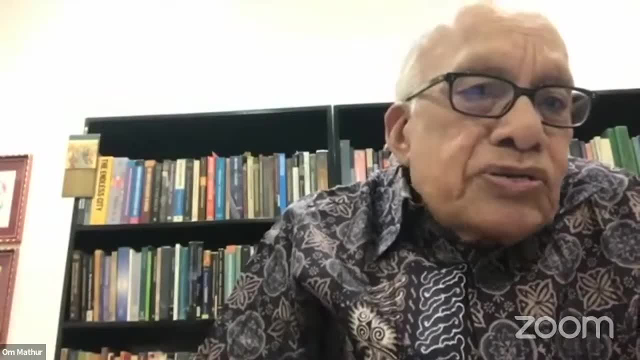 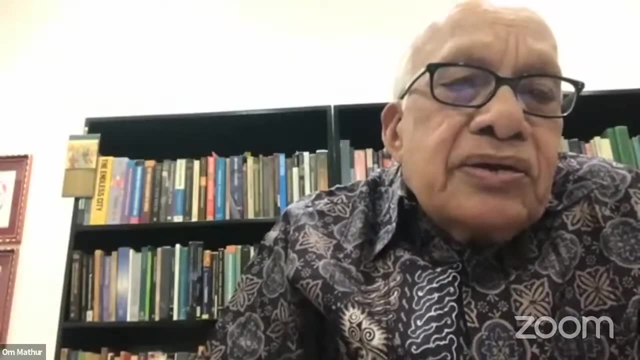 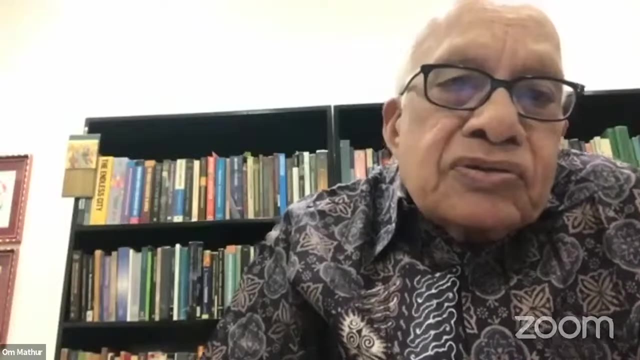 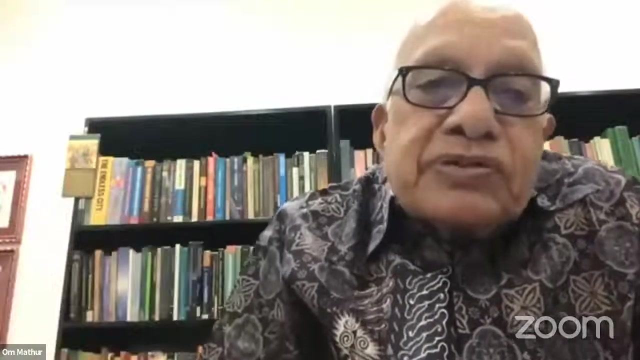 I think here, instead of changing the policy part, what's important is to change the practice here. My reading is that it does indicate some kind of a failure on our part to design the urban initiative, the urban practices. We have not been able to sort of design them to deal with such situations, such as the urban informal settlements, such as the tightening issue. In my reading is that if only our programs, initiative and practices had focused on urban informal settlements to begin with, the tightening issue, 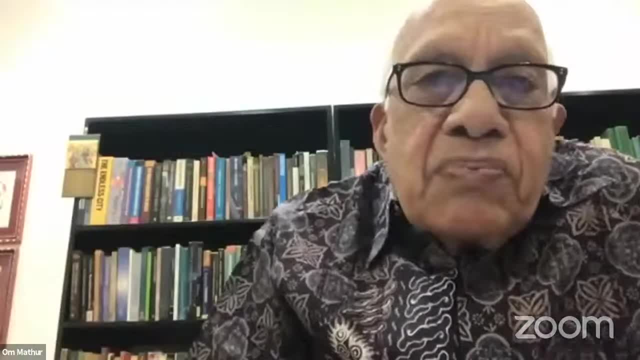 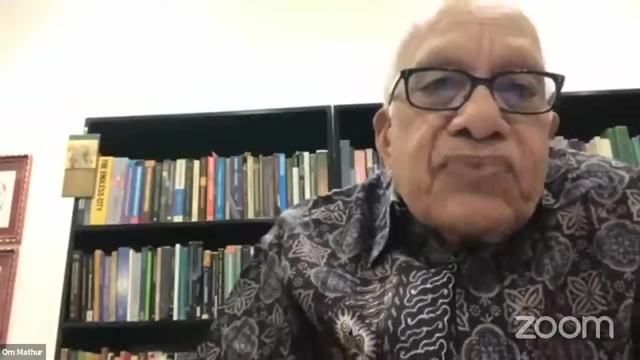 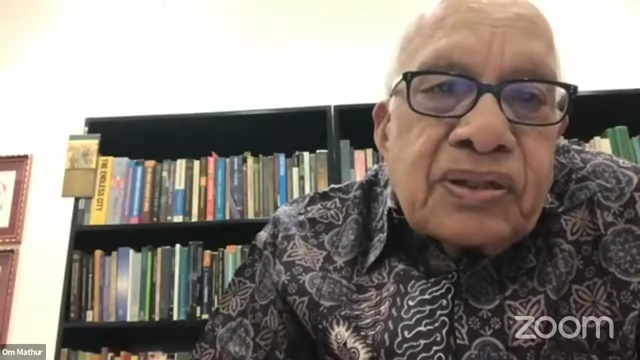 on the other hand, the labor, the temporary labor and the formal labor, if our programs had focused on them, then severity of the crisis that we have seen perhaps would have been far less than what we have seen over the past six months or so. 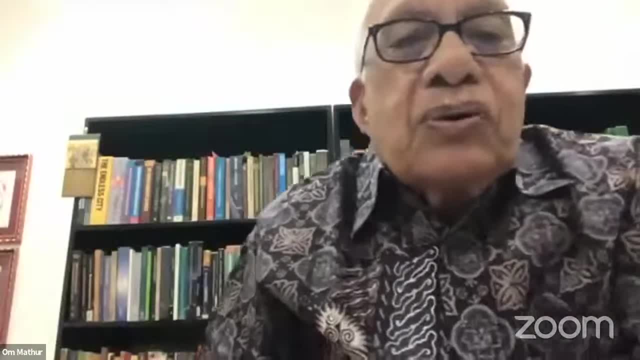 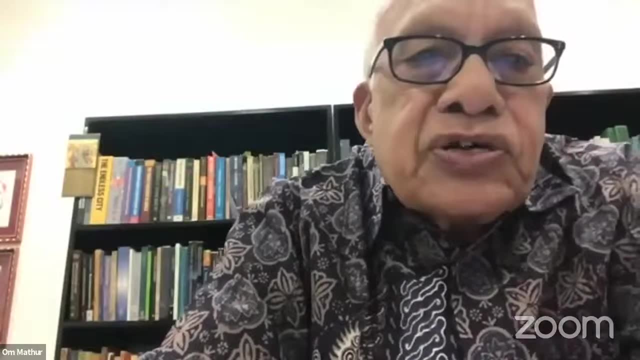 There is one point that I wanted to make. But let me make two larger points with respect to urban policy and I think that should really be the focus rather than being overshadowed by one single event, which is COVID-19. 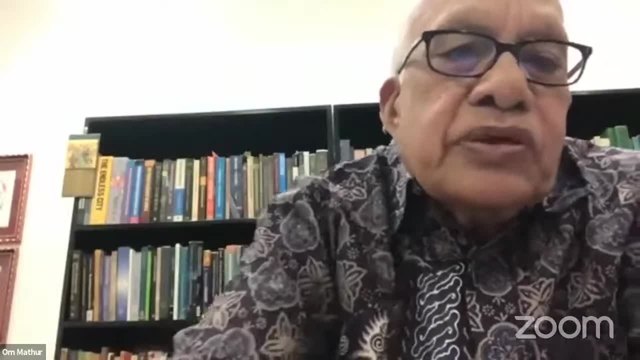 And I'm taking off from the concept note that you have mentioned. 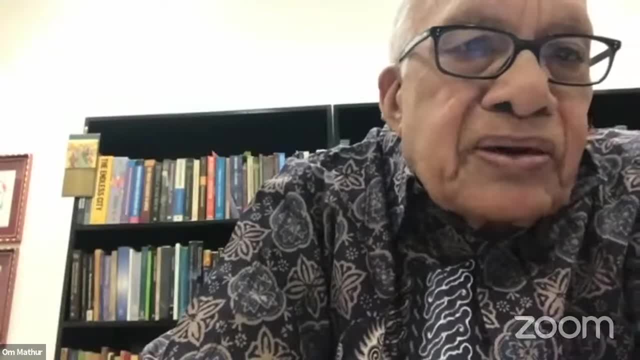 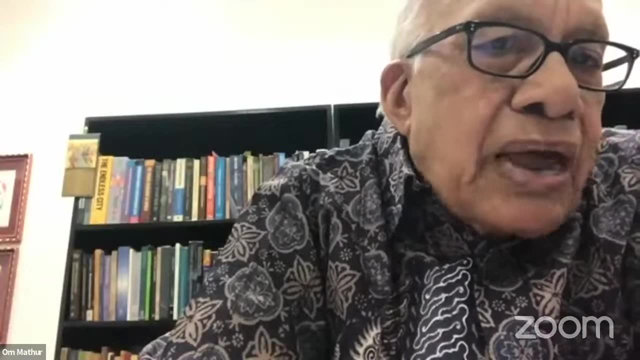 As you can see in India, I'm sure that all of you accept and as well as an IUA, the urban policies in India have been in a state, have historically been in a state of flux. 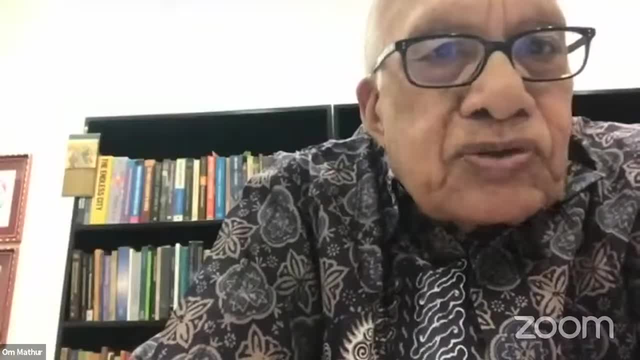 They've been changing over time. It's not like the US, 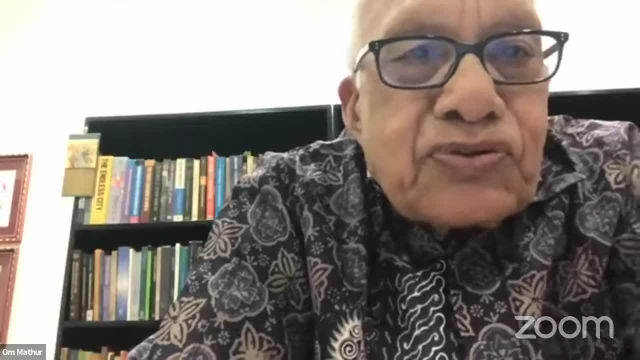 where you have an act that requires the president of the United States to submit to the Congress once in two years an urban policy report. It's not like that in India. 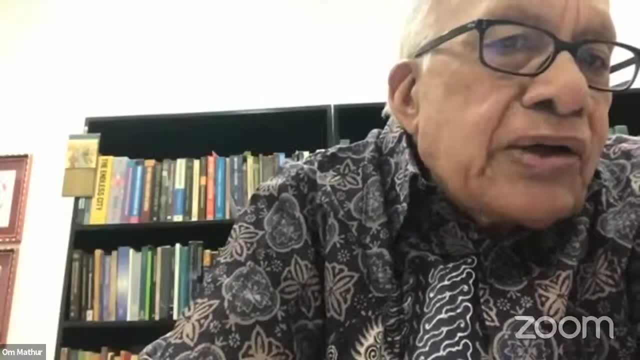 But we do have in India a mix of explicit and implicit urban policy. 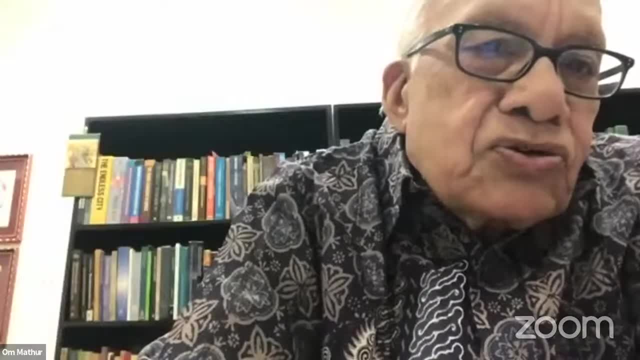 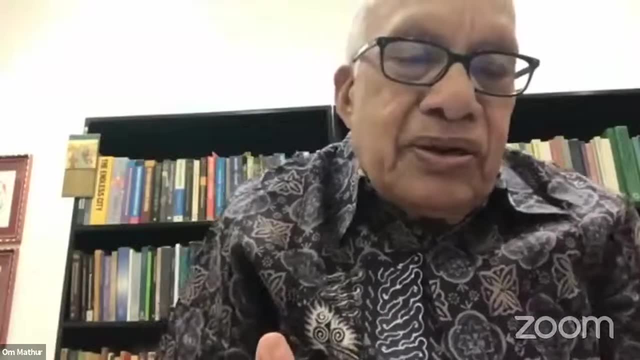 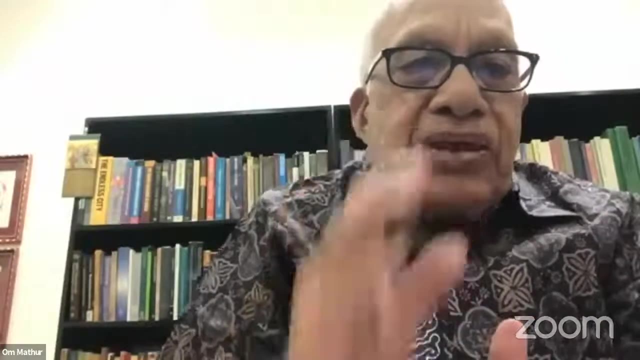 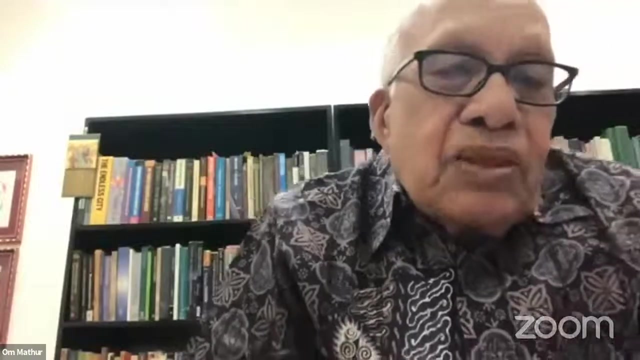 And if one really goes through the various documents, like the five year plans and so on and so forth, you will see that up to the seventh five year plan period, urban policies were based on equity considerations. There was a very clear statement in some of the plans that we should reduce the rate of urban rural to urban migration. We should reduce the growth of large cities and we should really focus on small cities and medium sized cities. 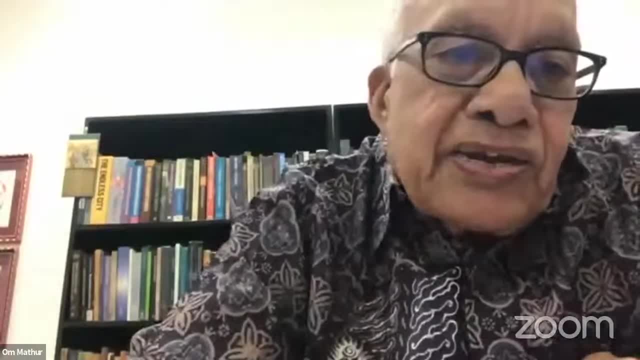 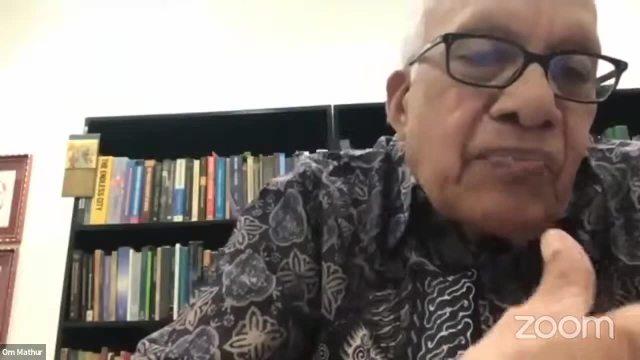 And that really led to the initiation of the IDSMT, EIUS, environmental improvement of slums, urban basic services and programs of that kind. 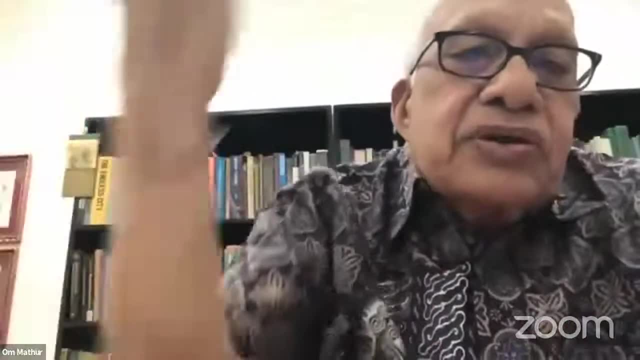 That was a dominant practice resulting from the policies which were really equity based considerations. 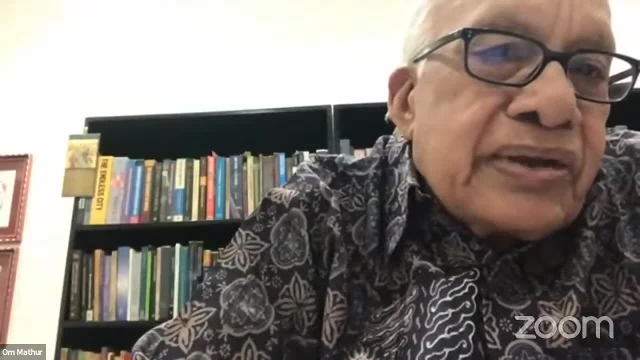 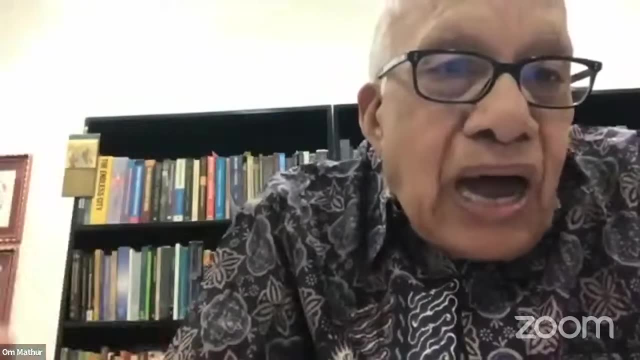 As we move forward and begin to see the connection between urbanization and economic growth, which we had not seen until then, our focus is starting to change. 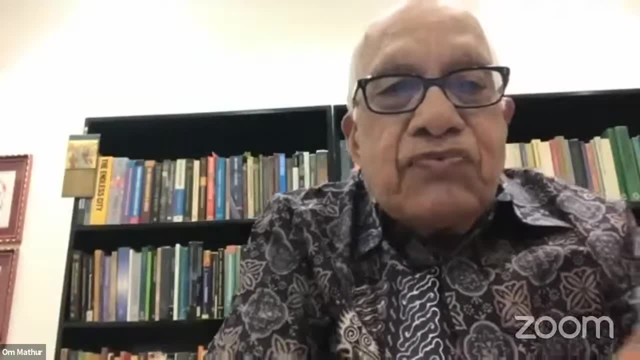 And from a small city and medium sized city, we moved on to mega cities. And programs that are the KNUR and many other similar programs. Now the shift is a very remarkable shift. 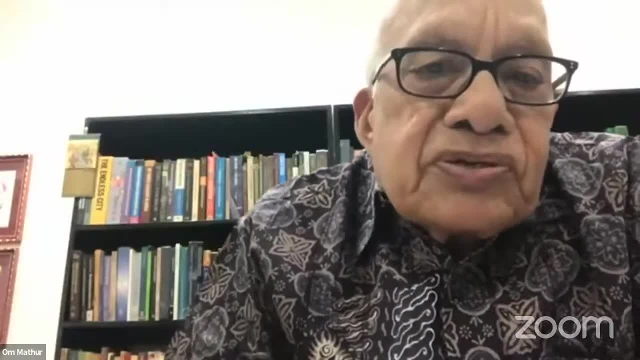 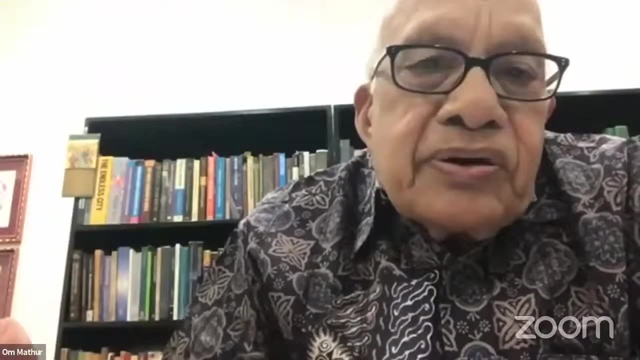 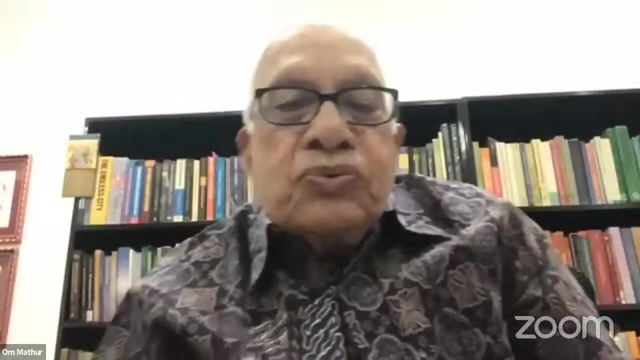 And the shift is really the outgrowth of a series of areas that were taking place between mid 80s and 90s, which included globalization, liberalization phenomenon, the FBI, the Indian markets were open to this one. 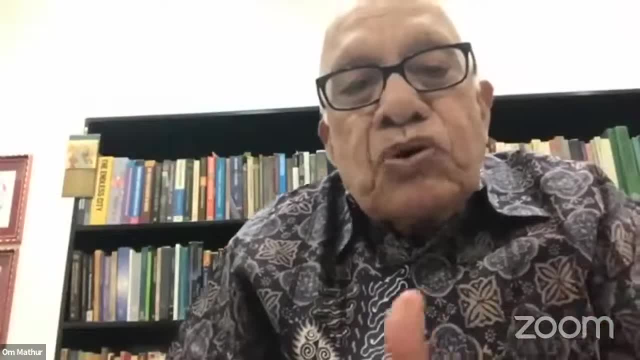 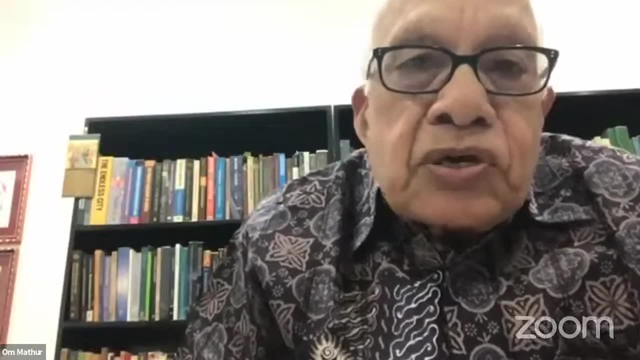 The import substitution being replaced by export debt growth, the open economy that all of these were changing our urban structures in very, very significant ways. If you see Noida, Gurgama, Bangalore, Hyderabad, New Bombay, they are all outgrowths in the sense of the changes that started taking place in the Indian economy right from 1985 onwards. right from 1985 onwards. 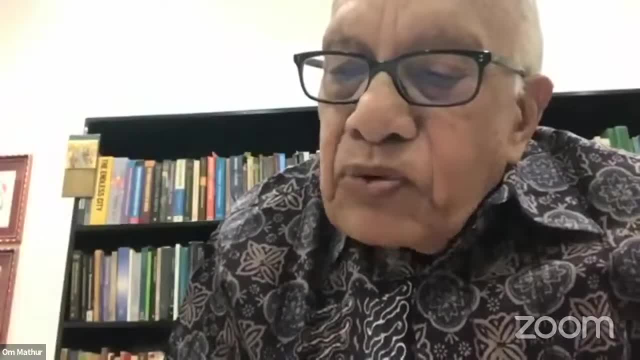 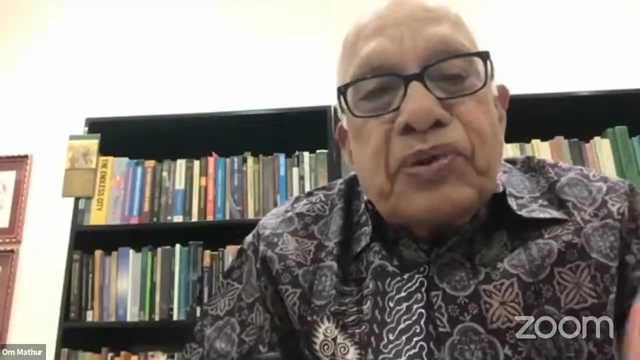 And we really came up with that point, new lexicon came into being that cities should be bankable, cities should be competitive, cities should be productive, cities should be efficient. 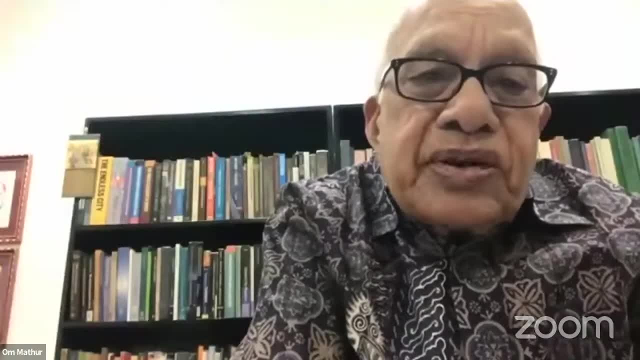 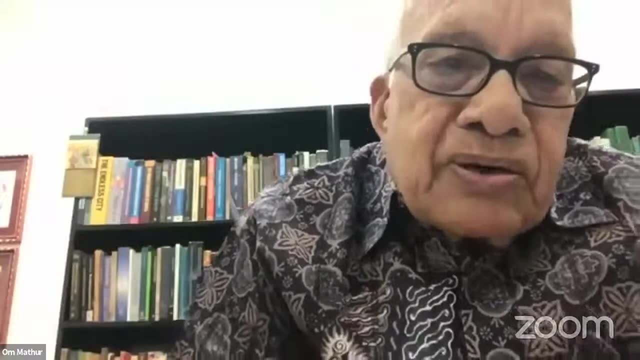 So from a state where emphasis used to be on equity consideration, the more dominant part of policy was to make cities more efficient, make cities more productive, more cities more competitive. 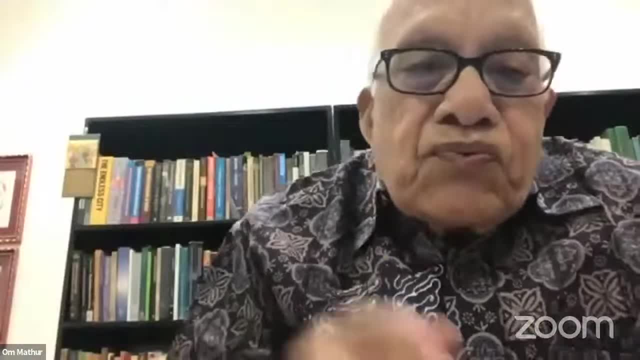 And then all of this was also it was certainly, we moved from a Hindu rate of growth 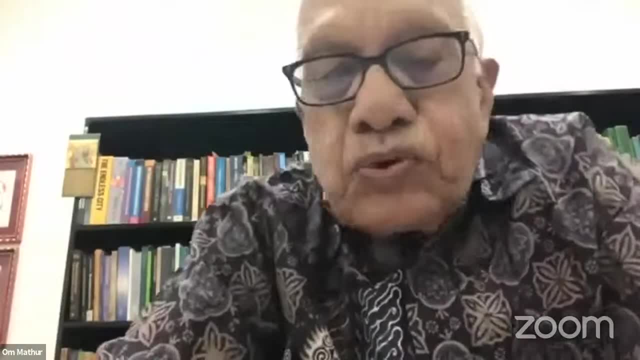 to a more progressive rate of growth of five to eight%. 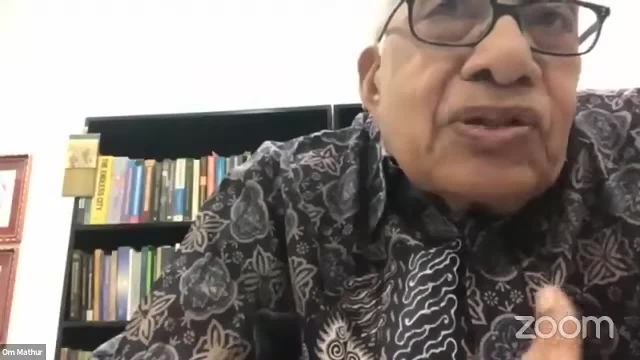 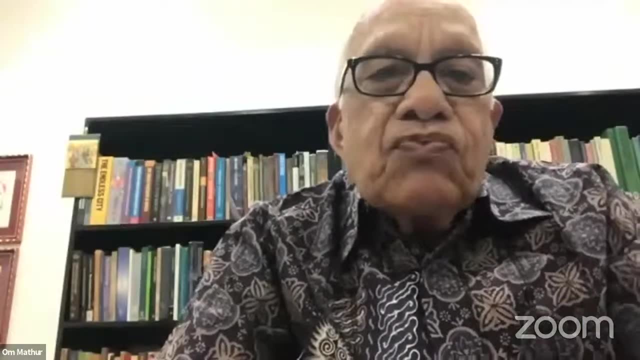 Now, very interestingly in this phase, we seem to be seeing urbanization reaching a kind of an inflection point. 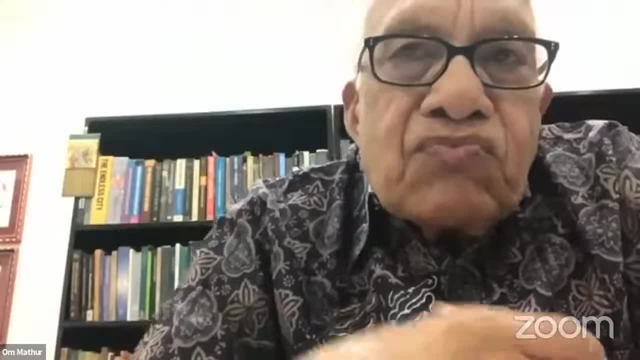 And it's reaching some kind of an inflection point on the counter. 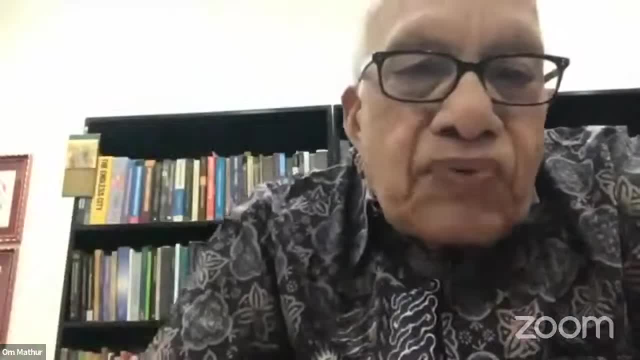 Once again, the new benchmarks coming in to which a reference had been made in the concept note. 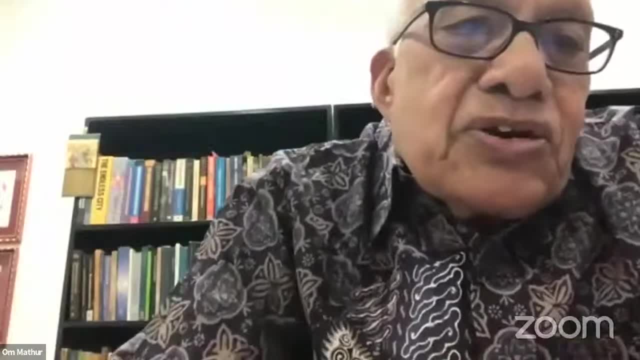 We are seeing SGT11, we are seeing climate change issues. We're talking about reducing our resource use per capita. 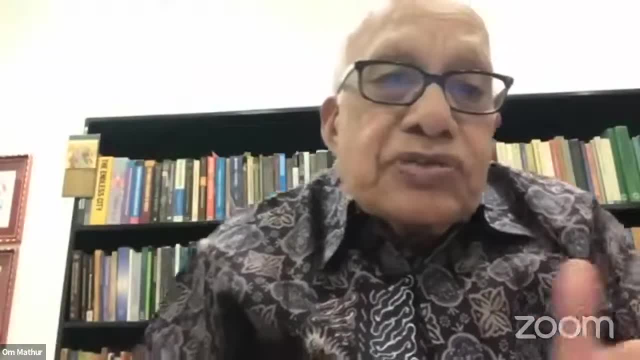 We are also witnessing, as I mentioned initially, very interesting phenomenon, which is cloud platforms, 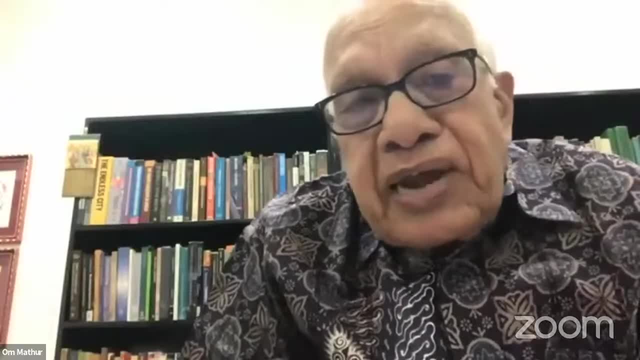 the AI, we are beginning to see the digitization and it's all the impact. 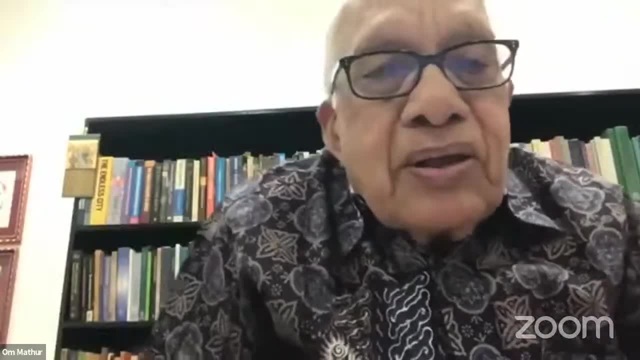 There's hardly any activity which is not defined in terms of particularly the digital technologies. 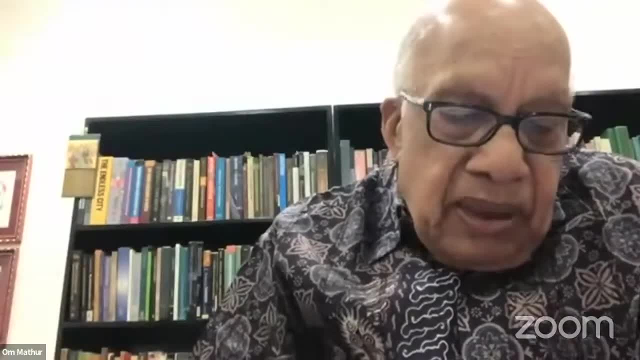 I do not know whether Hitesh you saw the article by our vice chairman of the NITIIO. 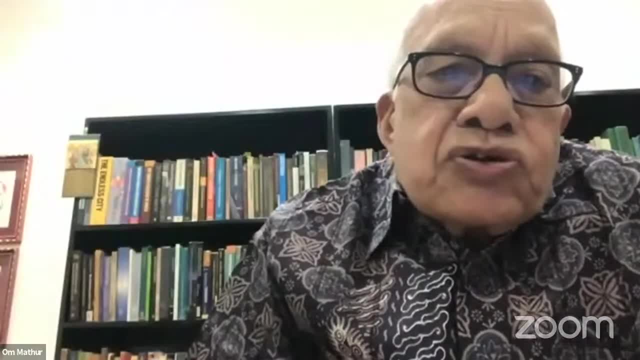 His reading is that digitization and cloud platform will make agglomeration economies, 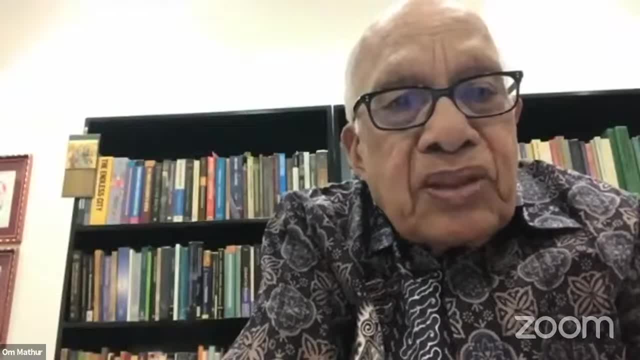 which is the central point of cities being productive and un-necessary. 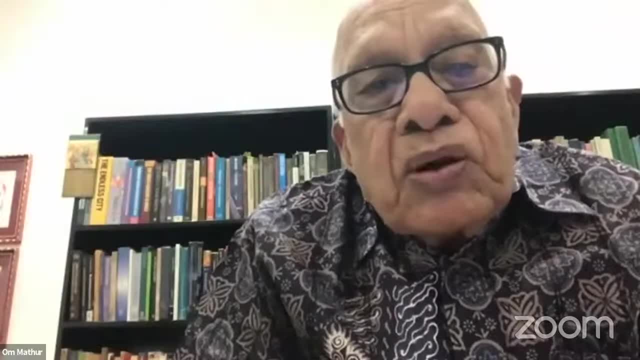 And that's the position that he's saying that digitization would make it unnecessary for people to agglomerate, will make it unnecessary for funds to come together and get advantage of intercity economies 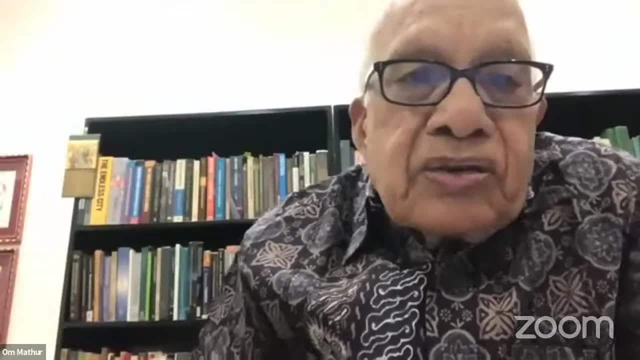 that we think are absolutely critical for cities to be very productive. 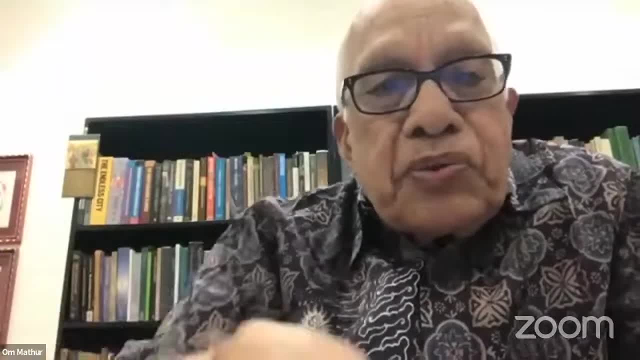 So we are reaching a point where we need to re-examine, not just in the context of COVID-19, I think, whether we like it or not, it's... 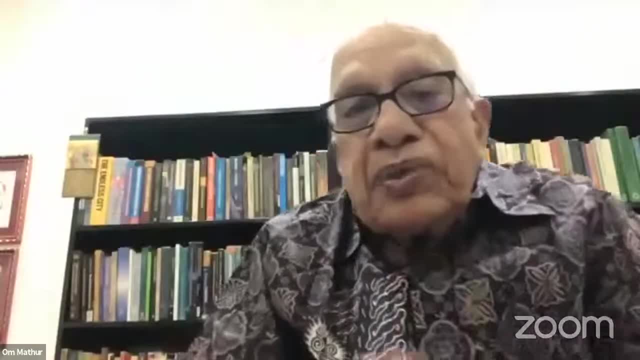 long-term impacts are not likely to be sustained. 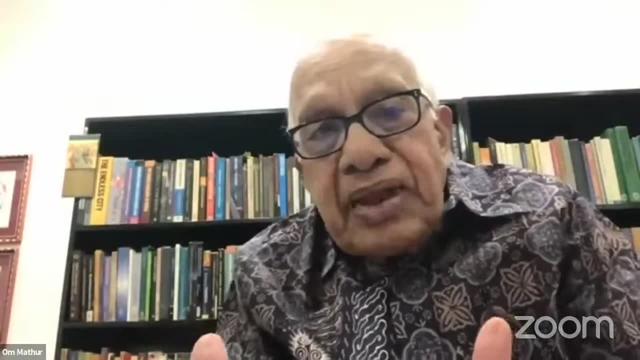 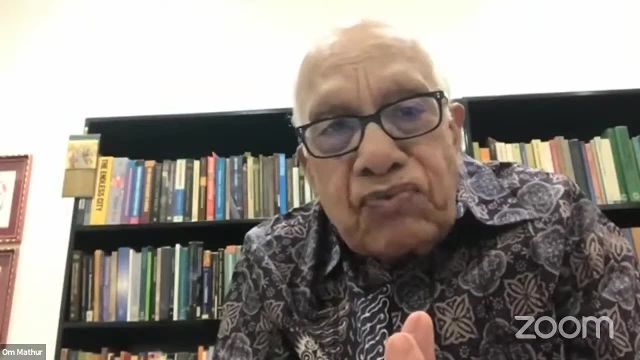 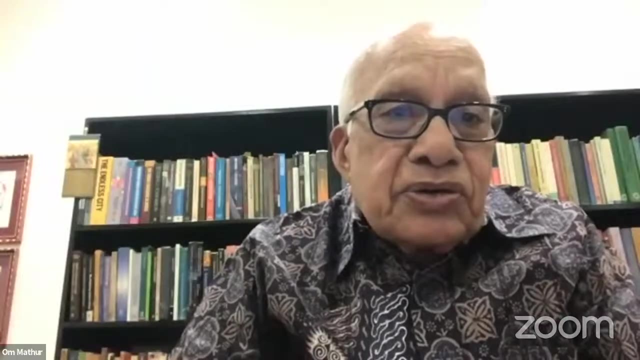 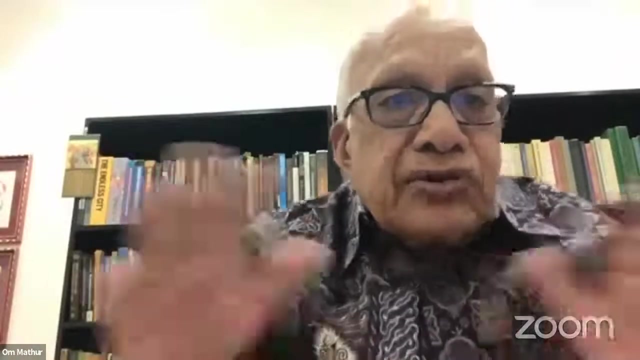 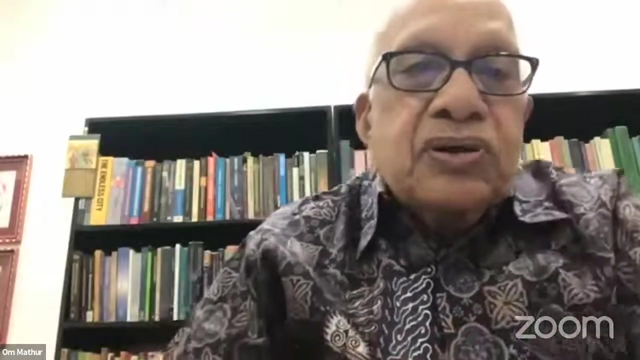 But certainly in the light of what is now happening, that if our cities were to be sustainable, if our cities to be resilient, if our cities to be inclusive or livable, if our cities to be simultaneously productive, what kind of equation needs to be written for optimizing the role of urbanization in the context of new emerging goals? That really becomes the more important policy issue that we need to be examining in the current context, rather than bogged down with only COVID-19 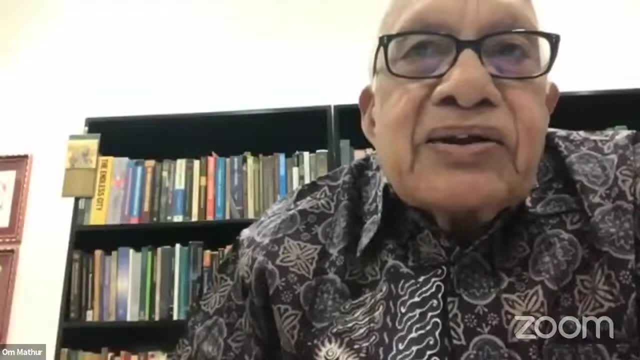 and its possible effects. I'm not saying that that is not taken away, that certainly has retrofitted all of us. 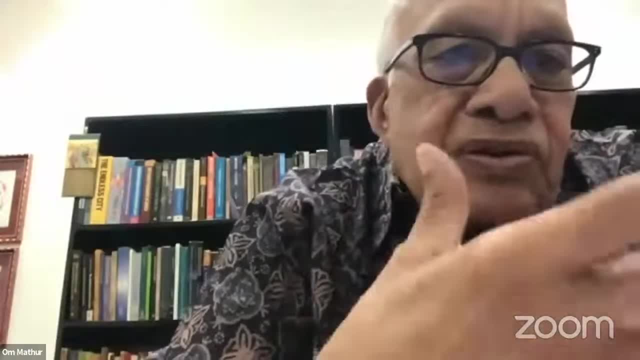 And some of the examples that you gave, working from home and its impact on the whole space use, 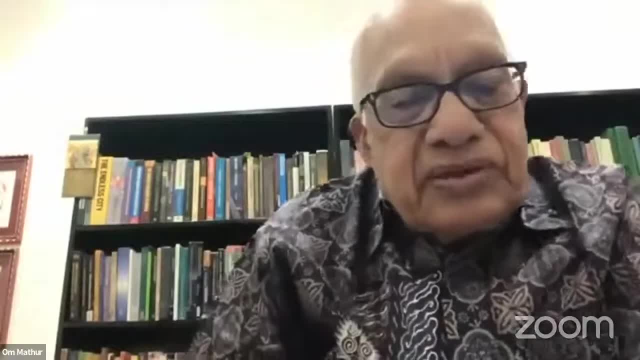 it becomes a part of the challenge that we need to face. 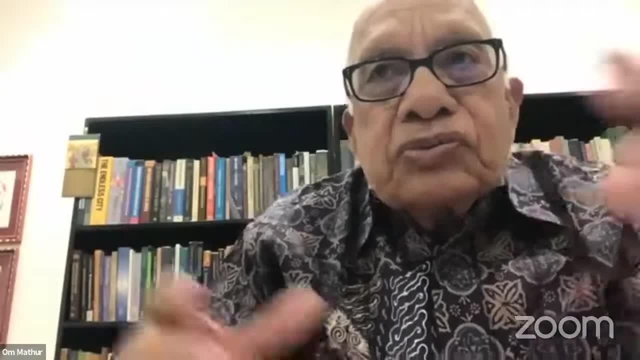 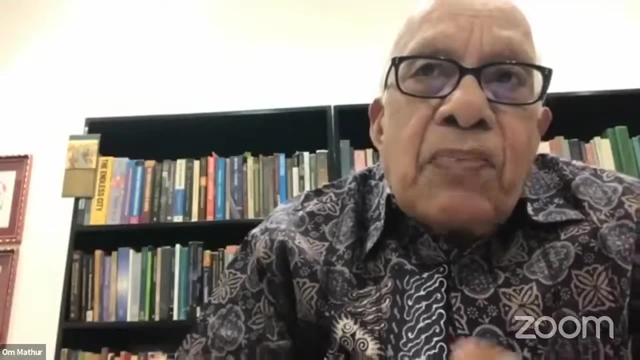 In, you know, if I sort of begin to see, if we put all of these things together, the impression that I'm getting is, apart from this new equation 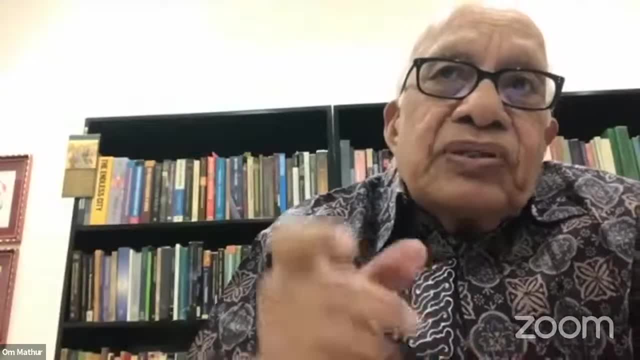 that we definitely have to write, we need to weigh very clearly where the payoffs are 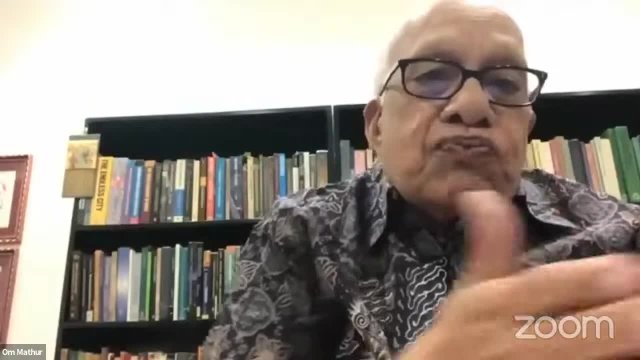 with respect to one, that world is flat. 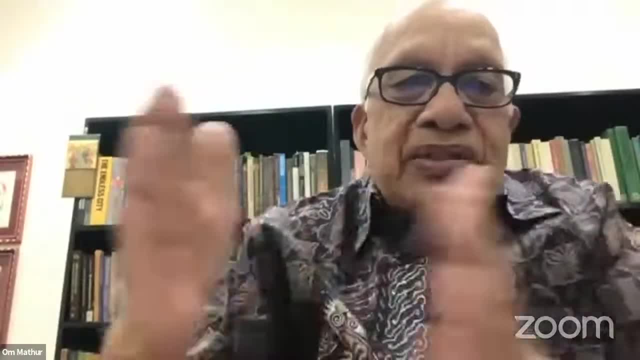 The Freedmen sort of thing, the world is flat, whether you locate it here, whether you locate it here, or whether you locate it here, they all give you the same benefits. 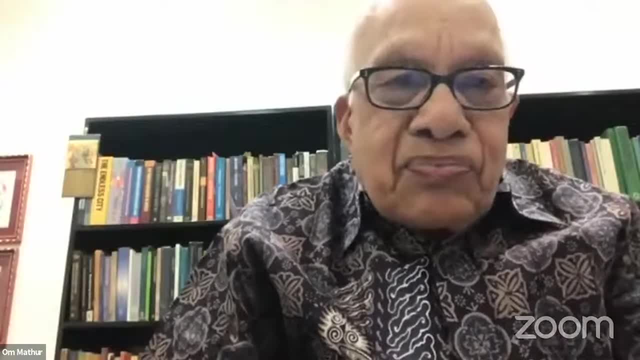 That's one kind of a scenario that Freedmen sort of brought in quite a few years ago, the world is flat. 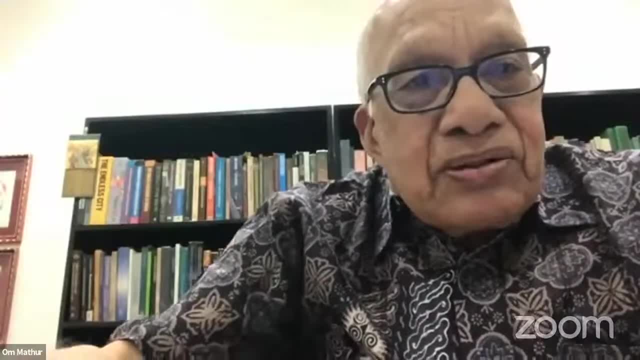 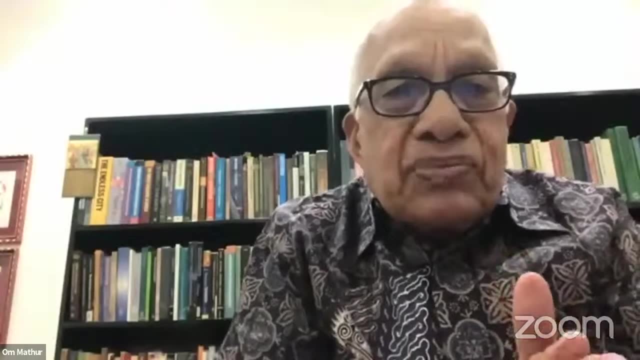 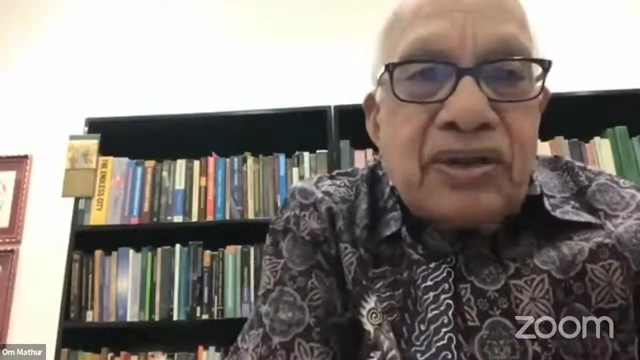 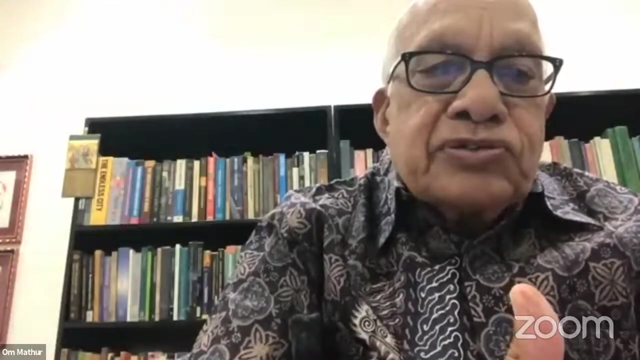 The second one is, no, it's not flat, but geography matters. Locations are still important. Now, the debate seems to be, beginning to come in the forefront, that what side are we taking? Are we working on a premise that world is flat, given that digitization is taking over, given that we have new international benchmarks, or where it's still in the framework 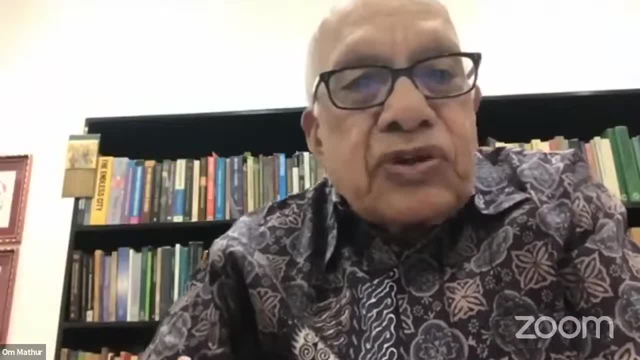 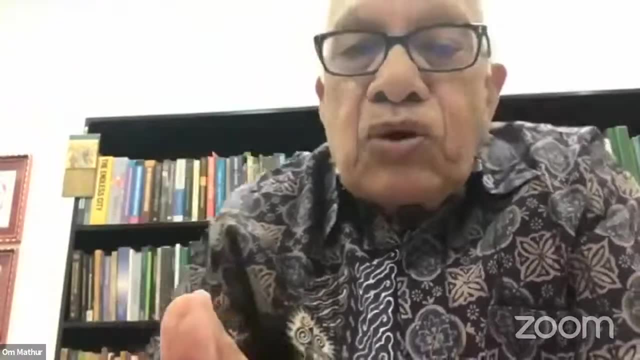 where agglomeration is still important, where geographies is still important and some location will continue to be important, irrespective of what we think. 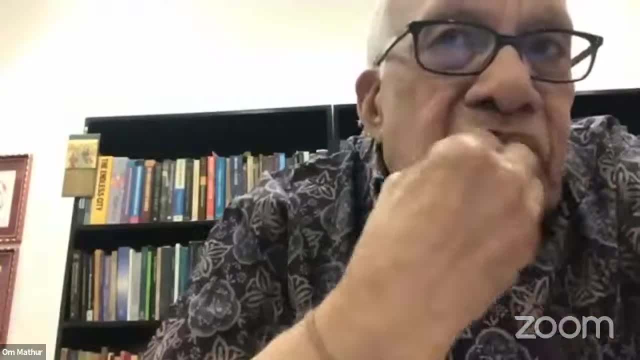 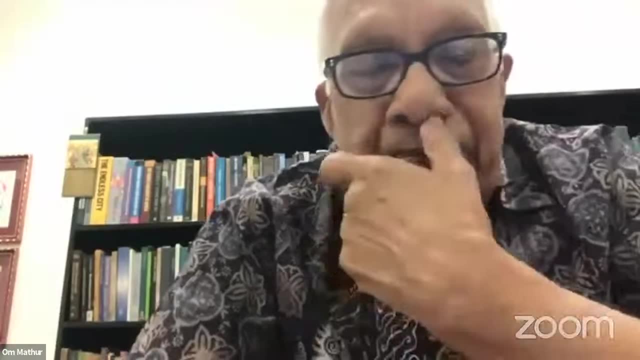 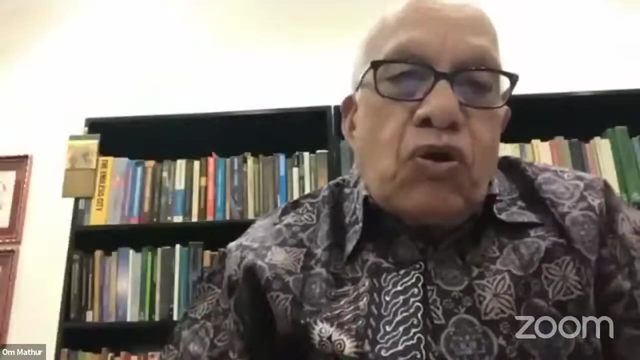 This really brings to me, reminds me of a colleague of mine when I was working in the UN system. His name was Benjamin Higgins, a Canadian urban economist who really talked about the dualism in technology and so on and so forth. 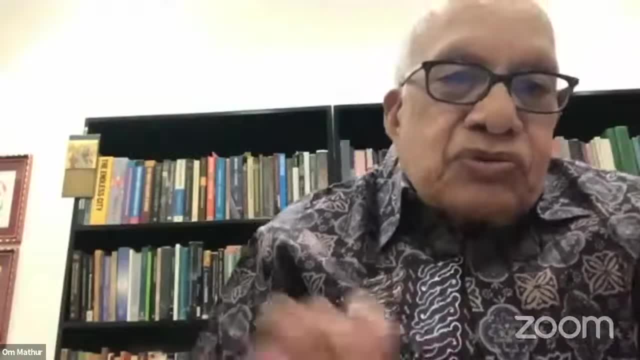 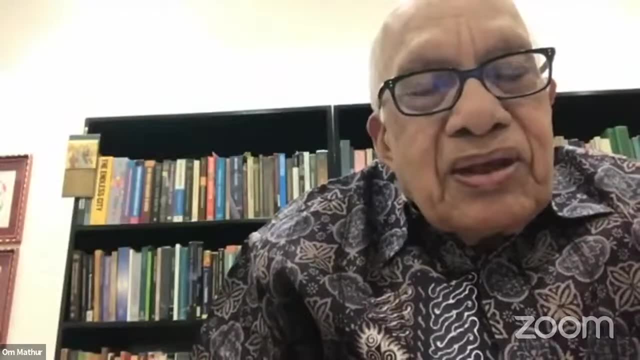 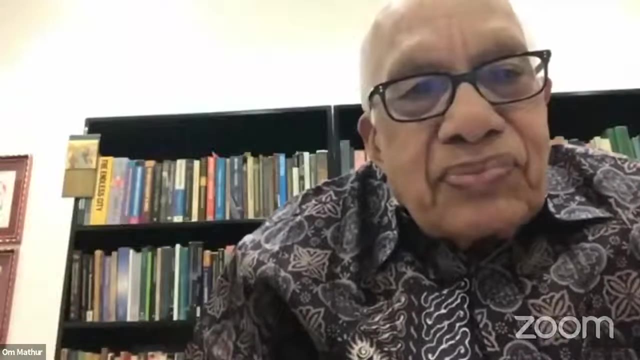 In those days, in the 60s and 70s, this kind of dualism was the central set, one of the central subjects to get from. He used to tell me that the only, the crux of urban planning, urbanization, and city planning, 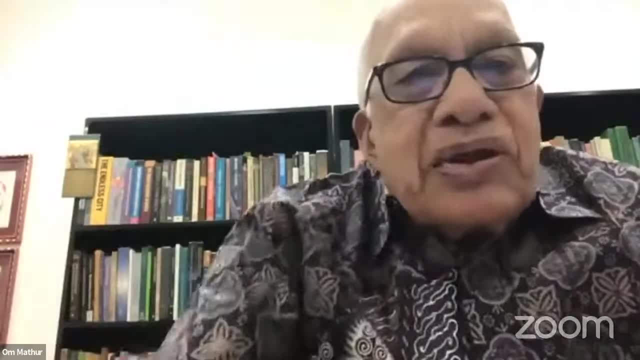 it is not just science as you people tend to believe. 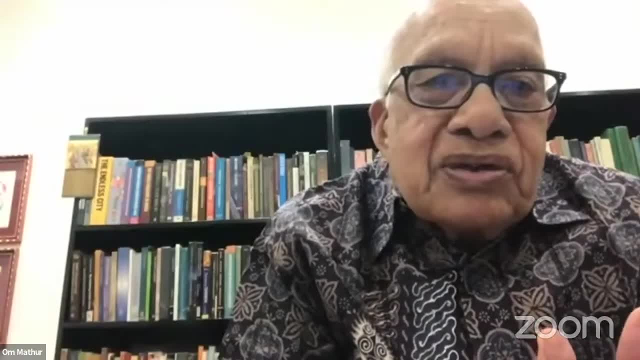 As we normally think that writing an equation will really deliver us the optimal solution. 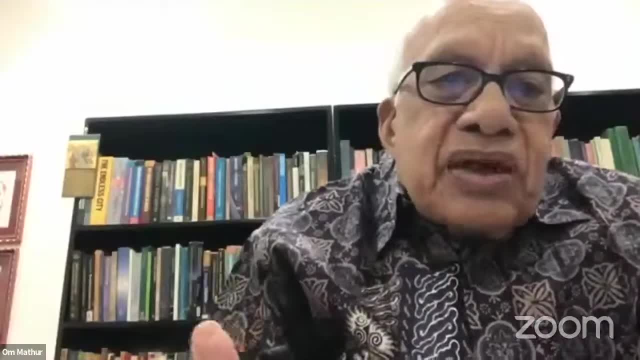 He said, look, you are entirely wrong. It is as much as science as an art. 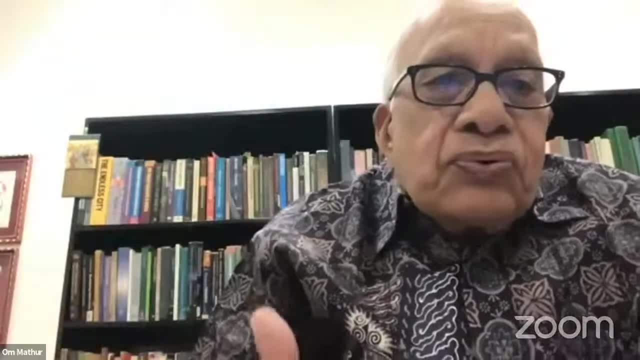 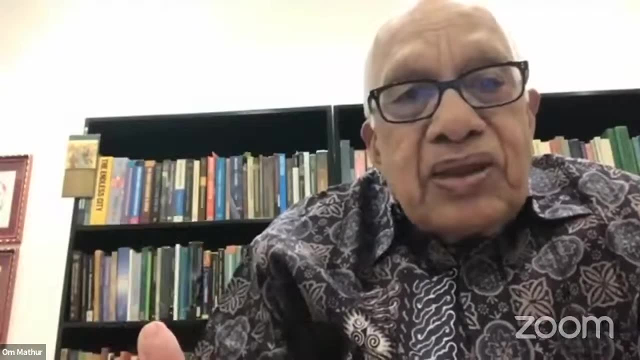 It is as much an art as a philosophy. And therefore, you would need to deal with urbanization, urban planning, city planning, as an art, as a science, as a philosophy. 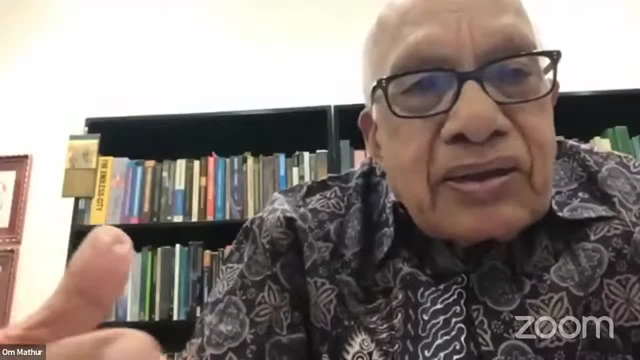 And you will begin to see the new light coming in. It will begin to, it will begin to look in that kind of frame. 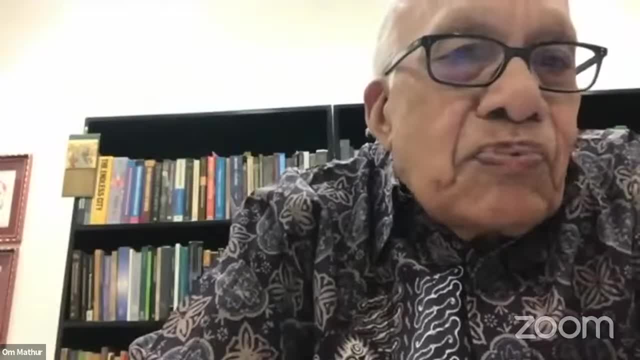 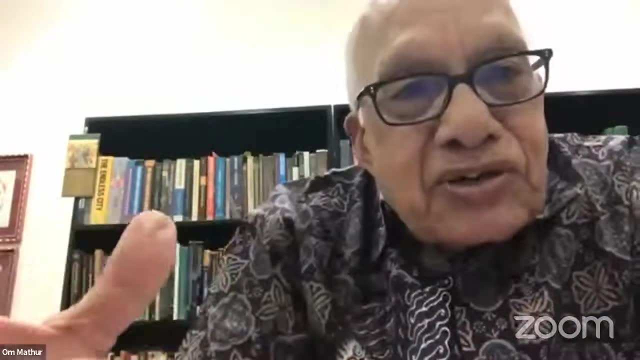 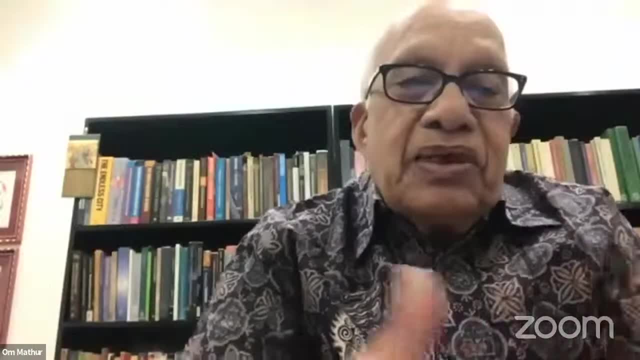 Where several disciplines contribute to it. Economics contribute to it. Sociology contribute to it. 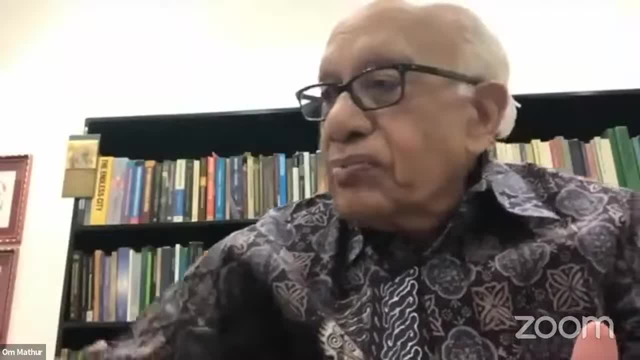 Political science contributes to it. Geography contributes to it. So a very large number of disciplines, 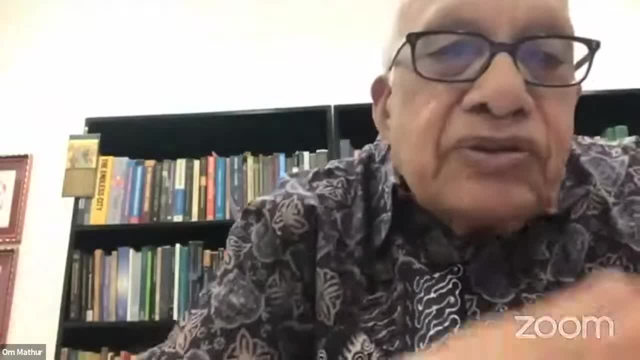 and therefore it is a product of a polygamous marriage. 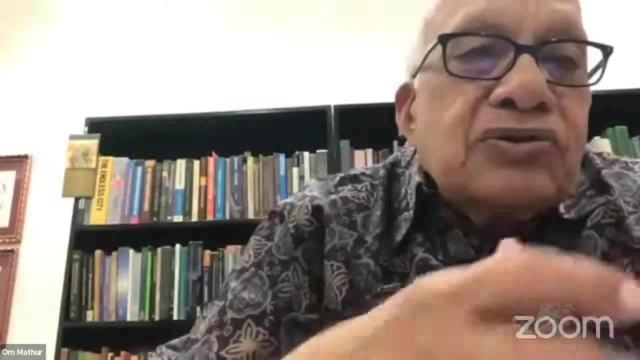 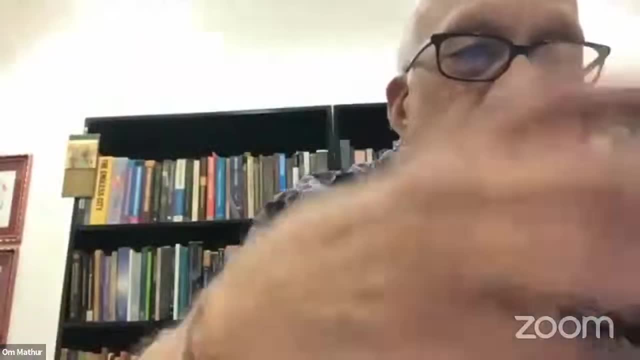 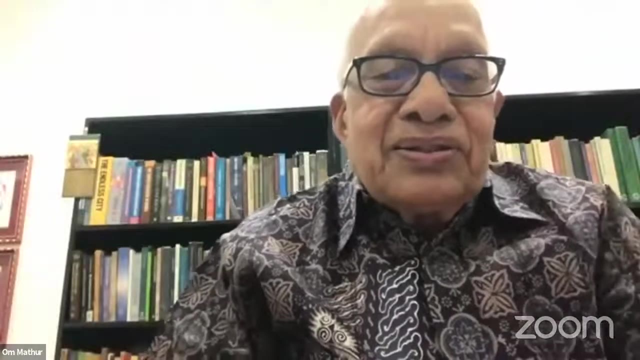 And you do need to recognize that you can't say, that you can't say that what I've said as a columnist, weighs more than what a social planner, or what a geographer, or what, as Hitesh said, is the training in the Netherlands provided. 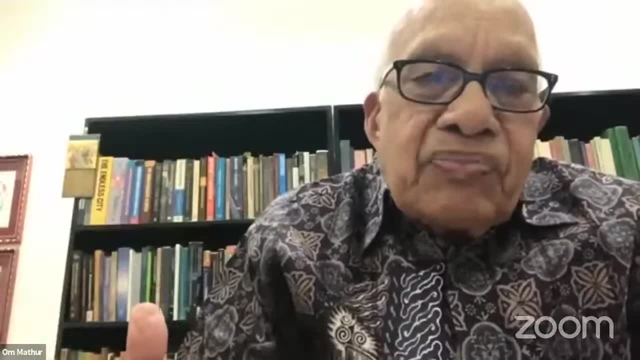 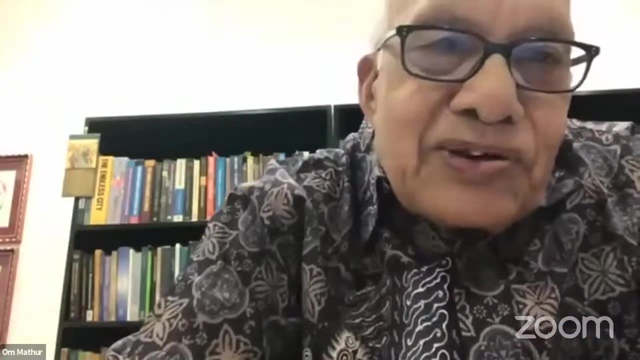 So one really needs to know where we stand. And what I understand is that Hitesh is currently working on an urban policy. And that's why I said it's a very good subject for me to talk about. 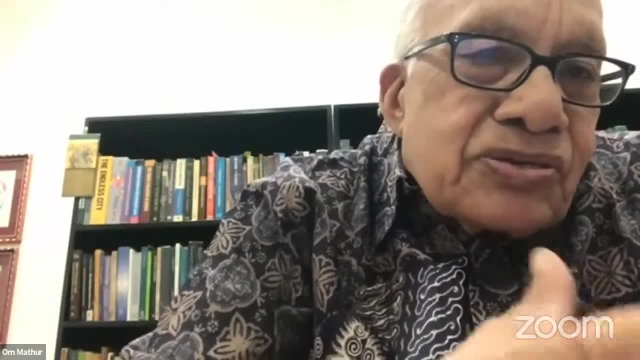 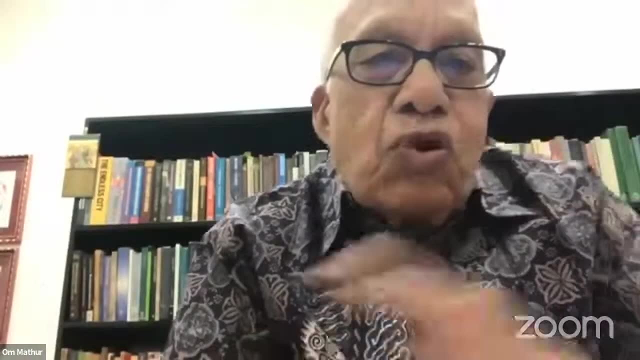 I think evidence-based research is absolutely critical for framing an urban policy. It is not just what some of us have been doing in the IEO these days, 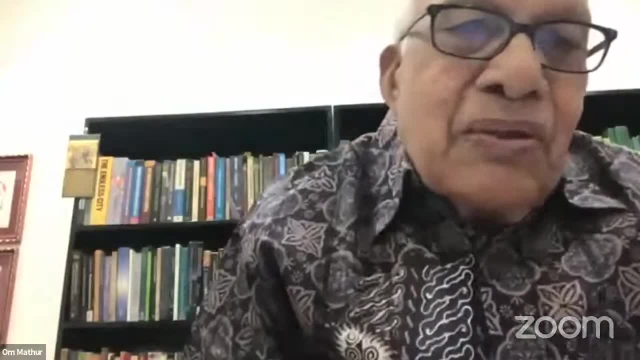 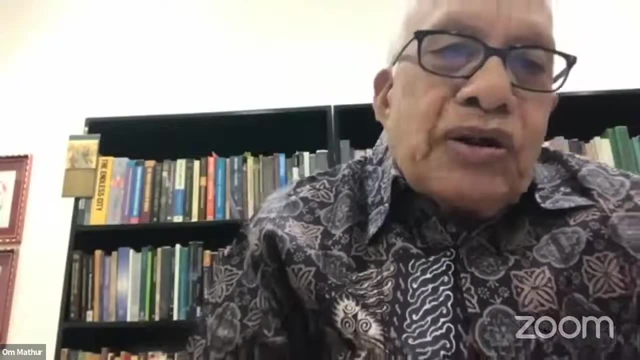 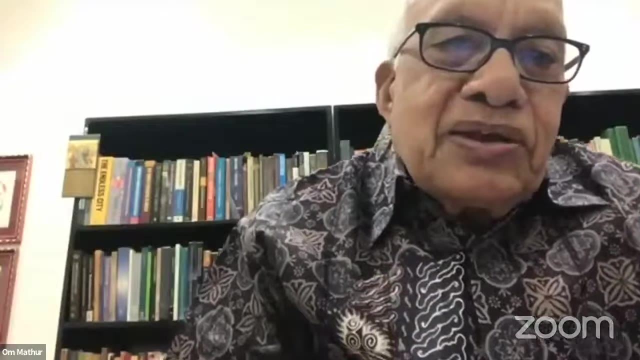 where, you know, you prepare some kind of draft, and, you know, you key your, you know, your urban policy to the $5 trillion economy by the year 2022, or a lower middle-income country that India will be by the year 2035, 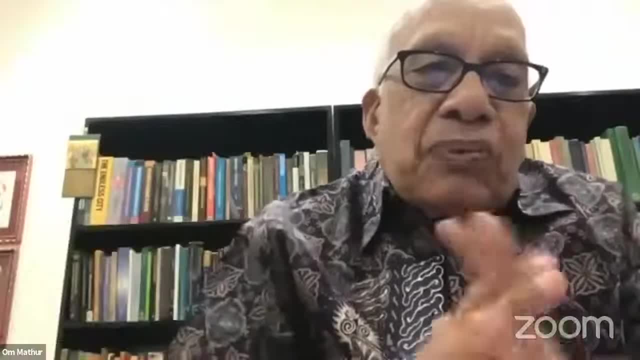 or a developed country by the year 2047, when we become 100 years old. 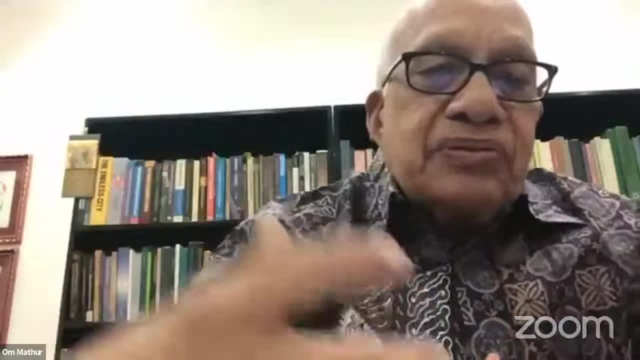 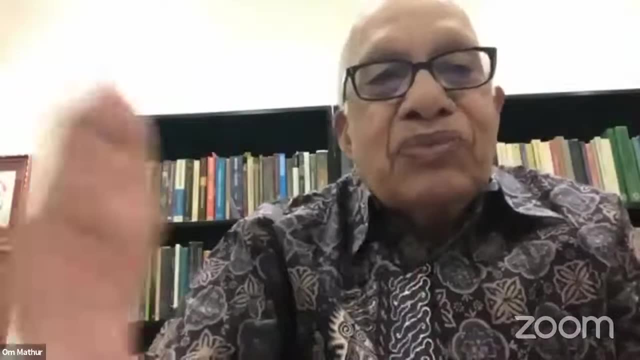 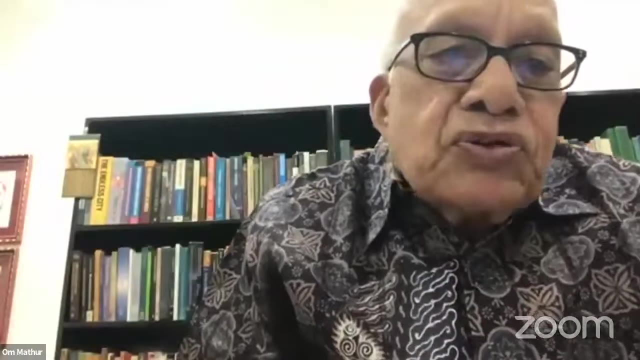 So those kind of, simply keying the urbanization in that kind of a framework is one thing, but doing an exercise which is evidence-based, which is research-based, where we have, you know, we have some kind of a better understanding of the kinds of parameters that I just mentioned is extremely important. 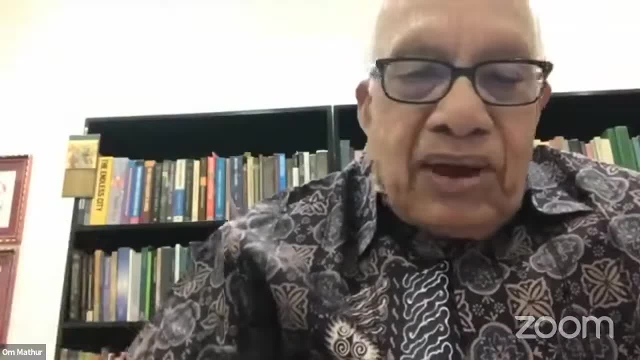 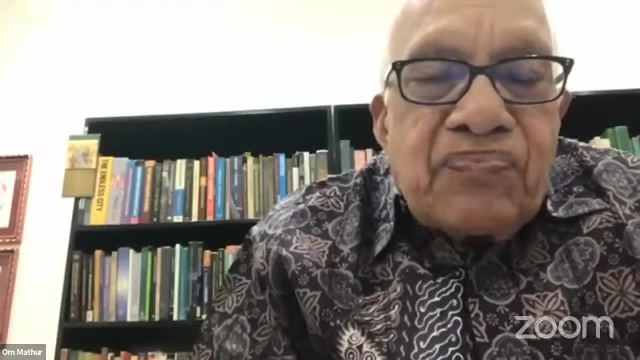 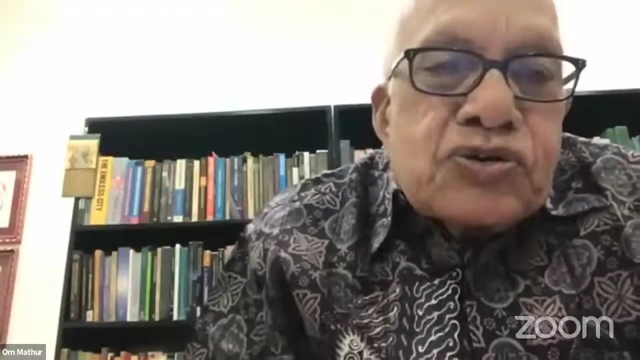 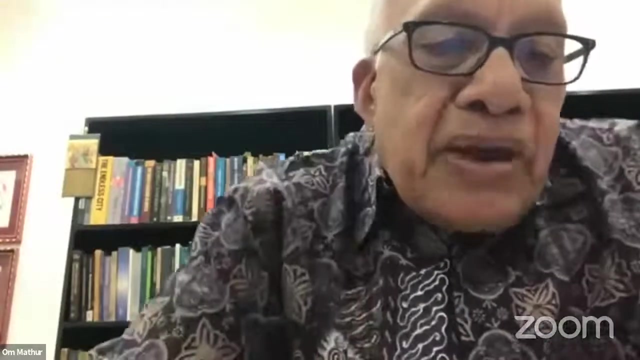 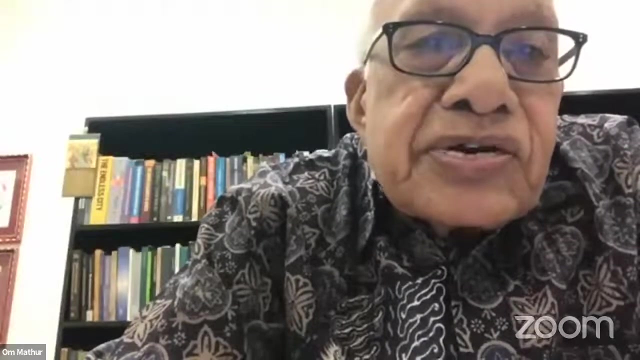 The last thing I was thinking about when I was thinking about what I'm going to say, I just came across an old book of mine, some pages of that one, the book is some, I don't know where the book is, by Edward Sodja. It was written in 2000. And I just read out three nines of that book. It says, it may indeed be both the best of times and the worst of times to be studying cities. 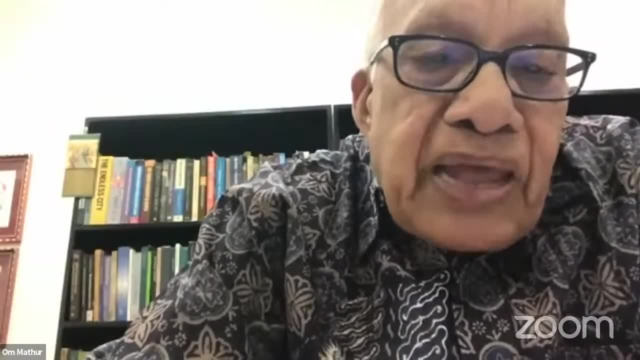 For why there is so much that is new and challenging to respond to, as the concept paper says, as your concept paper says, 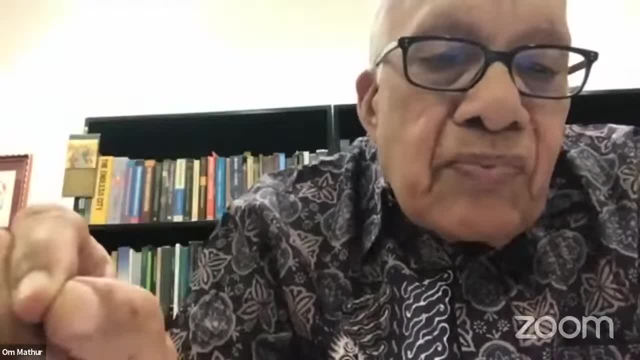 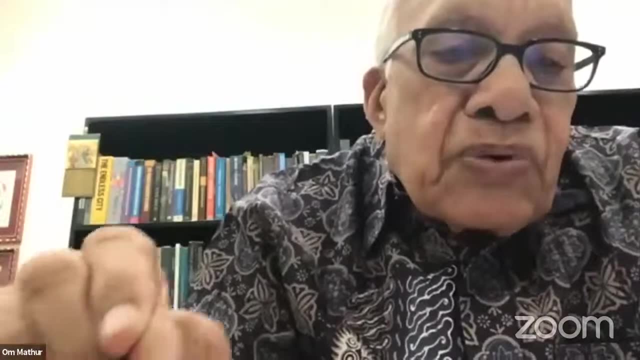 there's a much less agreement than ever before as to how best to make sense, practically and theoretically, of the new urban worlds being created. 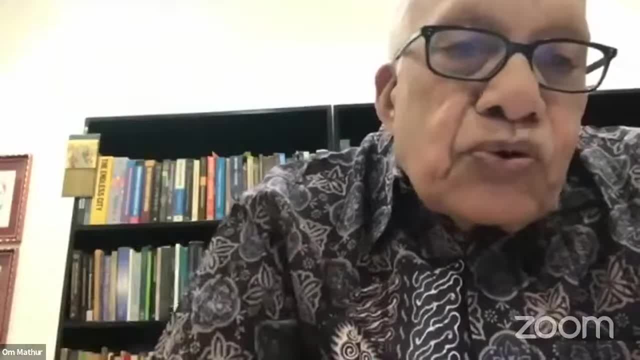 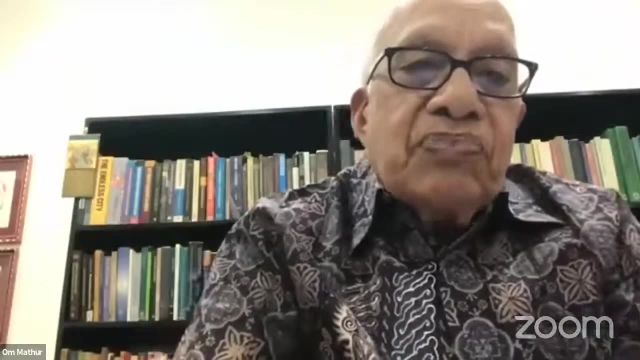 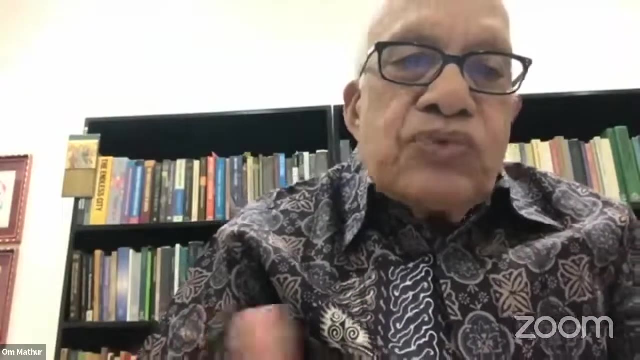 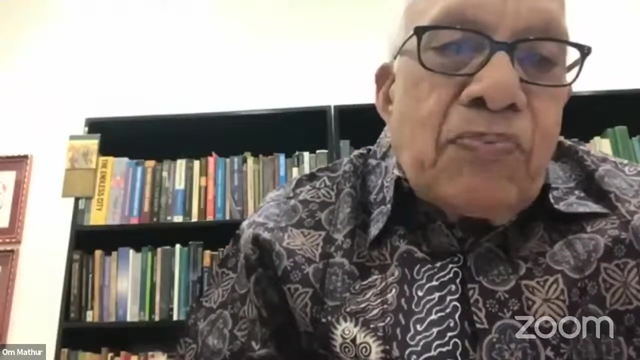 And this is precisely what Hitesh was saying, that are we going to deal with the new normal, or the new normal is going to be short-lived and we need to be looking at far more enduring parameters that confront us, which are really sustainability, the climate issues, the impact of digitization, all urban structures and so forth. 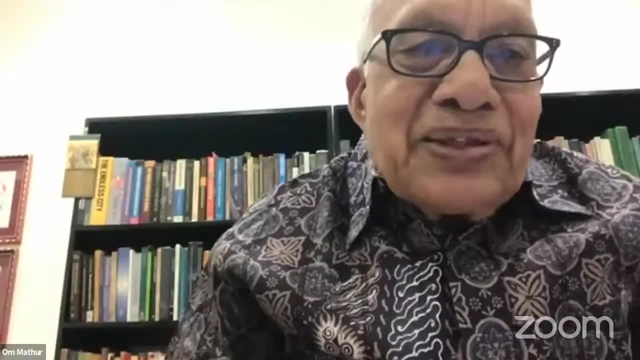 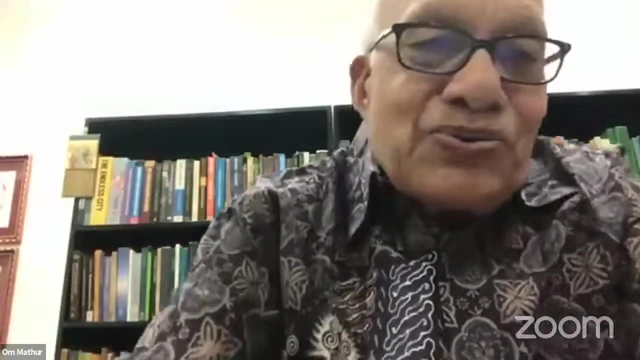 I think I have taken slightly more time than I had asked for, 15 minutes, I've taken 17 minutes as per my watch. And I would like to close at this point. 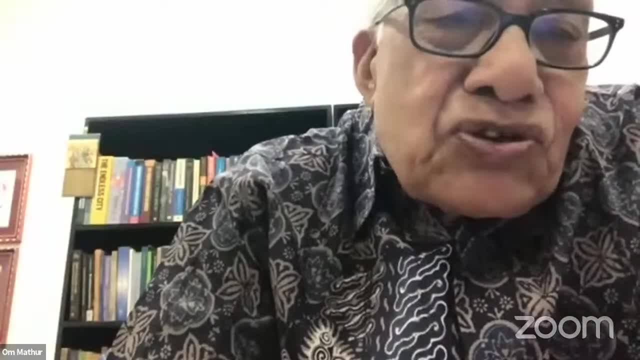 Thank you very much, Hitesh, for giving me this chance to be a part of this exercise. Thank you very much. 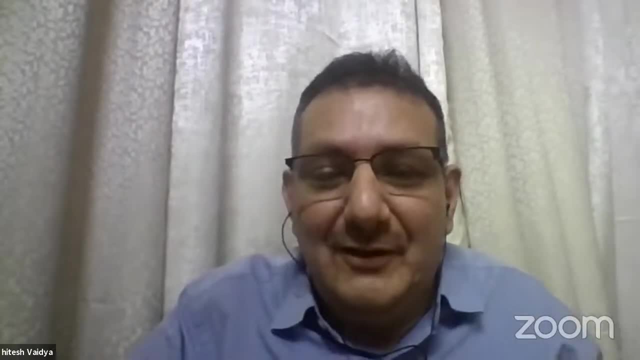 I think it was excellent articulation of the whole, you have summed it in, or I can say you have nailed it, everything, so I don't have anything to say. 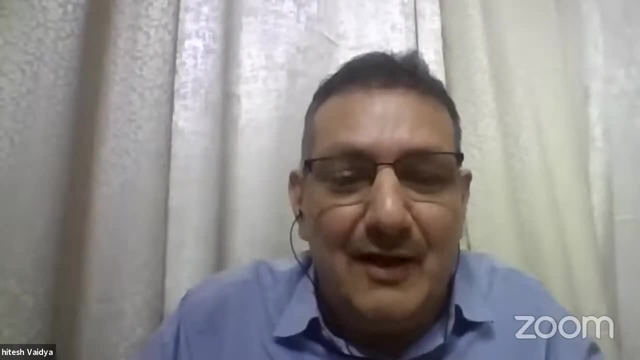 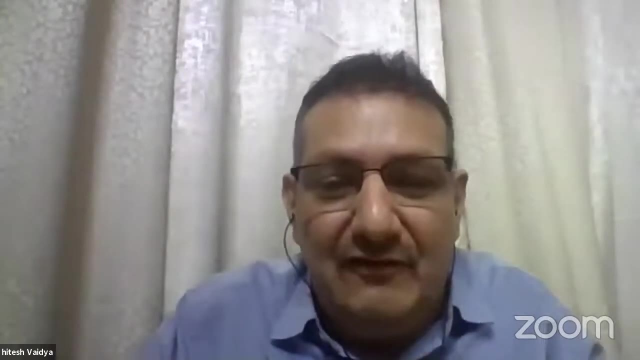 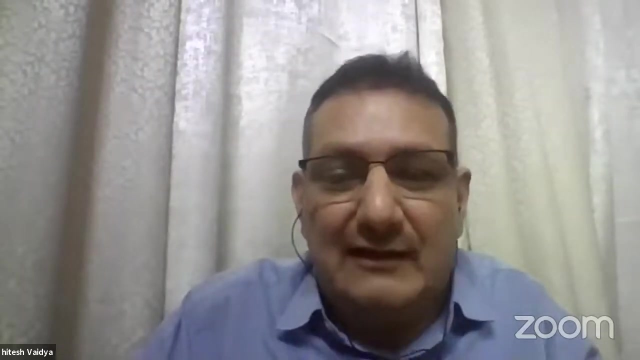 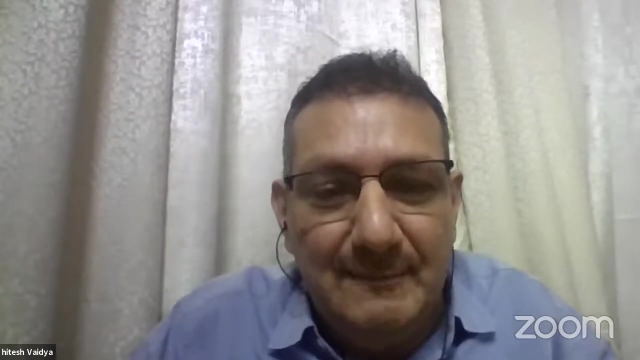 I'll come back to the question, but I see Mr. Amrit Abhijat, he's at the airport at this moment in time. So I was thinking in order to, we should not lose him, if we can give, if everybody, it's fine with everybody, we can bring him first and listen to him so that we can then carry on. So I'll request Mr. Amrit Abhijat to speak, if it's fine with him. 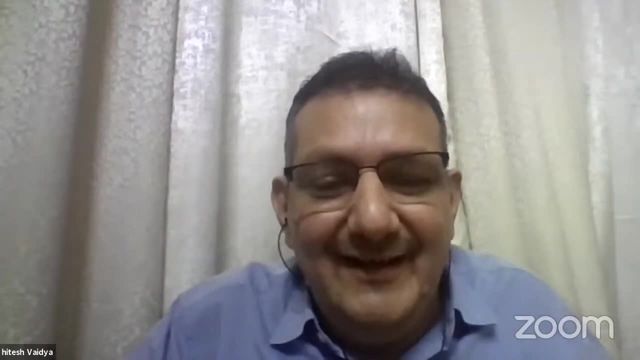 Yes, sir. Sir, you have to unmute yourself, sir. 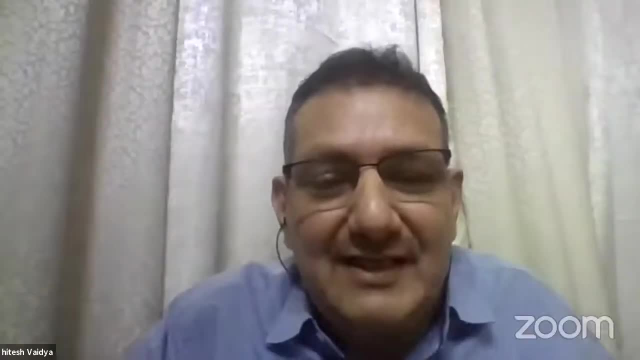 I have to unmute? No, sir, Mr. Amrit Abhijat had to unmute him. 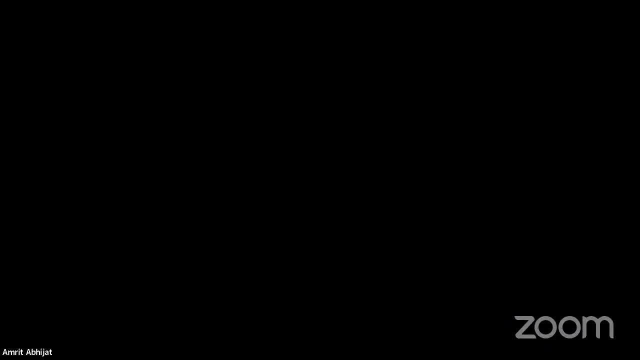 I will join after five minutes. OK, so. I'm in the queue. I'll join after five minutes. That's no problem. 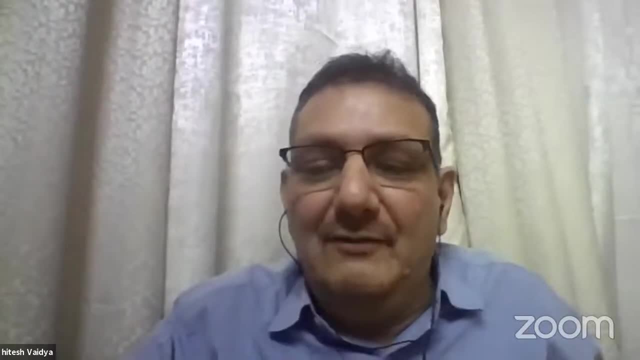 OK, then I will go to Professor Ramachandran, sir. Sir, I will ask Ravi to introduce. 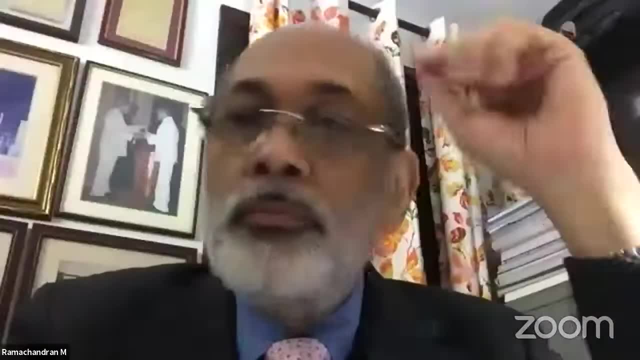 Yeah. Yeah. Yes. Thank you. Yes, sir. I'll do that. Yeah. Yeah, yes. I'll do that. Good. 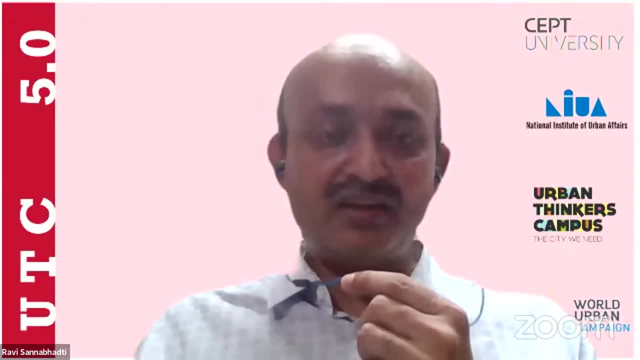 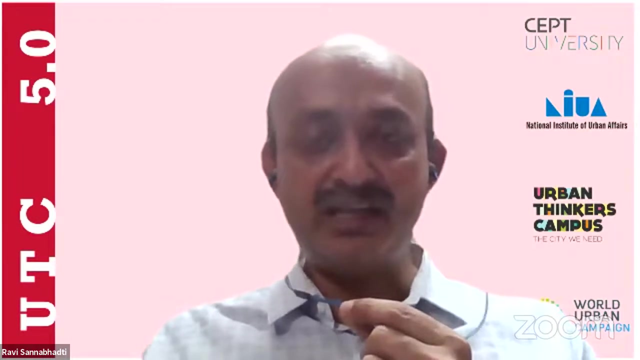 So I would like to invite Professor, Dr. Ramachandran just for everybody's kind of benefit, I would take this opportunity to introduce him, Dr. M. Ramachandran is a former secretary to the Government of India in the Ministry of Urban Development. four years tenure on this post. He was actively led to the urban reform agenda and activation of city systems in the country. He has been author of number of books on infrastructure and urban issues. And he basically, by education, he has a PhD in project planning. Due to paucity of time, I am not getting into all the kind of achievements that he has had. But I would limit my kind of introduction to just this much. And he has been kind of very modest in sharing with us this as his key achievements. So I would now request him to kindly address this gathering. Please, sir. Thank you. You can hear me? Yes, sir. 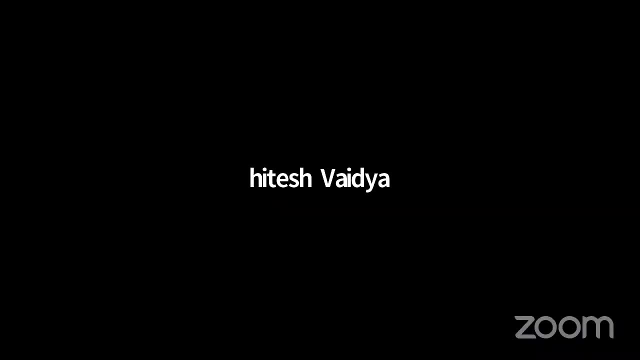 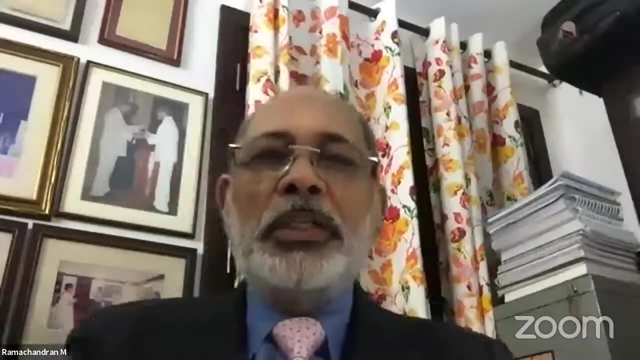 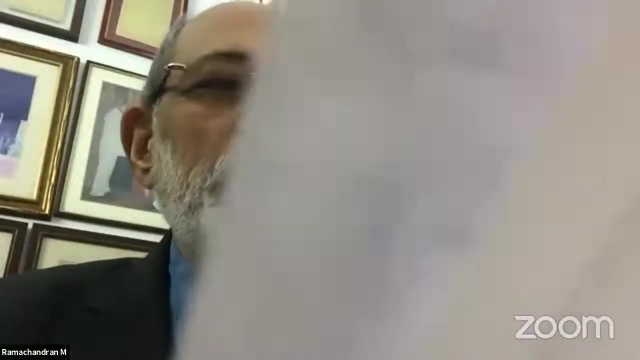 Thank you. And thank you, Sri Hitesh Vaidya. What I thought was I'll just list some points which need to be considered as perspectives on the need for urban policy changes. Without going into any background or basic details, I would like to list these points, which could be taken up for policy changes, as well as making local governments vocal in our governance schemes. 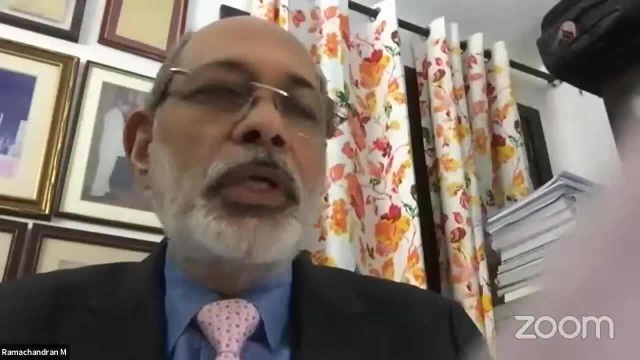 First is recognizing the model of urban development. And secondly, recognizing the importance of urban development in the local government. And thirdly, recognizing the importance of turns that thank you. 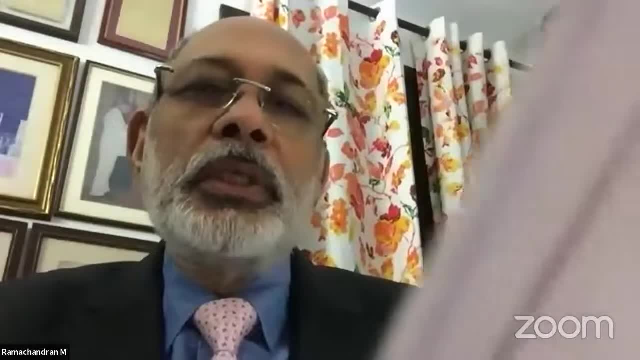 we see a few, you know? is a kind of sectarian leadership, right, of local governments, working closely alongside. You know politics versusbecause they often don't 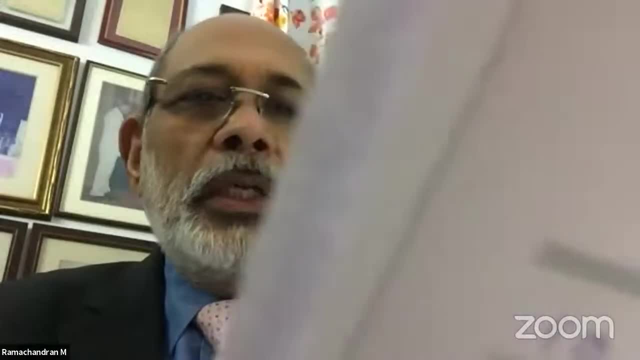 listen, but also if it's about Lights Japan politics. We have a focus here on climate change, you know, on the is a different area of society 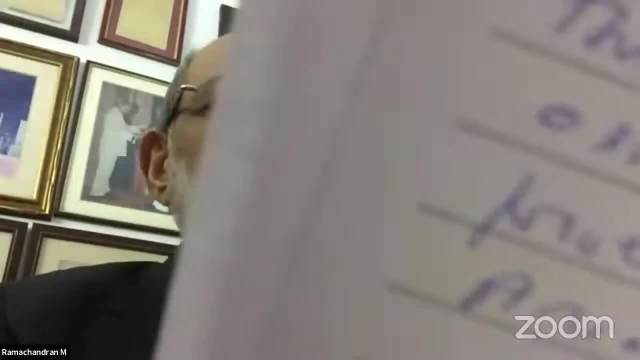 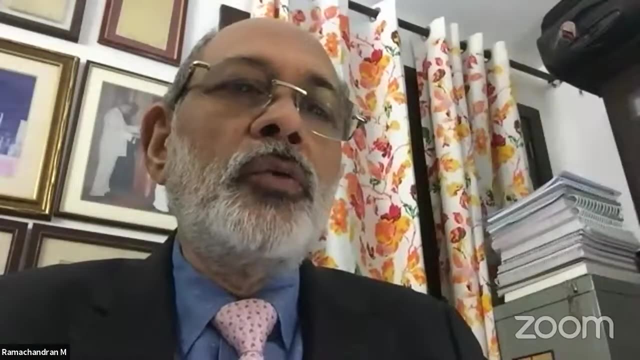 and even if we probably should seek engagement or strength to then you know, we are different countries, so we understand that, as is Nishant. 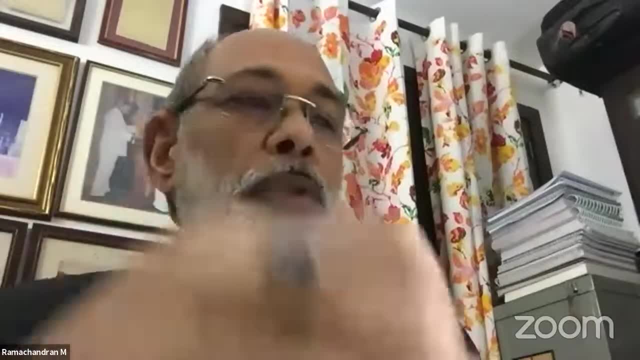 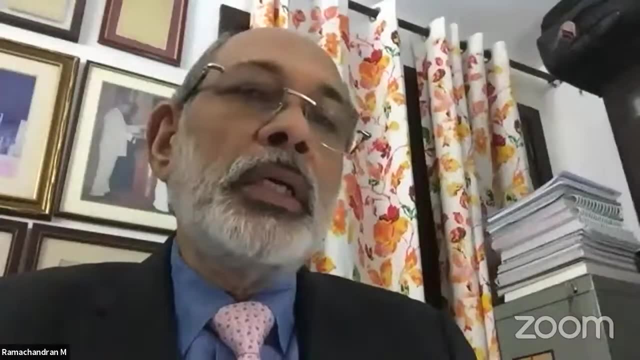 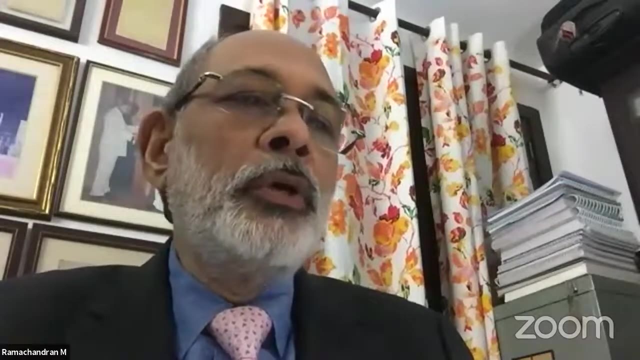 during the pandemic and demonstrated their capacity to ensure regular supply of water and electricity, proper waste management, understanding critical, undertaking critical tasks like disinfection, managing requirements of the people, particularly those who needed help, contributing to the requirement of maintaining social distancing, avoiding contacts, et cetera. Essential provisions were available closest to the residents mostly, and effective methods of addressing the problem of slum dwellers were also worked out. I also believe that the construction of large number of toilets under the Swachh Bharat Mission also made a big difference in the scheme of things. 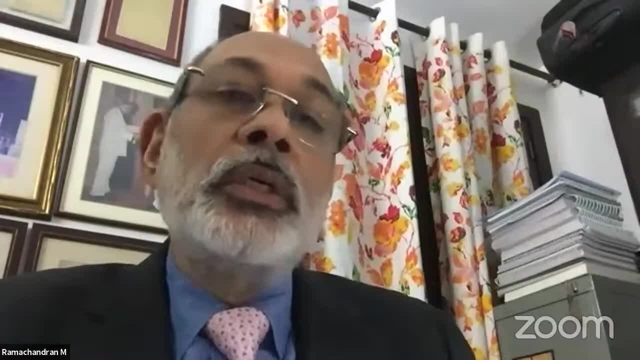 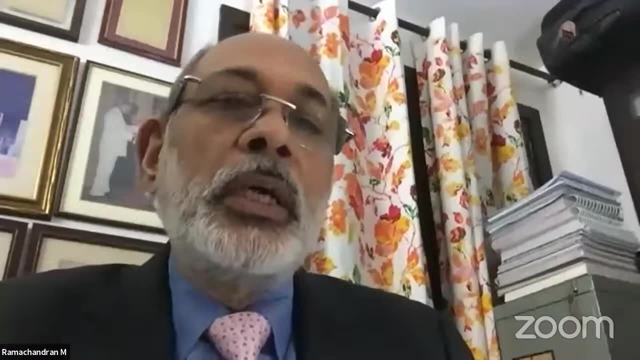 Central programs, particularly Amrit, has as its basis the primary purpose of covering all households with water supply and sewerage, and with active involvement of local bodies, fundamentals like this, can be better achieved. 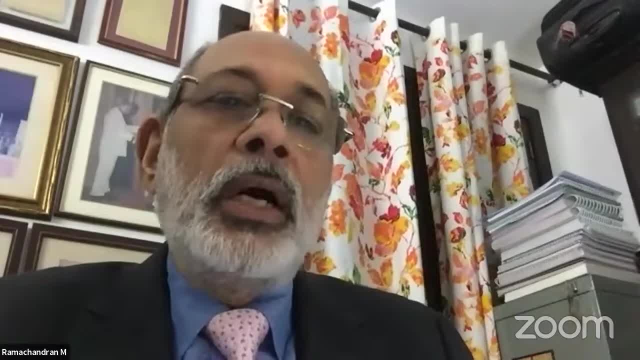 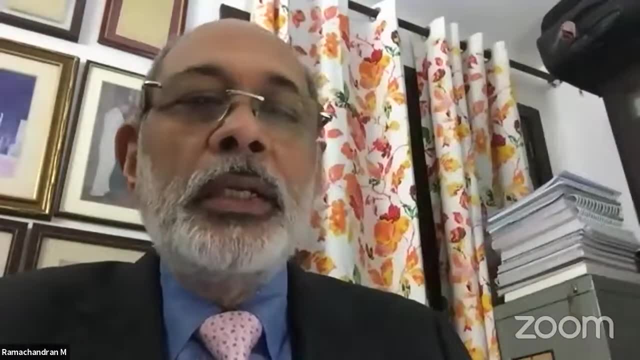 It may be mentioned that once again, under Amrit, transfer of all 18 functions to urban local bodies is a reform which would have been done in a 12 month period. 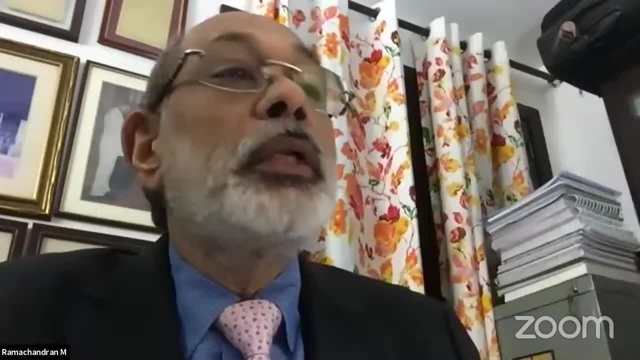 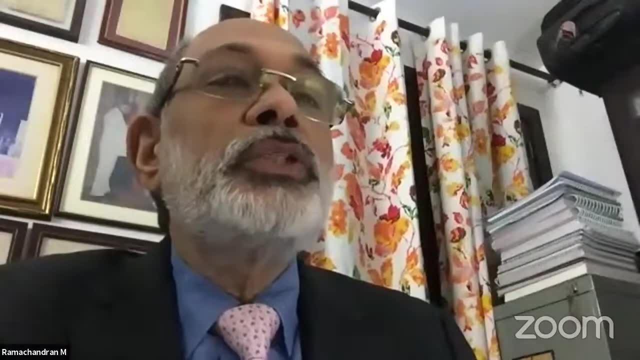 The second point is since the reform requirement is getting repeated mission after mission, I think it is time to move to a regime where any further central funding or support under any central program should happen only after an independent mission. 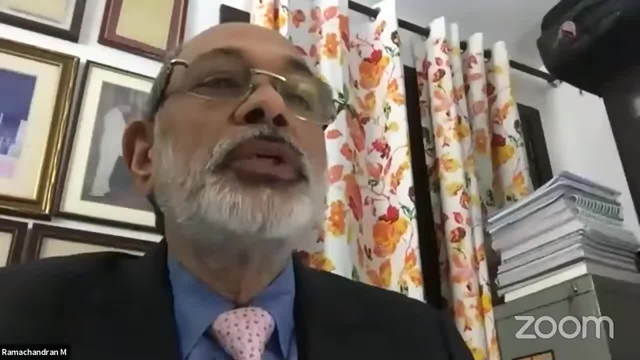 I think it is time to move to a new regime where any independent audit of the requirements of transfer of functions, funds, functionaries is undertaken. This could be questioned, but that's one way to move forward 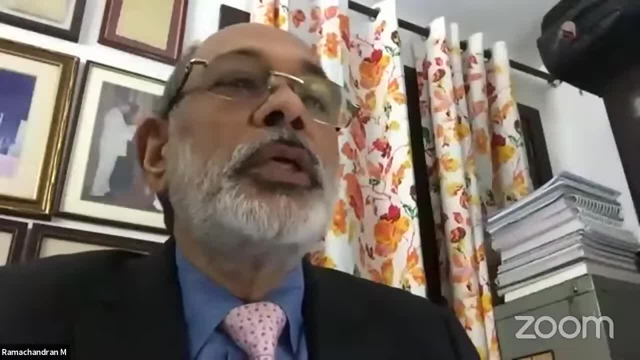 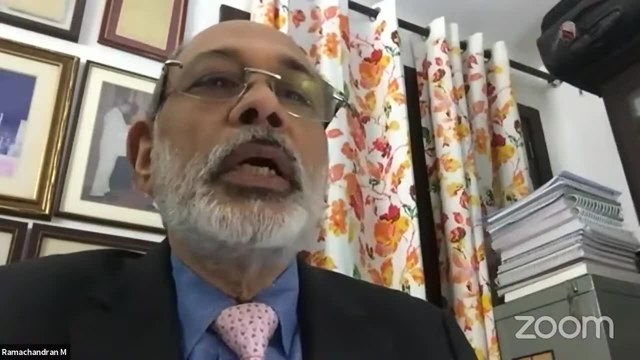 as far as trusting the local governance is concerned. There could also be a mechanism of independent eminent persons group reviewing and confirming that the transfer steps are in order in each state. 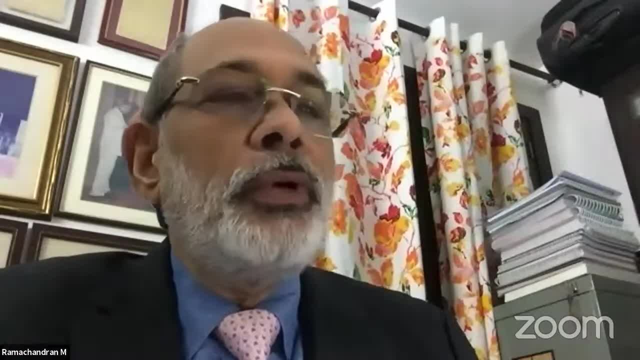 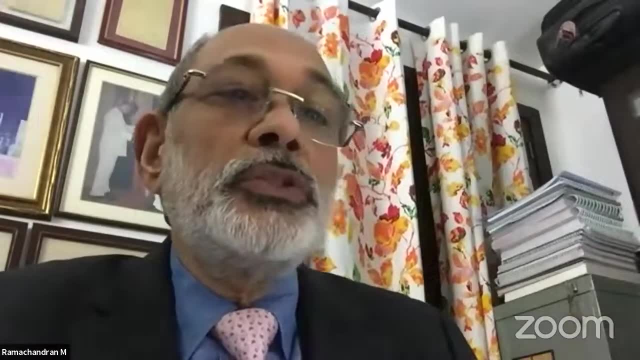 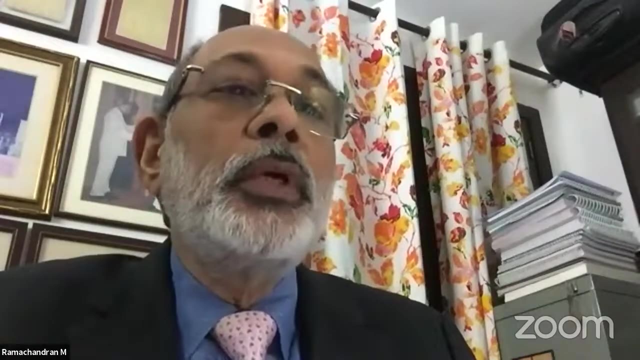 Third point is two important steps required now are that of having active ward committees, and functional areas of us or area units. The constitutional amendment provided for wards committee, of course, for municipalities having population of three lakhs or more, but hardly do we hear about these committees 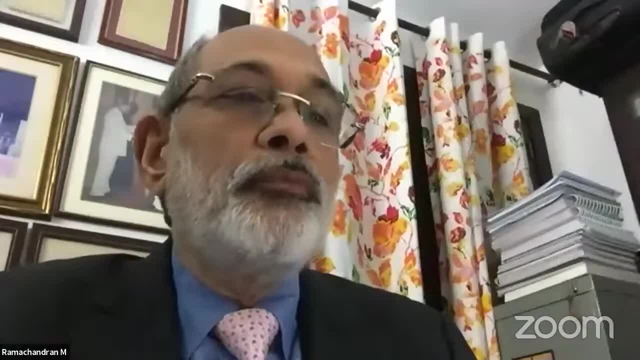 getting constituted or they meeting regularly. The word legislature may by law make provision 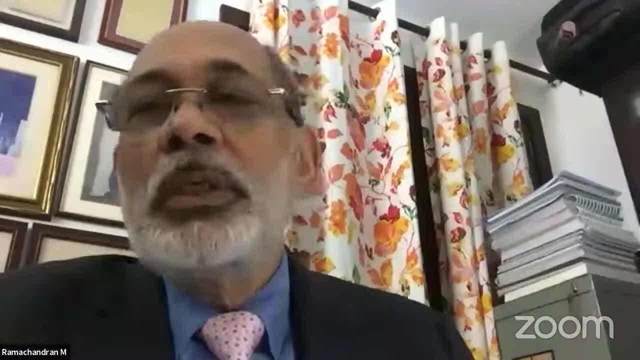 seems to have let the states go extremely slow on this provision. 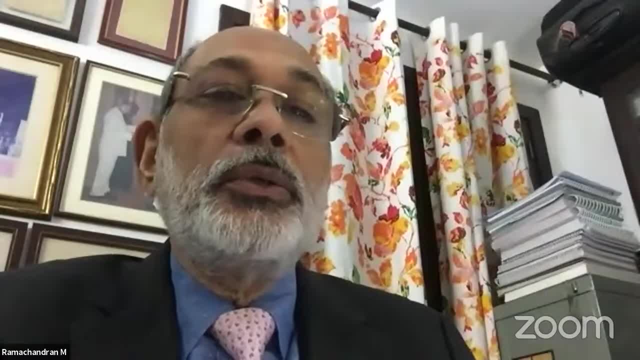 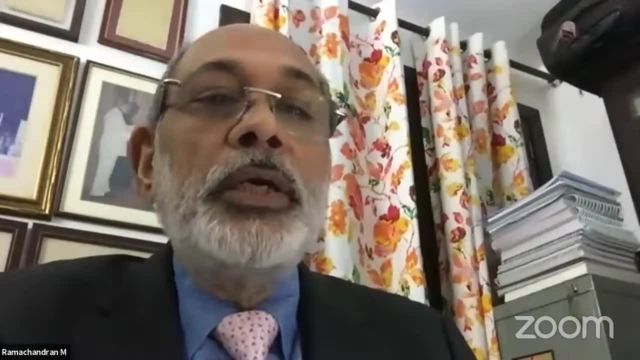 The model Nagara Raja Bill circulated to all states has detailed the rights and duties, activities, functions to be assigned, and the idea was to make people feel more involved 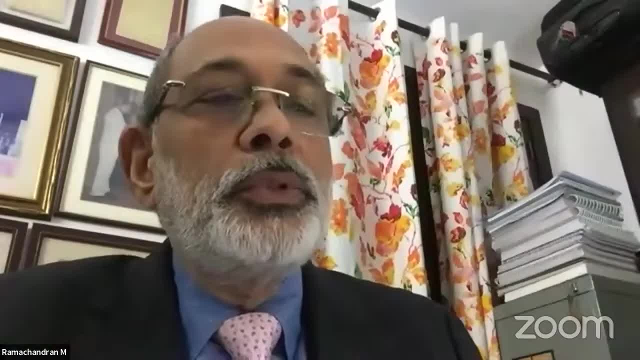 in the activities of the ward and be the mechanism to close the lias with the municipal body. 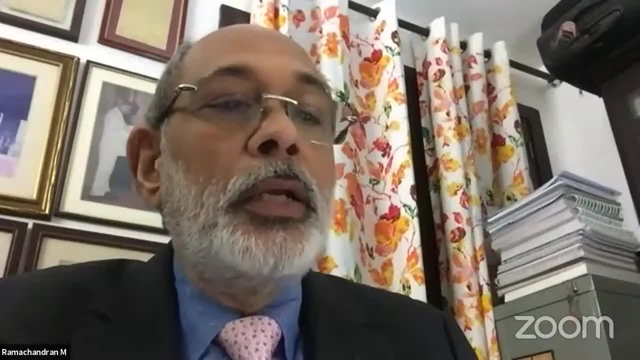 The ward committees could prepare budget for the ward and produce a ward plan aspect. 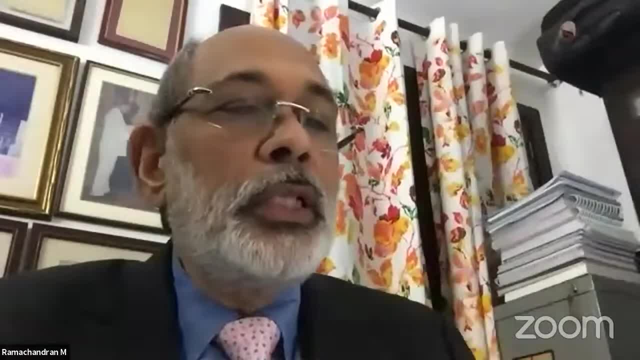 Since there is no communication mechanism between the local body and the people. Such a mechanism is required in all urban bodies. Fourth, traveling further down areas of house or area units need to come into existence at the level of each polling booth, which means population about 1000 into existence at the level of polling booth or contiguous polling booths together if the per booth number is low. Since the response to provide for such areas of house through community participation law mandated at the time of the national urban renewal mission with places like Hyderabad being the exception has been extremely poor. 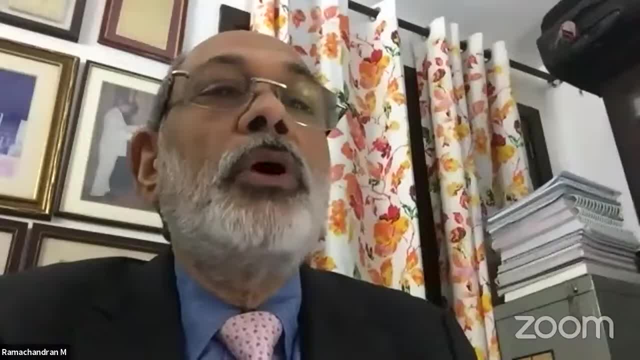 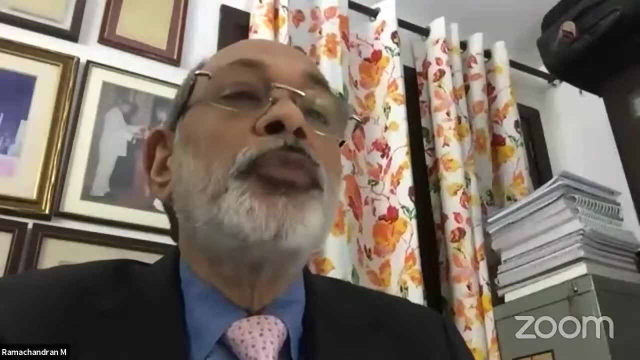 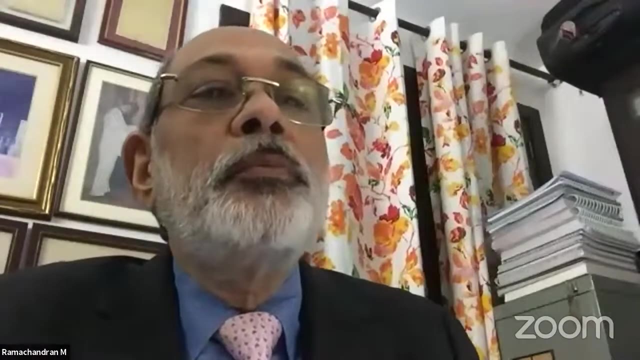 I would argue for such area level units being set up on the basis of an administrative or a council decision in case legislation is likely to take time. These area units can compile and keep basic information about people's problems and requirements and proactively involved in various activities at their level. 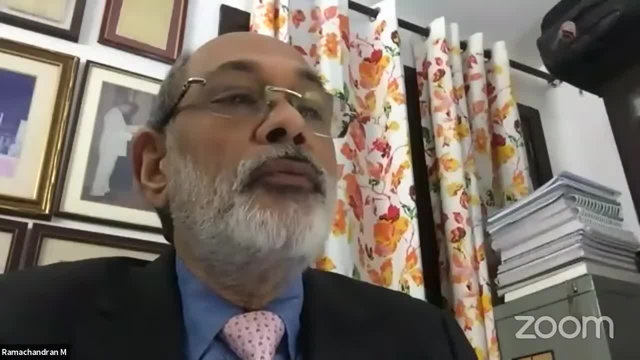 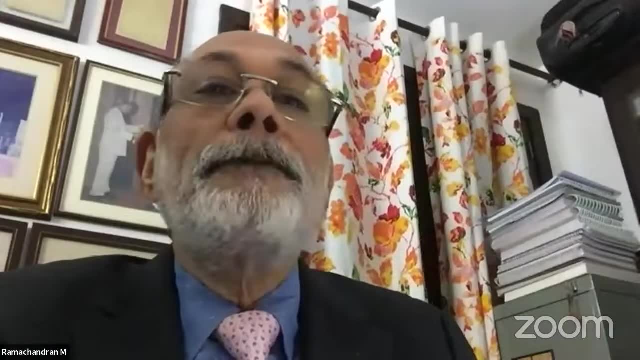 Instead of having an election process, we could have compact area units or committees with select representatives of professionals and others living in the area, 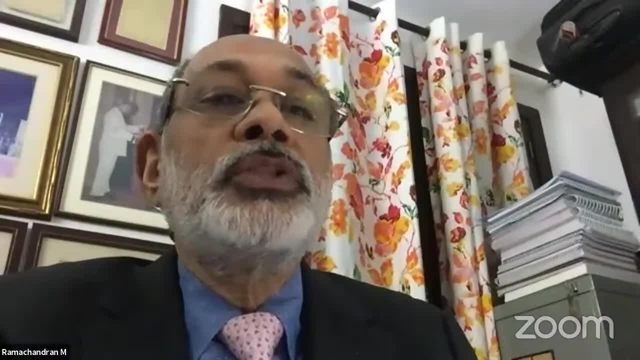 senior citizens, housewives, youth and poorer sections on a 50-50 basis among resident men and women. The pandemic has taught us a lesson 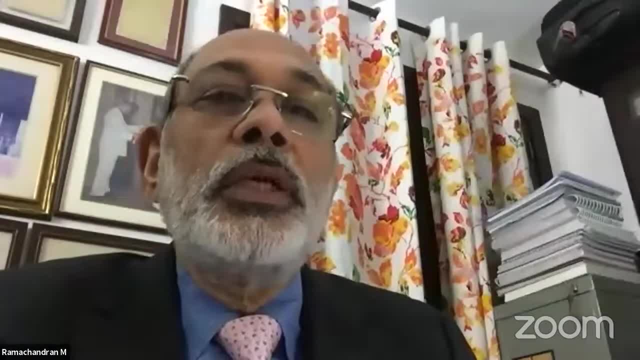 about the importance of togetherness at a local level and the body could be a significant part of our local governance. 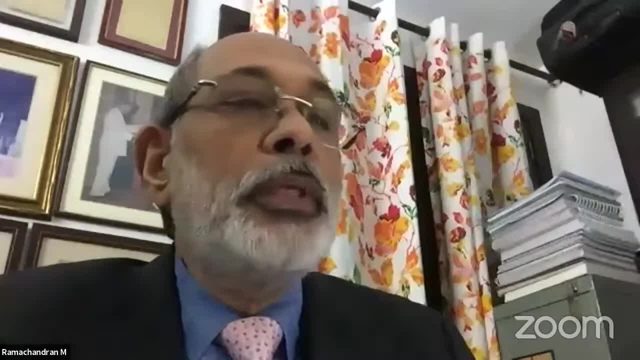 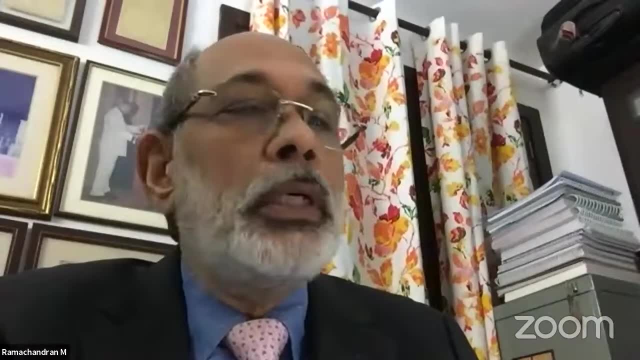 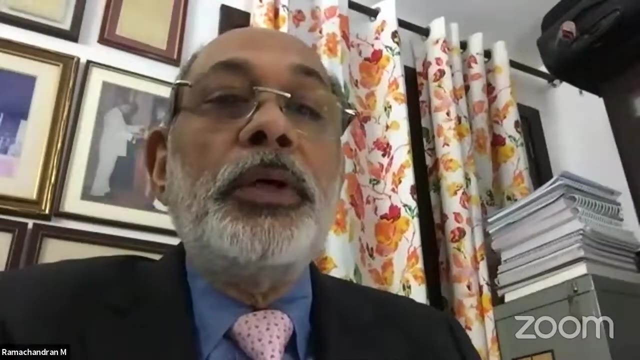 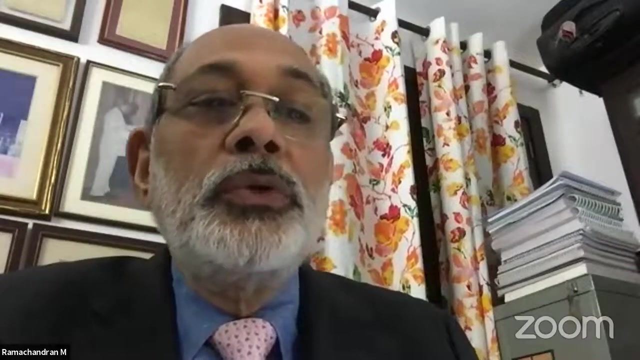 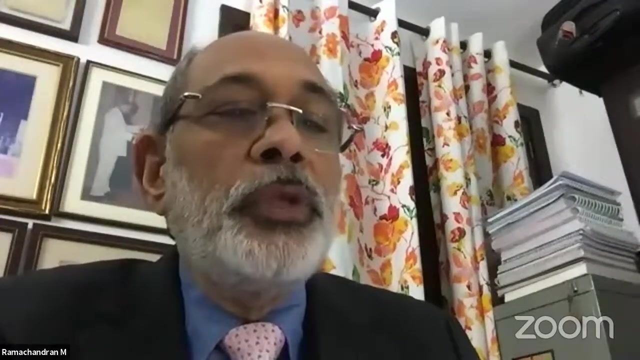 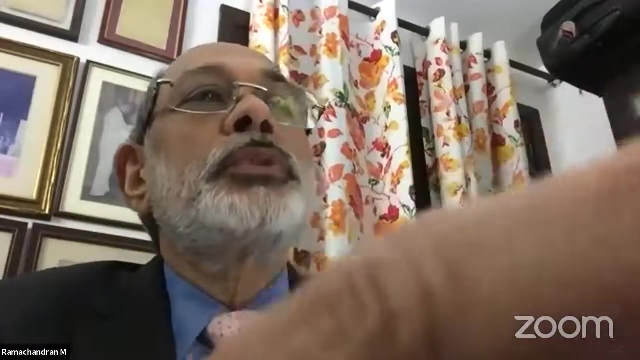 The fifth point, such bodies with active local involvement can play a proactive role in ensuring some of the basics which should take priority today, like the Amrit objective of covering all households with water supply and sewerage. This has to become a top priority now not only for Amrit cities but for all our cities and towns. These local units could actively monitor this and ensure that what is done is workable and every resident has this basic facility uninterrupted and not having to go from office to office to get problems rectified or sorted out. 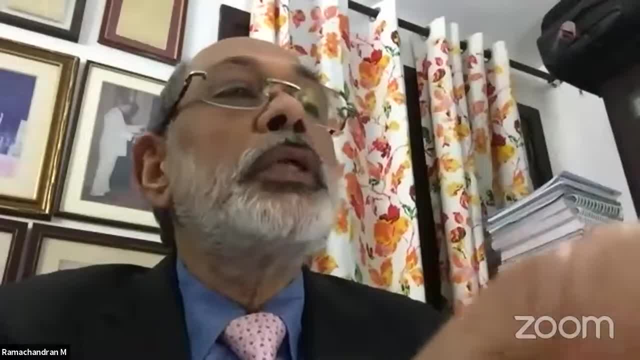 Sixth, the need to improve, enhance and further consolidate health facilities is something which, I think, got emphasized during the period. 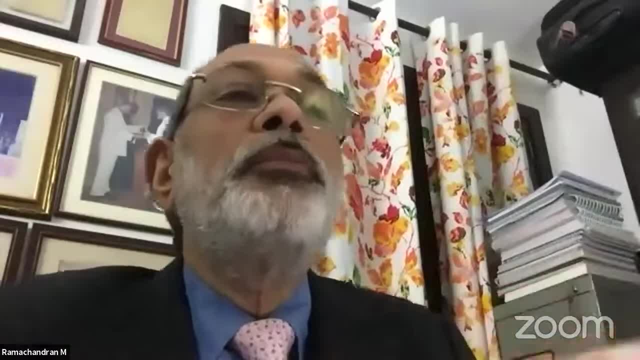 Each person's basic health data should be available promptly, linked to any visit to a doctor or a hospital. Now that the National Digital Health Mission 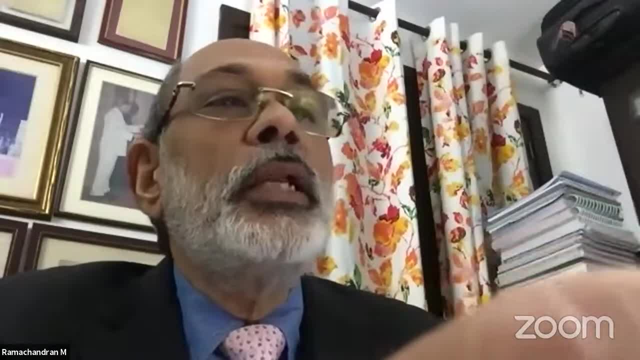 has been announced, the concept of every Indian having a health ID, which can be linked 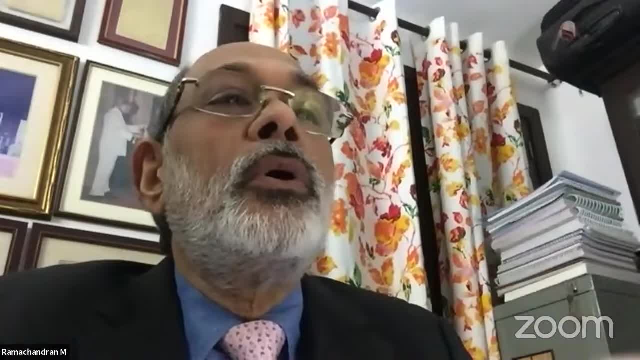 whenever he or she goes to a doctor or a drug store and having basic details like information about each disease, which doctors should be aware of. 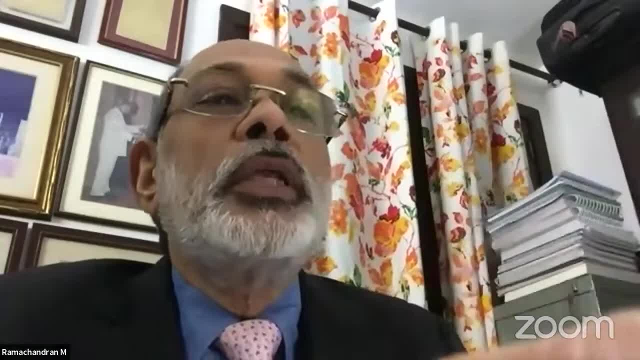 If the doctor gave what medicine earlier, what were the reports, et cetera, medical attention and help becomes faster and more direct. 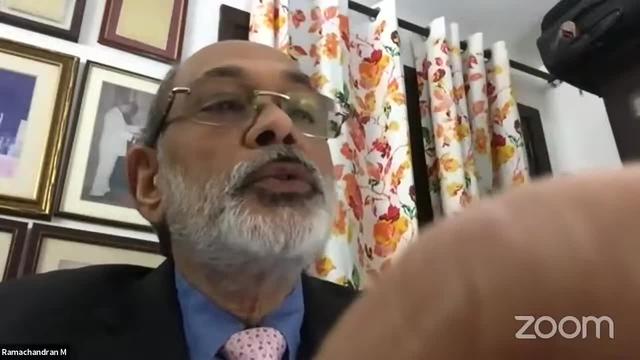 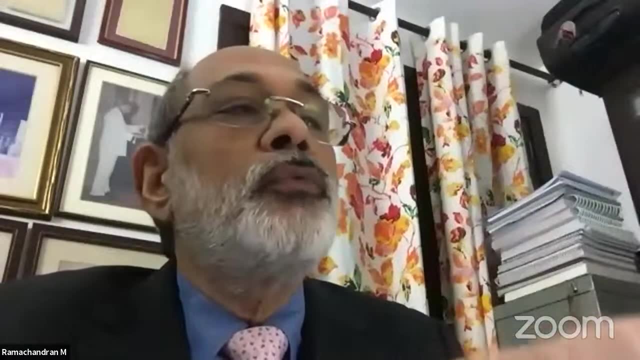 The local bodies should proactively facilitate this process and also link persons with difficulties like old age, physical problems, et cetera, with local nearest doctor or facility in a smart way. 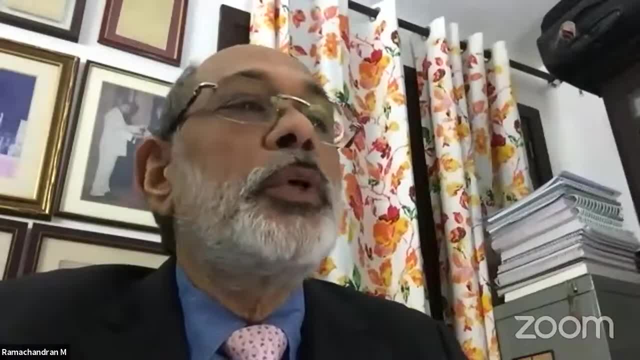 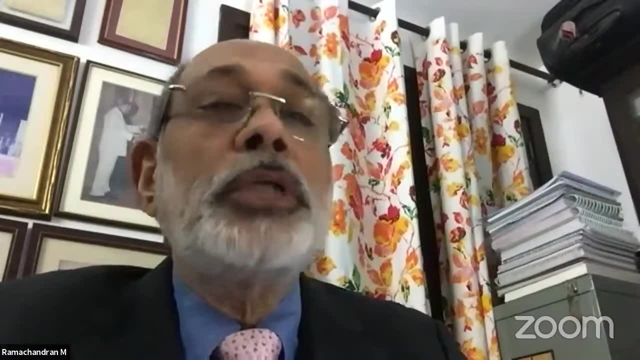 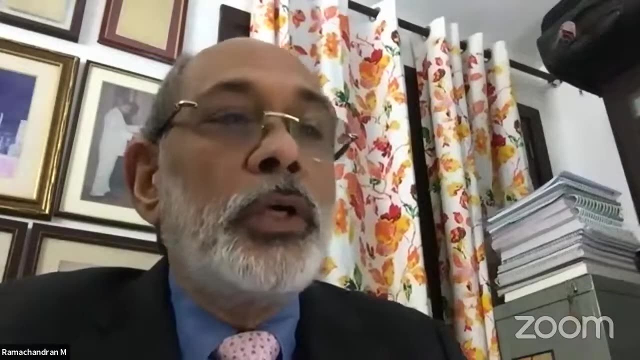 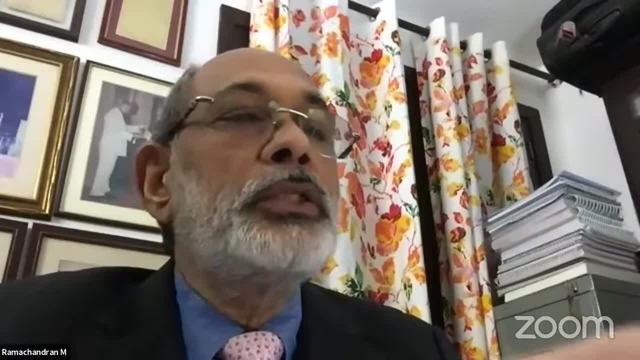 A thorough review of such retail shop less localities would need to be undertaken and land or building provided for these types of facilities. A thorough review of such retail shop less localities would need to be undertaken and land or building provided for these types of facilities. A thorough review of such retail shop less localities would need to be undertaken and land or building provided for these types of facilities. 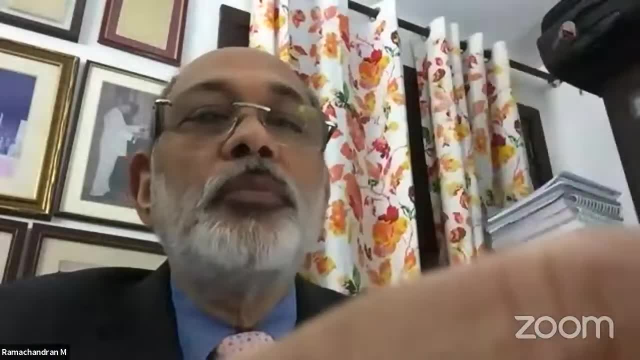 So, these are also areas where small shops are open to the public. The next point, the need for and importance of having more parks, 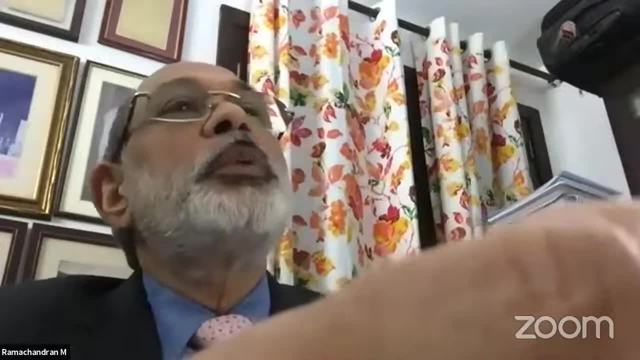 open spaces has come out very clearly. These are the only spaces which will be there for people to get out 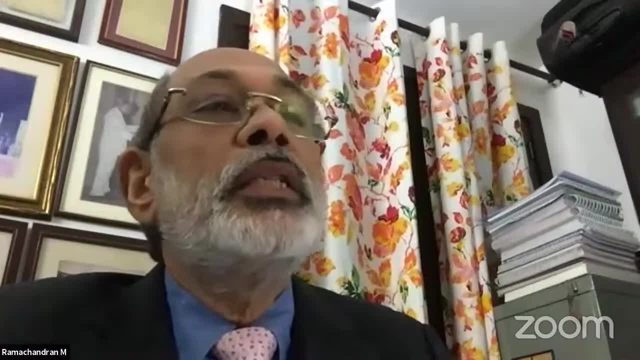 of their houses, flats, and spend some time in a healthy atmosphere. The 2014 URB-PFI guidelines proposing 25 to 35 percent land use 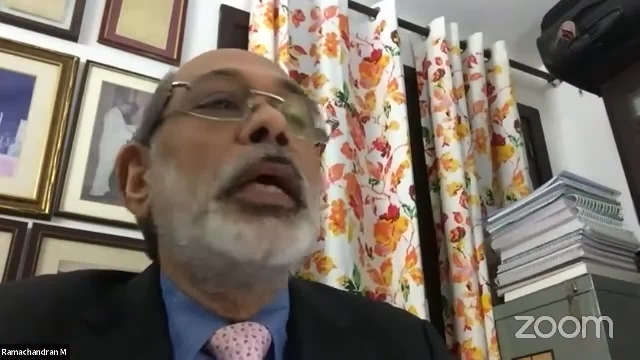 The 2014 URB-PFI guidelines proposing 25 to 35 percent land use for open and recreational spaces is not met in most Indian cities. 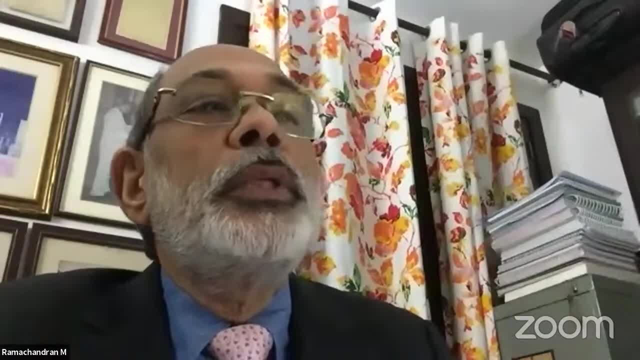 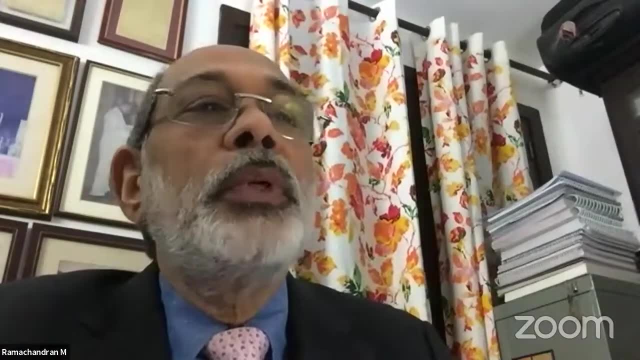 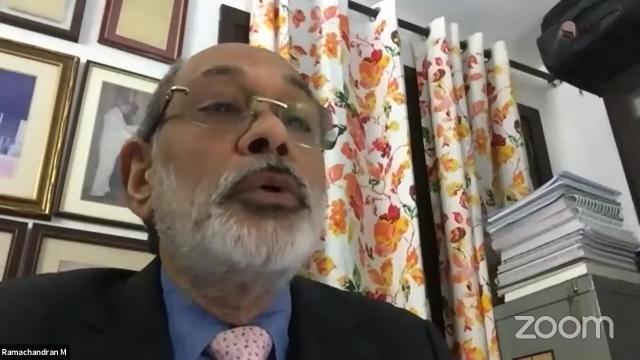 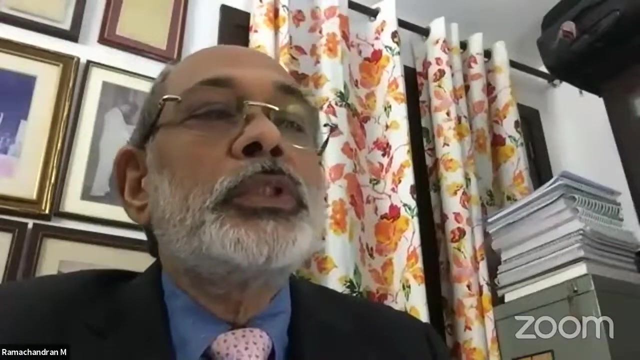 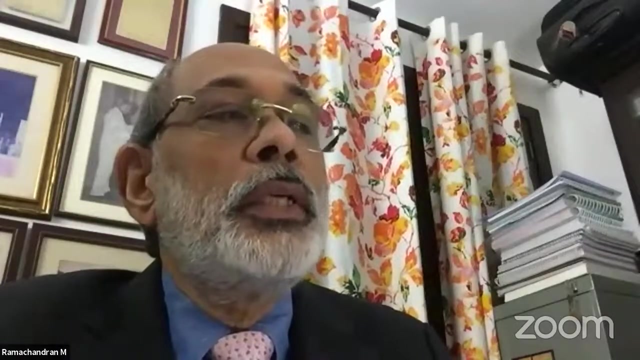 Another point which had emerged is that whatever urban green spaces we have are in the vicinity of gated colonies. So the vulnerable group of people living in congested areas are almost denied entry to spaces like this. I would go to the extent of saying that cities and towns should immediately opt for identifying and earmarking as much open space as possible in different parts of the city and keep them secure for public use in the form of parks, green areas, et cetera. 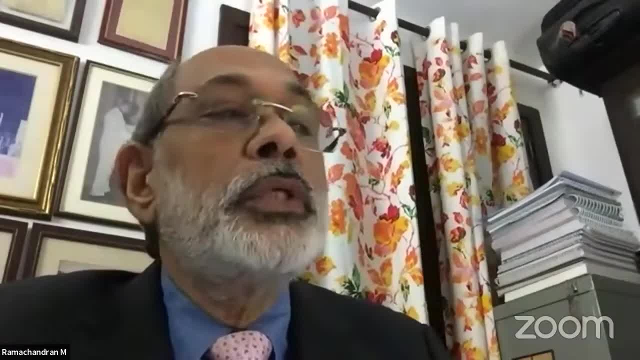 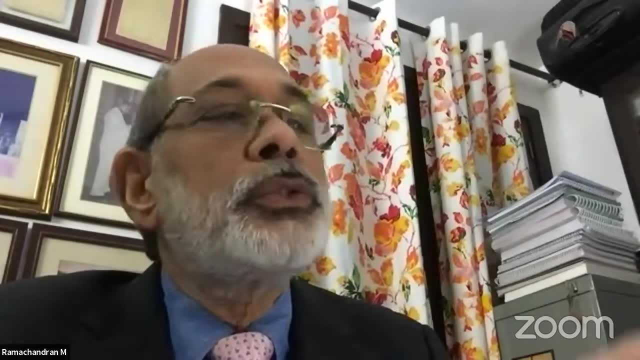 Another lesson we got was 42% of households in urban India had no room for social distancing as three or more individuals share a room in the households of the poor. 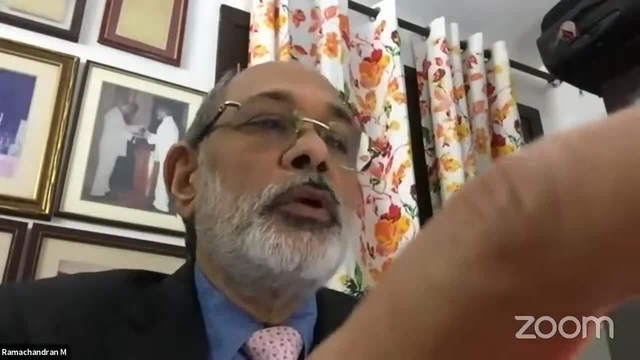 So this is another key issue which will have to be addressed through the housing programs to the extent possible. 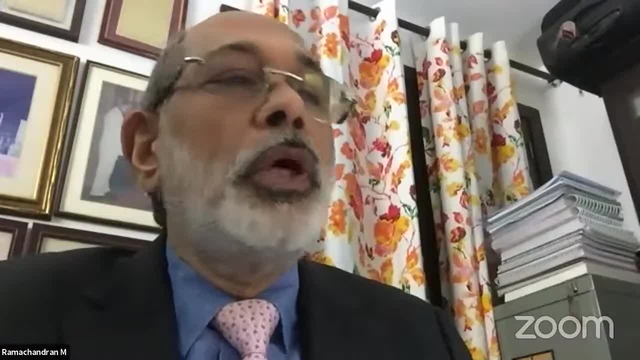 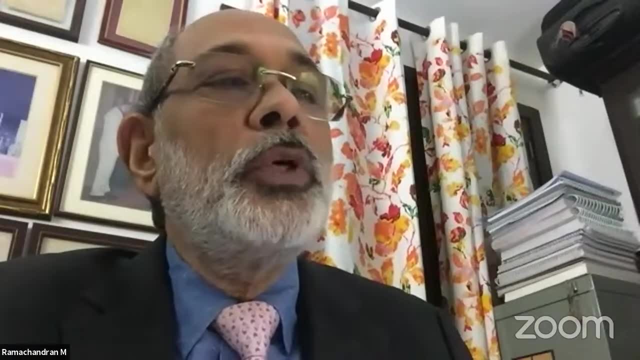 Moving on to the next point with working from home becoming the new normal, since all residential areas will have quite a number of such people working, the local authorities would need to do away with the restrictions like a house cannot be used as an office 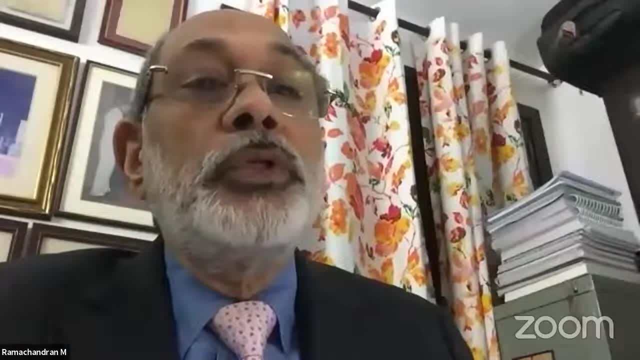 and take the route of issuing notices and start harassing. 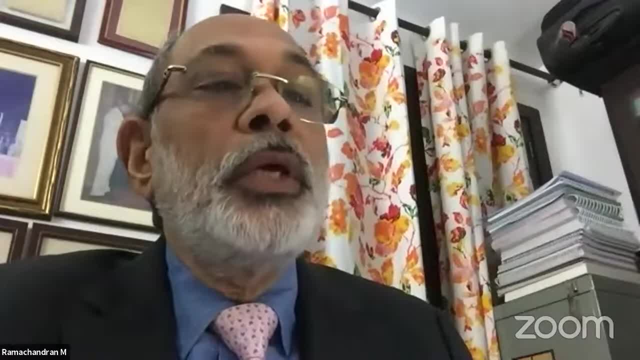 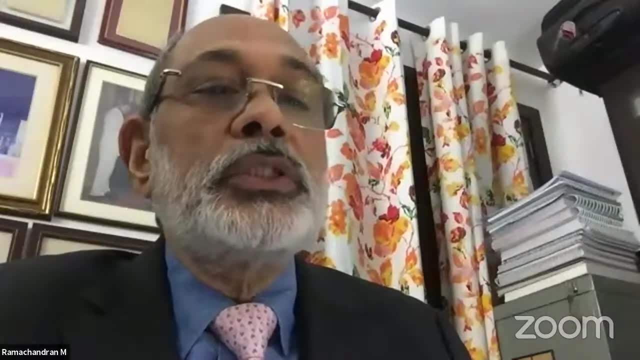 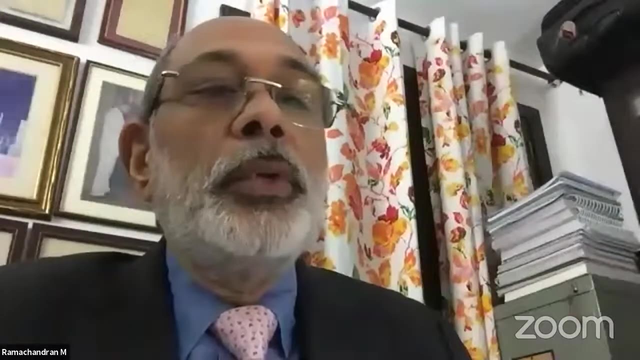 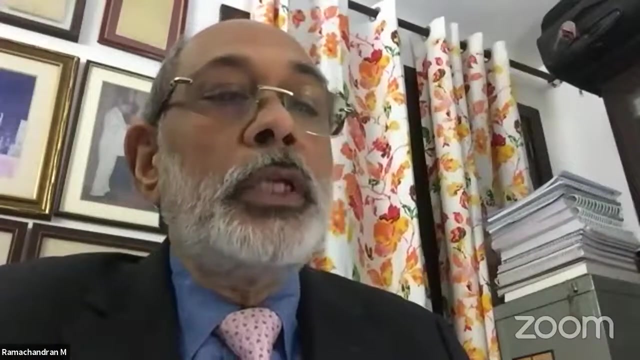 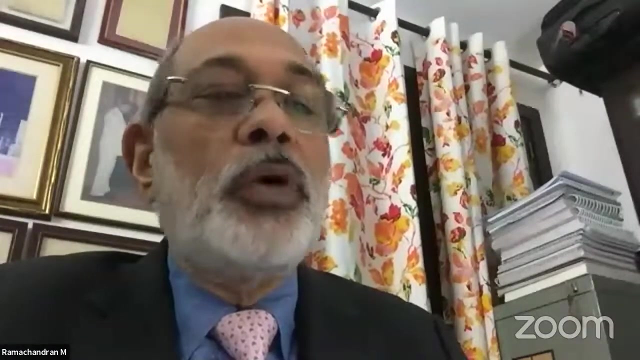 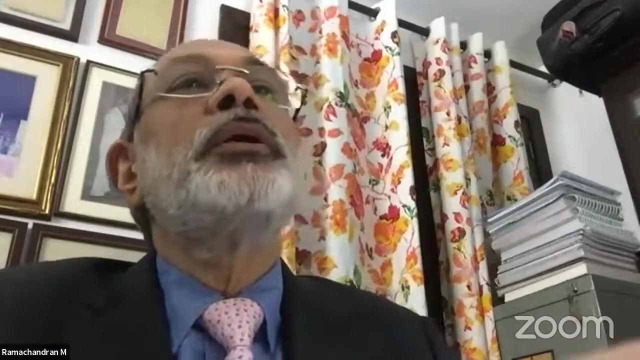 The provisions in this regard need to undergo modification and develop and control norms or regulations for future would need to be so structured or restructured. That such use is permissible and related requirements like some entries in parking, nearby shops providing tea, snacks, et cetera, will have to be provided for. One hopes telecom service providers, electricity supplying discos, and maybe availability of basics like wires, cords, gadgets, and the like in the local shopping areas also will have to be permitted as a norm. 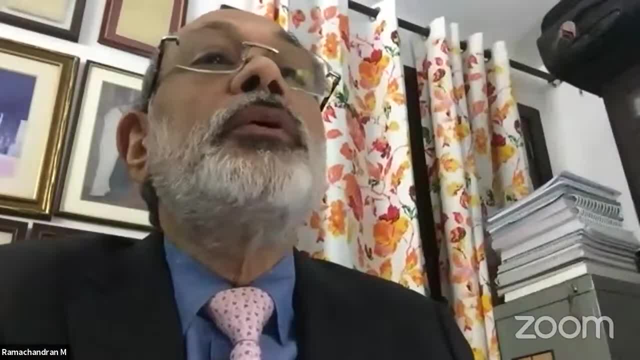 Point 10, there is a requirement that city-level plans should be prepared as to how to handle pandemic situations like this. 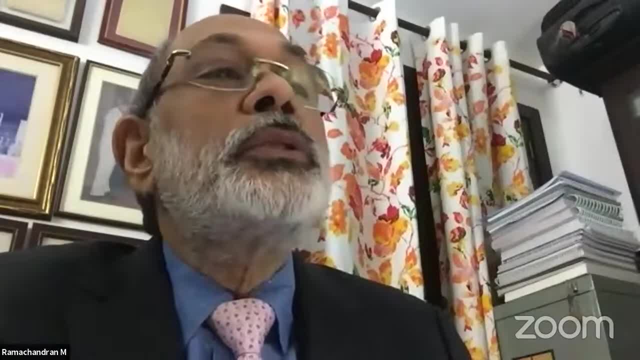 Are they being prepared? Are they shared with all residents? Is there community participation in this process? 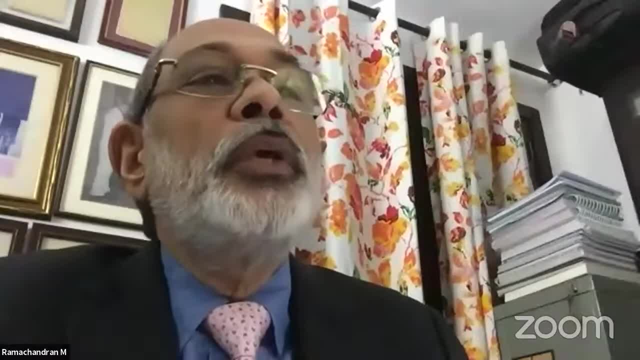 This is another area where the areas of house or area units can be effective and practically functional. 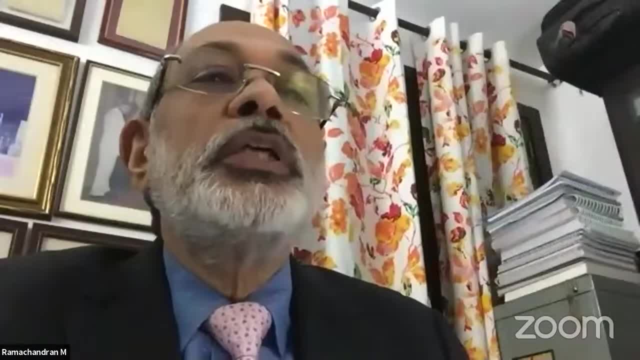 Point 11, becoming more smart, increasing smart features, would be another priority area for all our cities and houses. 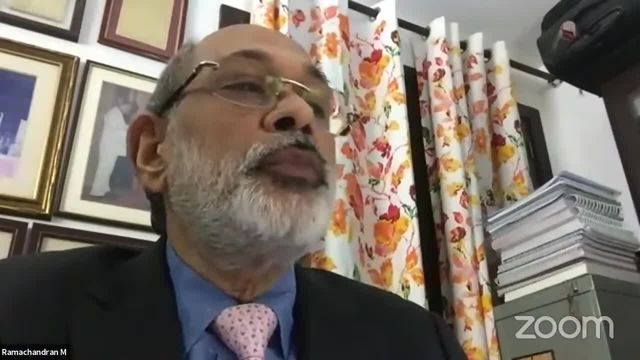 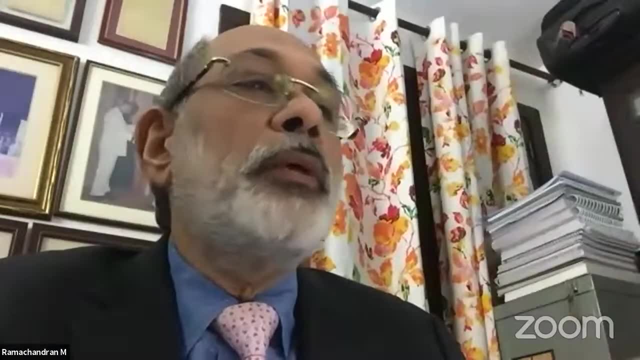 Not just the 100 smart cities. Across the country, urban areas have to consciously and consistently move to a regime where smart features become the order of the day. 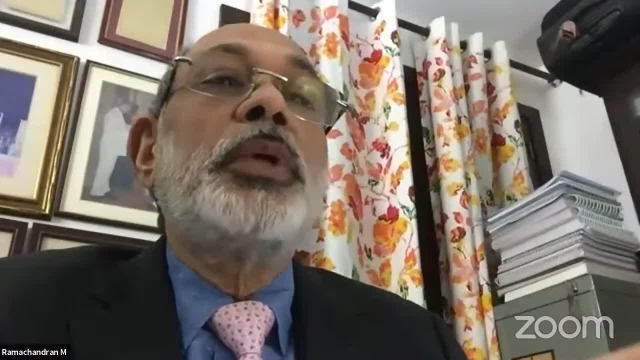 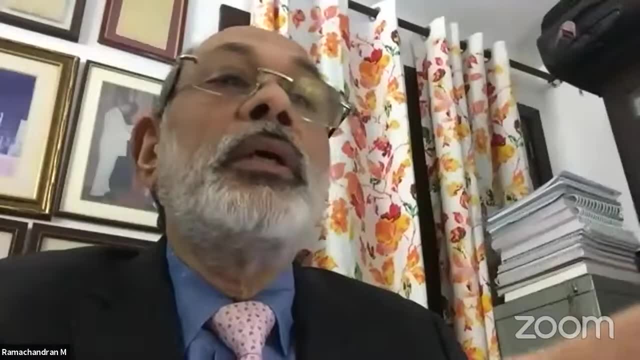 Be it smart water, smart urban services, smart mobility, smart health, or smart education facilities, with all these in position. Point 12, the city-level plans should be prepared as a norm. Point 13, the city-level plans should be prepared as a norm. Point 14, the city-level plans should be prepared as a norm. Point 15, the city-level plans should be prepared as a norm. 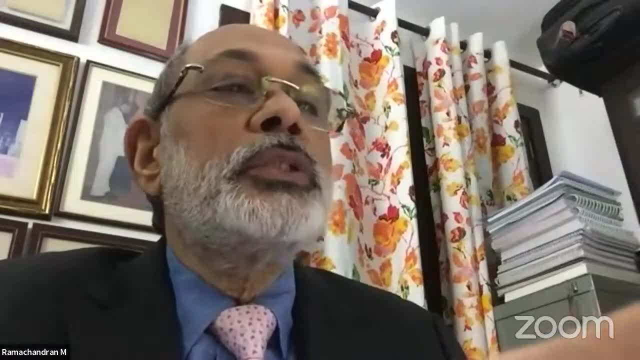 Life would be more comfortable for the residents. I think this is one prominent requirement which today's younger generations seek and insist on. 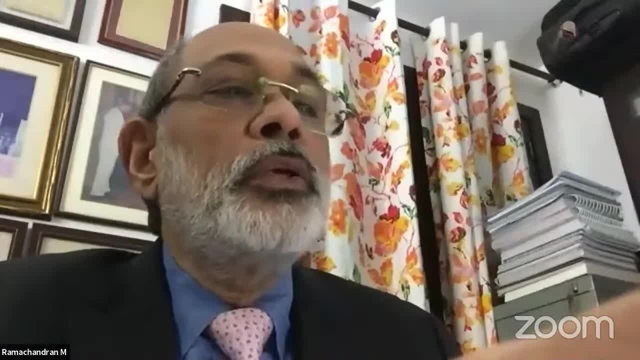 We have noticed in recent months that digital payments have been the order of the day in a large number of cases, making visits to banks almost unnecessary. 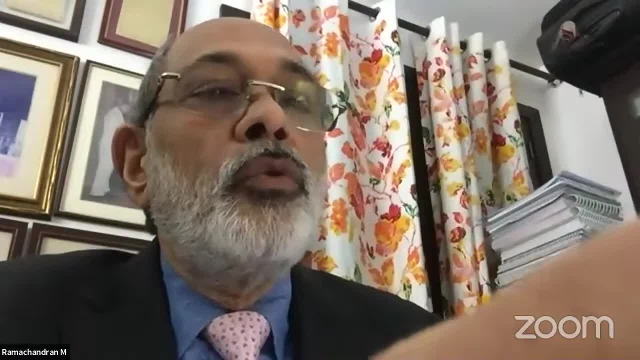 So leveraging technology to the best advantage will have to be a priority agenda. 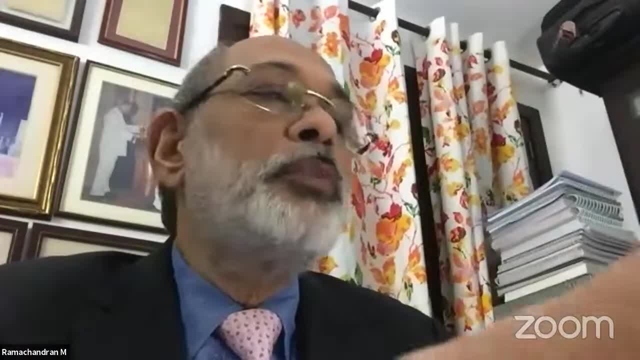 My last point, and at this stage it also becomes important to analyze how city administrations responded to the pandemic situation. 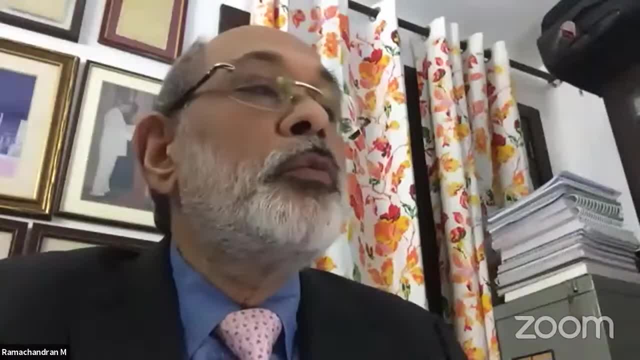 We need lots of case studies to bring out what worked, what helped and what needs to change in other cities. 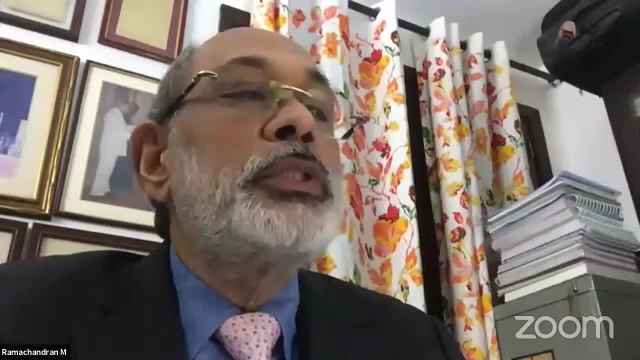 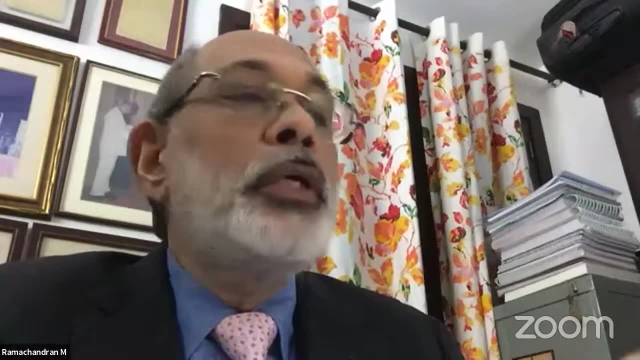 Just to cite an example, the Gurugram city authorities, their local body development authority, bus company all came together under one umbrella to provide coordinated services. Migrant laborers who had no other option were provided with food regularly. Idle city buses were deployed to take provisions to different areas of the city, in turn to sell basics. 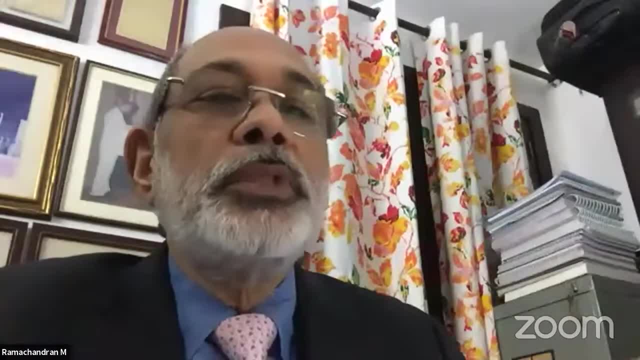 The integrated command and control center set up under the smart city mission was put to full use to coordinate and work together with the resident welfare associations. 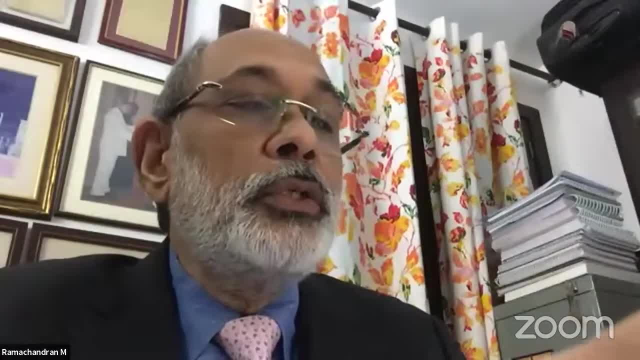 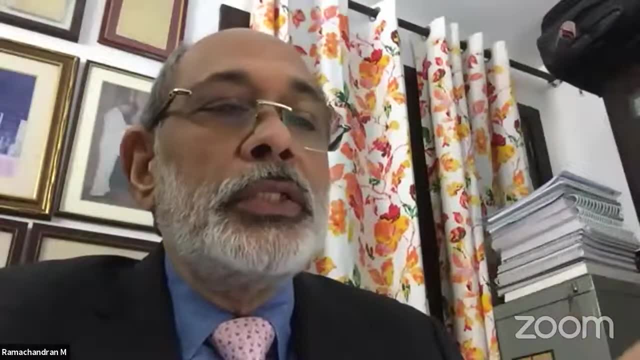 To cite one more example in Kerala, something like 19,352 ward committees deployed three lakh volunteers, kept tab on, kept tab on health conditions. 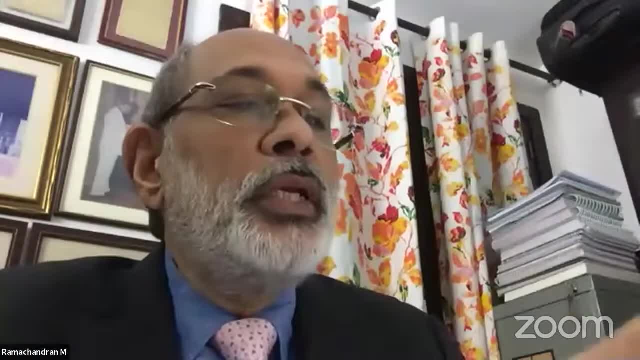 28 lakh food packets were delivered in 14 days. 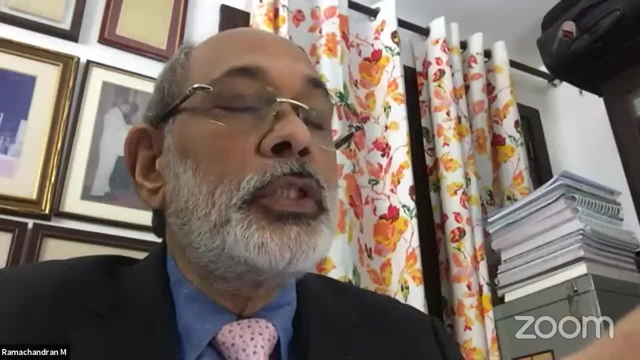 And with their initiative, they housed 3.2 lakh migrant workers. They called them guest workers in over 18,000 camps. 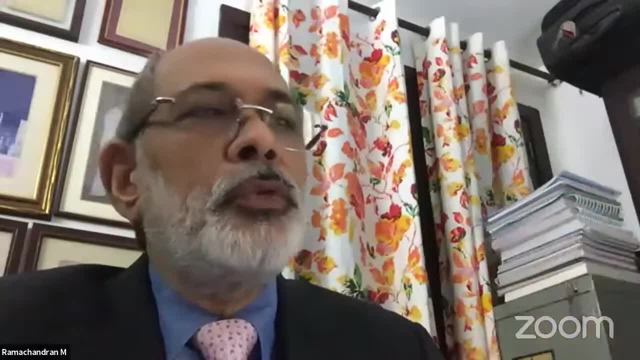 So there are good examples like this in different parts of the country. 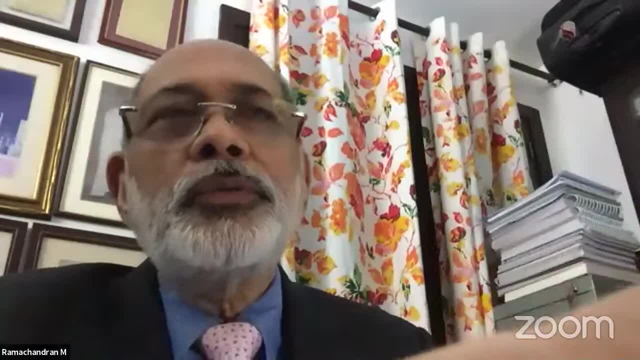 But we need to look at that. And one, take note as far as all the cities are concerned. Two, dovetail them into the changes which are required as far as R&D. 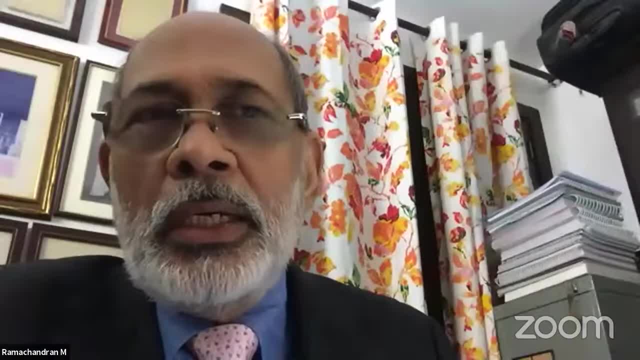 As far as our urban management process is concerned. That's all I have to say. 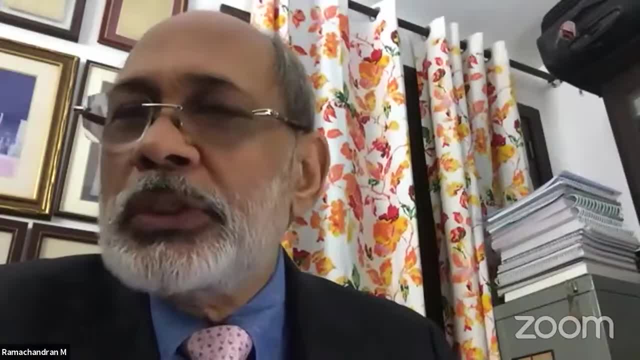 Thank you for this opportunity. I wish the deliberations all success. Thank you, sir. 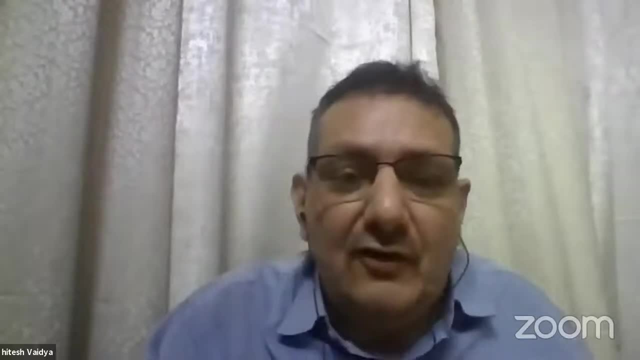 Thank you very much for a detailed, you know, points for not only how should we should build about, but also how we move forward. 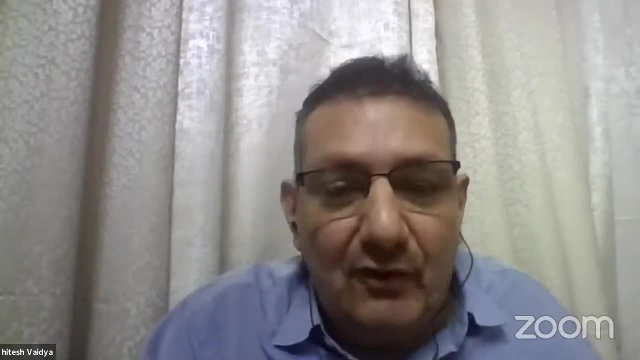 So I see Mr. Amrit Abhijat, we have lost him. He still must be the queue. So may I request Ravi to bring, Oh, Mr. Amrit Abhijat is there. Yeah, he's there. So I'm here. 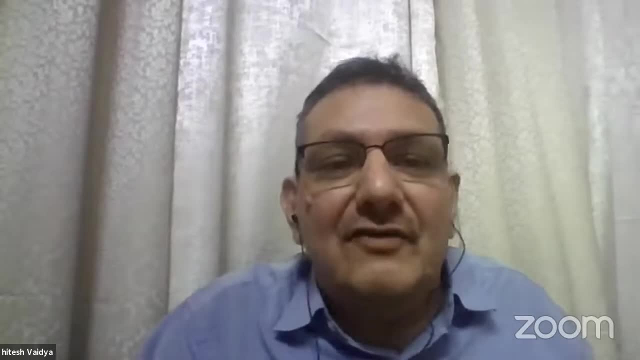 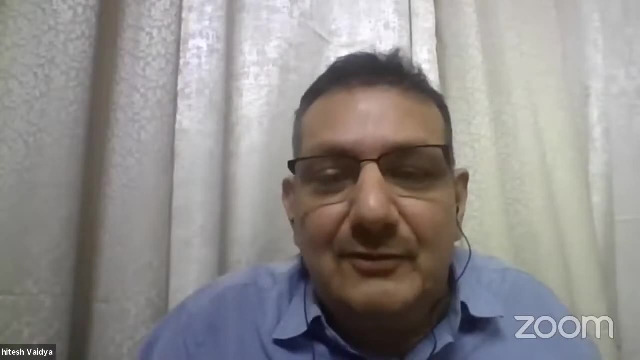 So, sir, again, Ravi, if you can quickly introduce Mr. Amrit Abhijat and then we can listen to him before we move to other speakers because it's very difficult. Otherwise, we'll lose him. 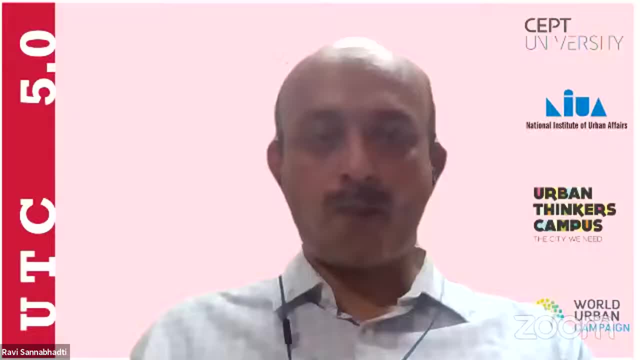 Then we will not be able to hear him. So, yeah. Yeah. 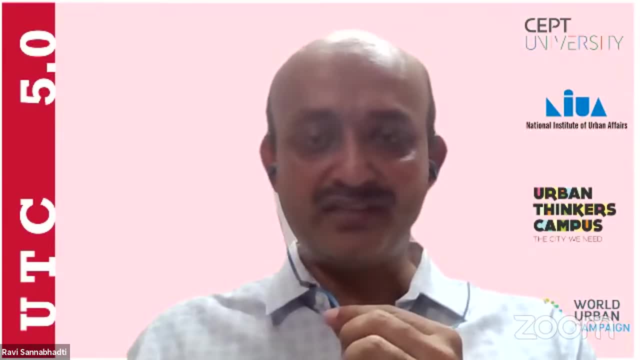 So I'll be very brief. Thank you, sir, for agreeing to be a part of this session, technical session on policy, reimagining policies. So. Without further ado, let me introduce Mr. Amrit Abhijat, who is an IAS of 1997 batch. 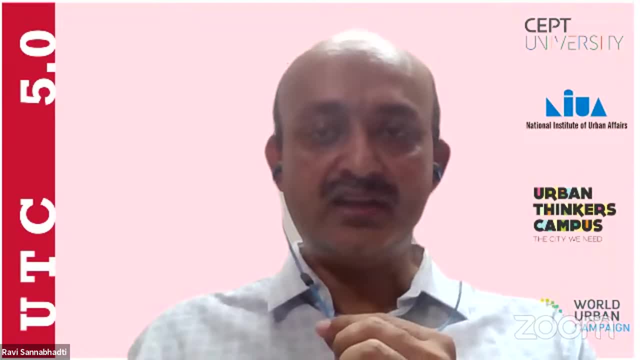 And he began his career as a joint magistrate in land revenue management and district administration at Mathura. 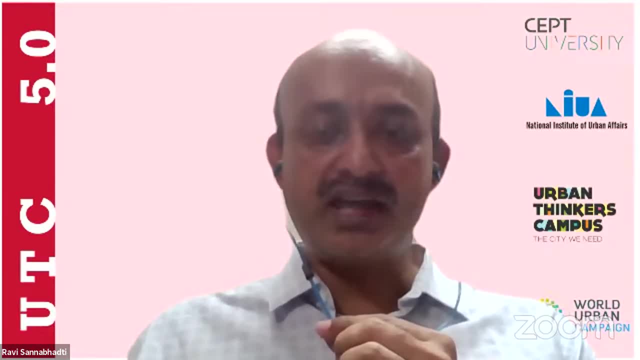 Right now, he is serving as a joint secretary and mission director in the Ministry of Housing and Urban Affairs in the government of India. 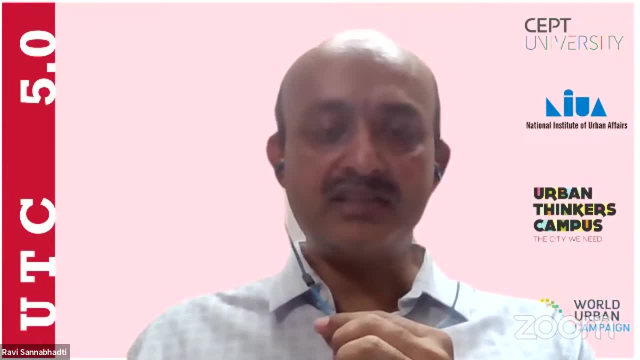 As joint secretary and mission director, the ministry, has assigned him to implement the Pradhan Mantri Awas Yojana, Urban, one of the largest housing programs in the world, with the mission housing for all by the year 2022. 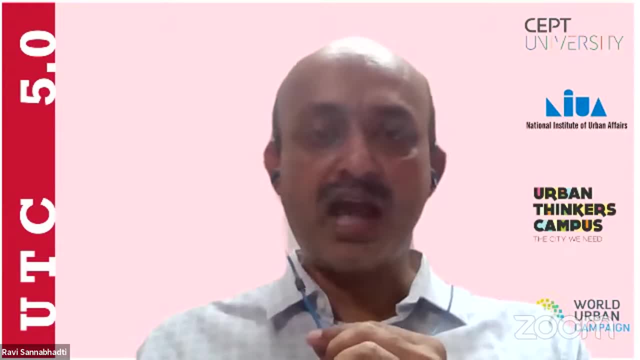 Of course, in the interim, he has served in a number of positions as district magistrate of various kind of cities and various districts. 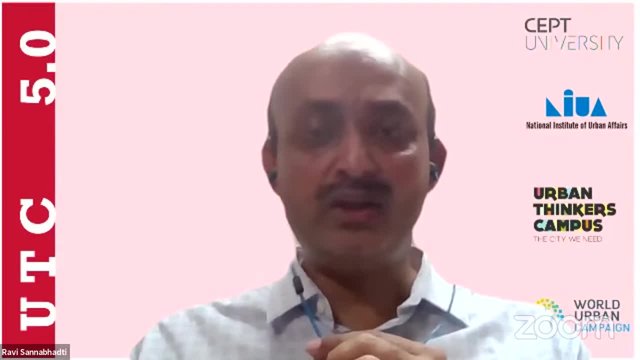 So I will not, I mean, since there is paucity of time, I'll not get into all the details of the same. But he is known. 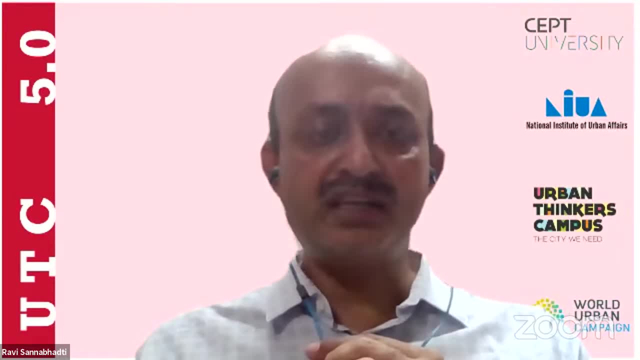 Or he has gained a lot of admiration because of his working style. And as a civil servant, he is known for implementation 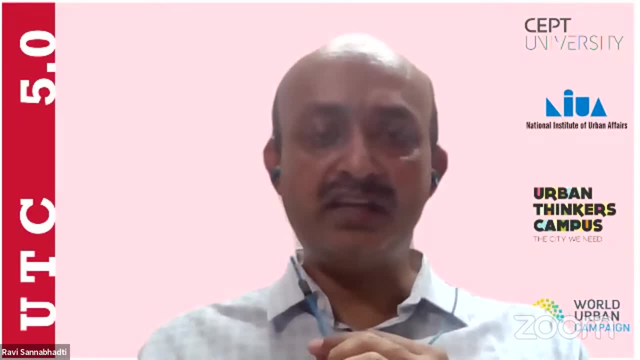 of various innovative ideas, such as Hello Vikas at Muzhavapur Nagar, to name a few, Zilla Prashasan Agra, or Facebook Agra, to create a common platform for public convenience. 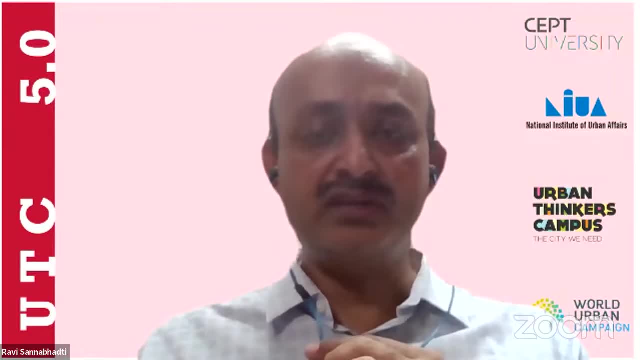 He was also instrumental in overseeing land acquisition project modalities and execution of the Yamuna Express from Agra. 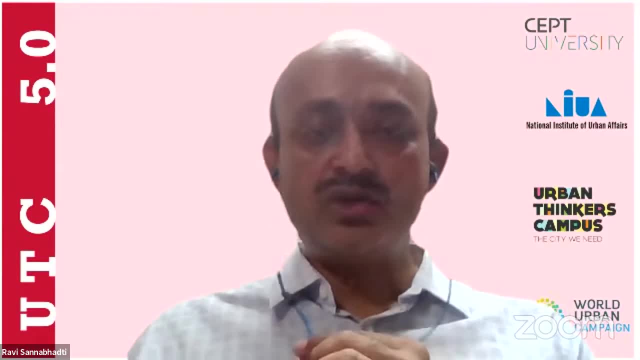 So I will not get into all the details of the same. But I would just say that recently, he also was oversaw, or he was rather instrumental in fulfilling a vision of the prime minister of holding a technology challenge on construction in Delhi as late as March 2019. So the global housing crisis is a big challenge for the prime minister. 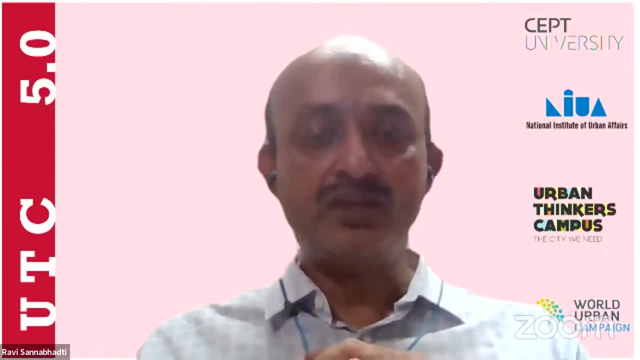 And I think that he will continue to work on this. So I will not get into all the details of the same. 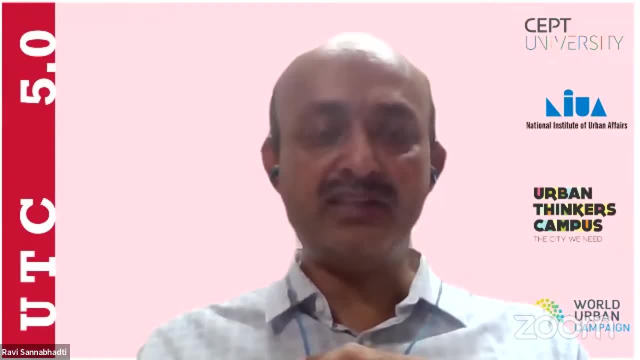 I think that it is still a big challenge for the prime minister to work on this. 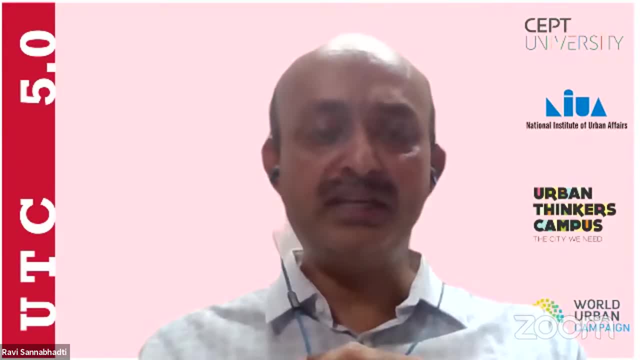 I think it is still a big challenge for the prime minister to work on this. And I don't think he can be an passport, 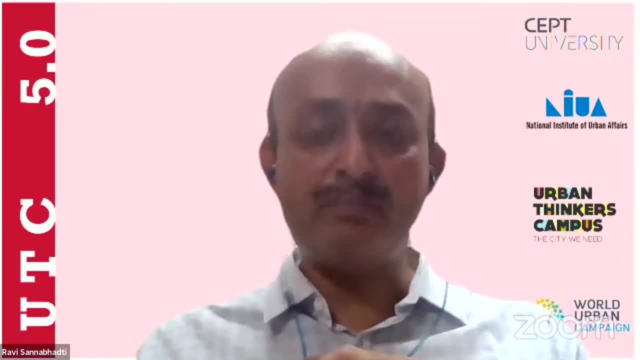 or a document, or a document or anything like that. And it's a question about the development 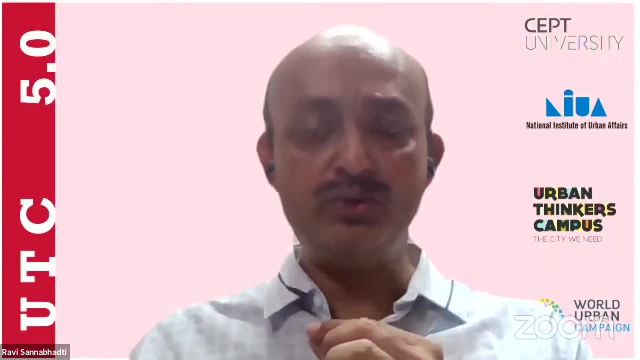 of the government and the government as you look at it, and the work being done. 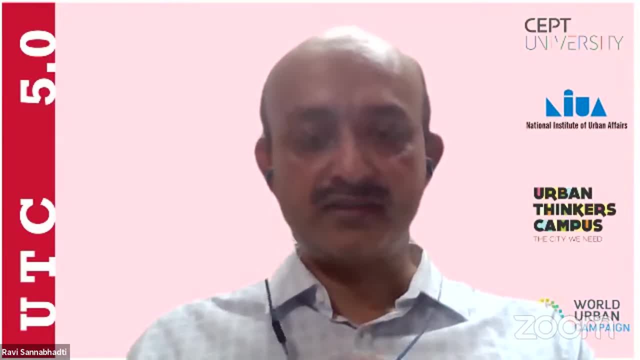 I think we are talking about a global housing technology challenge, India, which provided for an expo and conference, where all the stakeholders and exhibits in new technology, what to meet, 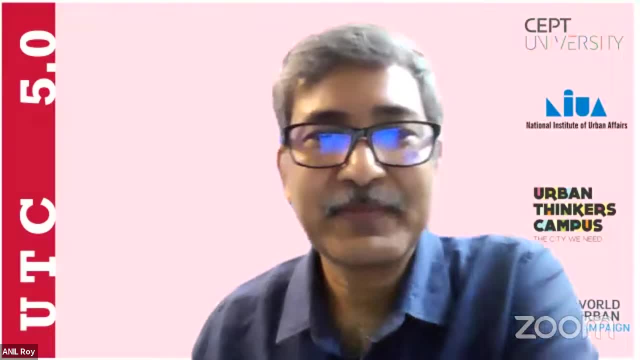 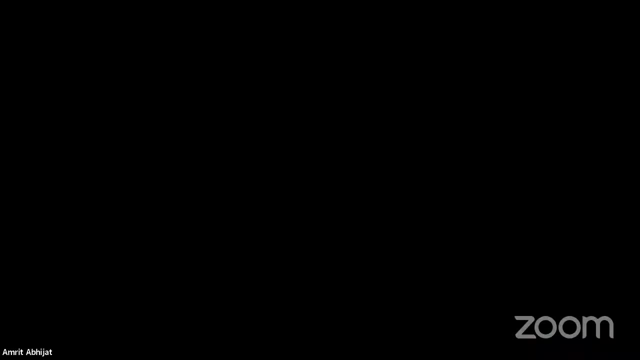 I'll be brief because I'm at the airport and I'm having a flight to catch. 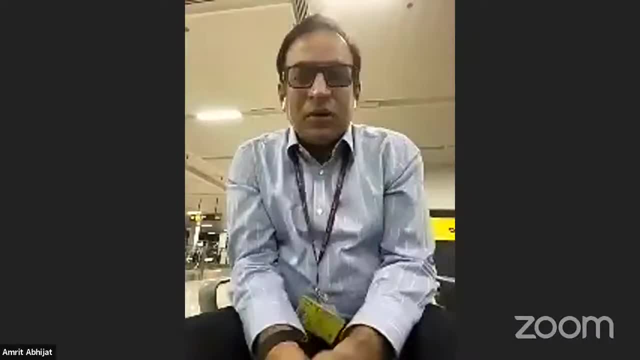 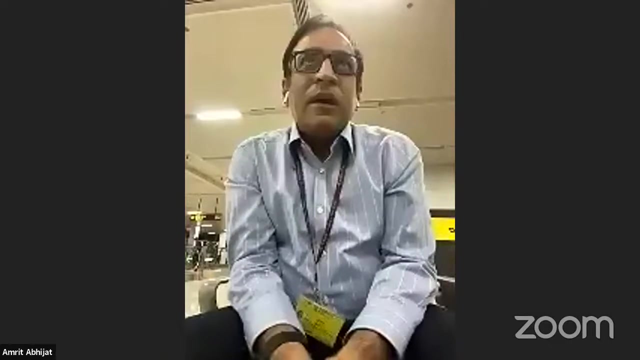 To just put it briefly, I would be speaking about the Pradhan Mantri Awas Yusra and how the journey has been for us here because I've heard the views of Professor Mathur and Ramachandan Sir who have dealt with the urban development for a very, very long time, including Hitesh Madhya Ji also. So not very much in a position to comment on large issues of urbanization and urban growth and development. It's much rather preferred that I learn from them. 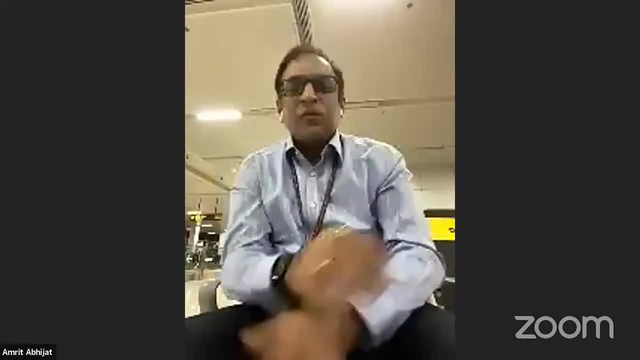 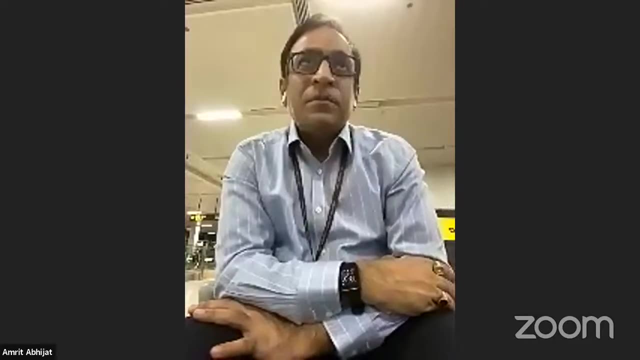 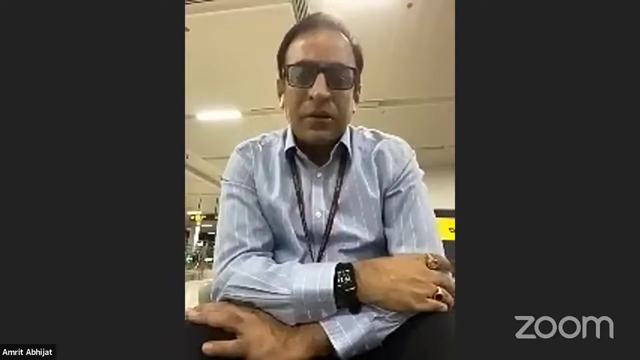 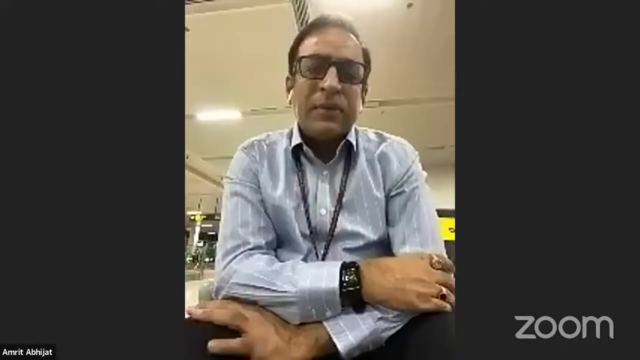 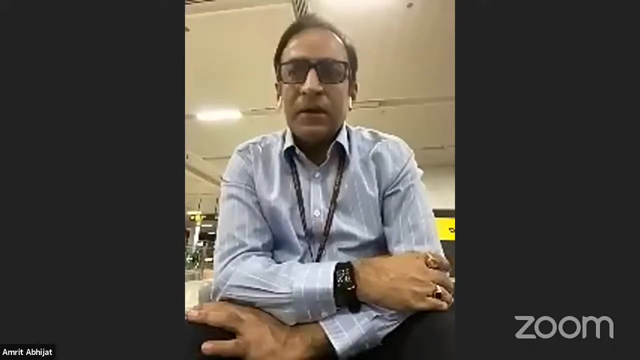 However, Pradhan Mantri Awas Yusra is the scheme that I've been seeing for close to about five years now and I'd like to talk about that, how the experience of managing and implementing one of the largest housing programs. in the world has been for me. So after the announcement of the Honourable Prime Minister in 2014-15, when the scheme came about in June 2015, we started with our baby steps and the next six months were deployed for setting up the architecture of such a mammoth mission and we literally started from sometime around 2016. 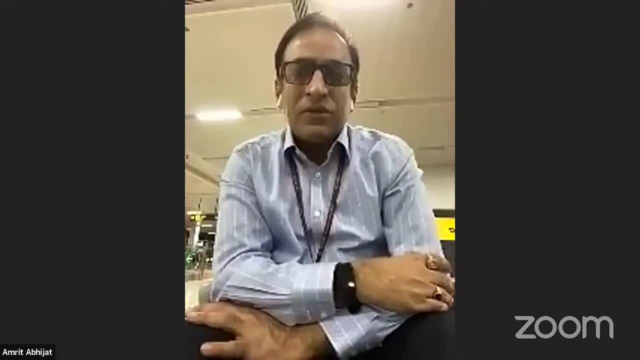 Pradhan Mantri Awas Yusra, to just put it briefly, looks at providing housing. 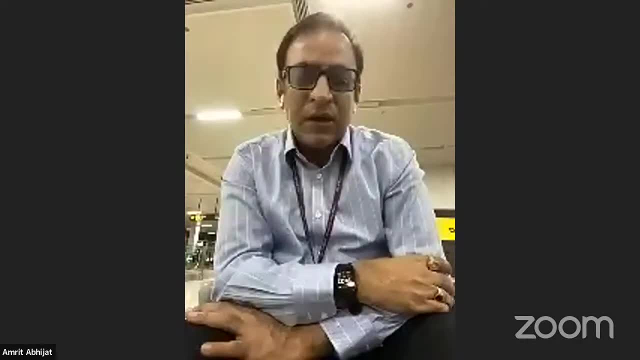 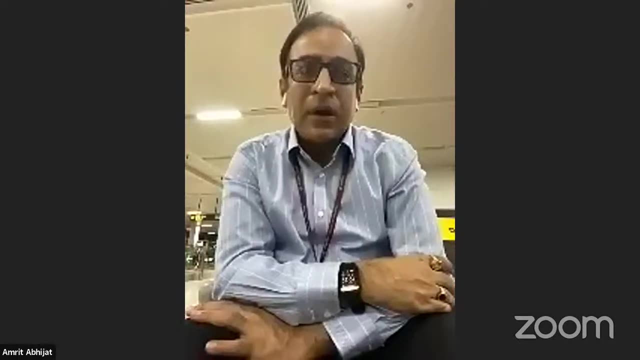 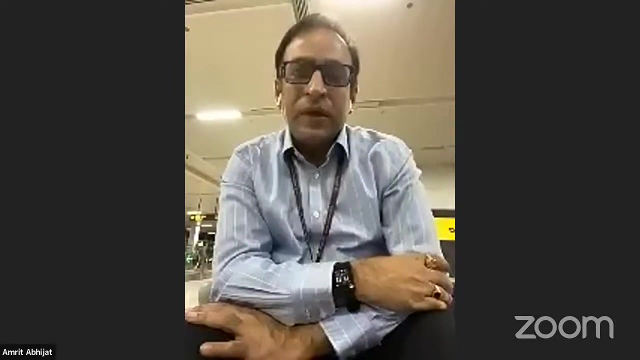 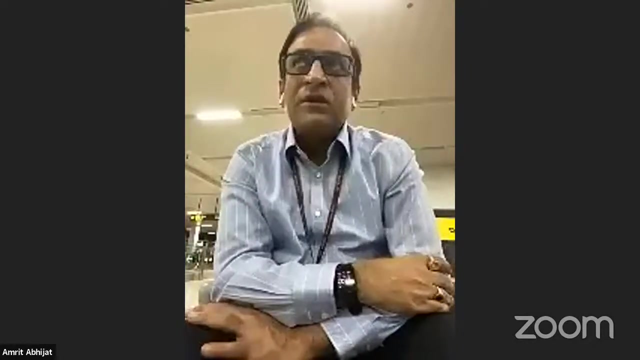 He's a fantastic person who was a very special person and I think, as I mentioned, he has been with us for a long time in this process and the last five years of my work has been really incredible for me and I think it has been very important for us because I'm really talking to the people who are helping people when they are having a hard time in the city to come up with solutions. This is an extremely important part of our efforts. So I'll just continue. Pradhan Mantri Awas Yusra, I'm always happy to talk with myself and I've personally been very impressed by the work that you do with the government and the government itself and also the Banvera Foundation. 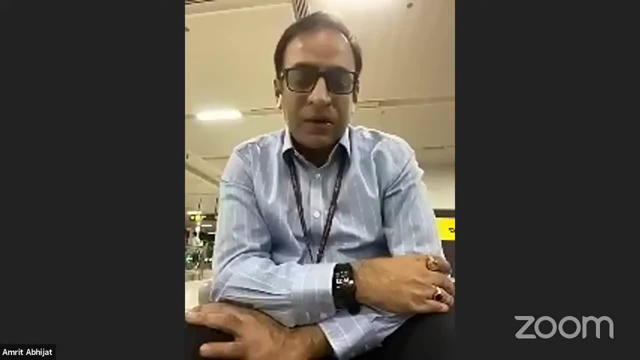 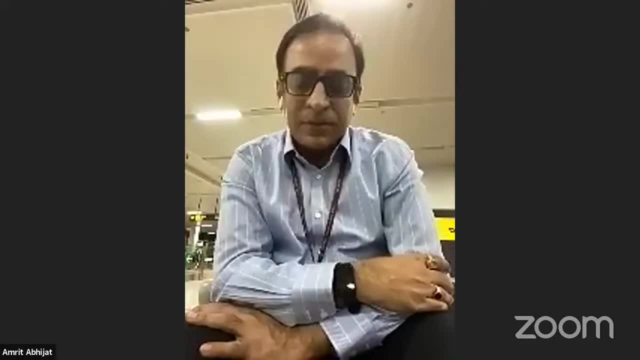 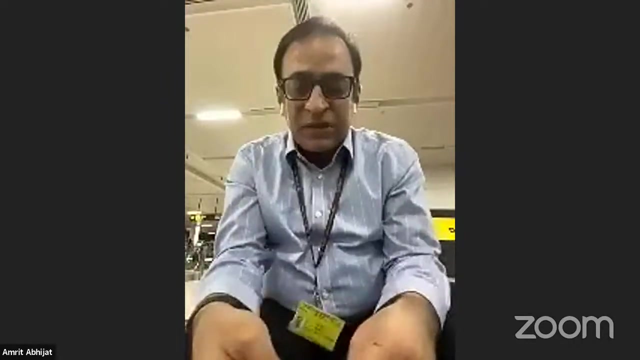 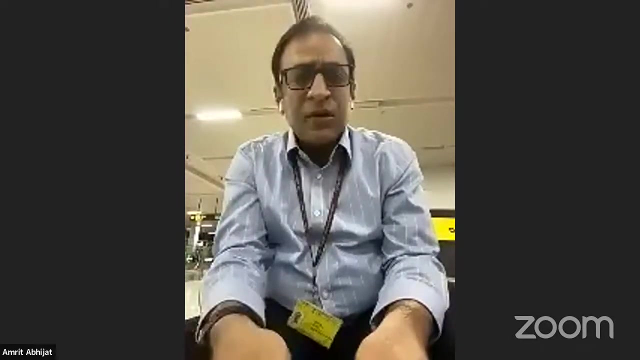 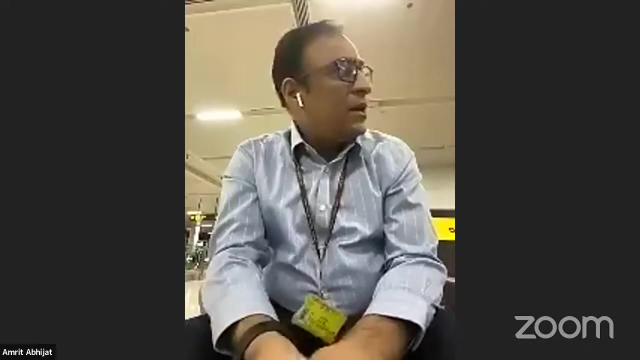 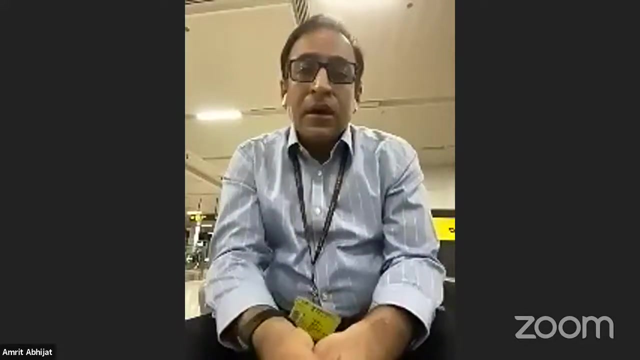 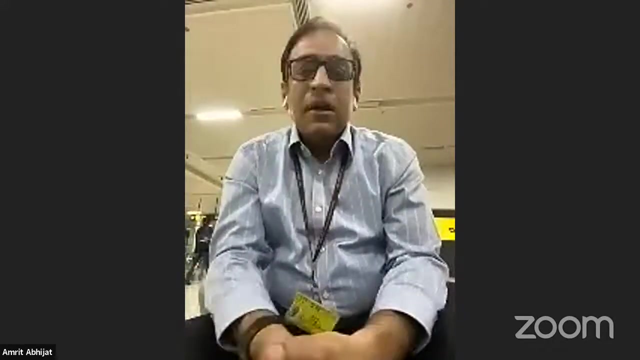 Thank you. Thank you. the largest program or in affordable housing in the world the scheme uh emanated from the experiences of the earth's wild gene in the arab scheme and other schemes like ray and nishap where it was felt that in order to make it much more comprehensive we will perhaps have to take a cafeteria approach of how to go about making this a success because it was seen that slums alone is not perhaps the problem but the with the urban growth industrialization and modernization and the growth of the service industry with large number of people shifting from rural areas to the urban areas it was well like uh imagined that we will perhaps need to have a multiple approach in developing what the people required and therefore we had four verticals in the scheme the beneficial in contribution followed by uh the uh 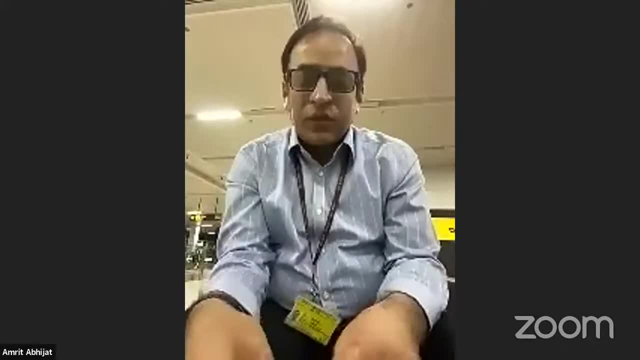 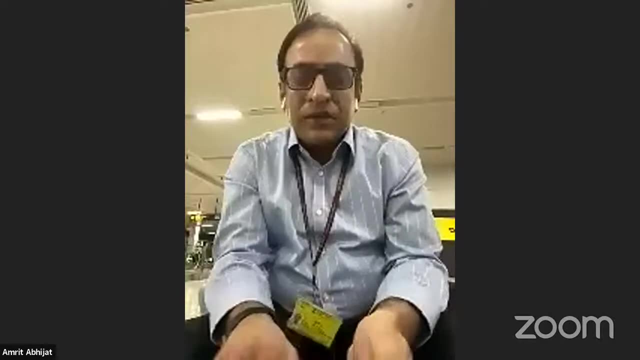 issr credit link subsidy submission and of course uh the uh clss which is the credling subsidy so uh this being the case uh we started off and it is very very important that we had element of 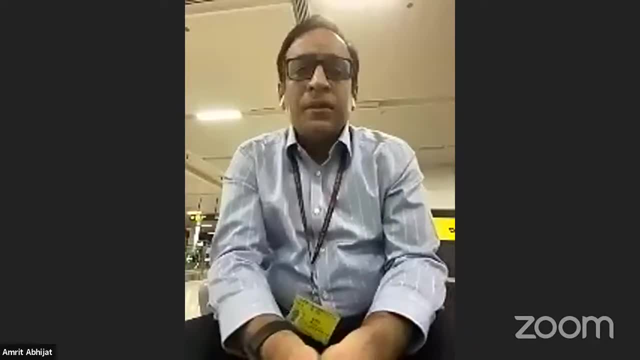 technology in built and about close to 15 lakh houses are being made uh under the scheme just 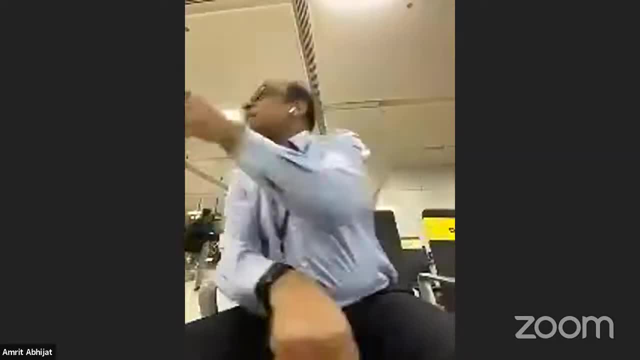 like that i think my boarding is taking place but lucky body okay okay so all in all i'm just to say 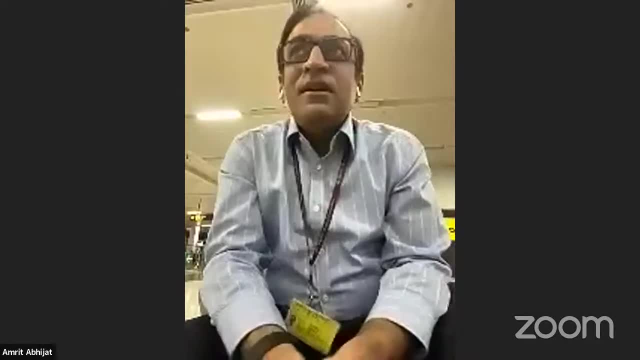 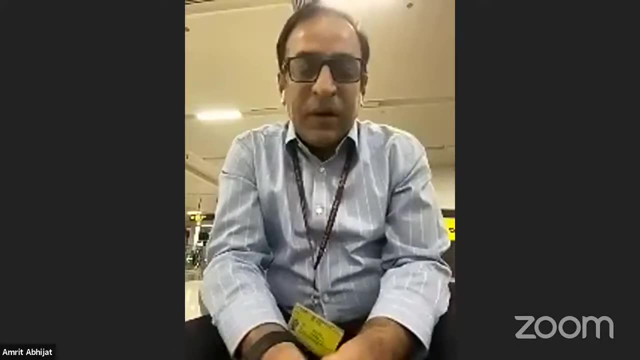 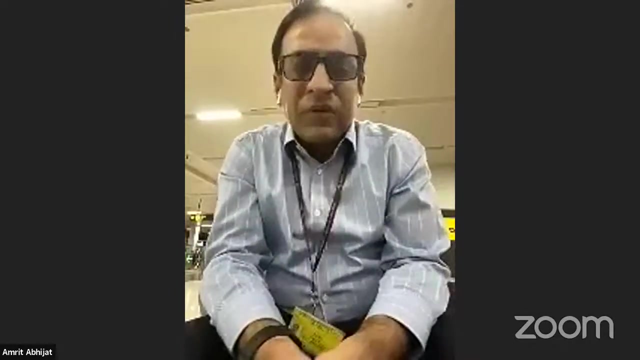 that uh the board has not been fantastic but we have a huge journey all the states have participated i'm sorry the boarding has begun and probably perhaps there's a gate change also but it's been worth the while all the states have participated i would imagine that the the success of pmy has largely been on account of the fact that the beneficially contribution made it possible 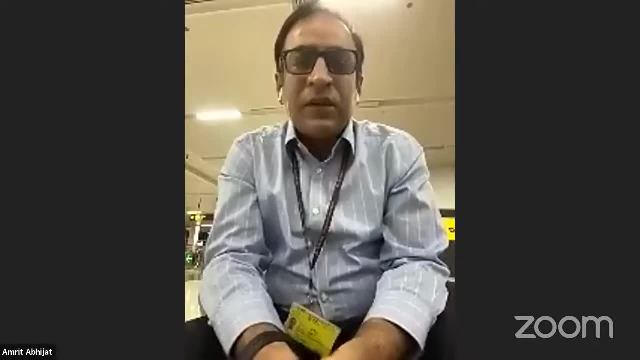 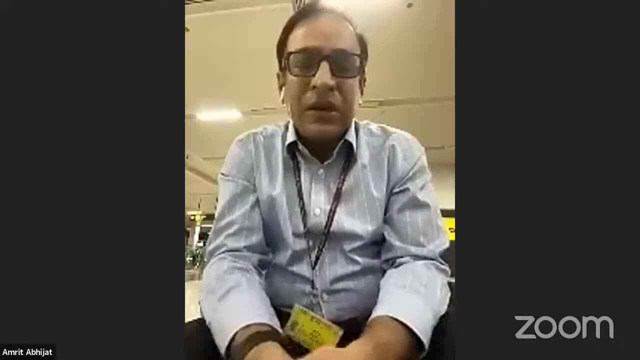 for people to invest of their own in their own piece of land and perhaps make a house of their own with the central and the state assistance credit link It was basically between the banker, builder, and the beneficiary. 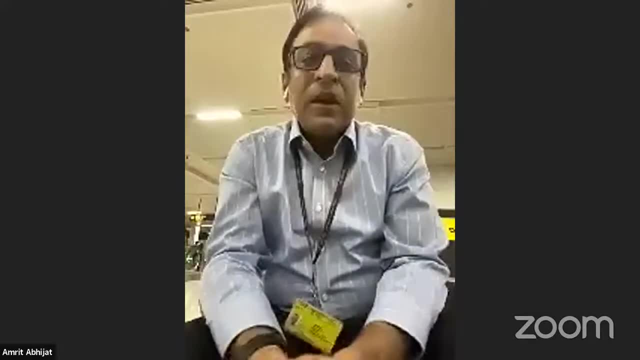 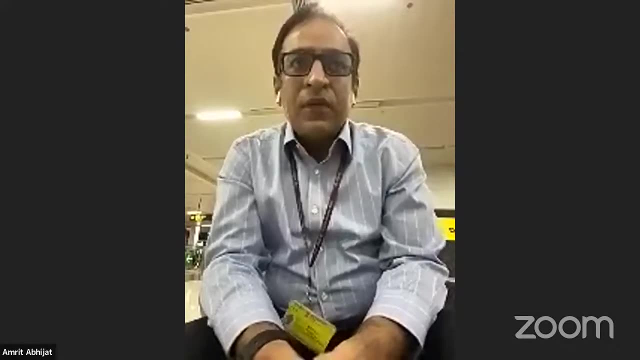 And ISSR is something that this platform is imminently capable of delving into because ISSR, I think, was a slow starter and we really need to do something. 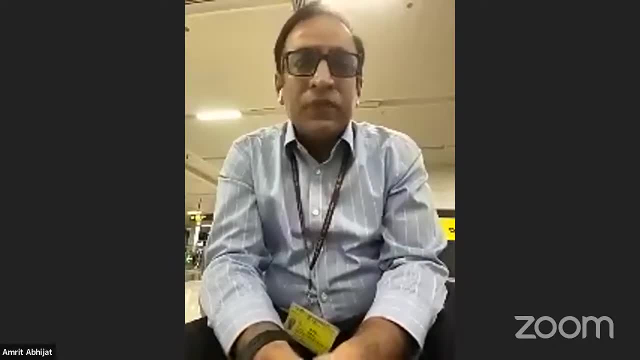 And the ministry is considering some inputs which may come up to be able to take care of the slumps that we have. 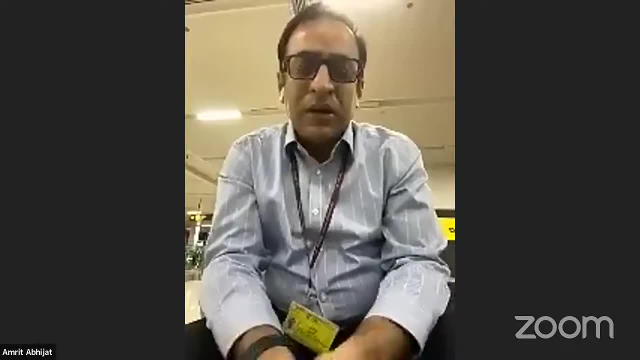 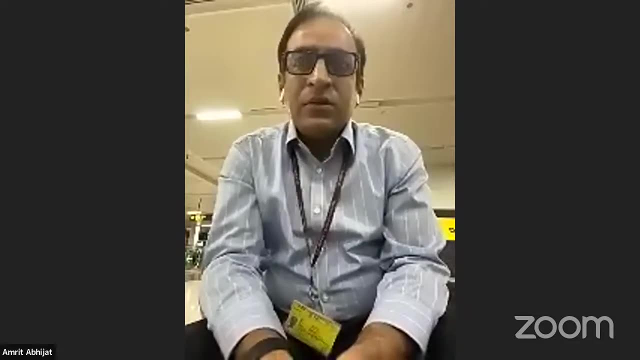 In the country, the AHP vertical was very, very good. And perhaps also in the western states of Maharashtra, Gujarat, it has done. This is, I believe, all I can deal with it. 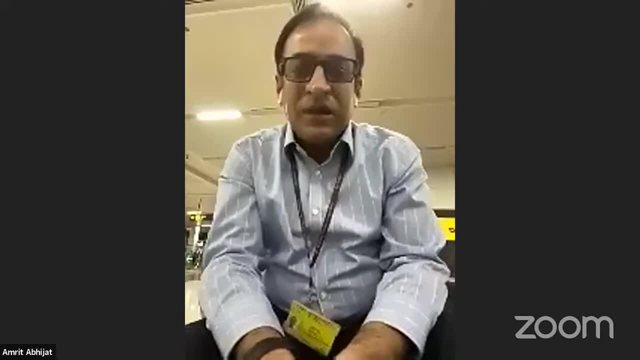 Another PMEY is the other functions of the other ministries' schemes and it makes it holistically possible for a total urban growth rather than just providing a house. 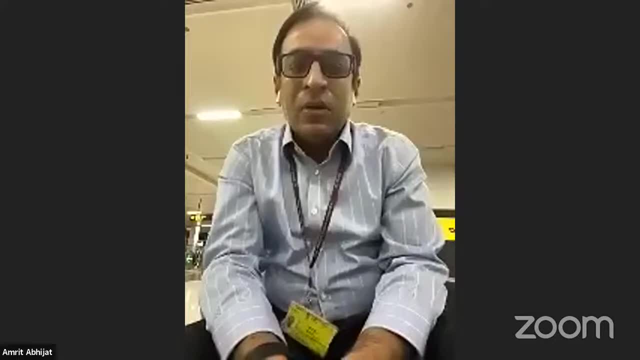 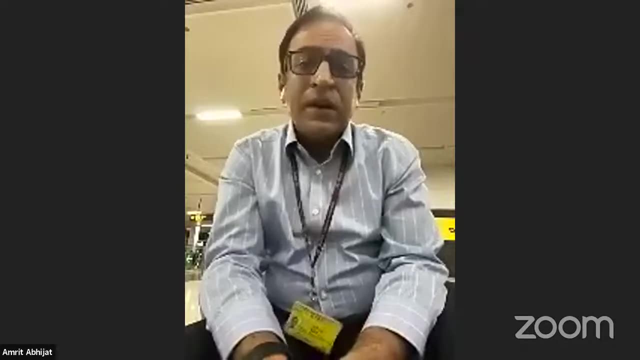 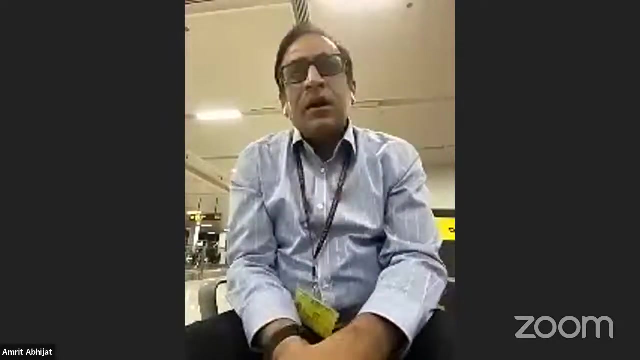 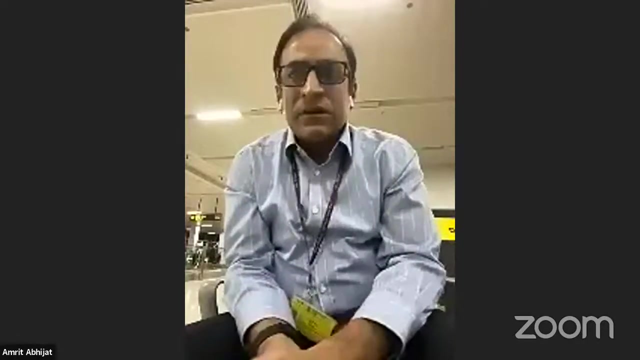 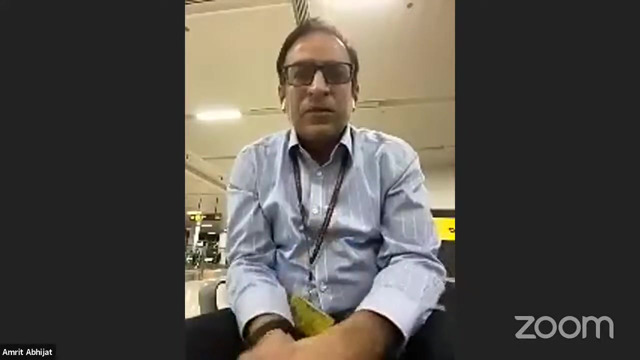 Very lately, we have done the ARHC, Affordable Renting Housing Complex, which... is an initiative that came out of COVID, but perhaps it was a felt need that was there for a very, very long time because rental housing is something that we did not address comprehensively earlier on. And though it does not address the rental housing question in entirety because that is something that the ministry is still working on, this ARHC scheme caters to the migrant population, whether they are the workers or industrial staff or salespersons, students, lay tourists, communities, which do go to cities on a migration basis. And they often have to shell out a large amount of money or stay in slums or informal settlements. 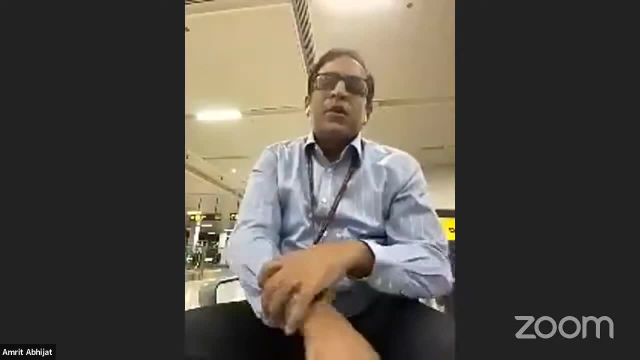 So it is becoming possible for the private entities as well as the government bodies through policy initiative without having to pay much. 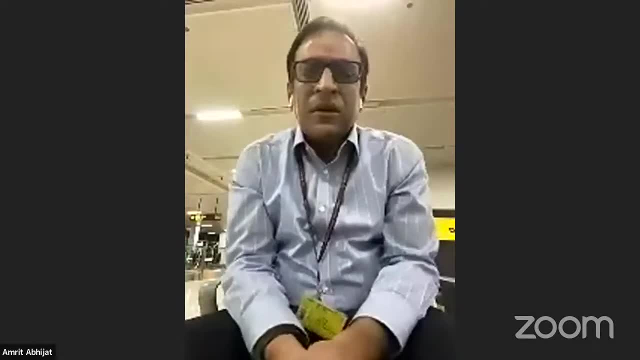 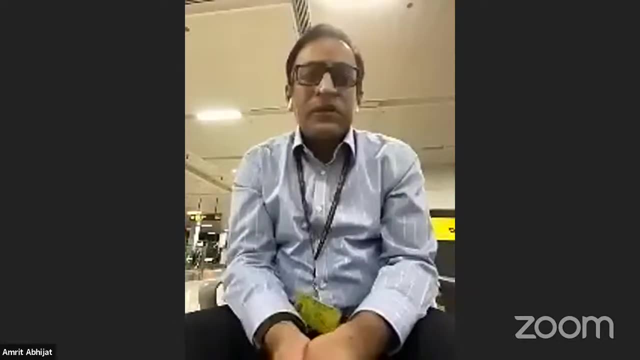 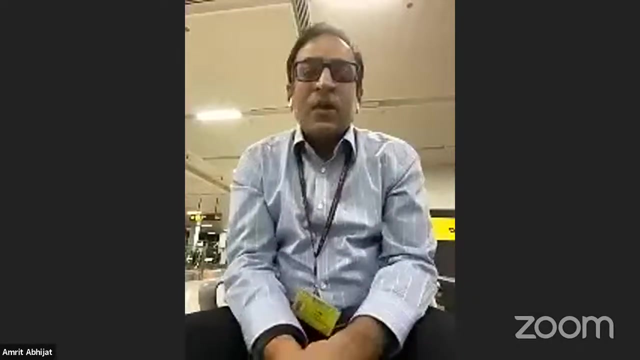 But through policy initiative, we have ensured that the IRR, the incremental rate of return, is very, very well laid out. And it becomes very attractive for the investors as well as for the governments and perhaps also for the beneficiaries to be able to shift to these rental housing complexes and work from areas which are very close to their localities. 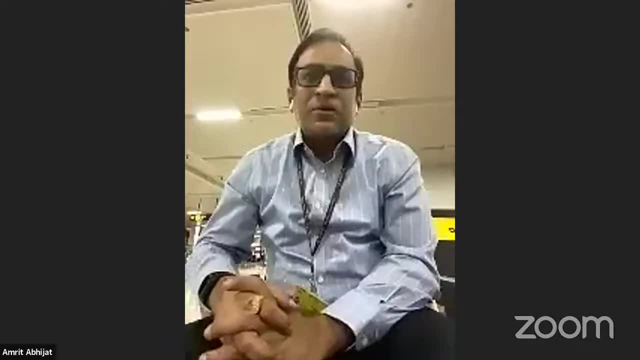 The incentives that we are offering are on GST, on income tax, on FIR, FSI. We are also offering a technology innovation grant. 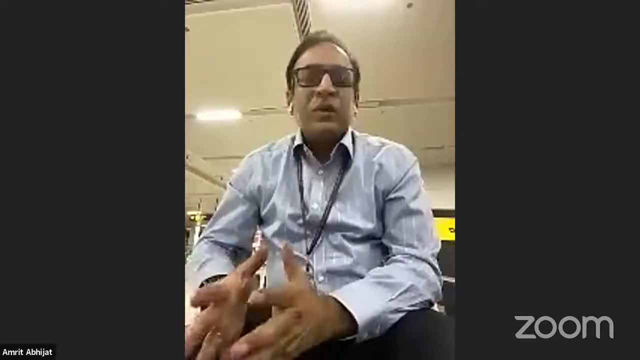 There are other kinds of benefits that accrue from this. And the rentals are, of course, at the lowest affordable rates. So this is largely the ARHC policy. 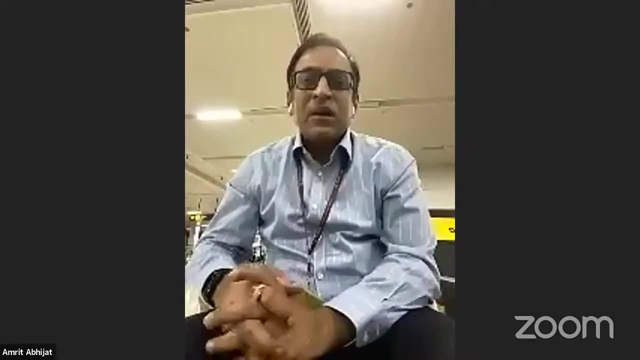 And we have done close to about 67 lakh houses are being constructed. 38 lakh houses have been delivered. And out of the 108 lakhs that we have approved so far, out of the target of 112 lakhs. 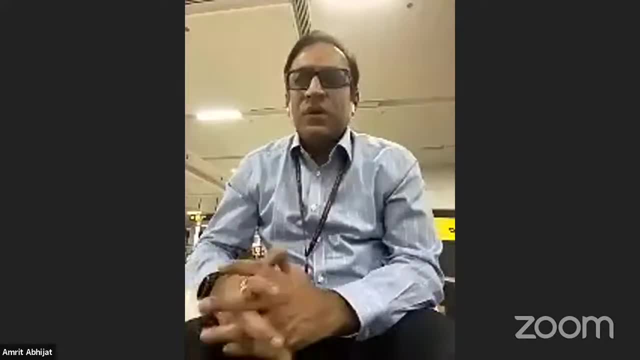 As we move on, there are challenges of finance, challenges of delays because of COVID. But we are very certain that we will be able to meet the target well in time. 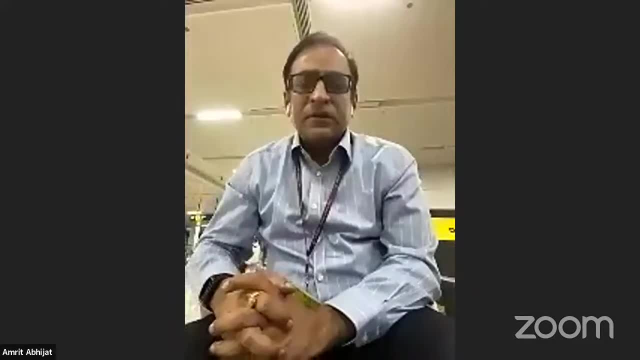 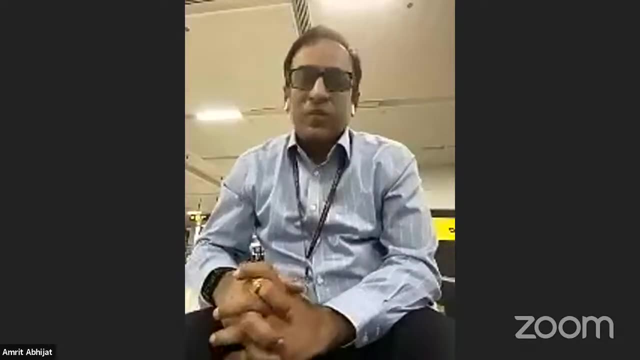 And we are very proud that the states, the people of this country have participated wholeheartedly in this program, not being an incremental housing, but being a very, very comprehensive, well-led up program. That's all I think I can afford right now. Thank you very much. 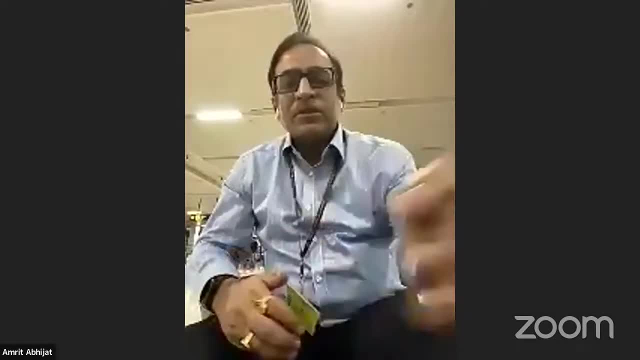 I'll be just moving to take my flight to Patna. Thank you very much. Thank you, sir. Thank you very much. 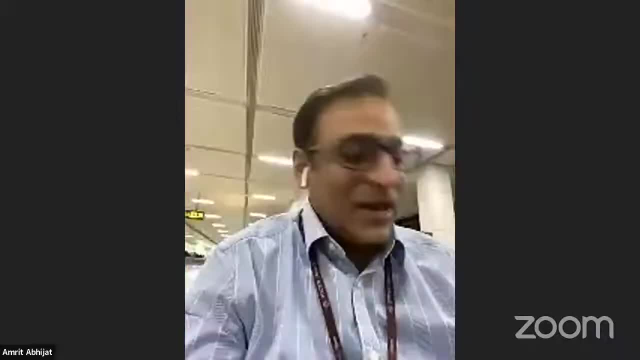 And thank you for spending time and joining us. Thank you. I'll have to rush up. 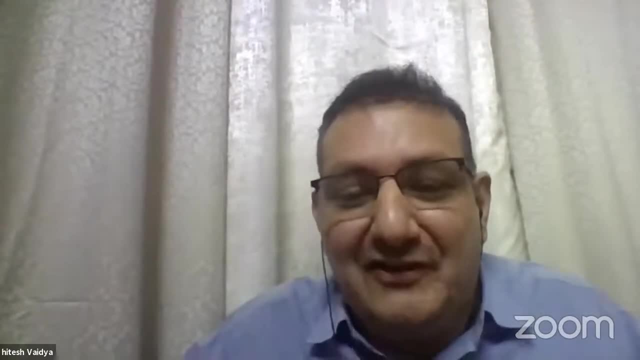 You really lead for a reimagining how we should reimagine the transformation of urban India. Thank you for being with me. Thank you very much. Thank you. Thank you. Bye. Thanks. Bye. Happy journey. Happy journey. Yeah. 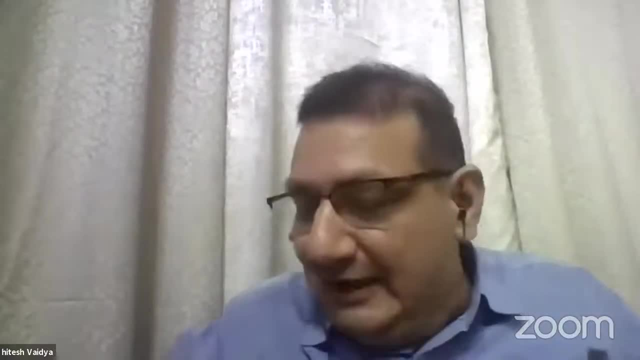 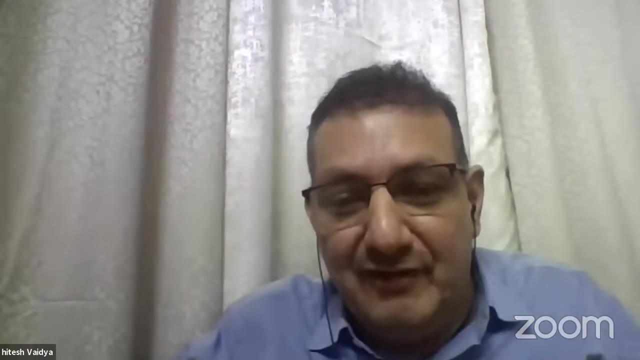 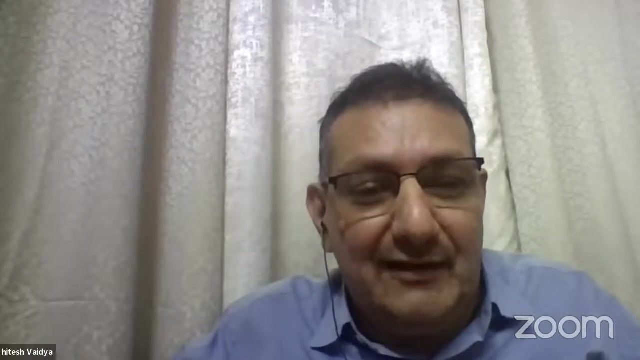 So now, you know, we are the next speaker, which we have, you know, we I've been lost in this whole COVID. The one thing has been the Zoominars and webinars, and I have been moving on from the daring cities to the practical cities, to the inclusive cities, to the resilient cities and number of cities. But I particularly, yeah, I think we'll take instead of daring cities. We need a daring thought leadership. 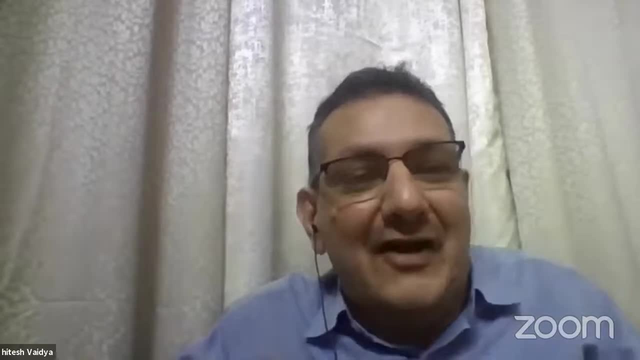 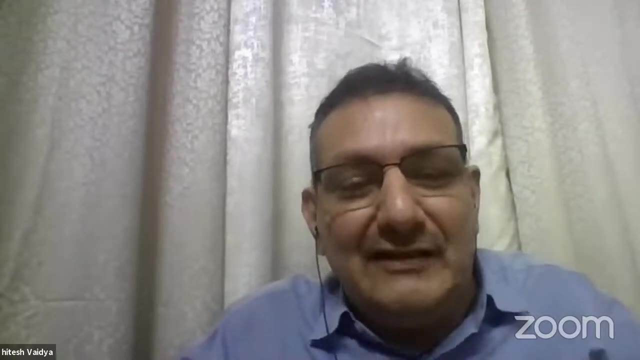 And now the next speaker, I will ask Ravi to introduce is Sheila Patel, who is, you know, brings this whole daring thought leadership towards the new or reimagining of India. So over to you, Ravi. Yeah. Thank you, sir. 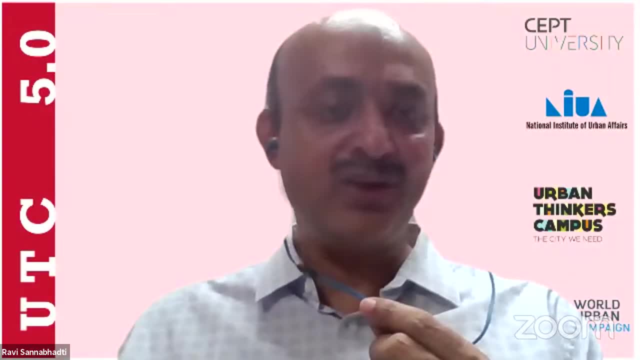 So I have the honor. of Introducing Sheila Patel, who is the Founder Director of the Society for Proportion of 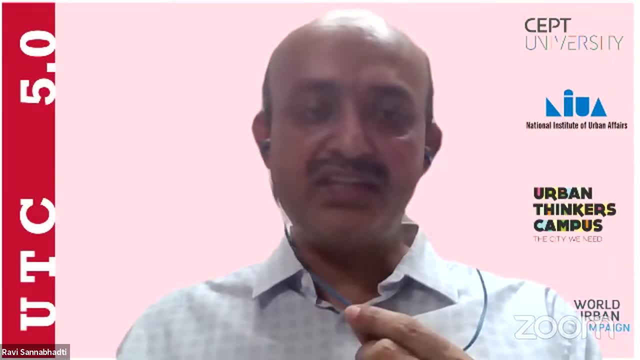 Area Resource Center, also known as PARC, an NGO that has been working since 1984 to support community organizations of the urban poor in their efforts to access secure housing and basic amenities, and also to seek their right to the city. 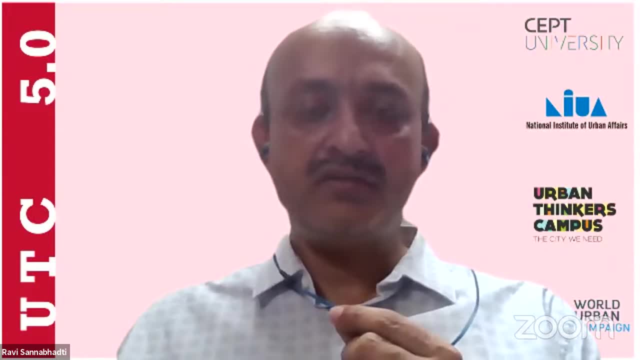 She is widely recognized nationally and internationally for seeking urgent attention to the issues of urban poverty, housing, and infrastructure, and bringing them to the radar of governments, bilateral, and international agencies. 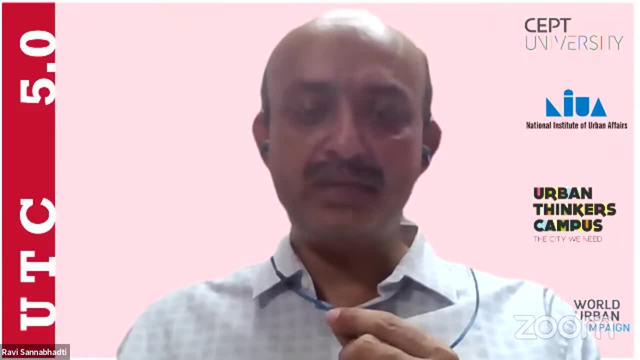 SPARC has also been working in alliance with two community-based organizations, National Slum Dwellers Federation and My Lump Dunn, and as a collaborative, they are active in 70 cities in different states of India. 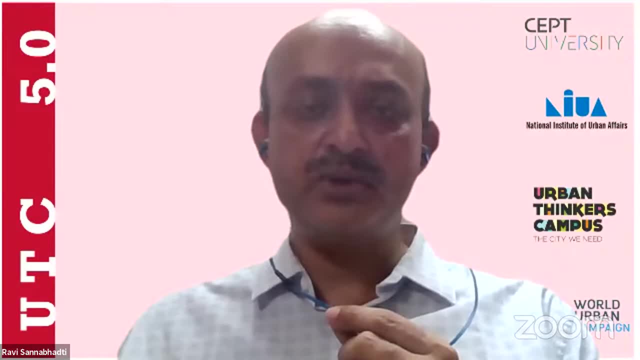 Since 1999, she has also been Secretary and Chief Executive of SPARC, Samudha, and Nirmal and Sahayak, a non-profit company set up to assist slum communities take on construction projects in cities to provide slum dwellers to build homes and sanitation for themselves. 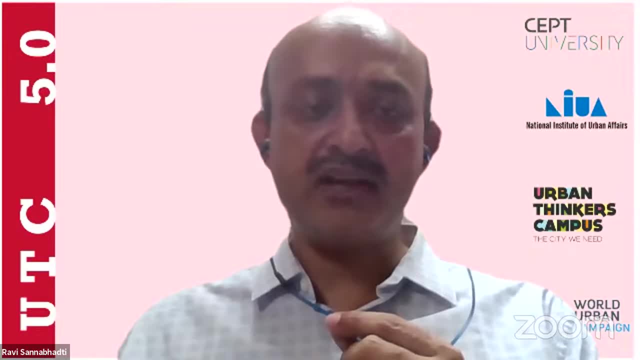 She is a founder member of the Slum or Shack Dwellers International, an international network of poor people's organizations and NGOs that support them in Asia, Africa, and Latin America. So she is currently the Chairperson of SDI also. 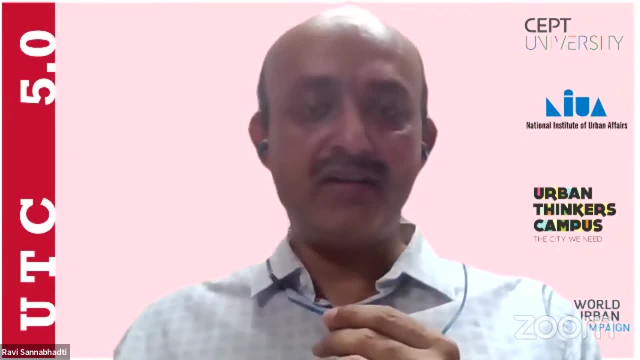 It's an honor, ma'am, to welcome you to this and look forward to your address. 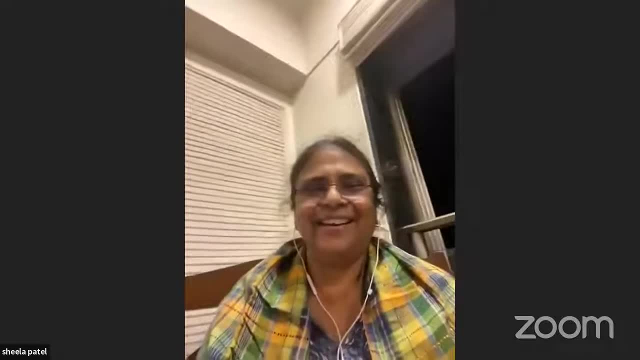 Thank you so much. Thank you. 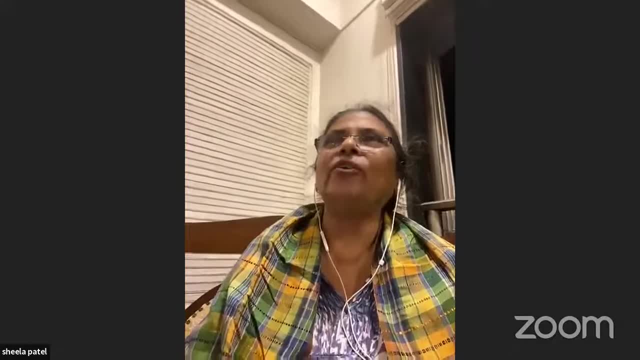 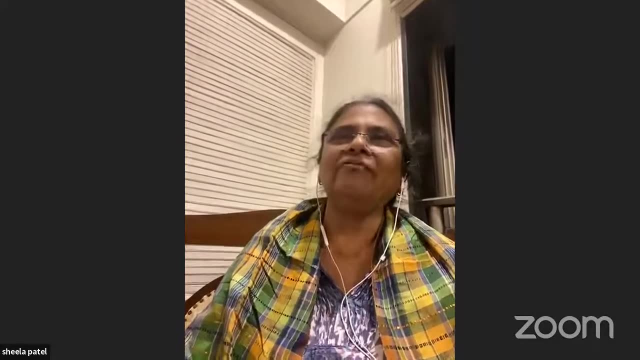 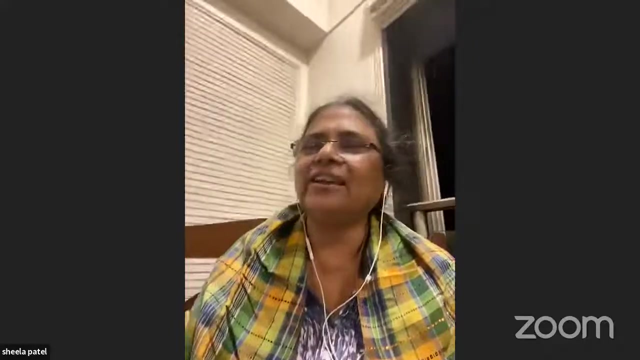 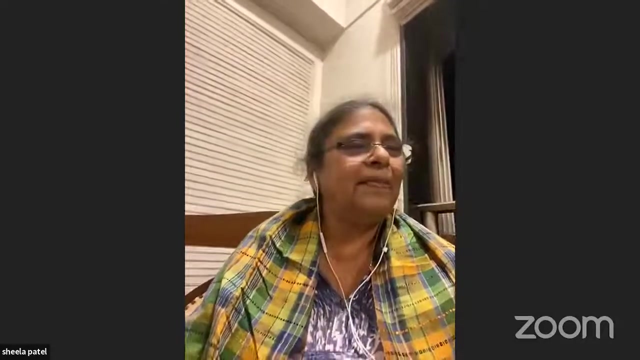 It's a very strange situation to follow three speakers, two of whom I have worked very closely with, Professor Mathur and Mr. Ramchand. When I was part of the JNNURN group of people advising and participating in it, those are old days. 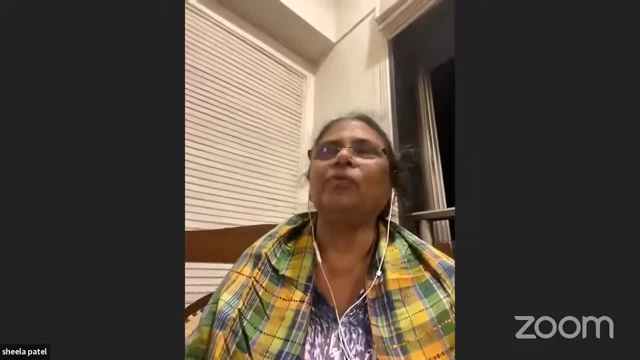 And I think my role in this particular group with whoever has been, I'm seeing a lot of 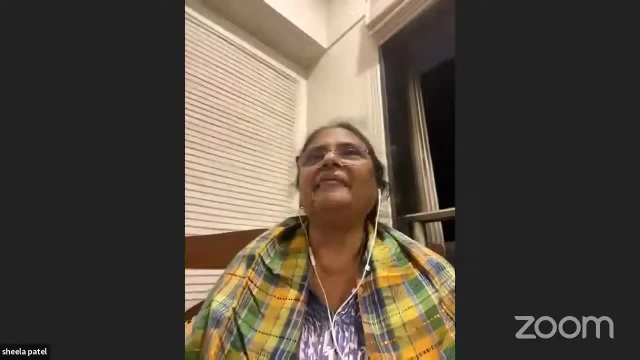 people have left, but whoever is there is to be disruptive. 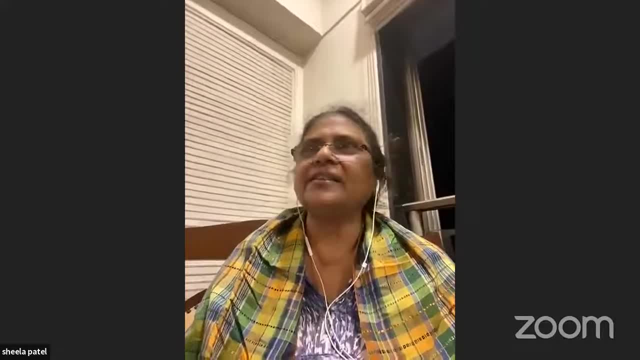 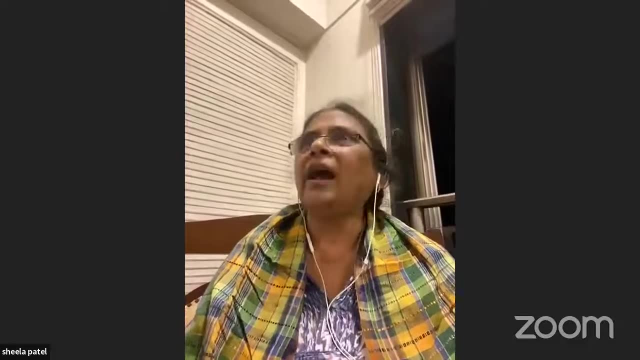 We've heard too many prescriptions. Too many. Too many points of views of what should be done, who should do what, how it should be done, how we should be proud that we are the largest program. The point is that we are a country of 1.3 billion people and we have officially about 38% to 40% people living in cities. And we have two more. Two more. So that's it. Thank you. 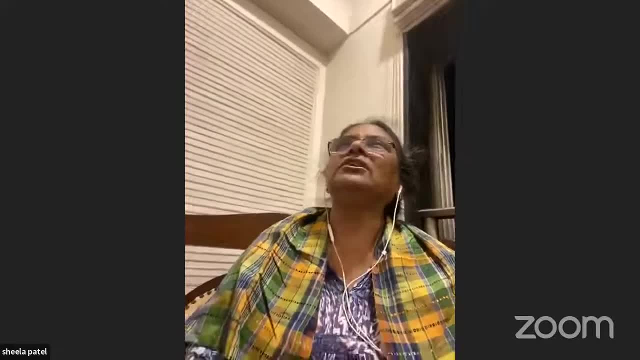 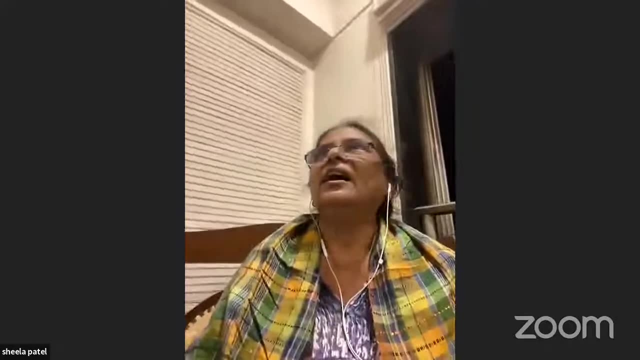 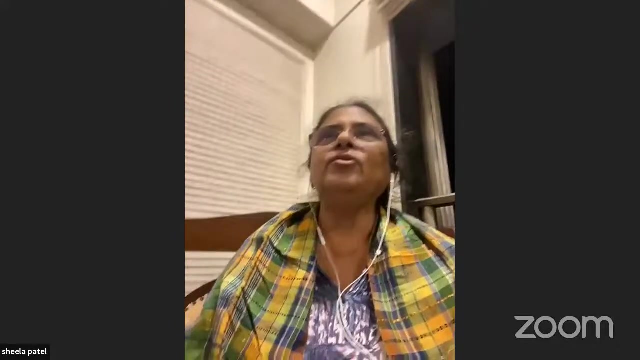 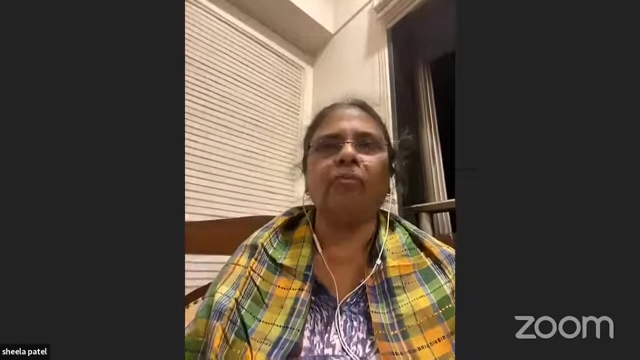 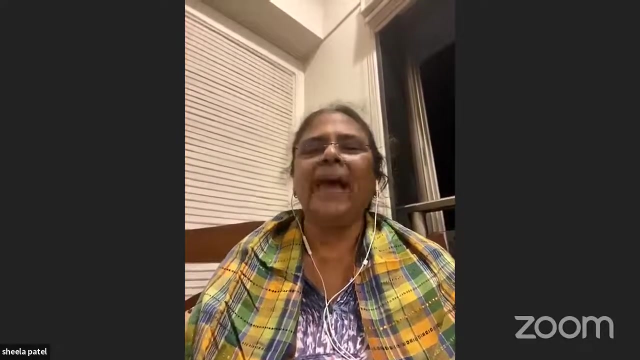 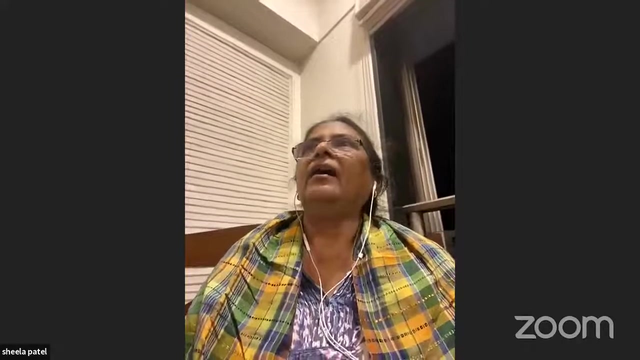 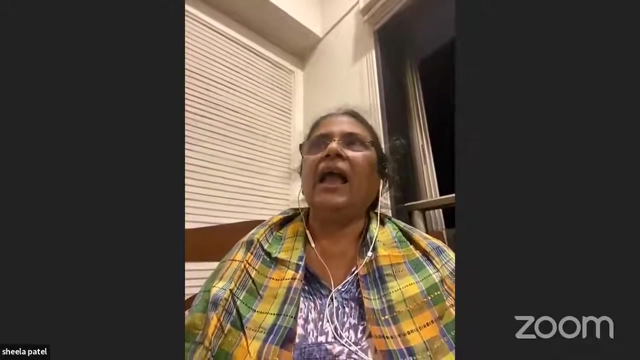 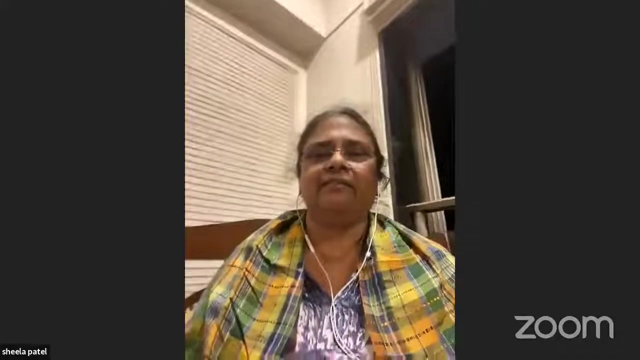 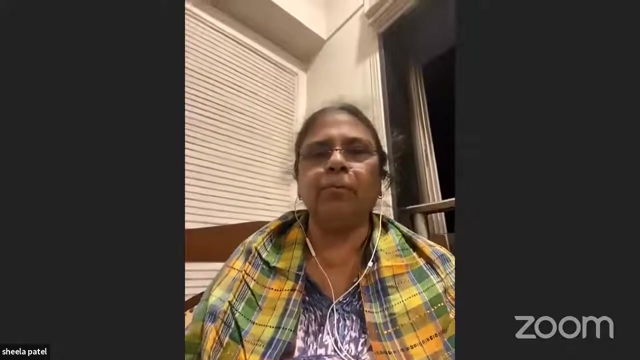 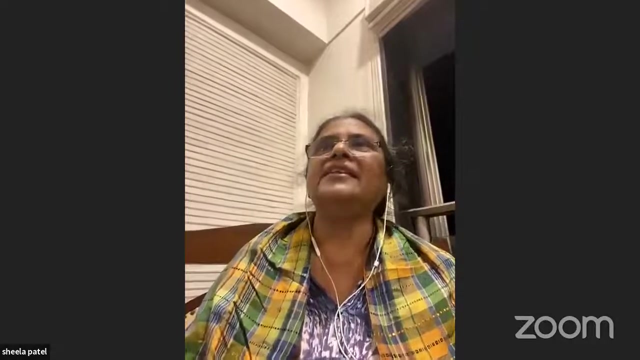 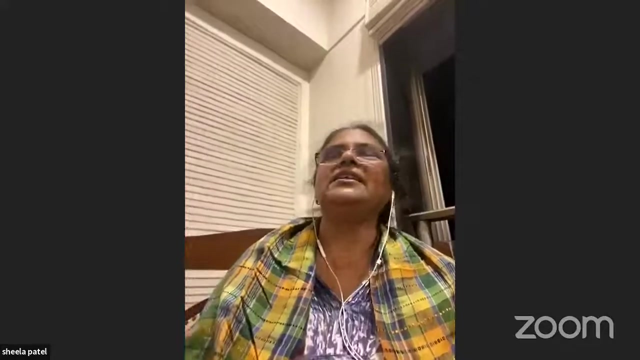 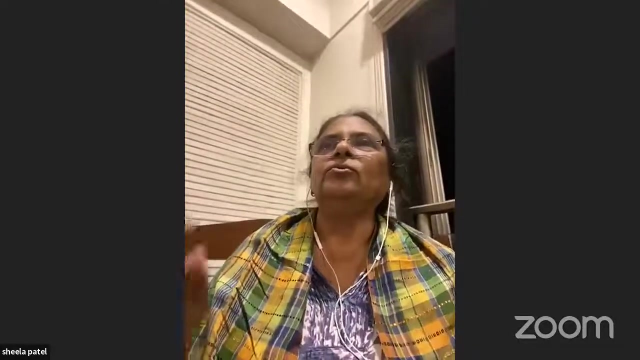 200, I think 2,000 city, 2,000 towns, which state governments don't decide that they are cities and they are large villages. And we talk about technology, but we cannot seem to extract enough knowledge to acknowledge that 40% of these 40% living in cities are living informally and that number is growing exponentially. So what is the community of planners doing? I think you are all trapped in the 18th century. When COVID came on, I was listening to the history of epidemics. And the laws that have been enforced nationally today are the laws of 1895, when there was the plague epidemic. And the whole culture of planning, which we first imported from Victorian England, still remains the basic fundamental tablet in which the formal city is serviced by the informal city through land titles that were given to those who were partners of businesses. 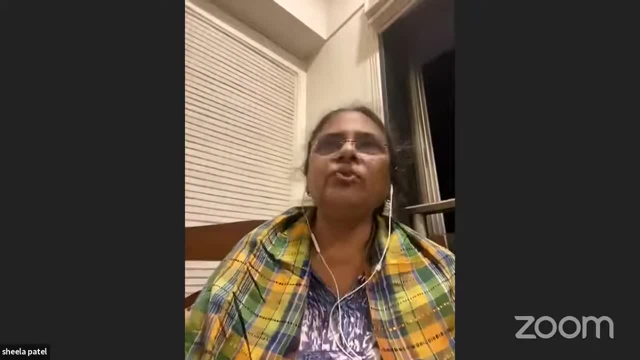 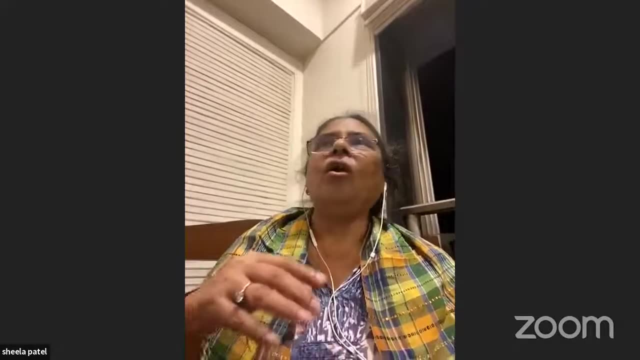 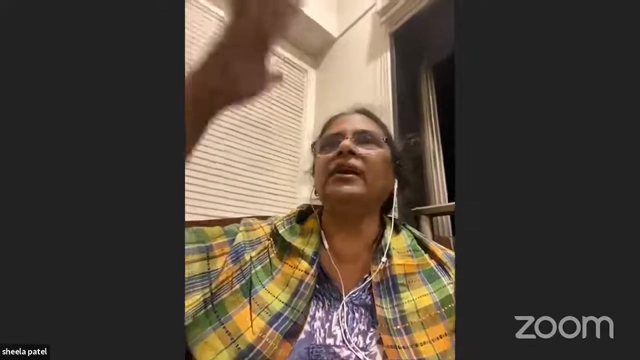 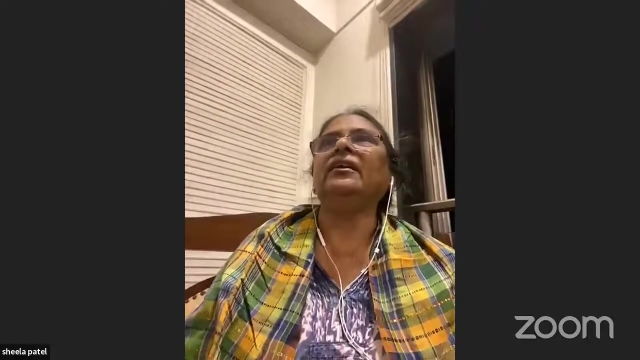 And even today, the land ownership remains the same. So without all this fanfare of data, statistics, mapping the universe through satellite imagery, we still are not acknowledging the tenets of citizen rights. 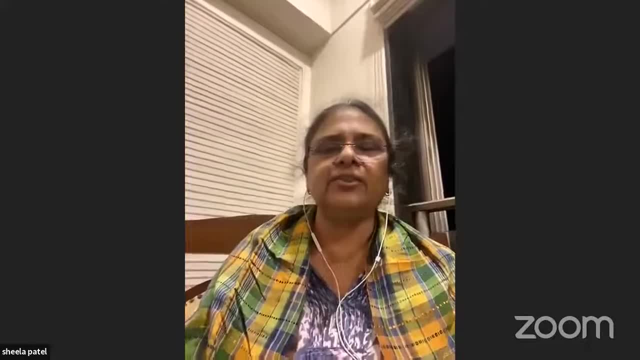 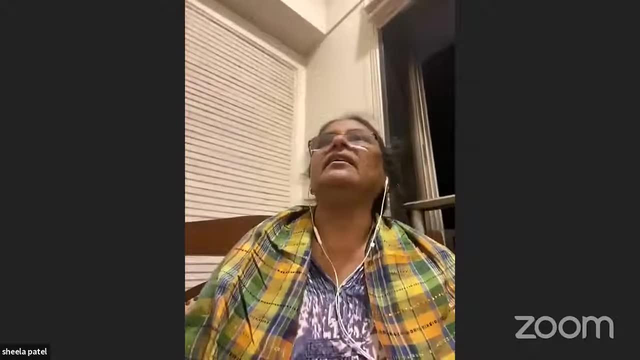 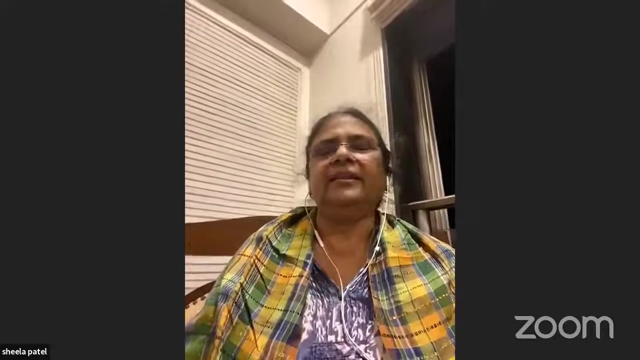 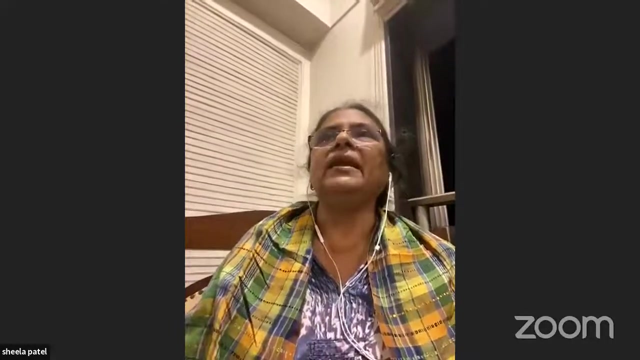 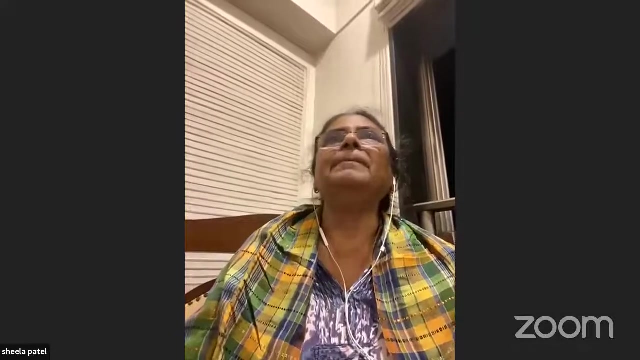 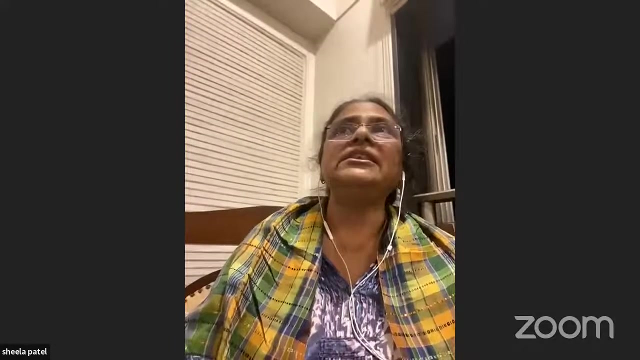 To what constitutes the majority of people living in cities today. And every single planning professor, educator, and student has to feel deeply apologetic that you have institutionalized a system in which this exclusion is legitimated with evictions, with non-investment. And with complete, complete and total lack of acknowledgement of what the informal sector contributes to all of us who live formally in cities. 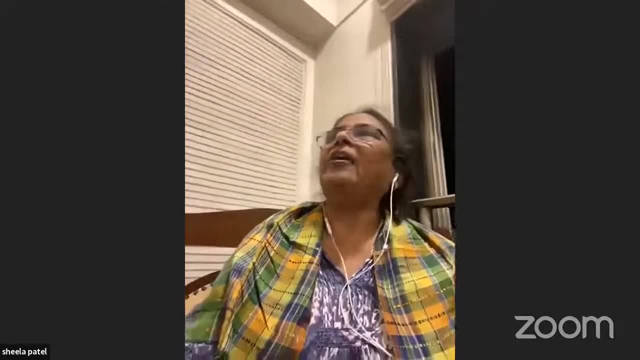 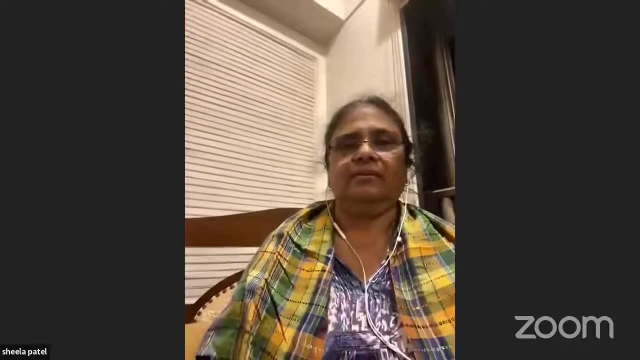 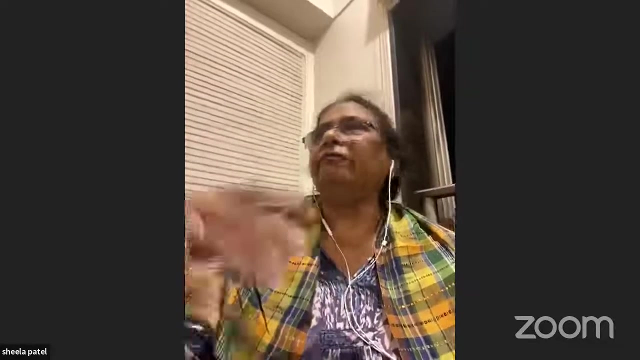 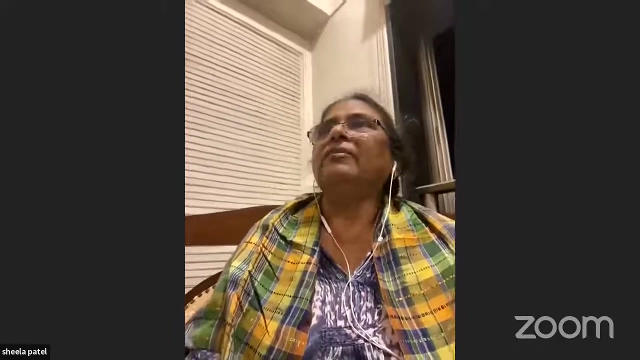 Everybody says that COVID has opened our eyes. It has removed the scabs of the old wounds. I don't think so. I think that this is just something. Which is like the floods and the famines and the droughts and all the terrible disasters that we face. We will shrug this off and go back to the same old normal. Because we are not ready to invest in equity in cities for the last 150 years. 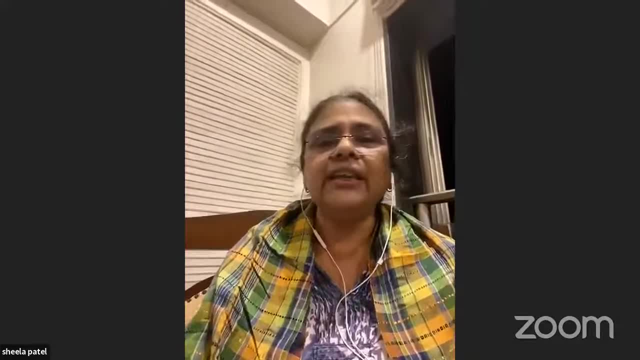 And so what kind of disruption do we need to change? You can't do that. You know, this urban thinkers campus. 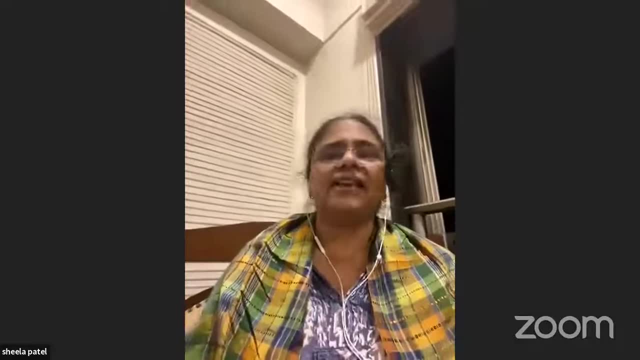 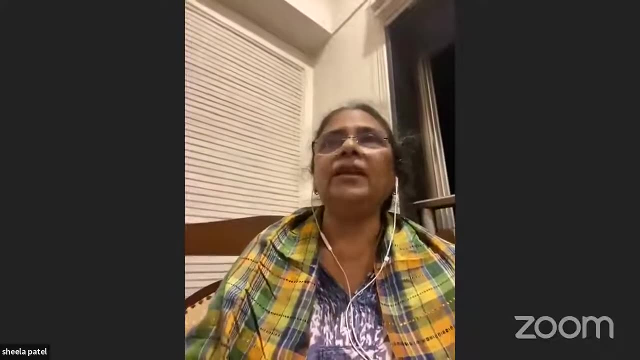 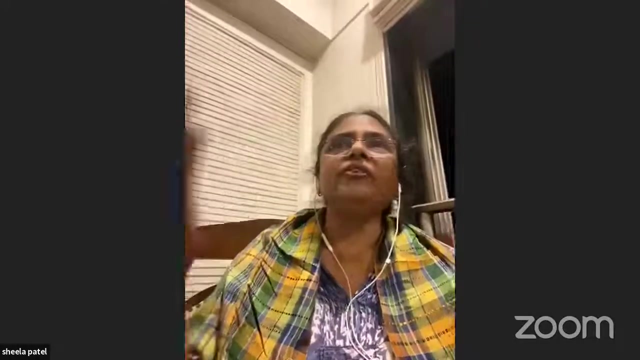 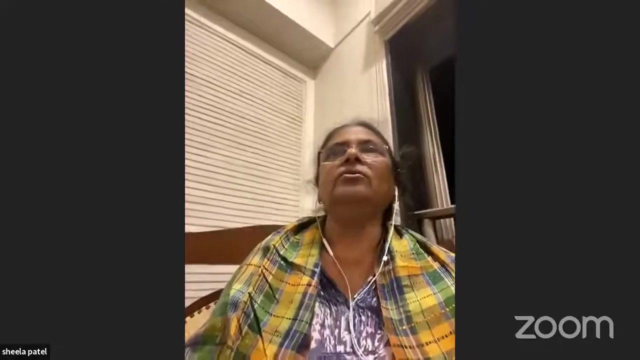 I don't know whether you have the courage to start this as a movement to say, start with acknowledging the reality of what is not being done. Our present and past secretaries at the center give prescriptions about local democracy. Yet they continue with the same regime with different names 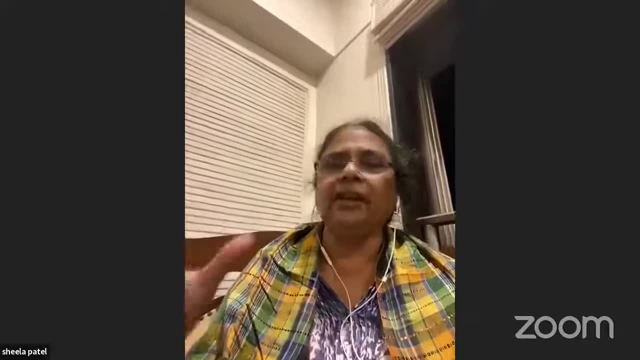 and feel proud that you have provided 15 lakh houses. What is that number in relationship to the requirement? Who has calculated what poor people pay as a poverty penalty when they build their houses incrementally, destroy time and again, where they pay five times more for water, where they can't shit properly in a dignified way, where during COVID, the WHO and the FAO and their local institutional arrangements 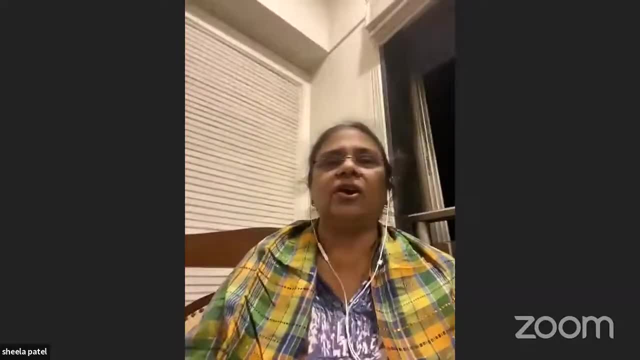 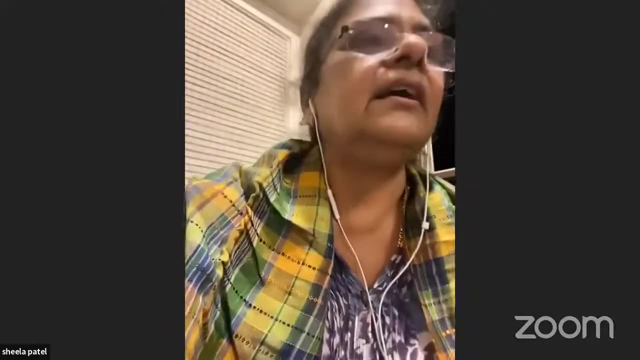 have not provided any SOPs on what happens in informal settlements. So the question for us is, 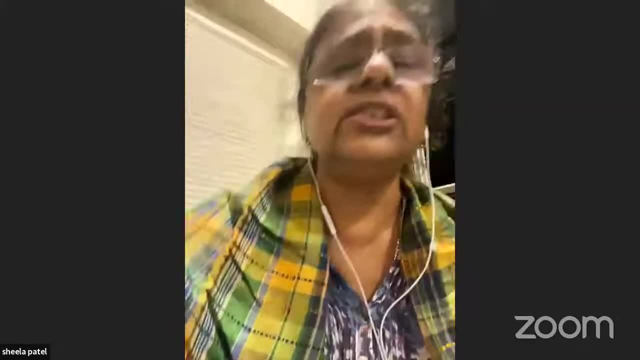 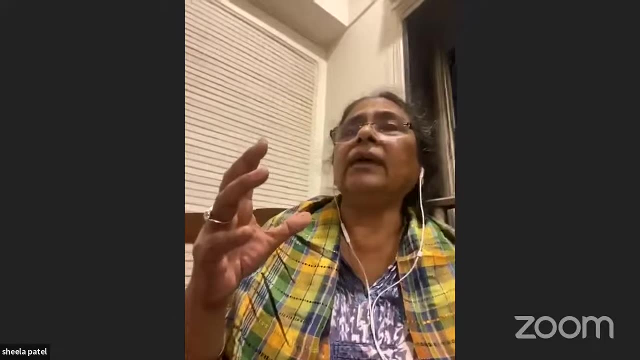 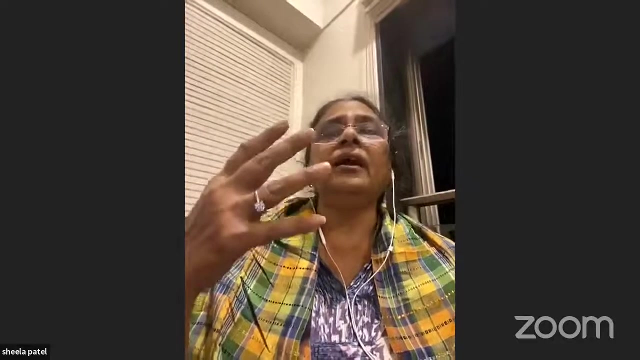 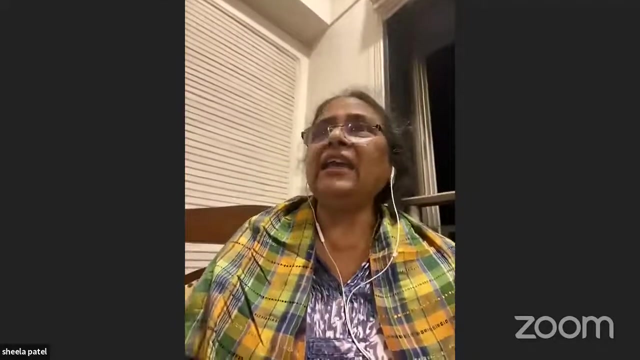 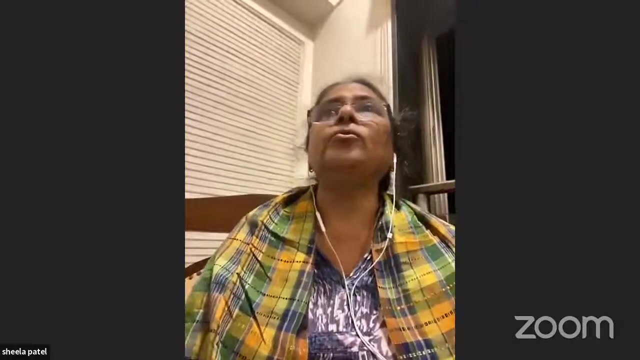 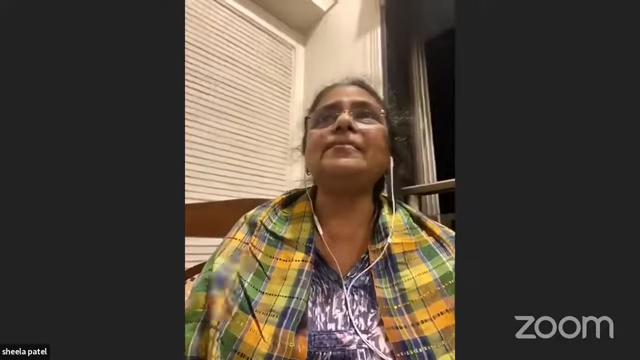 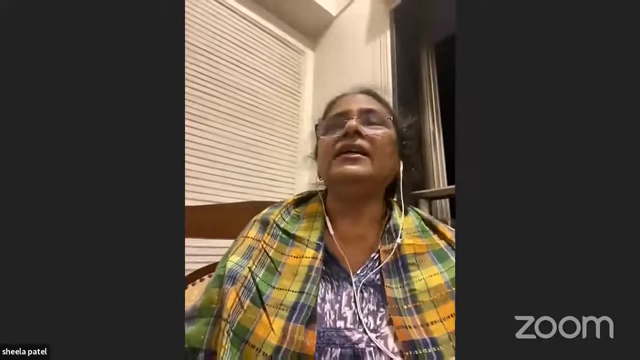 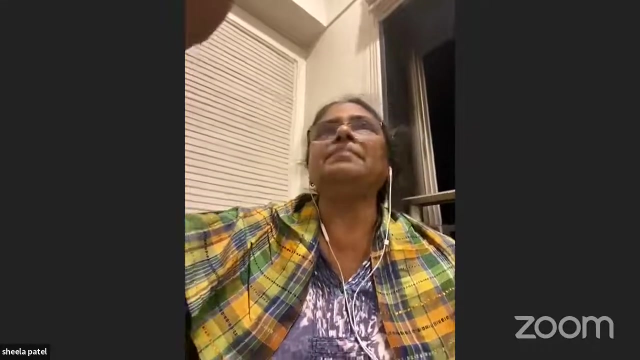 why? Why aren't educational institutions and planners and people who design cities either in the government or in the private sector or in universities take this problem by its neck and say, what changes in our educational system do we need to put? What are we going to put in place to transform the urban space so that the investments we make today transform cities tomorrow? You are all these prescriptions that people are giving cities don't just, it's not like, it's like taking, it's not like you can just turn around and say, now let's do like this mayor of Paris is saying, let's prepare a city that is a 15 minute city. Your life has to go around. It's become a big buzzword everywhere. 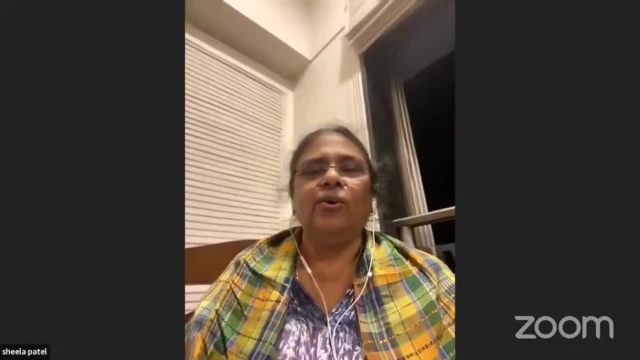 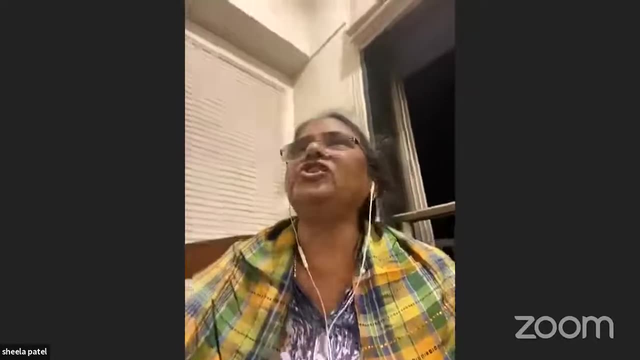 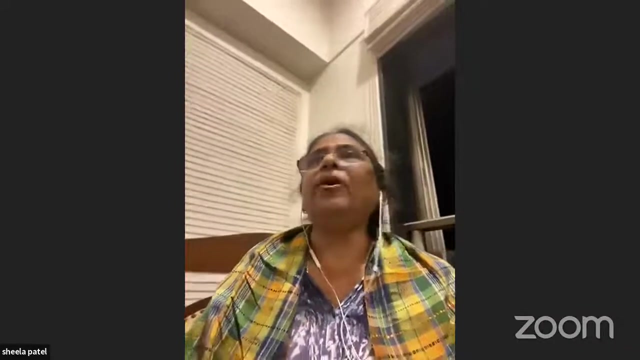 I was talking to the mathematician who is our advisor, who I'm going to talk with next week in another webinar, who's very excited with this concept. He's going to change, he and the mayor of Paris are going to change the city to become a 15 minute city. And my point is, instead of looking outward, we have to look at the situation we are in India. 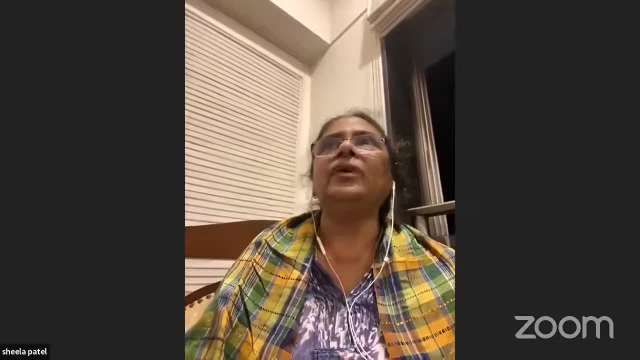 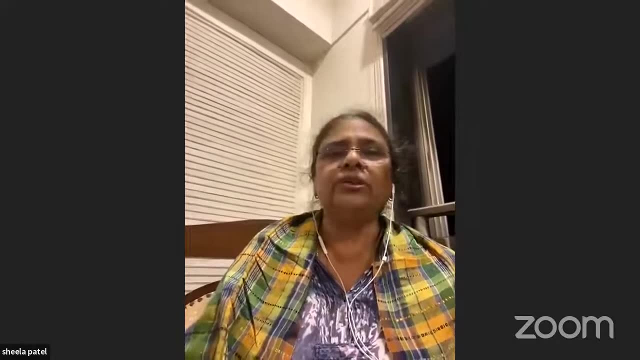 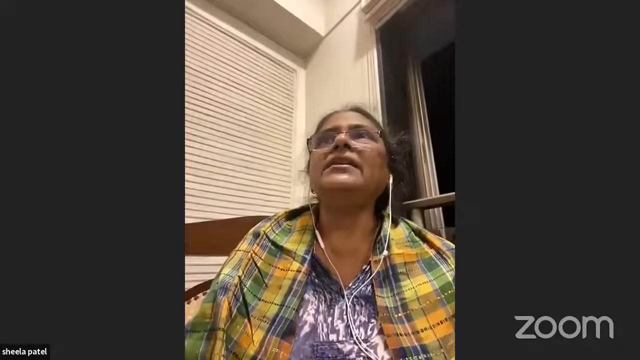 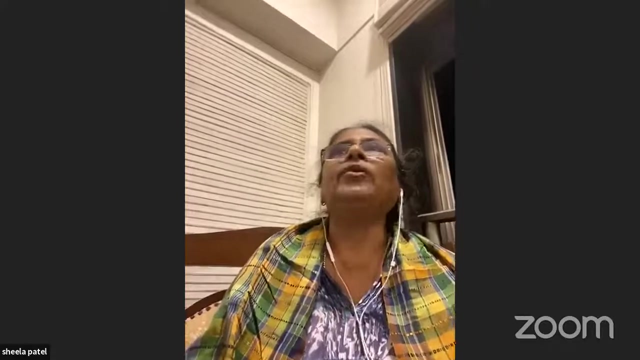 We are still a country that is going through a transition, where the mobility is determined by lack of opportunities and a complete lack and a denial of what is a good quality of life, which is urban and rural for those who are the bottom 40% of our city, of our country. We're not looking at that. 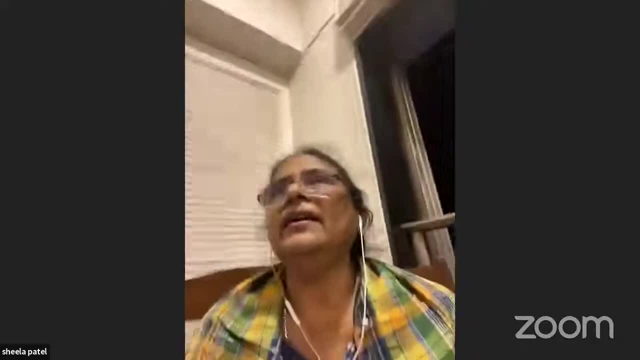 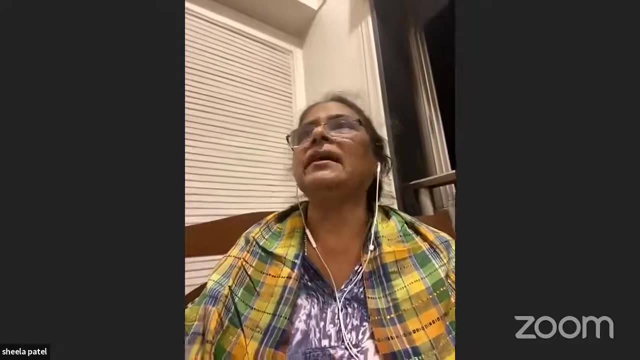 So I think we have to start off by saying, that the informal sector is not going to suddenly change by being given some formal label. 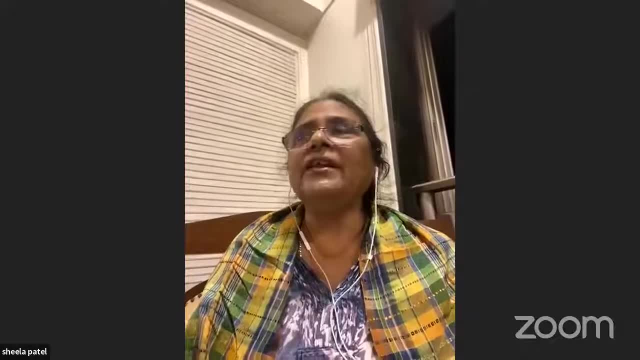 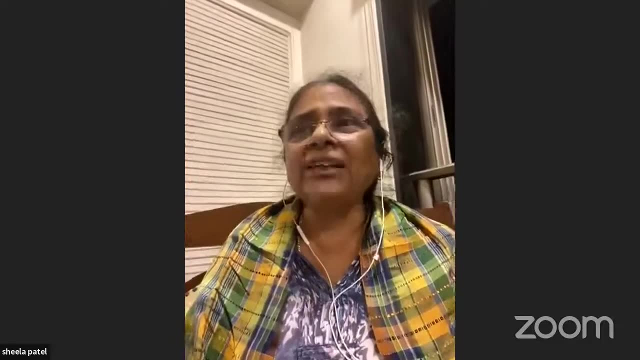 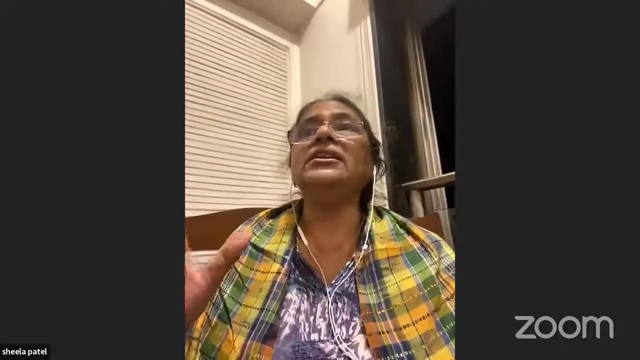 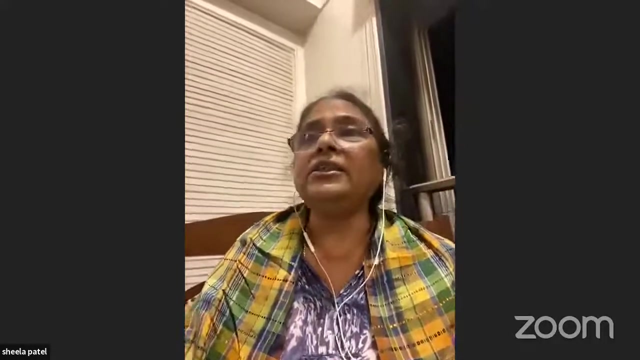 So what does your evidence building, what does your documentation of people's lives, what of the action research that you have the potential to take, can tell you the transformation that is possible with a combination of what poor people can do better for themselves, and what support and institutional backup that is needed to transform their lives. 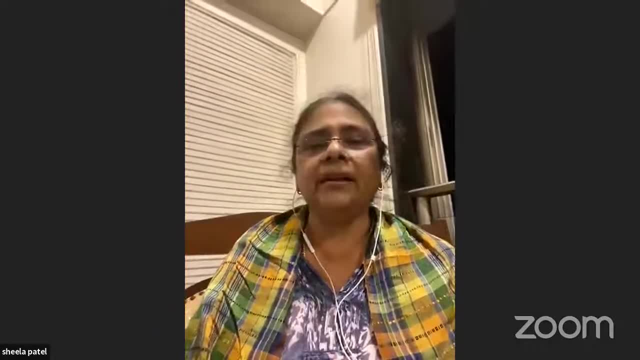 Their lives is going to grow incrementally better. It is not, there's too much volume and too little interest in this country 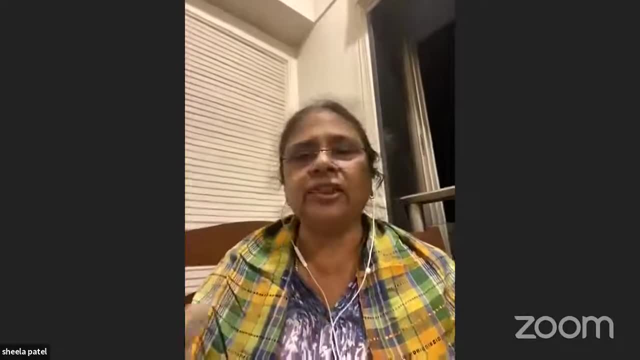 to do the kind of transformation that our secretary is talking about. 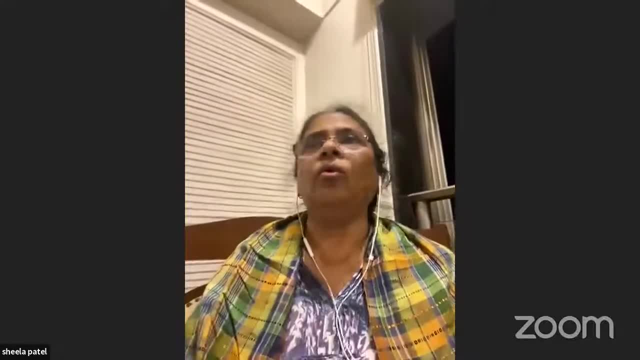 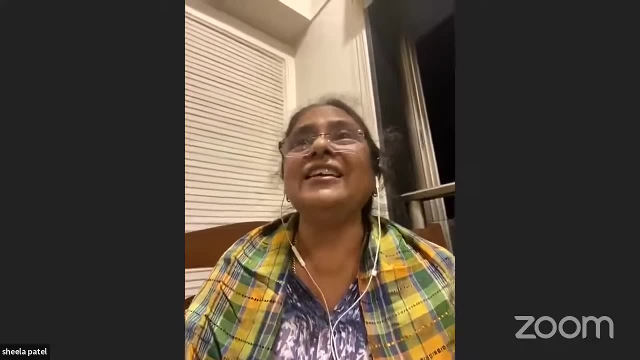 People are investing in their own homes. How are we going to improve that? How are we going to make their homes and their settlements resilient to the horrific climate challenges that we are now about to face? 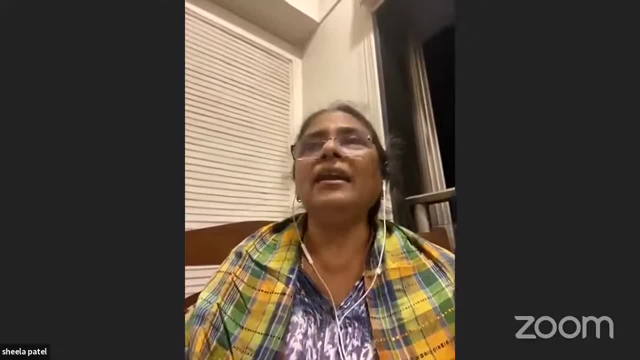 How are we going to change the manner in which we are going to deal with the fact that our country is going to be water stressed? 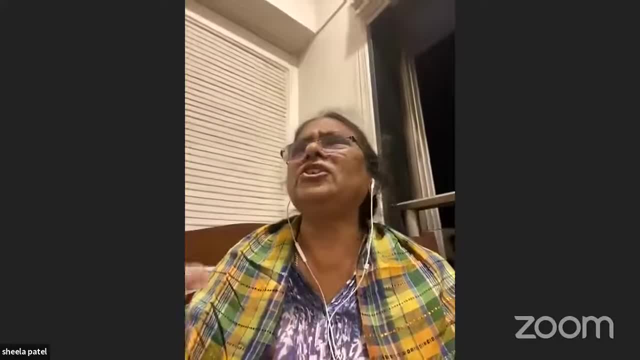 You know, we're so excited about digital technology and artificial intelligence. 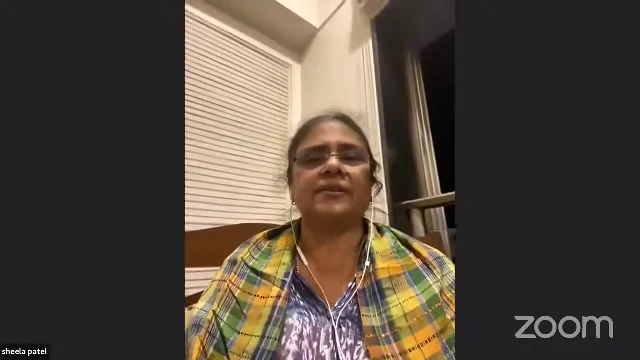 How is all this going to improve people's lives? More importantly, 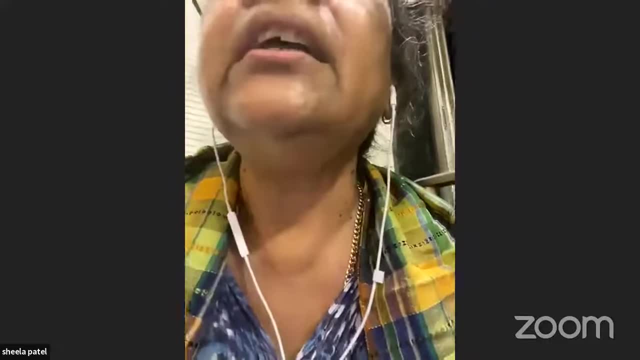 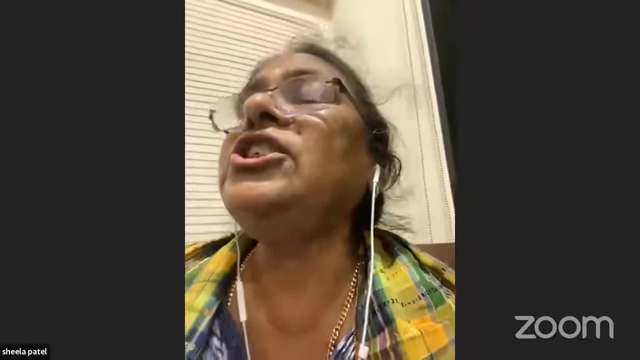 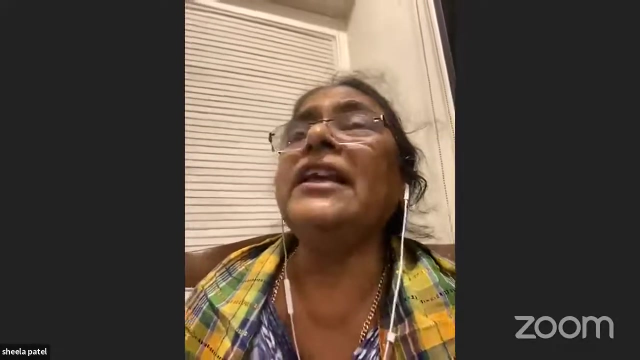 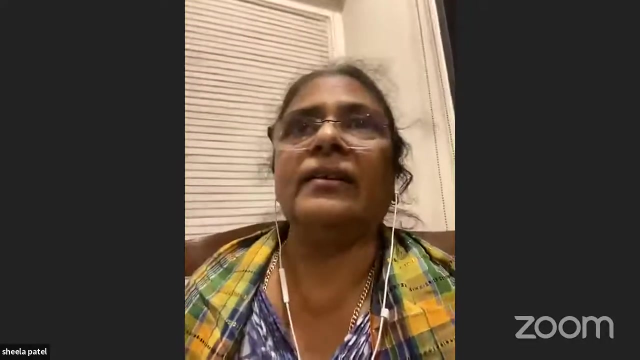 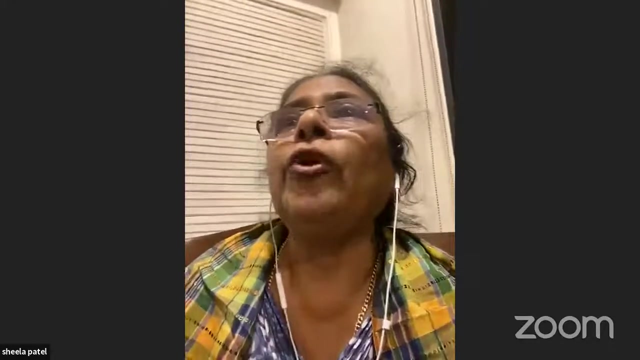 we are not looking at the challenges that we are going to face by ignoring women and children in cities. There is no gendered exploration about anything. There is no acknowledgement, even in this COVID period, of what is happening to women and children. We just skate over it. We hear these one and two and three city institutions say, we need to have one and two and three city incidences of collaborative practices to make change happen. 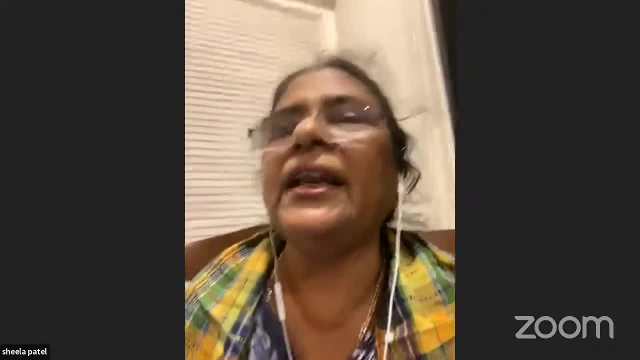 What's happening in the 5,000 cities, including the city I live in? My city, my state, everybody's at odds with each other. 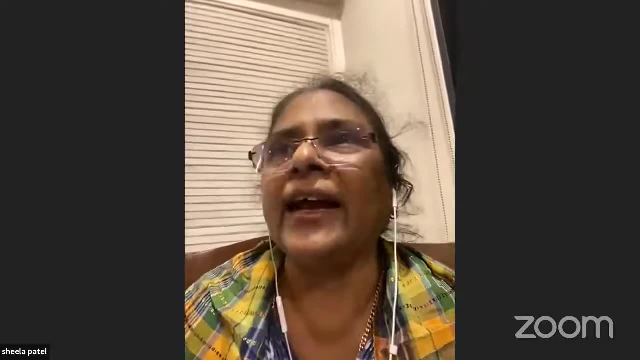 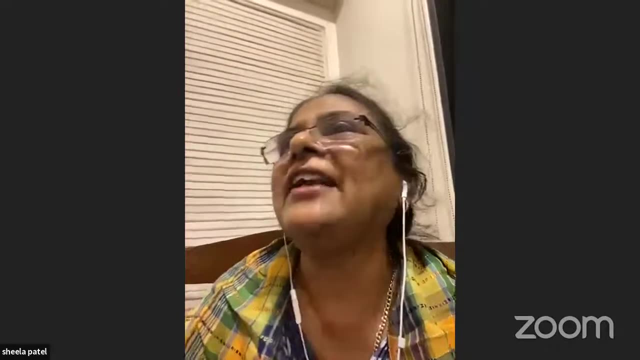 You take a newspaper, you have one page saying things are getting better, you get the next page saying it's getting worse. You have international organizations that are giving you different scientific theories. 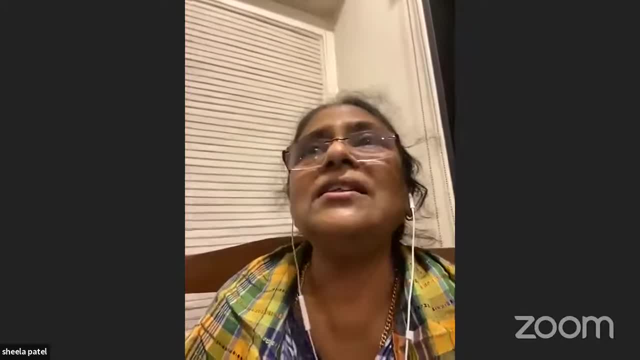 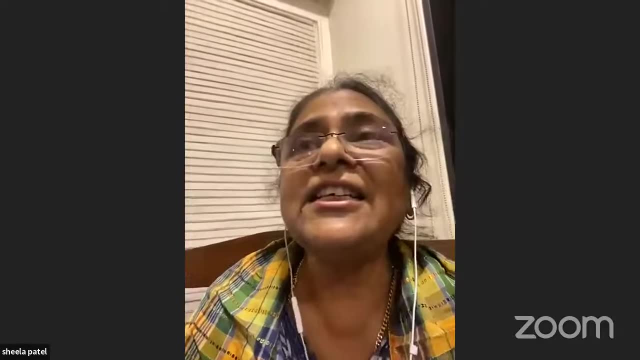 So in the midst of all this, what is the role of all of us who take a responsibility to address cities 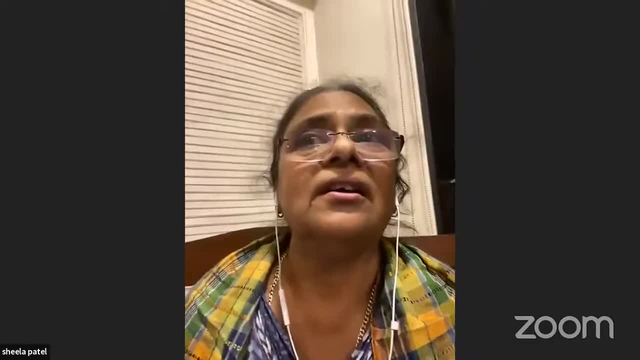 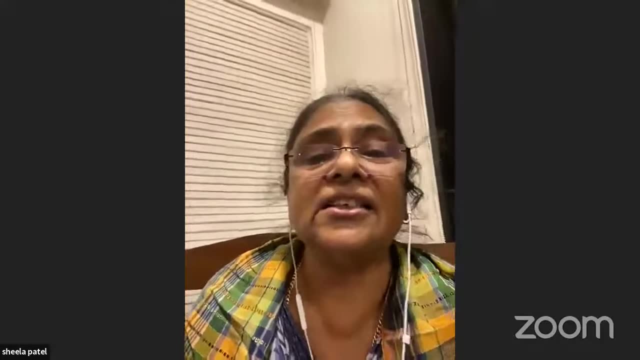 that are going to be resilient in the future, not only to accommodate equity, but to accommodate the increasing disasters that we are facing? 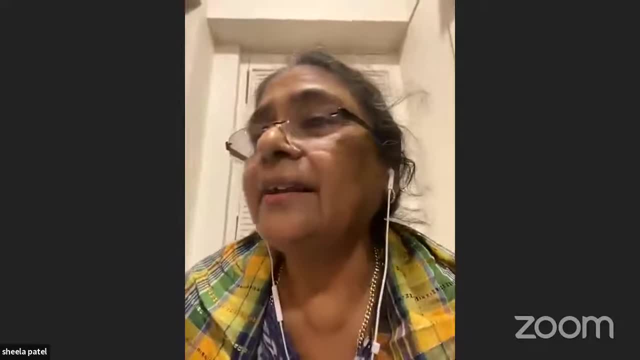 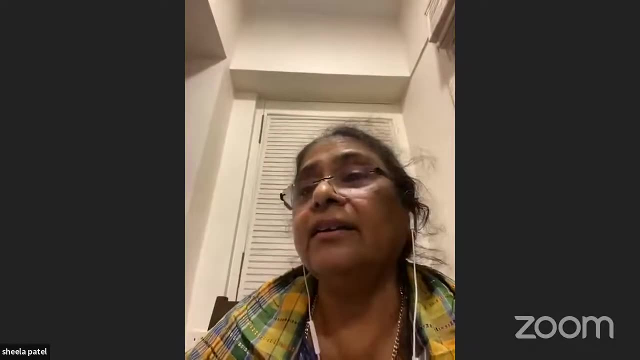 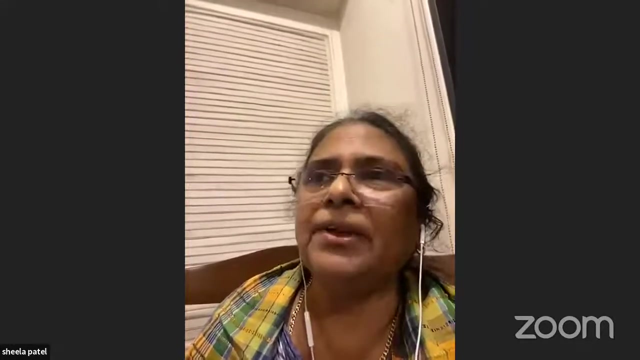 So I want to say that the real challenge that I think that I would ask every urban thinking campus to do is to start by seriously creating a partnership between the local municipality, the network of poor people, 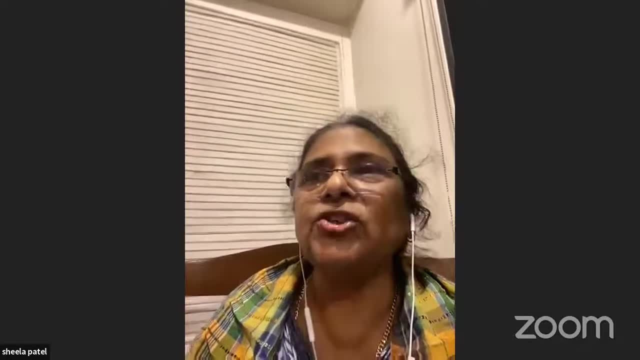 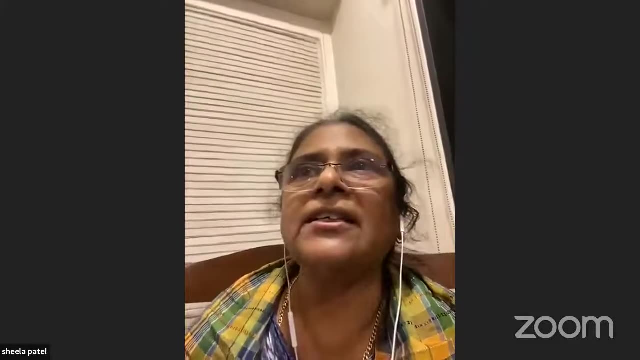 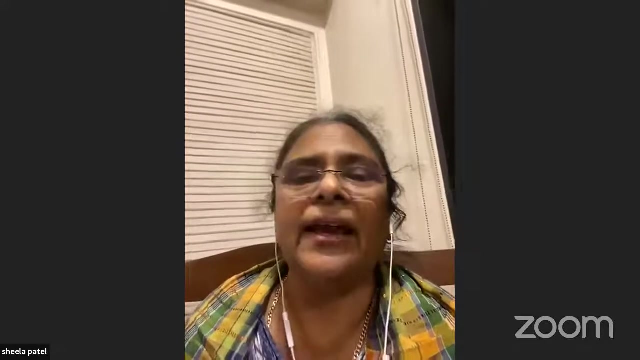 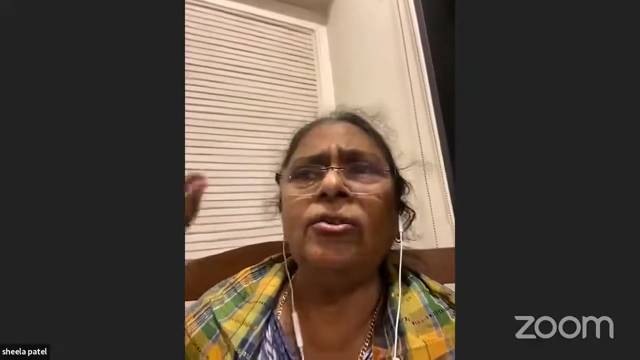 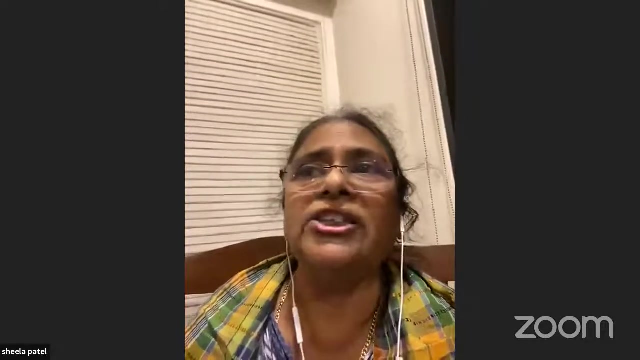 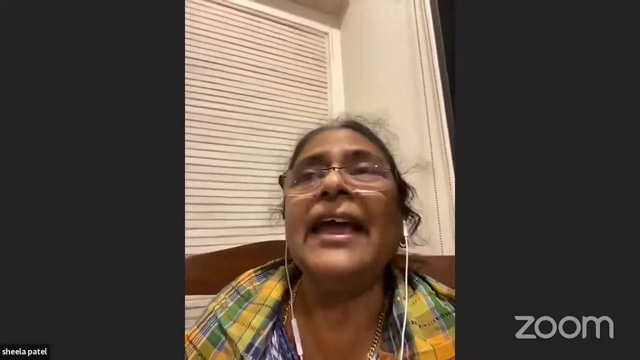 and the academia in that city. Elite institutions, SEPT being one, planning schools that are run by government, elite private universities, are not going to be the ones that are going to change local dynamics. You all, as elite institutions, have to invest in every university, every municipality, in every type of town, and create local knowledge that works for local planning, local design, local challenges, and then aggregate that upward to look at what policy will facilitate that. 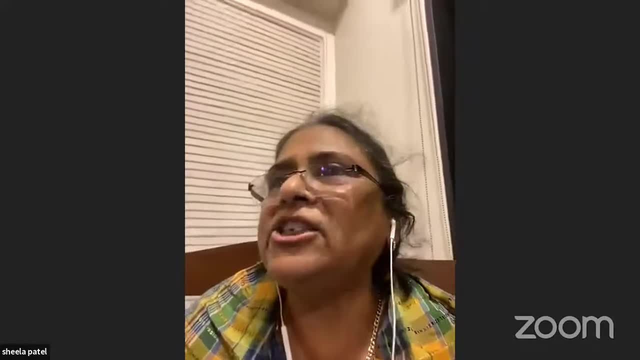 Just now, whether it's Niti Aayog or it's the ministries, the ministries don't talk to each other. 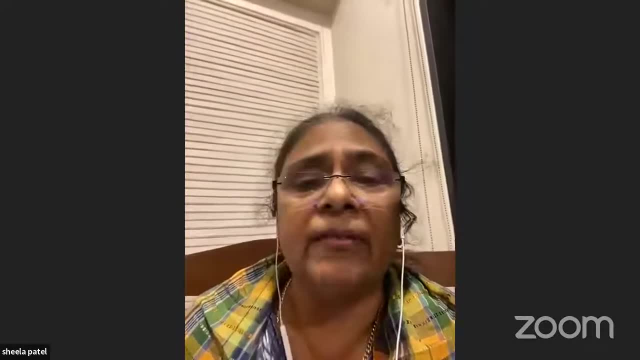 The food supply ministry doesn't talk to the urban development ministry. The water supply people don't talk to the electricity people. 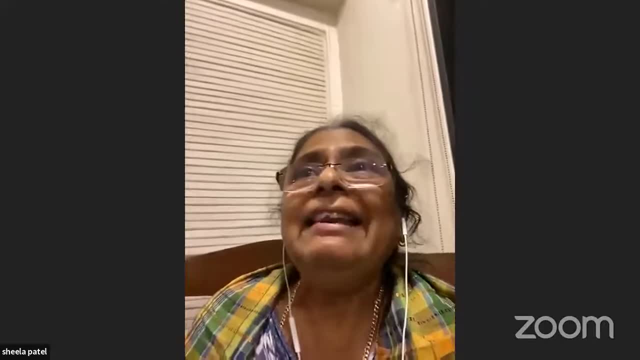 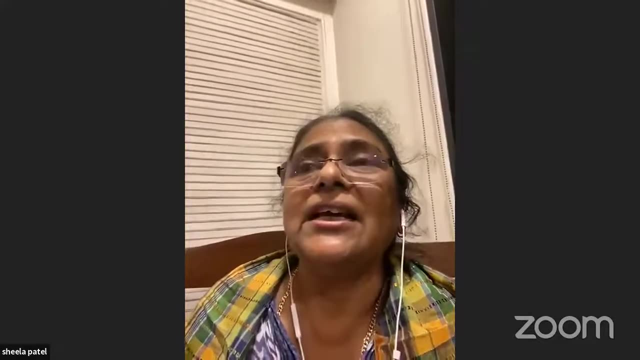 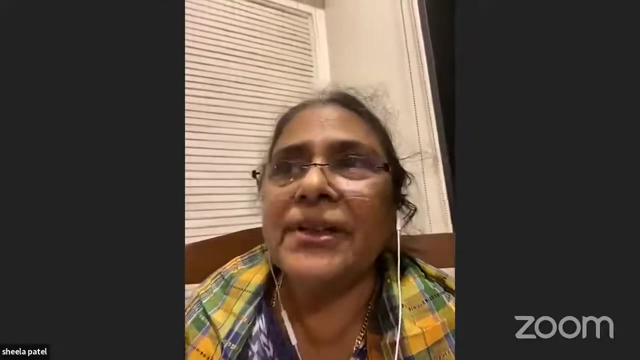 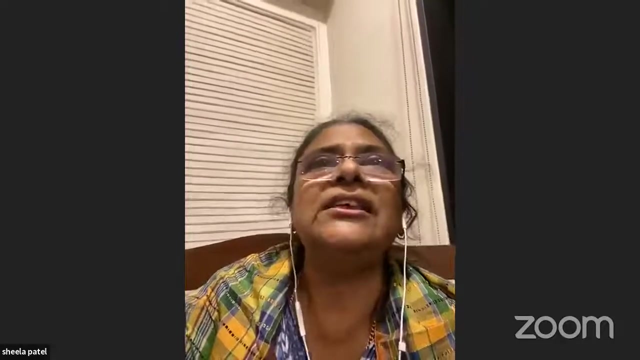 So my point is that let the granular local reality produce local solutions that then those of us who are operating in multiple cities, in multiple states, that bring the aggregated insights to produce a national policy that overarchingly supports that. 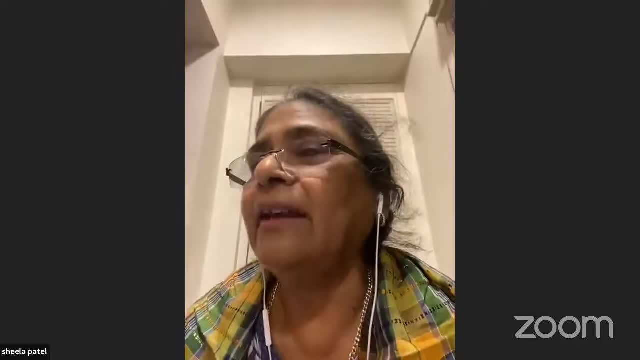 So I want to stop here and basically say that we are all on the wrong path. 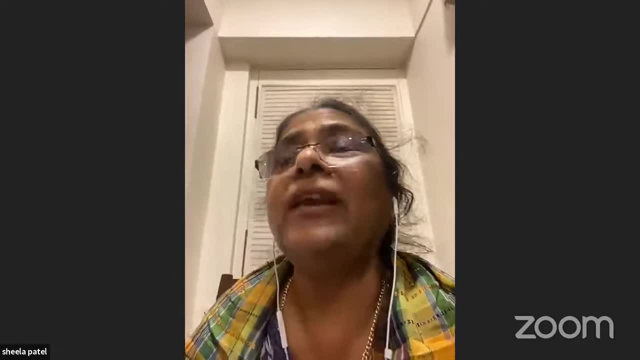 If we don't have the courage to change, you will have this conversation. And if you invite somebody like me, 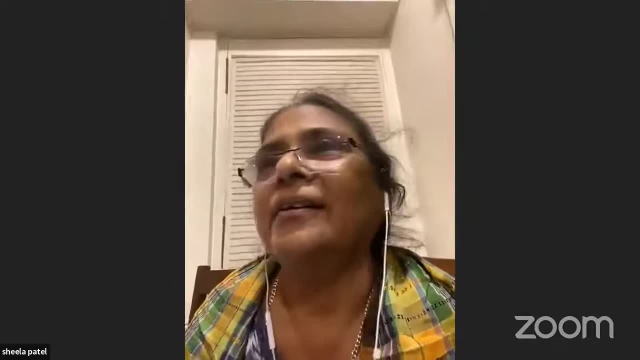 you will have me singing my same song because I'm doing this for the last 40 years. 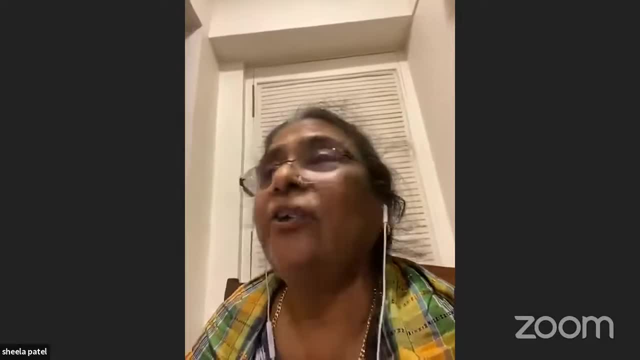 And I see no change. I don't see anything except the amazing resilience of people who are living in survival mode. 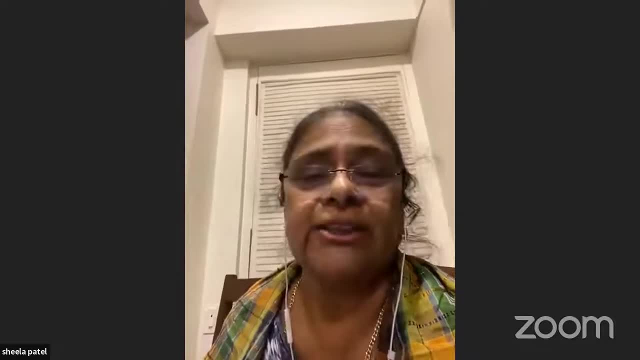 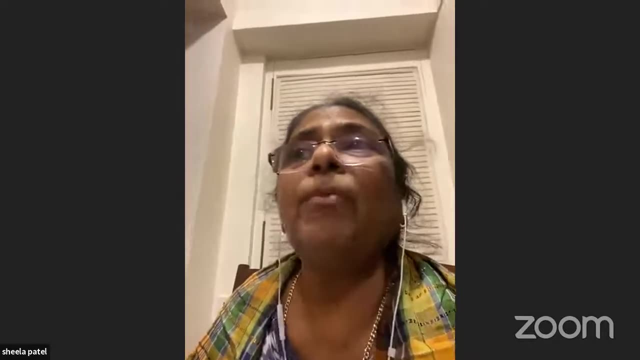 That's not the way we should bring up the next generation. So all of you who are in educational institutions, you have a deep obligation to make that change. 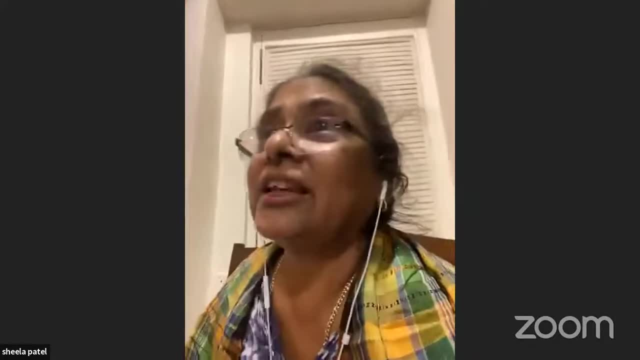 And so should you, Hitesh. NIUA also has to change. So thank you very much. 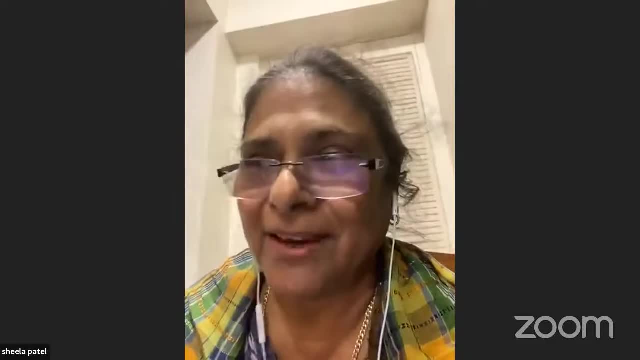 I hope those of you who stayed back will agree with me. Thank you. Thank you, Sheila-Ma'am. 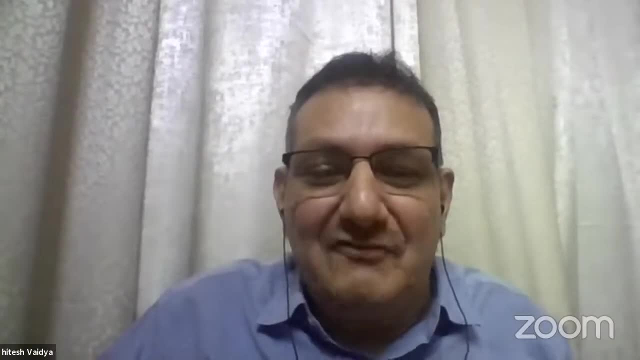 And I think, you know, as when I said that we need not daring cities, we need daring leadership. 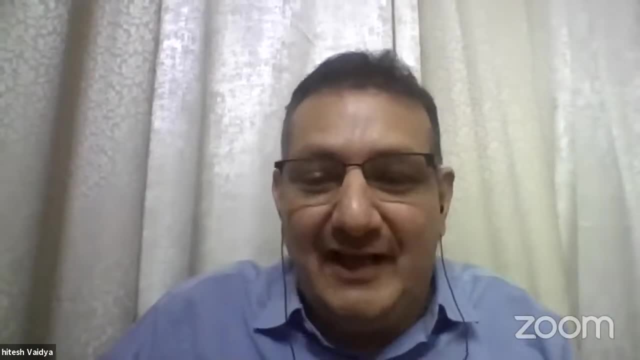 I think you are the right example for daring leadership. And, you know, you can't be so pessimistic. 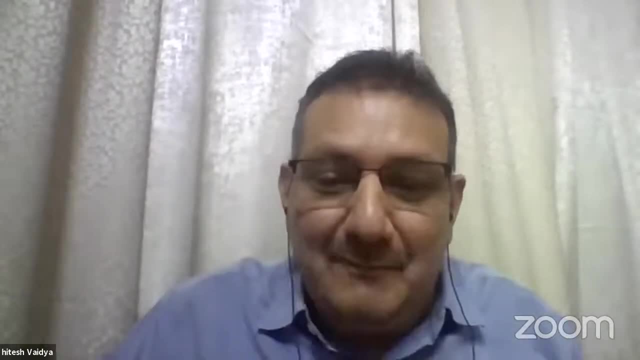 And I must say that. You have students who are trying to take, you know, bull by a horn 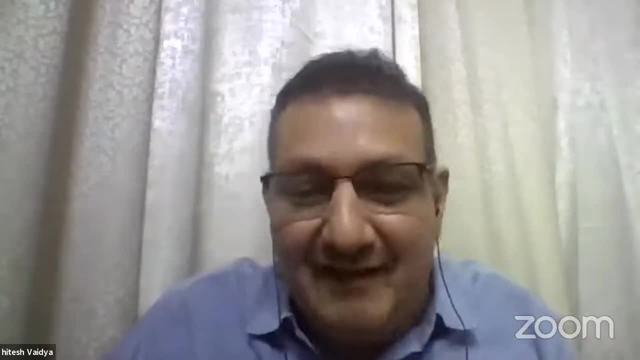 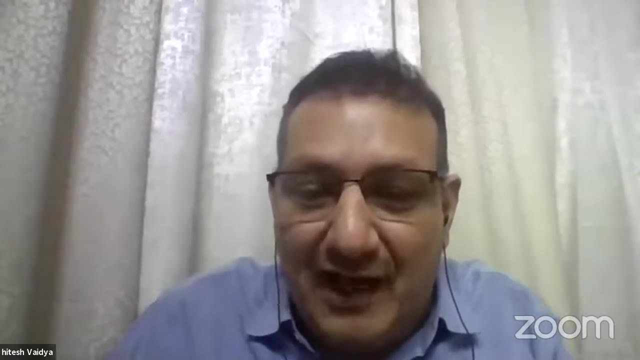 and trying to make a little change. I'm not saying that we have done. But we are trying to take that step forward and take that legacy which you have really created for the last 40 years to a next step. 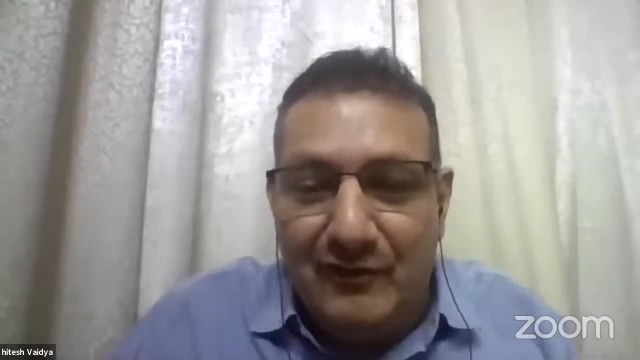 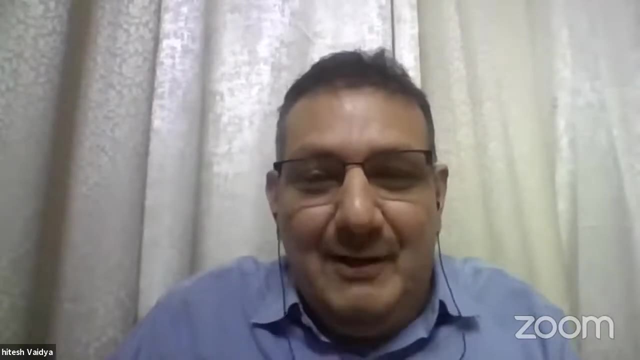 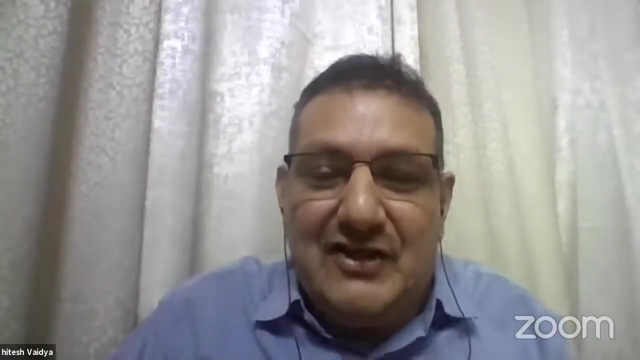 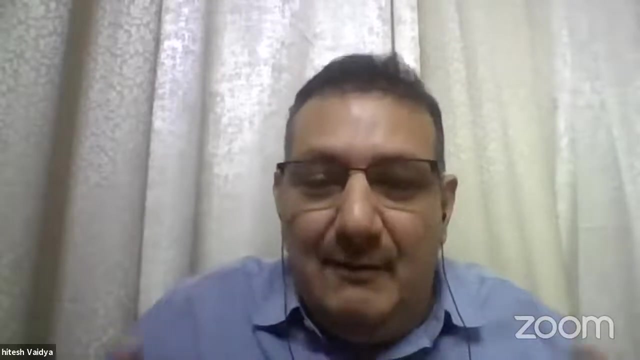 As you all know, that change is slow. We are also moving. Maybe something, as I said, we can pass on to our next generation. And they have to take it forward because this new generation, which I see as so many students here, is the aspirational generation. This generation is looking forward for new solutions. And I think they will make if we leave behind the great thought process. 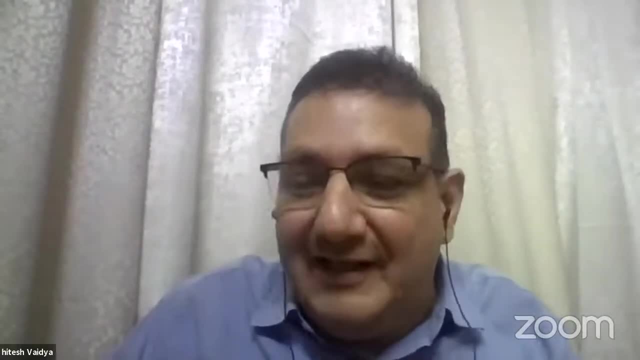 So I think you have really talked about whole radical transformation. And I think that's what we need. 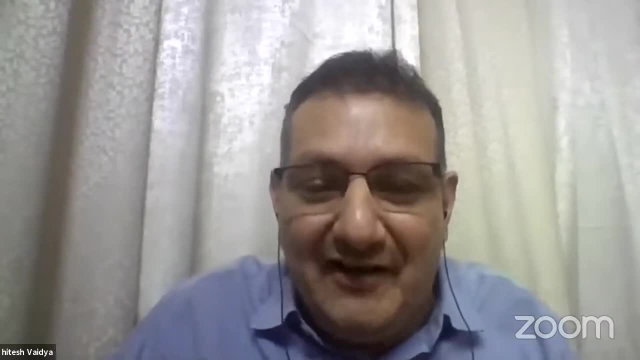 We need to shake it much faster and much harder than what we are doing right now. 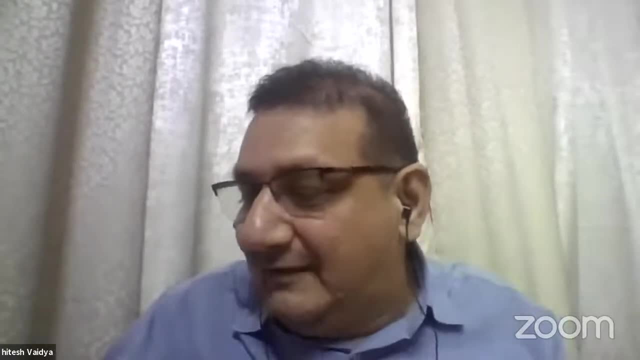 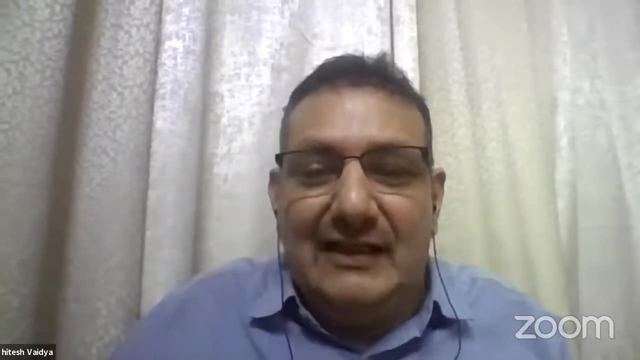 But I think two points before I go to the next speaker. I think very nicely you put it. Where are the planners? And what planners we are looking for? You know, I think that's what type of planners we are building. 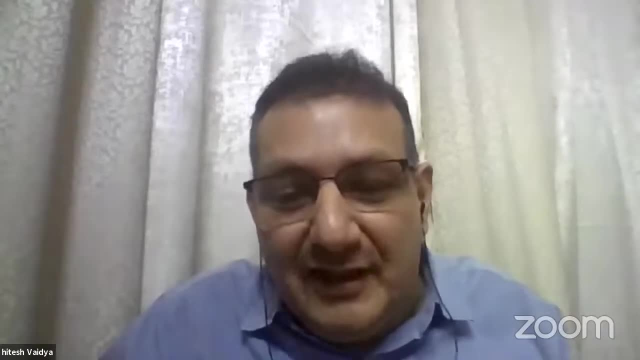 And I am one of the planners which have been built, which have not turned into a planner, but become a glorified. And I will not say that, you know. 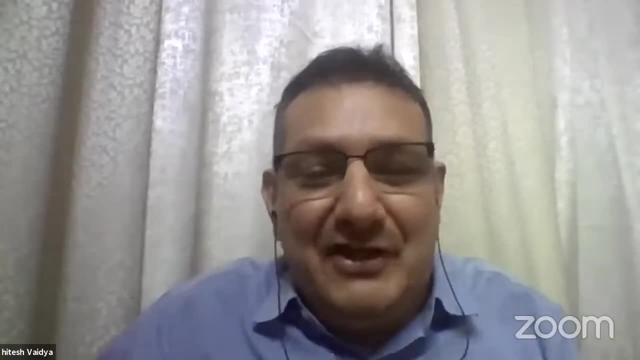 So we need to change. And I think this aspirational young youth will make that change. A change to happen. 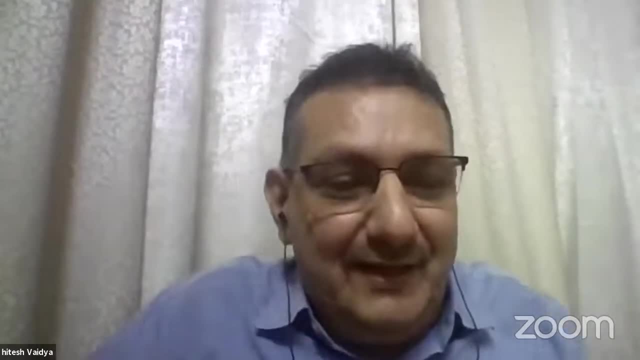 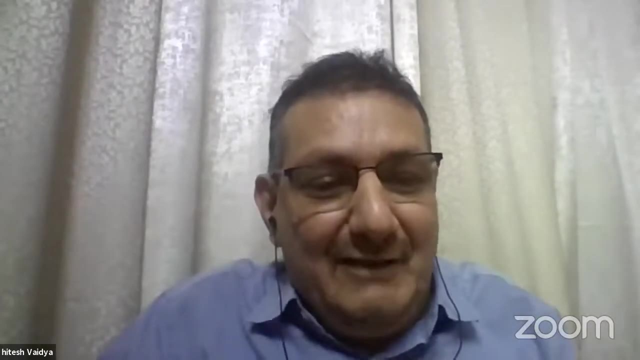 So now I will request the next speaker, Mr. Massimo Miracoli, who has been waiting for quite some time, listening to the Indian side of story. 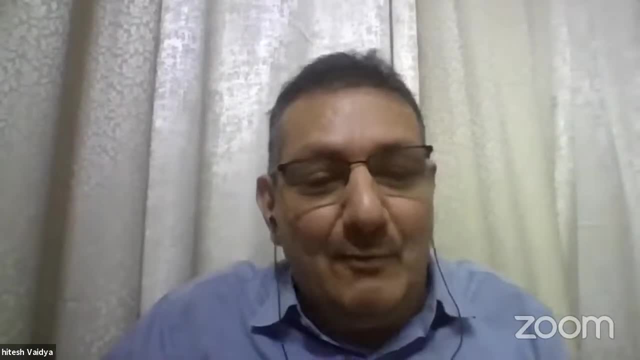 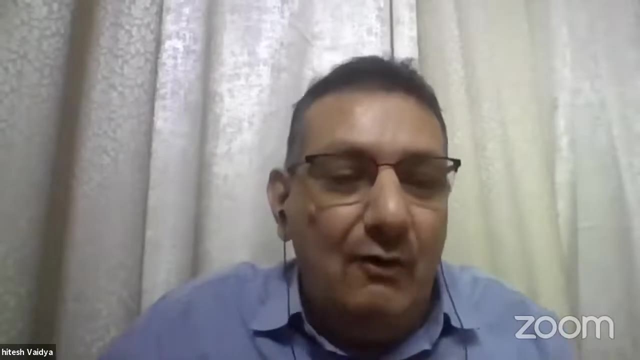 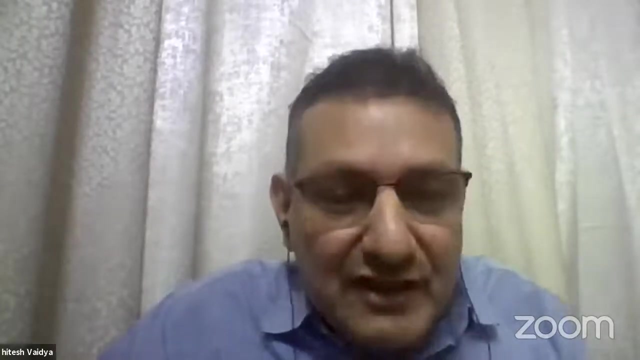 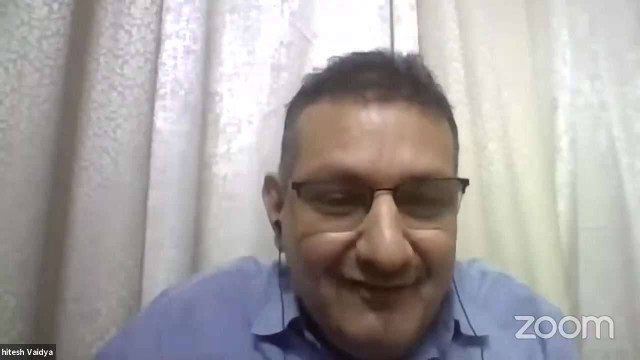 And he brings a lot of global practice from Milano, how they are looking at urban policy framework, pedagogy and practices, and how both of us, we can learn from them, and, you know, showcase some of the work which we are doing, which others can learn. Because, you know, even though we are becoming very harsh on ourselves, which I don't think we should be, because, you know, over the last 40 years, and I, one place where I not agree with Shilaji also, 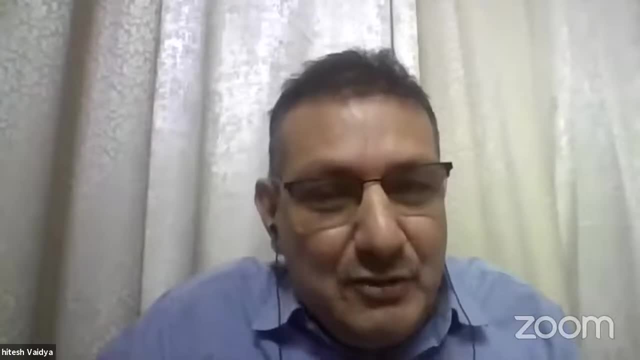 that, you know, last 40 years, India has also graduated. India has also learned. 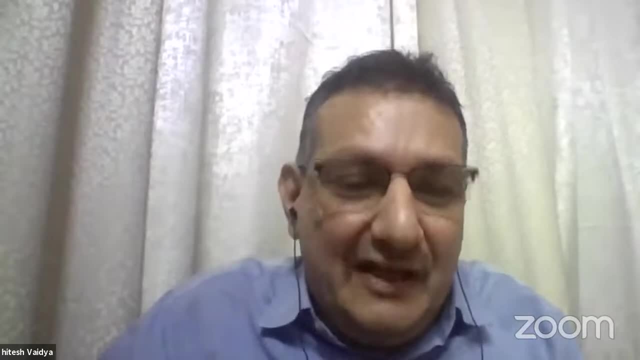 India has also moved. Because of our complexity and our scalability, 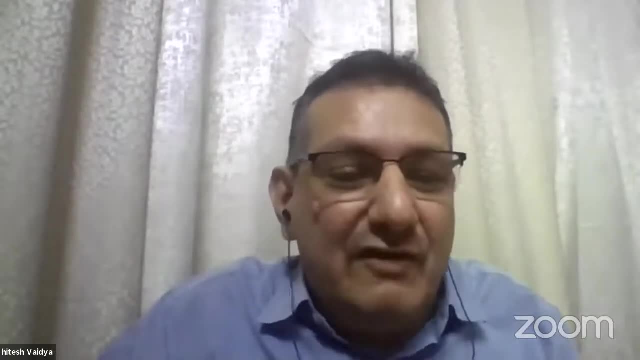 is a challenge within us. And that's why we may not have a right solution, and the right thing, but we are also moving forward. 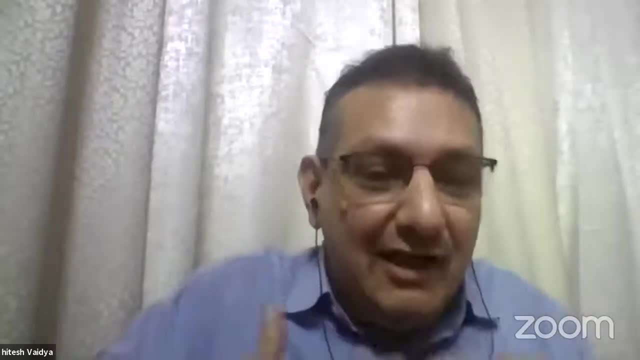 So, you know, we would be happy to contribute, not only learn from us, but also with our experiences, our lessons, we can also contribute to the global discourse. So, with that, let's not be too harsh on ourselves. 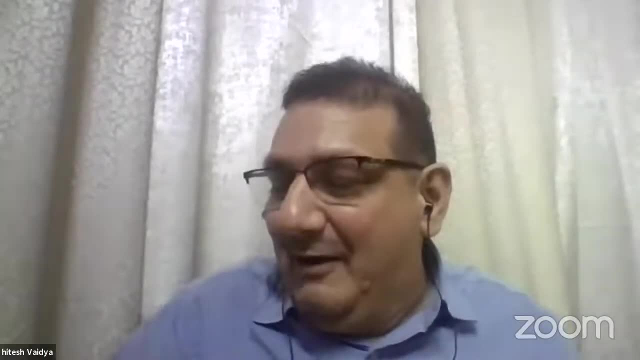 I request Ravi to introduce Massimo to the audience. Ravi, over to you. Yeah, thank you. 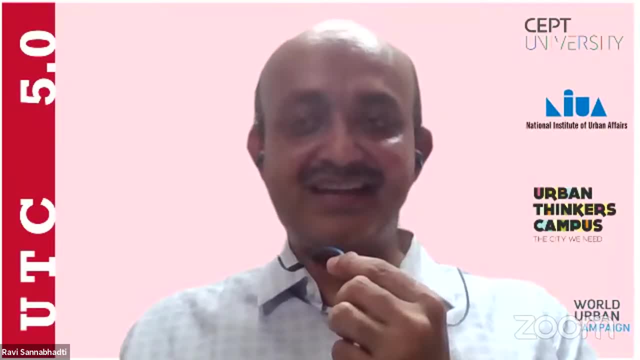 I would say, I would like to, before I introduce Professor Massimo, I would like to thank him for his immense patience. 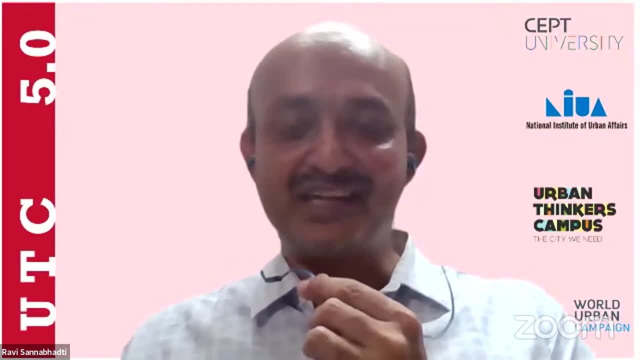 We had scheduled this quite differently, but thank you for waiting, sir. So, 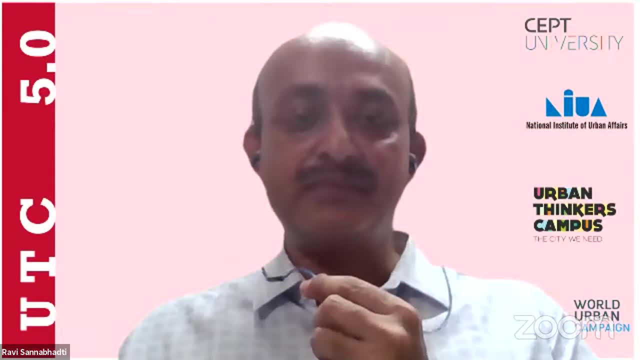 Professor Massimo Precoli is a full-time professor at Politecnico di Milano, Italy. 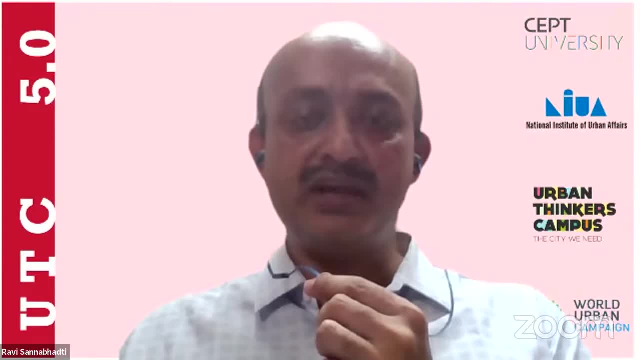 After an MSc in Architecture and a PhD in Urban and Regional Planning from IUAB Venice, Professor Precoli has been for 10 years a tenure track Assistant Professor in Urban Policies at the Department of Architecture and Urban Studies at Politecnico di Milano and faculty at the School of Architecture and Society. He lectures on housing and neighborhoods and urban ethnography. 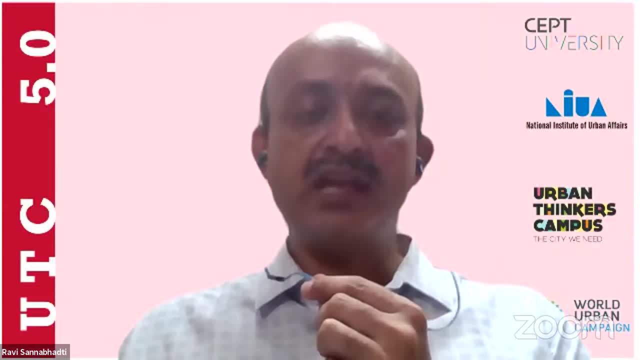 In 2009, and 10, he was Alexander von Humboldt Research Fellow 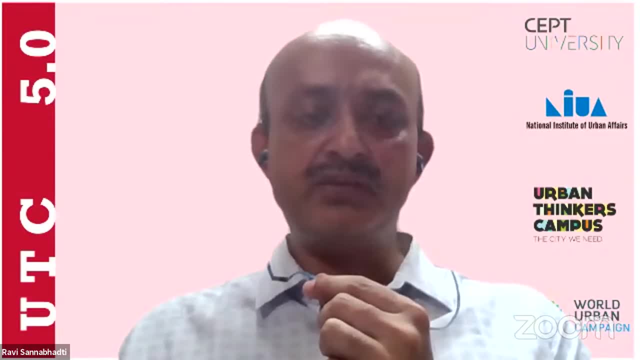 at Humboldt University, Berlin, and Heaven City University, Hamburg. 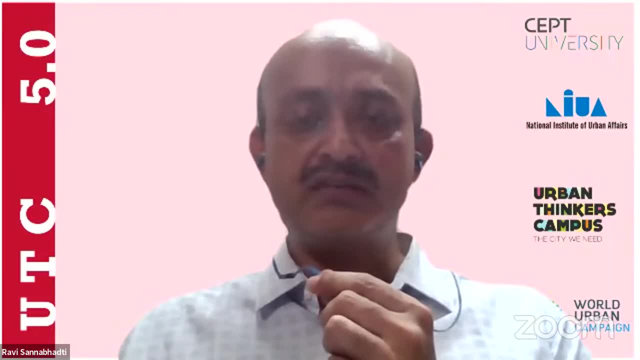 In 2014, he was awarded a Velux Visiting Professorship at the Center for Urbanism at the Royal Danish Academy of Fine Arts. 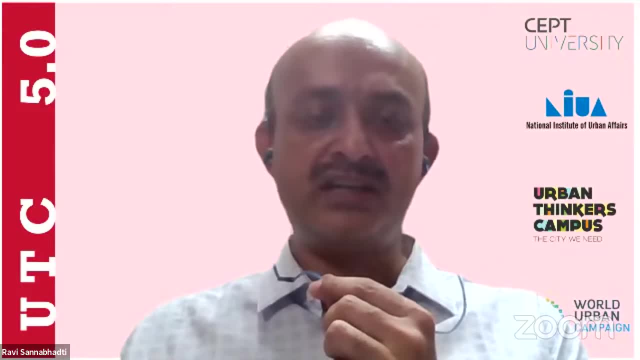 In March 2015, he was appointed as full professor at the University of Luxembourg. His research interests focus on urban regeneration processes, urban and housing policies in the context of post-industrial cities, social change patterns at the urban level and restructuring of local welfare policies, emerging forms of urbanity, dwelling and inequalities. 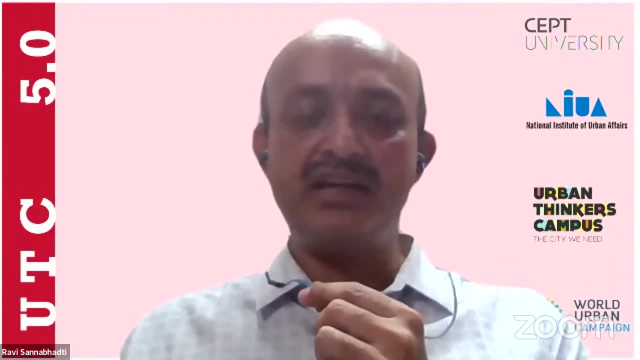 On these themes, he has been developing several international research projects, consulting. 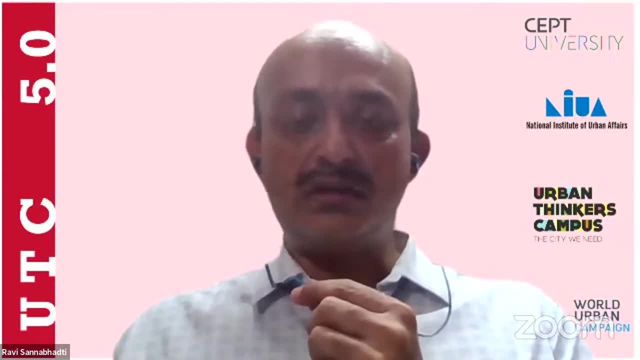 He also is interested in consulting with local governments and publishing books and essays. 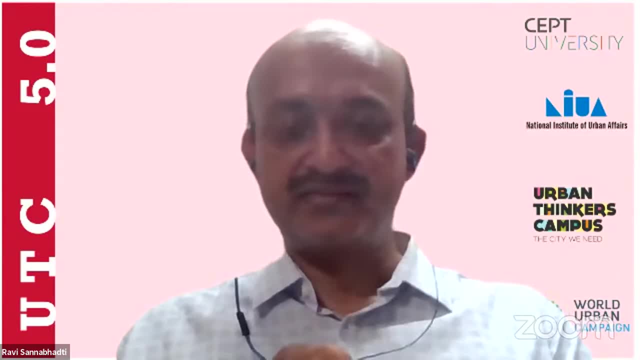 I would welcome you, sir, to address this gathering. Thank you very much. Thank you very much for the invitation. 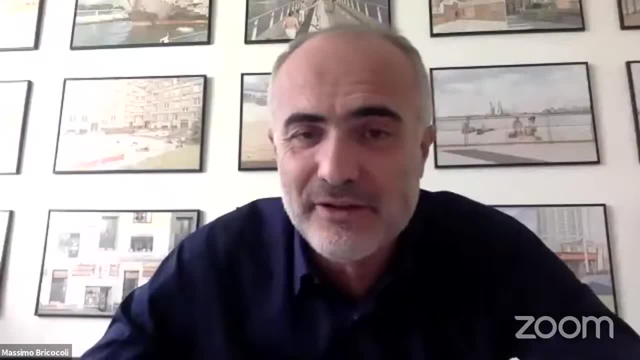 The first comment I would like to do is also, it's really very interesting to follow all the colleagues. 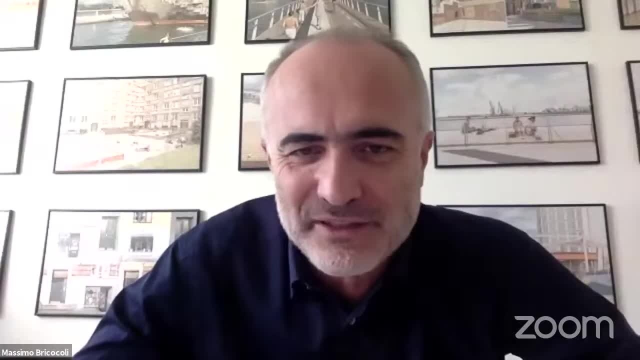 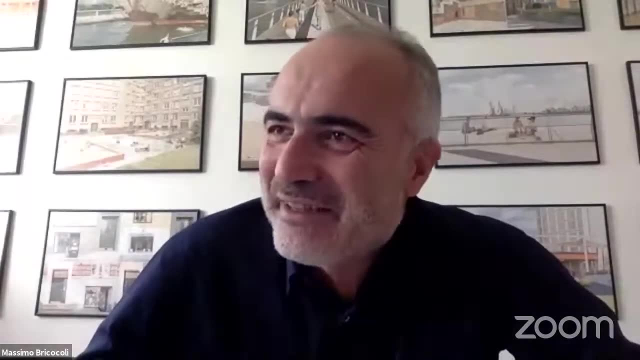 And I was thinking that I think I dare and I'm critical in my context, but Sheila Patel definitely is much more. So I am sticking after her. I think she was quite provocative and I think we all need to have frank discussions. So this was really interesting. 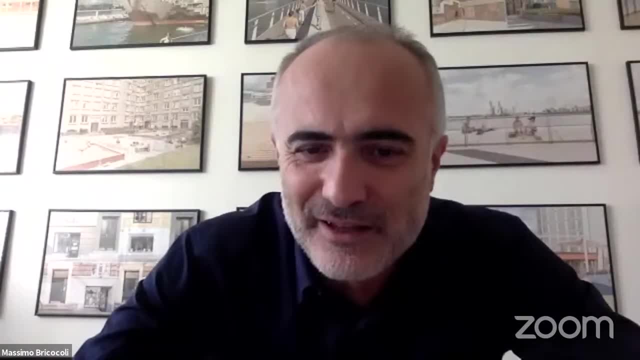 I prepare the presentation. I thought it's also good for you to just to get some images of. 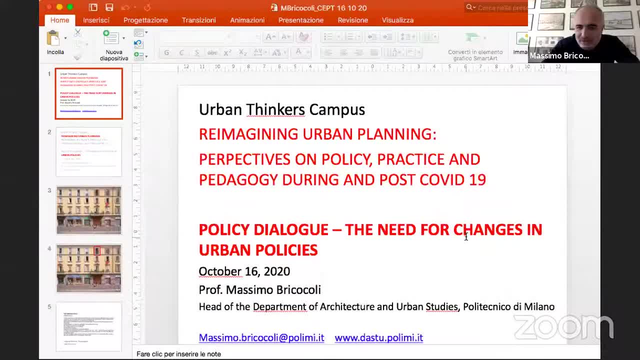 And I hope let me know if it's working. 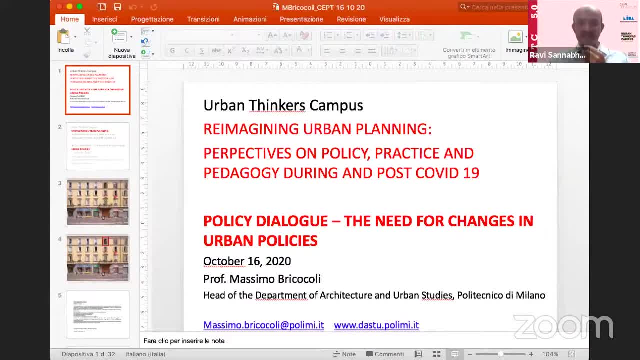 It's working. It's working. Okay. Yeah. If you can just turn it full screen. Yeah. Thank you. Okay. 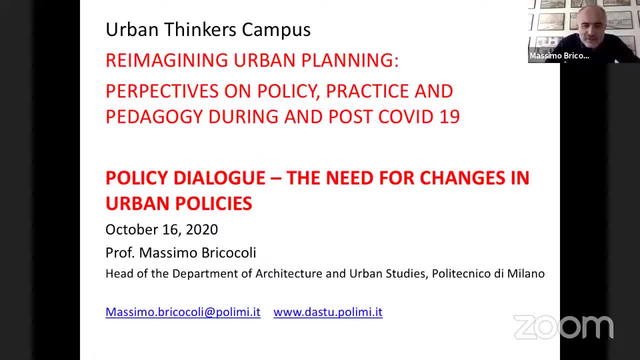 So I thought that the, I really took seriously the title of your program 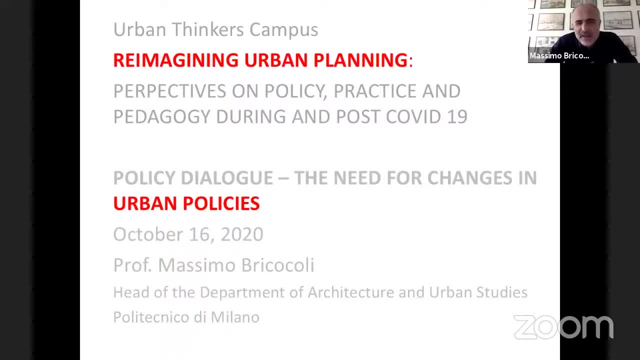 because it's re-imagining urban planning. And then we are discussing about urban policies. So it's a bit like an opposition that I'm creating, a bit stereotypical, but you gave me the chance to think how in this period, in this year, starting from March in Italy, the COVID pandemic really put me in a position where I can say, well, you know, urban planning is very important. 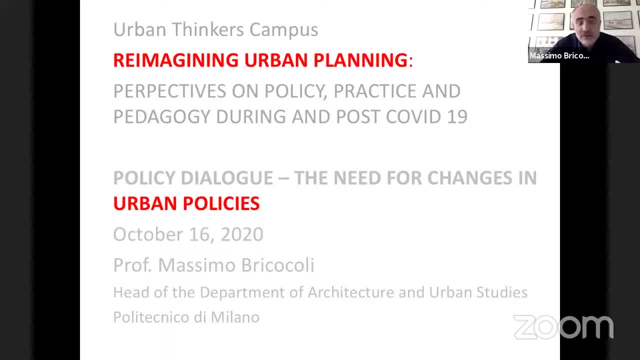 It puts into tension, attitudes in urban planning, which just to sum it up, I think still in Europe and in Italy, urban planning is very much based on a vision of a growing city. While now we are really facing the issue of a transforming city, a city, which is already existing and where planning should really deal with very different issues and not just with the growth. So, thank you very much. 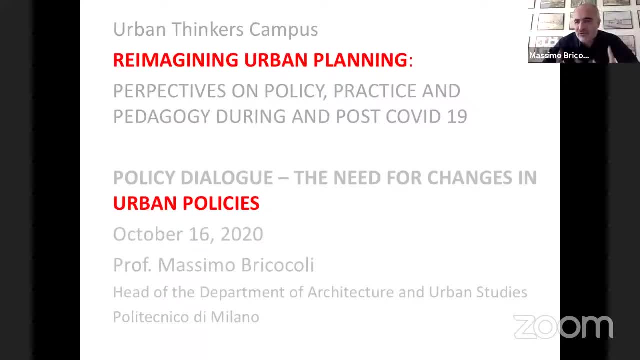 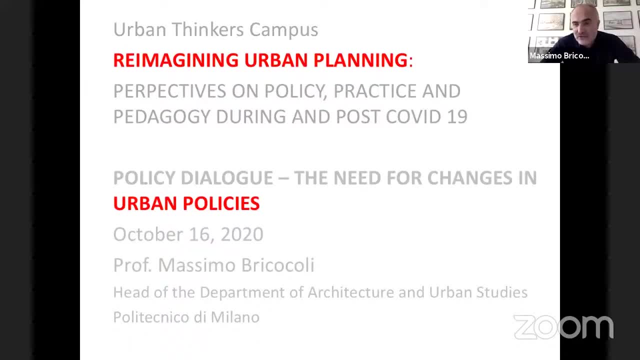 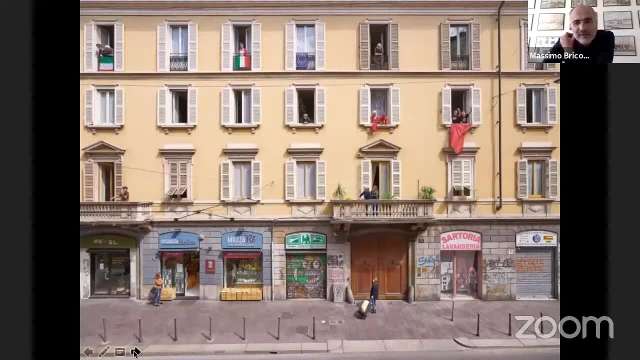 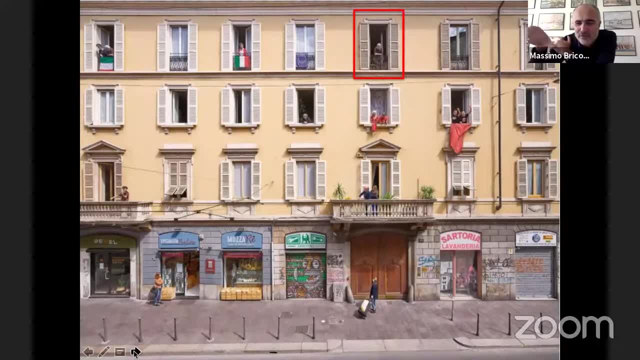 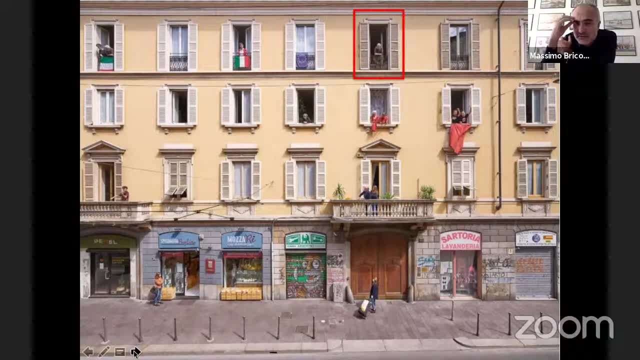 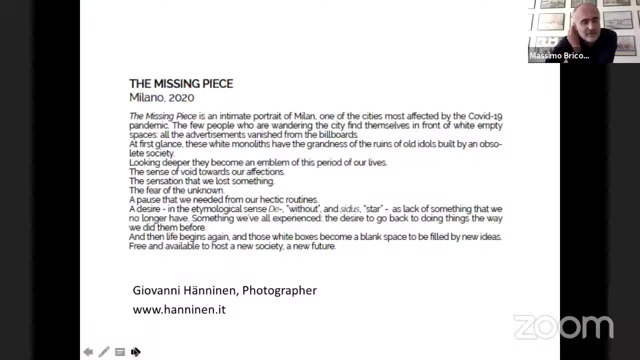 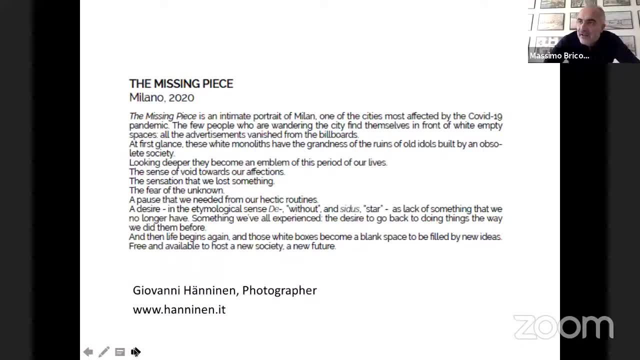 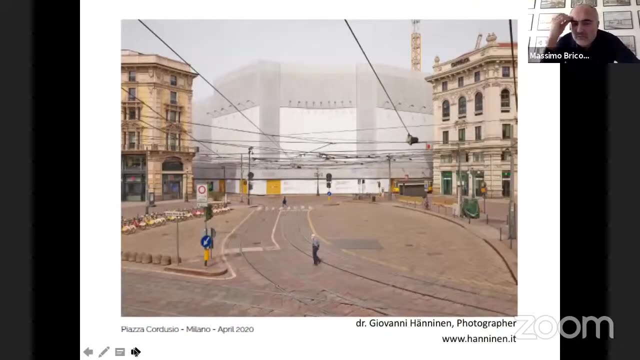 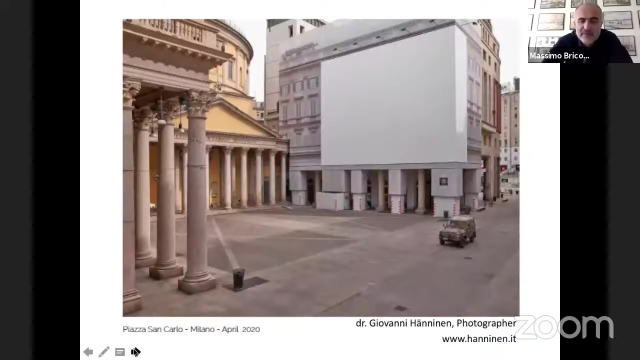 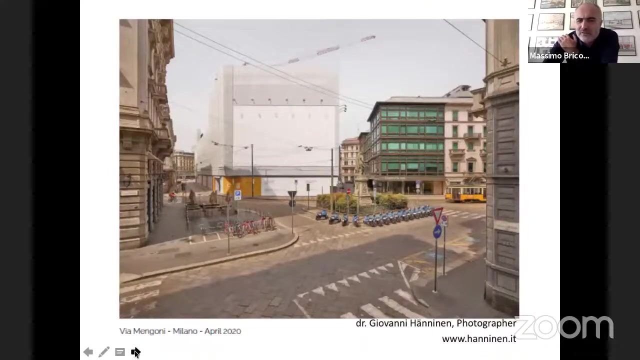 I can how he realized that all the advertisement boards, all in a sudden, just in one week, they all turned white. And I think this is a very symbolic metaphor of how much we were unprepared to such a sudden change. And I think this is really an issue for urban planning and for urban policies, how we deal with uncertainty. And so it was really like a city like Milano, which is very active, in which every square meter on a facade is a very high value, because you really have to pay a lot to put an advertisement. In just a few days, it became all white. It's like being erased and everywhere. 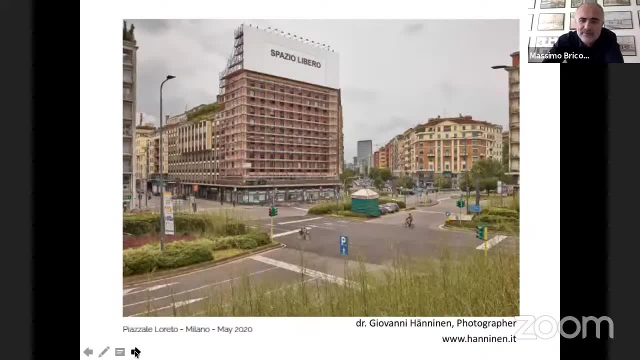 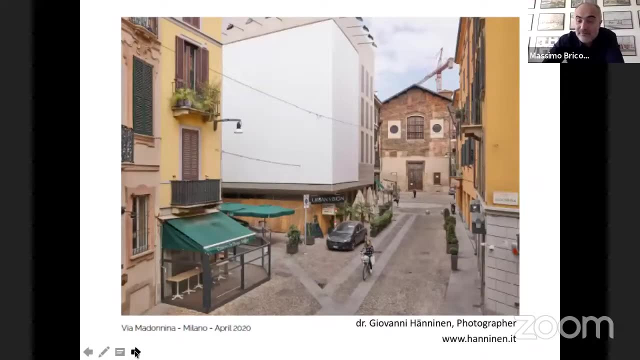 Somehow it's something we don't even realize, because we think it's normal to have advertisement, and then all in a sudden, this disappears, and it was really very impressive. 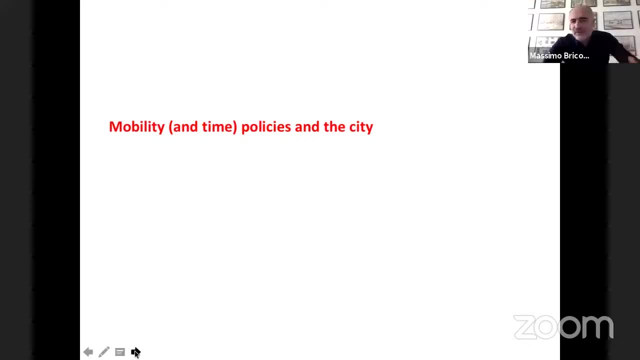 A second, so after, when we started to go back after the, so unlock, the lockdown was over, 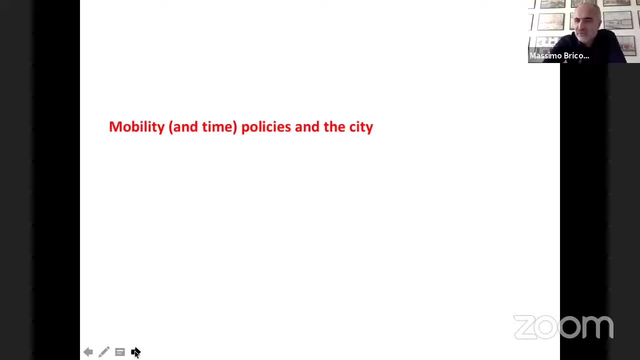 there were some, urgent issues which really needed to be dealt with. And to me, it's really interesting to see 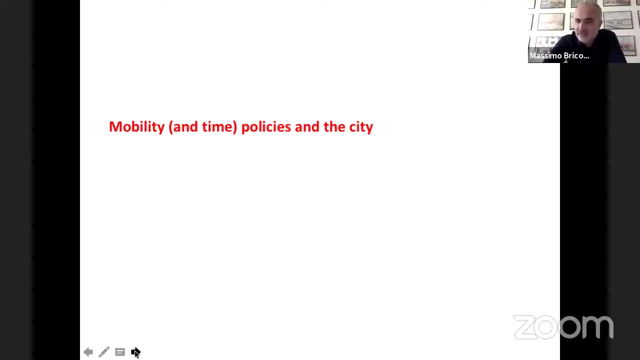 how urban planning and urban policies have been dealing with issues that I've personally been working on in these years, but it wasn't a kind of acceleration. And you may have heard in Milano, 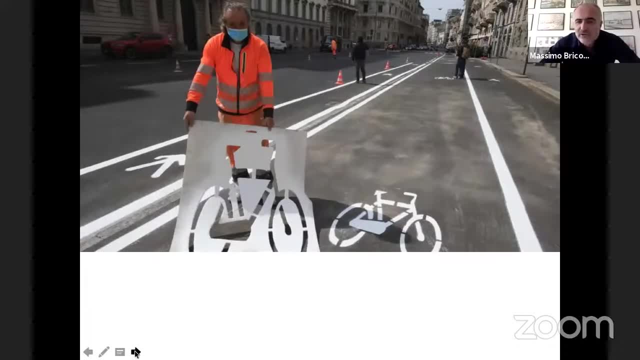 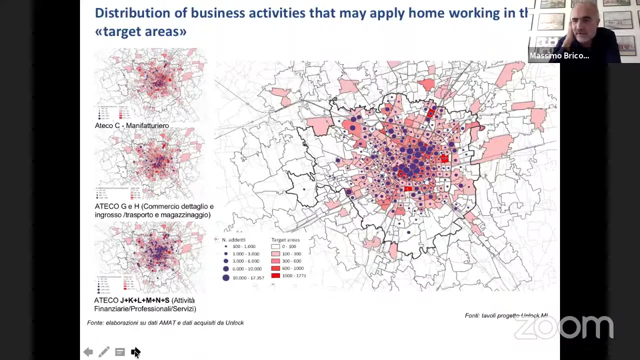 one of the first decisions was to draw kind of pop-up bike lanes. So in many roads, in many major streets, after many discussions about having bike lanes, bicycle lanes in the years, in one week, somehow it was decided to have these pop-up bike lanes. But more after it, the main issue became how to organize mobility, how to reorganize mobility, and how to deal with public transportation, which was absolutely in pressure, and still it is. And this is one of the work we have been doing as kind of policy advisors for the city of Milano, to work on this issue. And what I would say is that we realized that in a city like Milano, which is very much planned, and it's very rich, and the administration is very structured, 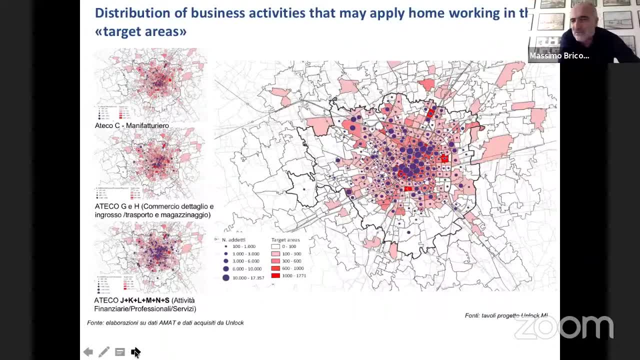 we had very little information on how the city is working. So this is the work that my colleagues 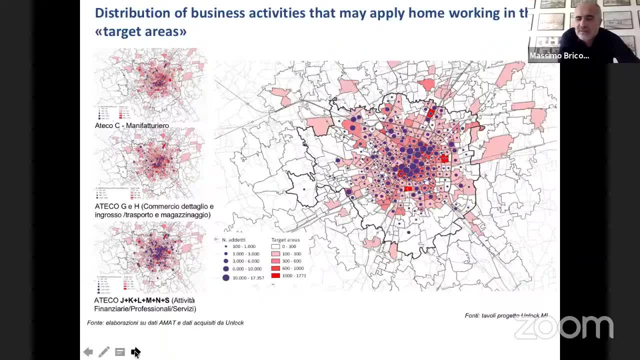 dealing with mobility developed. And we have been working on, for example, the urban planning, but it was, we realized, for example, that we have very little information about all the private 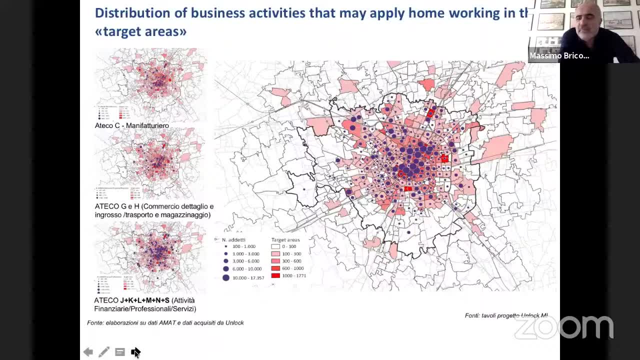 sector activities. So how many people are in a skyscraper, which is used for offices? It's like, 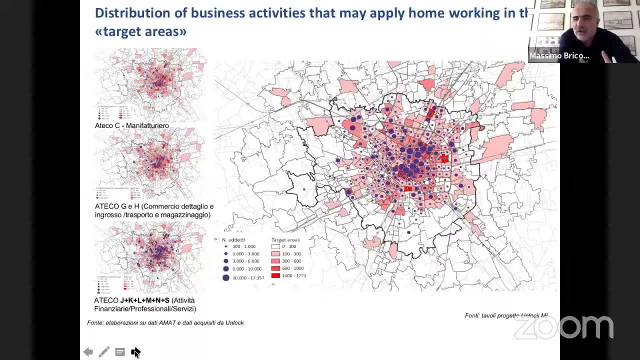 it's very rough data. And when you have to develop policies for smart working, home working, and to relate to mobility, it's like planning has not been 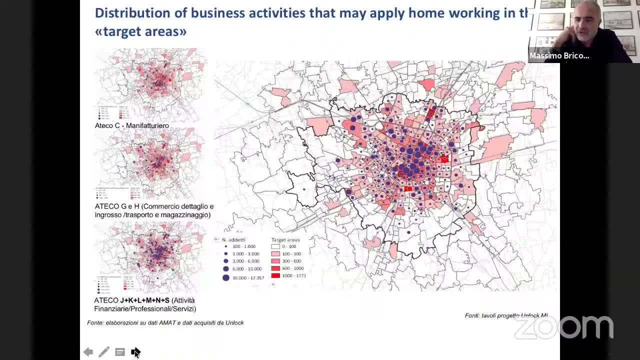 been dealing with the existing city. So very much oriented to work on new developments and to draw new schemes, and very little knowledge on the existing city, which in our context, all over Europe, this is the main main issue, we are dealing with a city which is not growing, 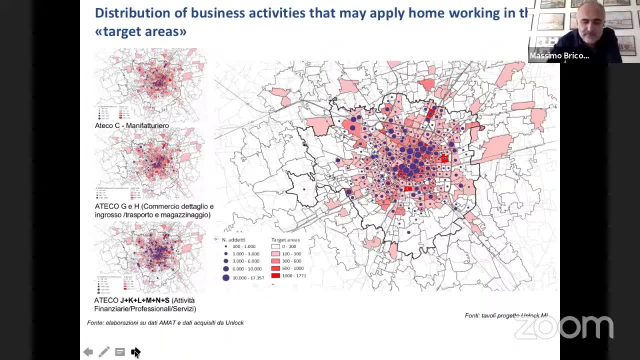 but it's changing very intensively. And another very relevant issue was 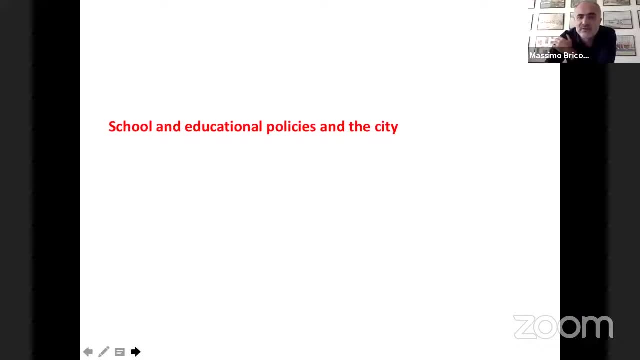 schools, because after the summer, our schools would start. And the issue is how you can deal with social distancing in schools. And, and, and there, what emerged is 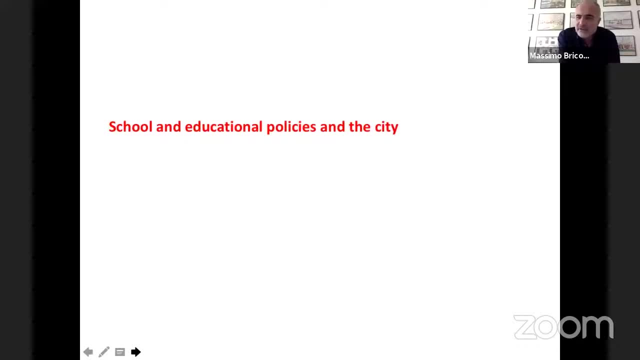 that there is an incredible gap between how the urban planners have been dealing with schools, as kind of standard services. So you have a catchment area, you design the size of a school, but this is not the case. So, you have a catchment area, you design the size of a school, but this is not the case. 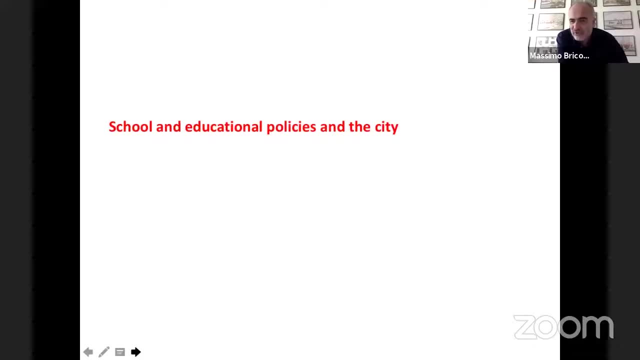 So, you have a catchment area, you design the size of a school, but this is not the case. So, the scheme for developing and for grow for a growing city and schools in our city are very old, they are there since decades, it's not a matter of building new schools, but to understand how 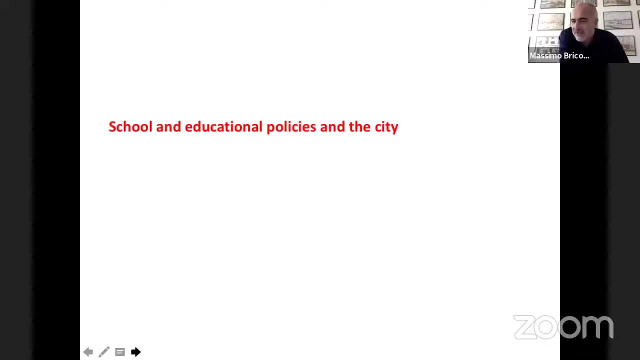 existing schools are working. And we realized that planners had no knowledge. And so all the educational policies and the school policies that needed to be developed in these months, there was no basis. So, 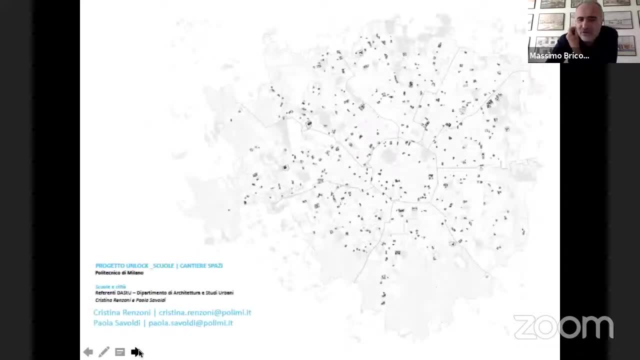 here you see two colleagues of mine, which you see here mentioned, Christina and Sonia, they developed an incredible work with some younger colleagues and they met all, here you see the map of Milano and you see all the primary and medium high schools of the city. 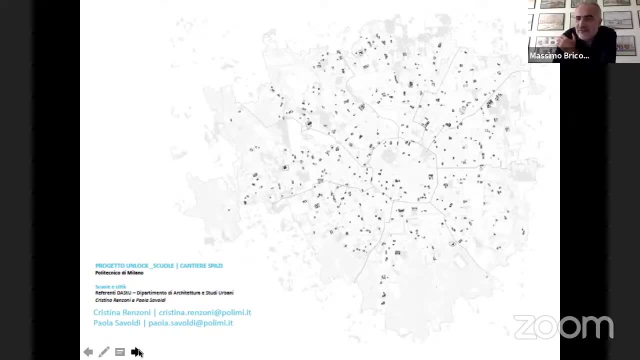 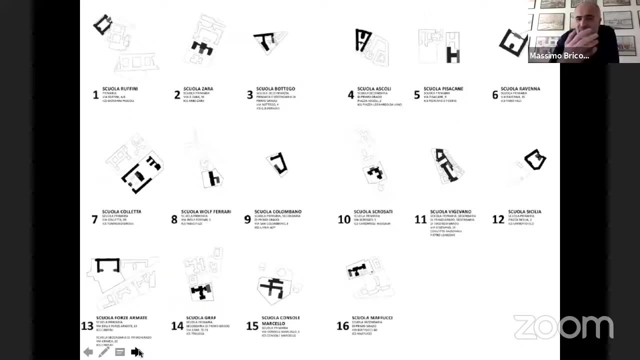 So, it was a tremendous work to be done, but it was really relevant to map the problems of an existing city, not of a growing city. So to understand it's a kind of catalog of the different schools, different typologies. And then you have the big problem with the city, the development, 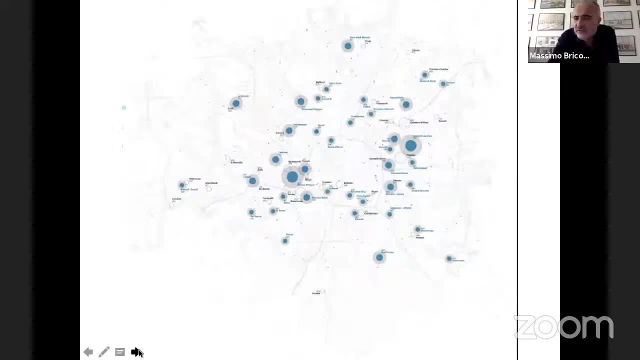 technologies and to then focus on the most critical areas where schools are at risk of not being ready to open because there is no possibility of social distancing and so like 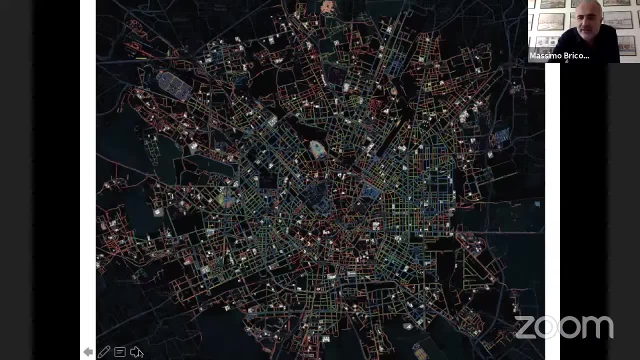 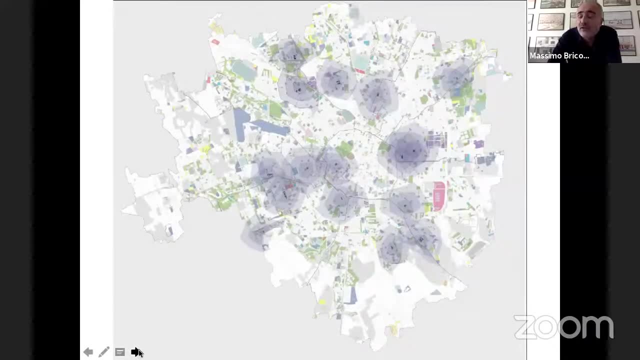 this is a map of all pedestrian so of all sidewalks and they developed more and more an analysis on on at the level of the neighborhood and here we step into the issue of this 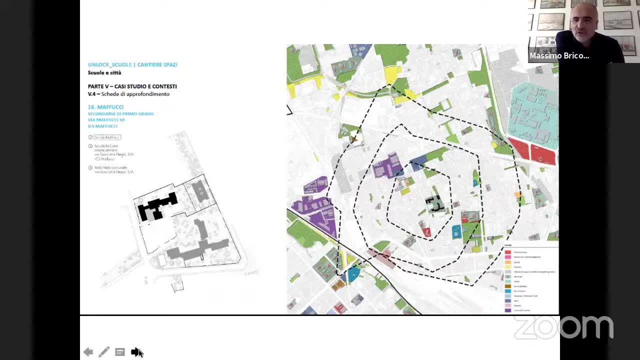 now the kind of renewal of the issue of the neighborhood as the context in which in fact you can really have a life now within 15 minutes this was a bit the reference so which are the services that you would require in case of limitations i think it's a very interesting issue because you 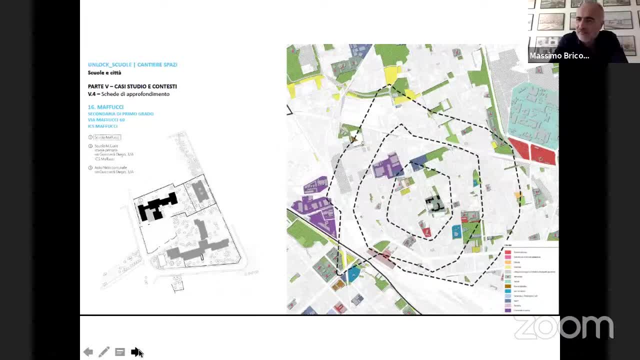 it really on the one hand we have digital tools and we all learn how to connect with people far away but then there is this materiality of daily life which became incredibly incredibly relevant and on which i i really believe that planning planning has too little knowledge we have it 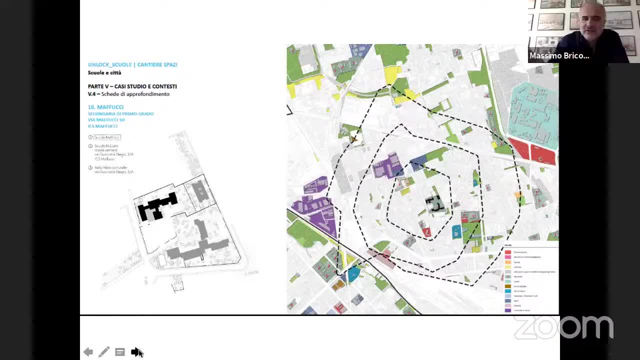 when we do some focus but on the on the city scale we we we have lost a bit the understanding of how the city 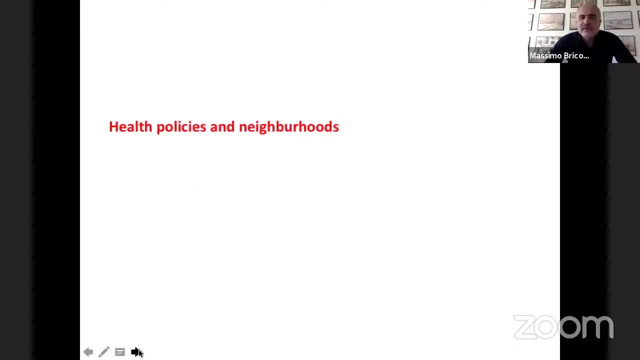 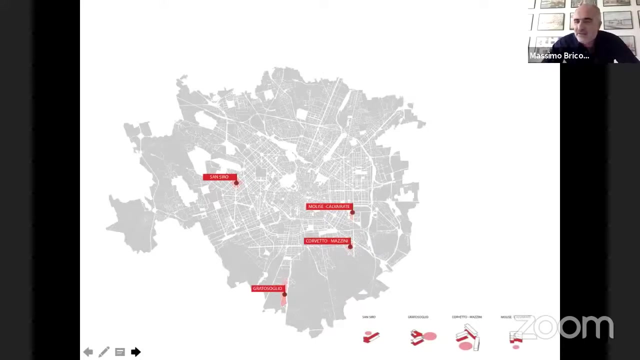 is uh transforming and another field in which i could really see these uh distances uh everything which concerns health because more and more planners have left uh the issues of health somehow have become something very specialized so uh more and more based in a hospital so the planners were really into planning for hospitals for large specialized hospitals and so on and so on and so on but these are mostly the places where we have as i said we have to have really specialized centers which are top level very relevant milano is a main center for qualified hospitals for the whole country so we have kind of health tourism people who come to milano because we have very good hospitals but we realize how important it would have been to have health centers at the neighborhood level and these were completely lacking and in some areas these has been really dramatic So, of course, I can be probably optimistic because I was kind of, for many years, I was working on this issue of bringing health to the local level, bringing health into communities. 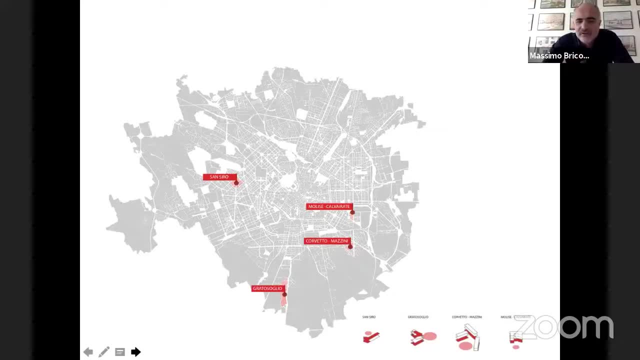 And this is a map, it's always Milano, and you see here four pilot projects which are starting in two months in some public housing areas which are the most disadvantaged of the city. And it's a program which is combining housing policies with health policies. 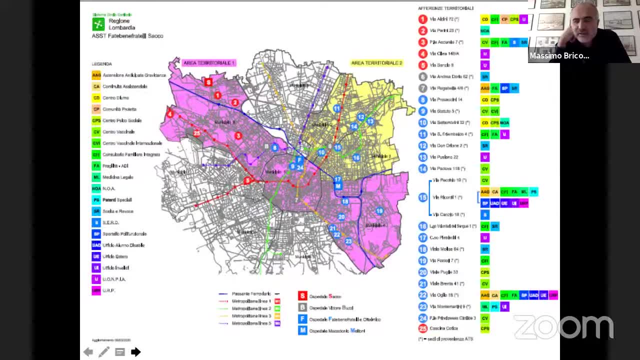 So this is a map which was drawn by the health agency, one of the several public health agencies in the city. And I was really finally very glad to see that a health agency, which is very much based on hospitals, is now looking at the city. It's just considering the city as a basis to work. 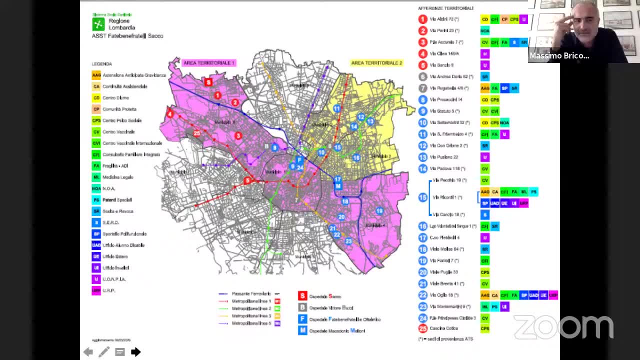 And I think that for planners, this is really important because they don't have knowledge of space, they don't have to draw this map, they really had to ask for help because it's not their vision. They normally are based on the hospital. 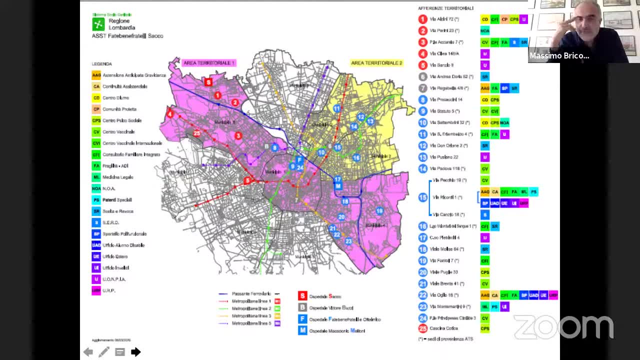 And I think it's really an incredible terrain for new policies which are matching. Different approaches. 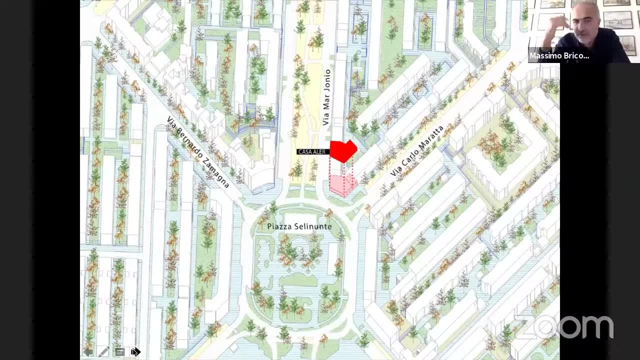 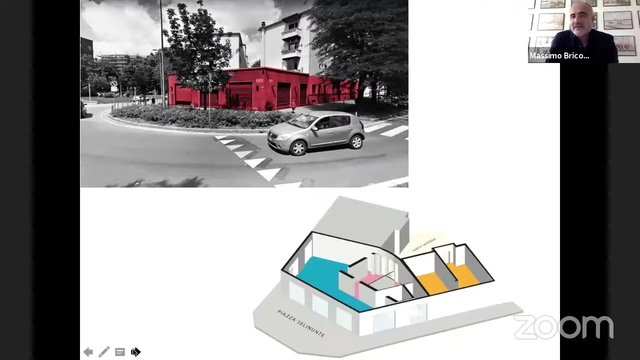 And here you see it's a map of one of the four housing neighborhoods in which some local community health centers will be based in order to avoid that people have to go to the hospital to have some basic services. And we have been supporting them in identifying some spaces that could work. And that could be available. 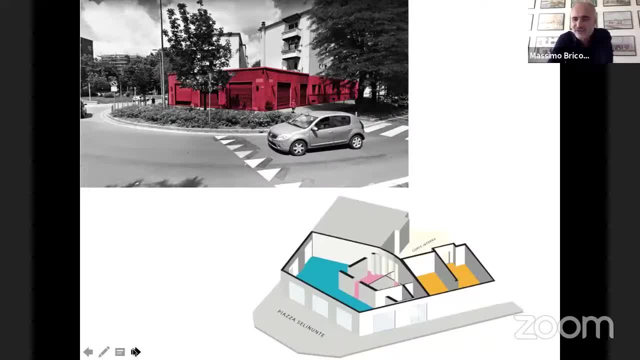 So former shops, for example, this is a vacant butcher, which will be transformed into a local health center. 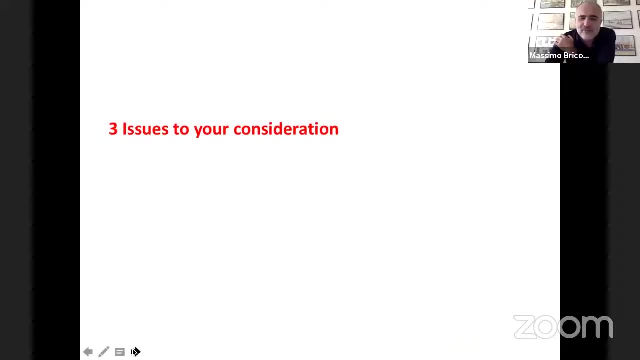 So I would end with three issues that I would put for your consideration. 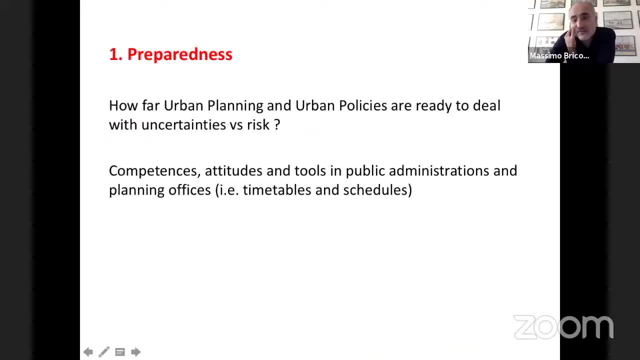 The first issue that I think was relevant but now really became an urgency is to understand how far urban planning and urban policies are ready. deal with uncertainties. And I don't mean risk, because we had a lot of research and discussion on risk prevention, both in urban planning and in urban policies. But I think that risk is somehow something that you can quantify. There is a lot of work, you can have figures, you can have projections, but the situation now was really challenging because it was really not considered as a risk. It was completely uncertain and I think that the first images of these empty white walls were shocking, something that you cannot really anticipate. And I think it's a serious issue for planning and policies because it really requires competences, attitudes and 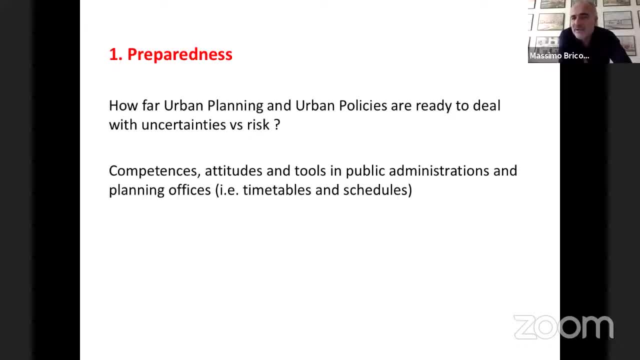 tools in public administrations and planning offices. For example, we are dealing nowadays very much with planning as a risk. So, it's not really a risk, but a risk. And I think that there 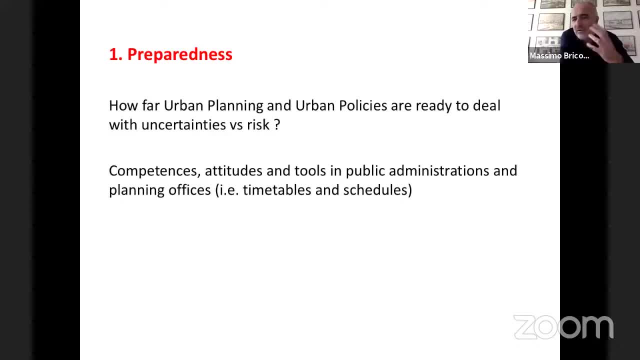 planning, rescheduling how space works in the city, so to change the timing of schools, changing the timing of offices, and we have little competences because mainly urban planners 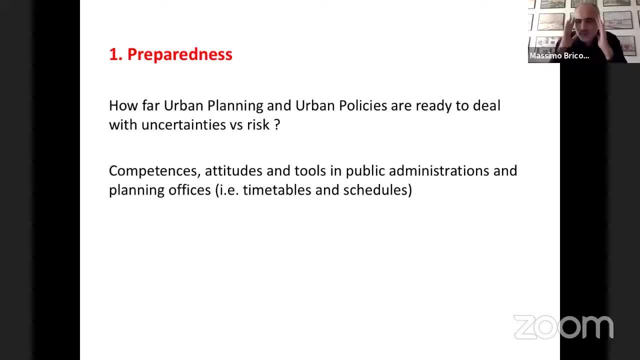 are very much structured to work on site development, on very physical entities, and much less into this policy orientation, which also seems very light and not relevant, while now it 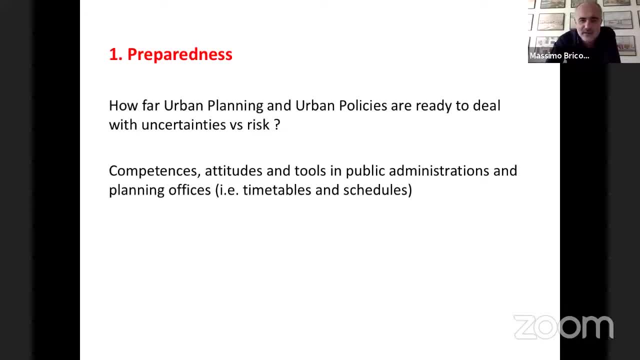 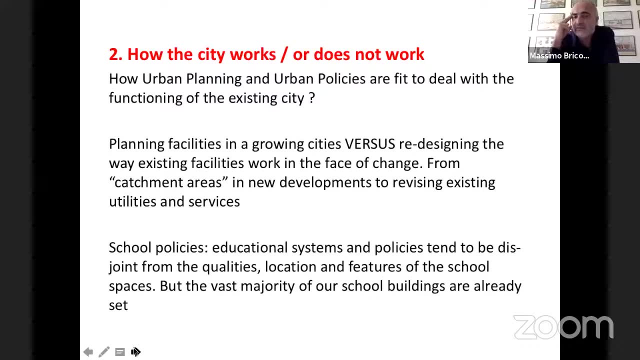 is really a hard core issue. And the second point is how urban planning and urban policies are fit to deal with the 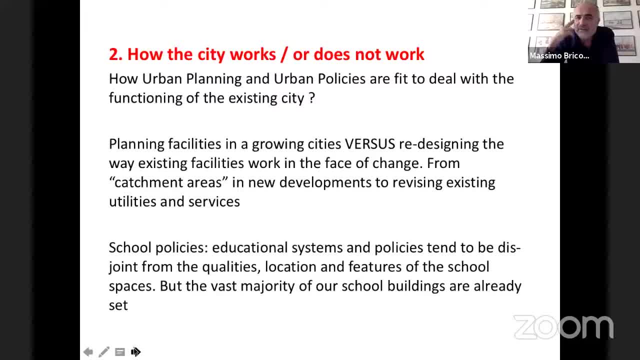 functioning of the existing city. I already said, I think planning is a discipline which developed in dealing with growing cities, so planning development. 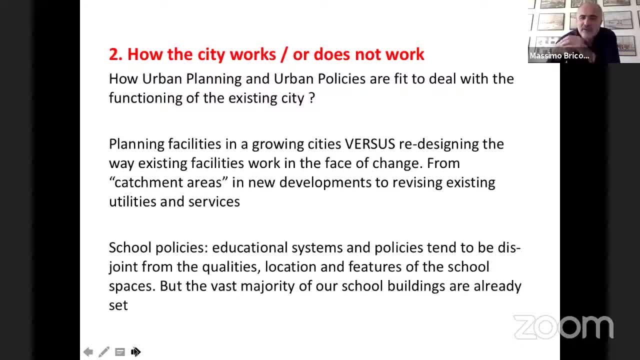 And now, it's really an issue of redesigning the way in which existing facilities work in the face of change, so it's not a matter of catchment areas, but it's really revising what is already there. 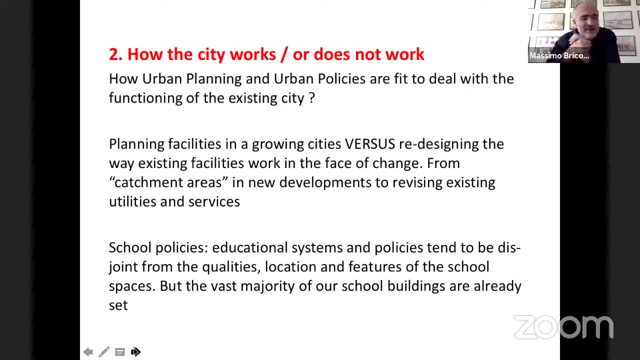 And this, again, I think also there is a kind of, it's like a taboo for planners to deal with small and little things. Many would prefer to work on more, not small things, but smaller things. Yeah. Yeah. Yeah. 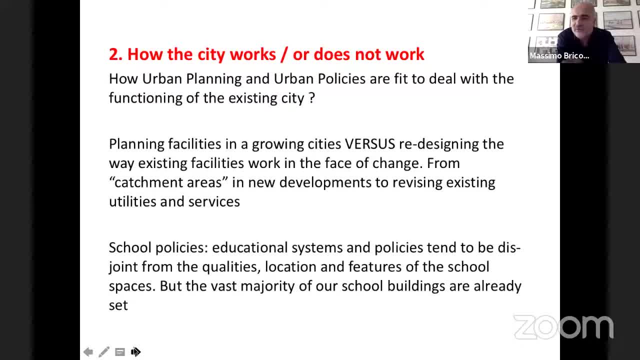 And I think that's something which looks more relevant, like a new development for a new neighborhood. But this is really what we need now. 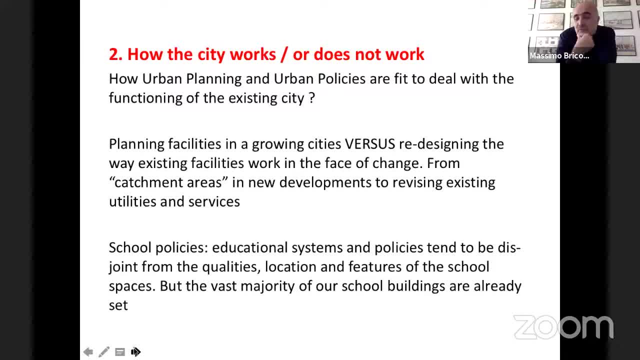 And the example of school policies was really relevant because anybody who is dealing with educational systems and policies, they don't have any knowledge about space, while we bring this knowledge. 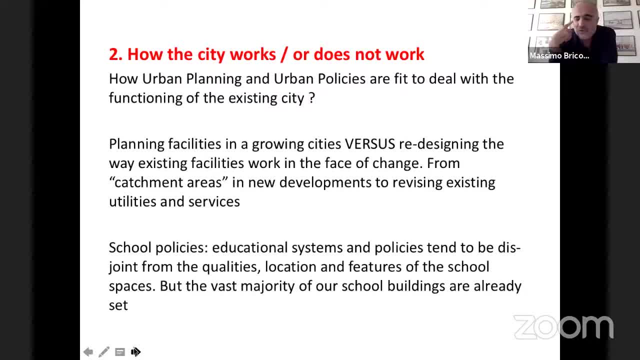 And we are realizing, for example, how much schools in this situation, in these 15-minute circles. 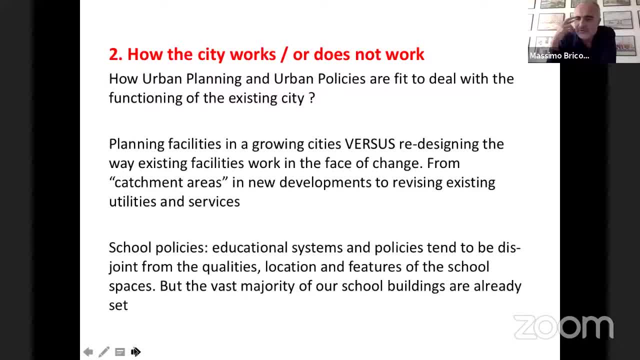 How much schools can really become centers for the daily life, because it's really one of the sites where all families of different ages converge. 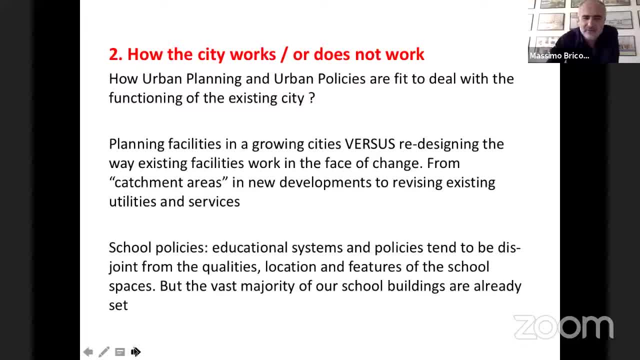 And we always undervalued these kind of spaces. So the third is a bit of a provocation, I would say. 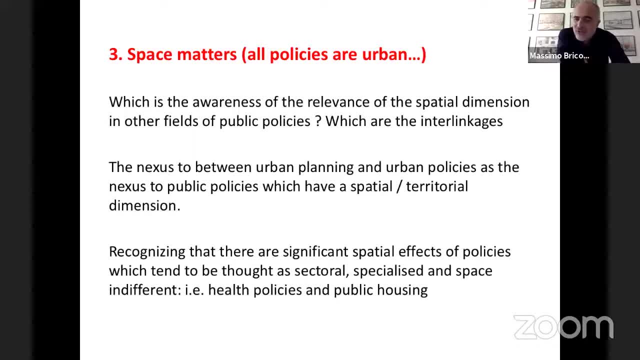 So I really believe that space matters, and it matters for all policies. So when we say urban policies, I think it's a definition that it's not so common. It's not so obvious, or it may be different in different countries. Of course, you can have an urban national policy. You can have a city national urban policy. But I'm really realizing that space is so relevant in other fields of policies, which are not urban in strict sense, but space is really relevant, and they have a very relevant impact on space. 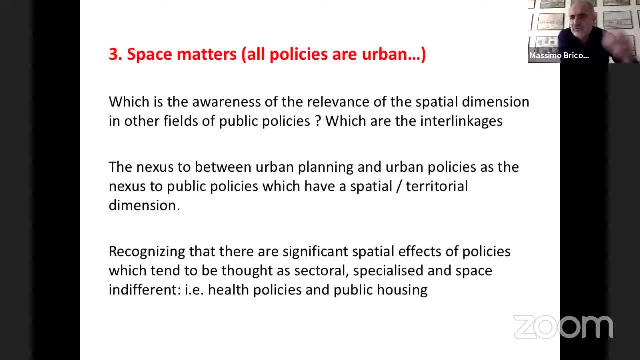 An example of health policies, I think it's really important, because between the hospital and the local community, there is a huge distance and a very different attitude. 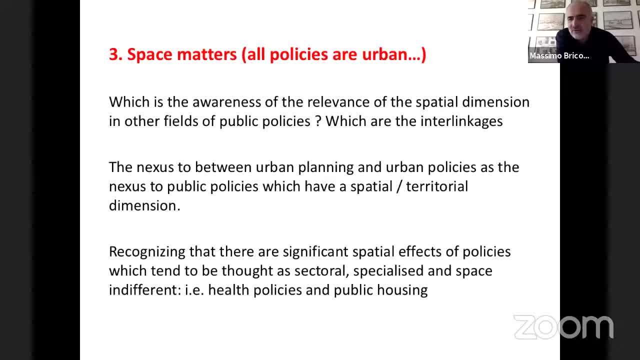 So we really would need to retrain, to train lots of staff in the health sector to work at the local level. 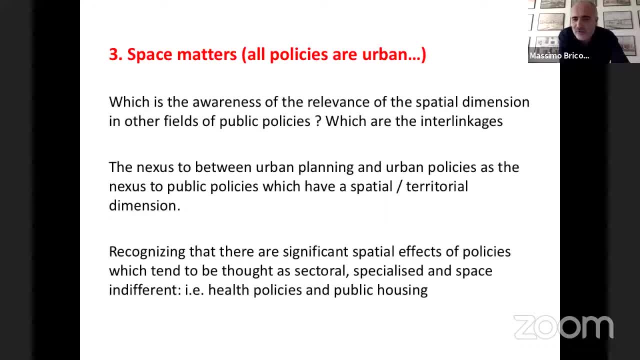 So I think that there are very significant spatial effects of policies, which we consider sectoral. They are specialized and space indifferent, while in fact, they are really relevant for urban development. Okay. That was it. Thank you, Massimo. 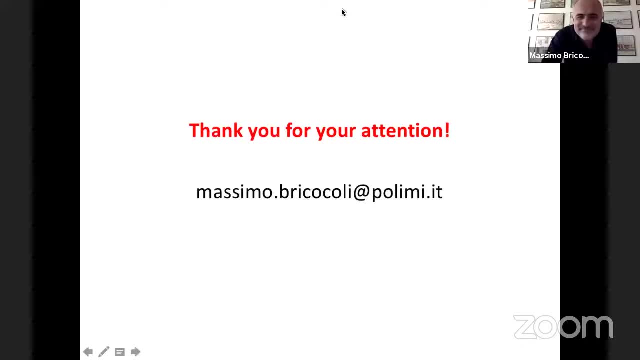 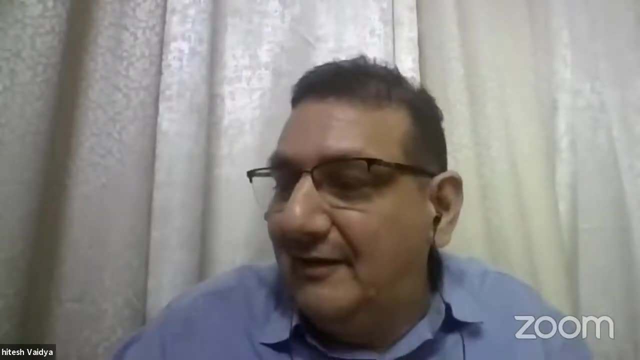 And that was a great presentation, and I think it really gives us all perspective how we should really reimagine our cities moving forward. 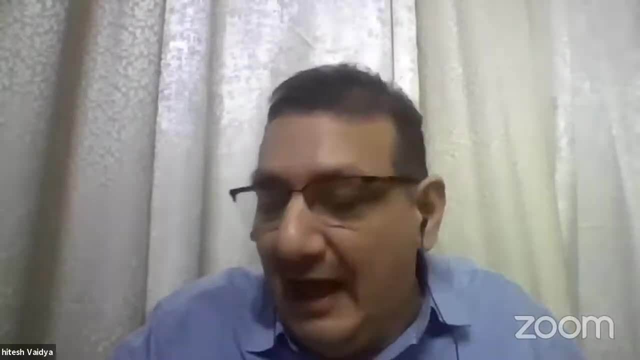 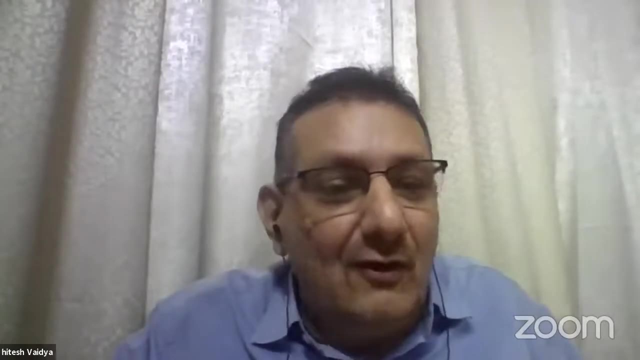 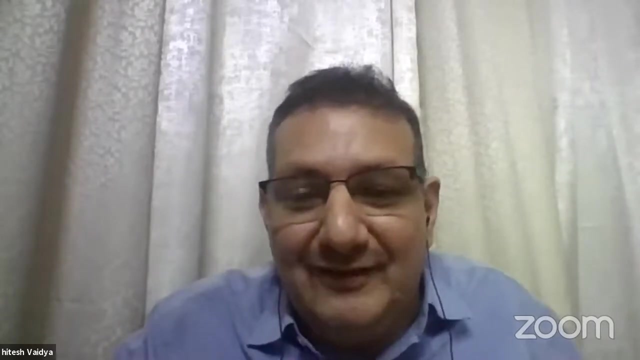 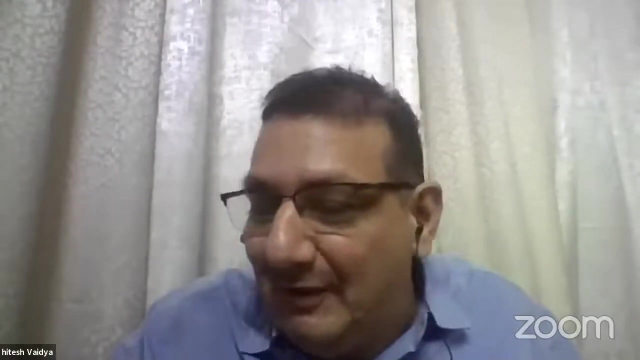 But, you know, we are also running short of time, and I just want, we are having a lot of questions on the chat box for the speakers, and I will, you know, in order to manage the time before I sum up, I'll take one question each from each of the speakers, and then we move, come up with a, you know, summing up, which is not easy right now, but I'll try my best. But right now, the first question I will, has come from, I don't know if you can hear me. I can hear you. 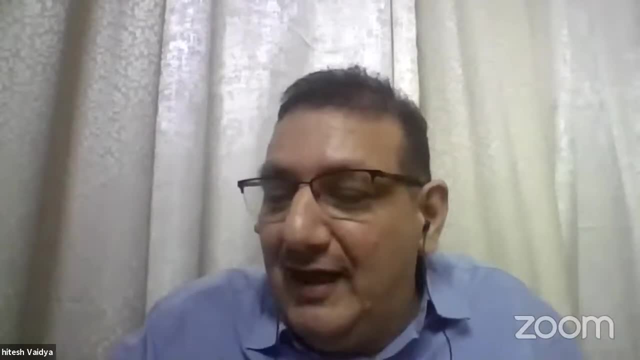 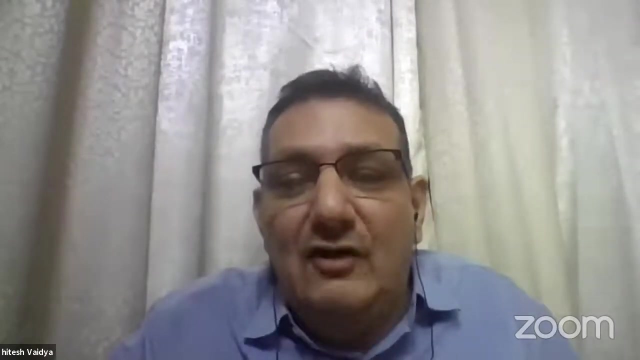 So, the first question is from the chat box to Professor Opey Mathur, sir, and it says that you have emphasized on evidence-based research, and you do talk about it is very critical for policy development and reimagining cities, but looking at the organization and institutions and their way, how do you see them focusing towards evidence-based research, you know, both in terms of finances as well as their priorities? Okay. Professor Mathur, over to you. I'm not sure I really understand the question. 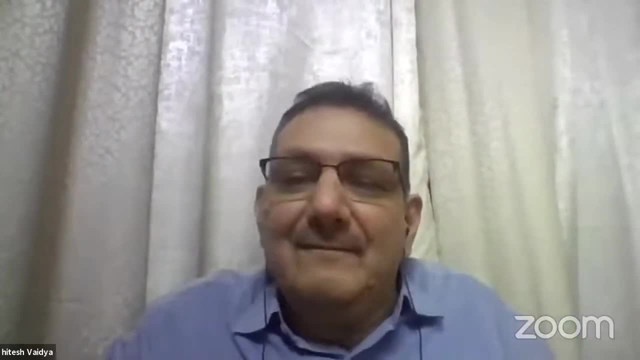 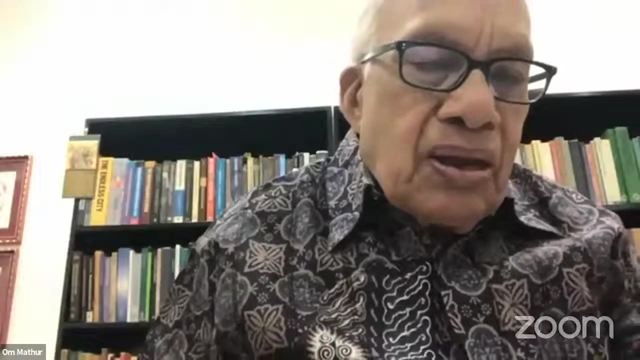 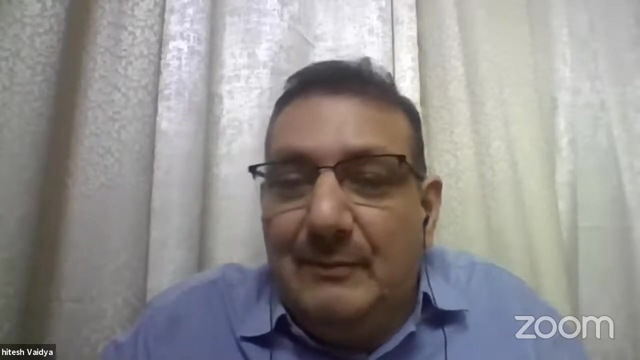 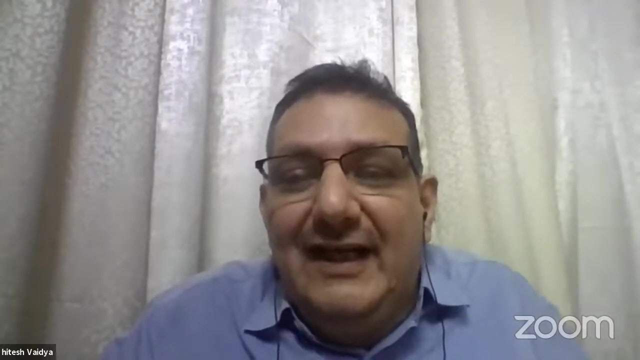 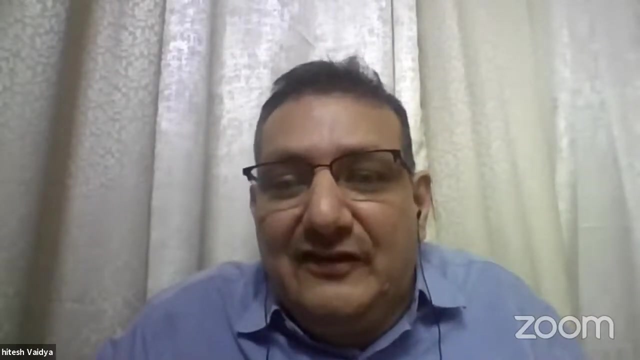 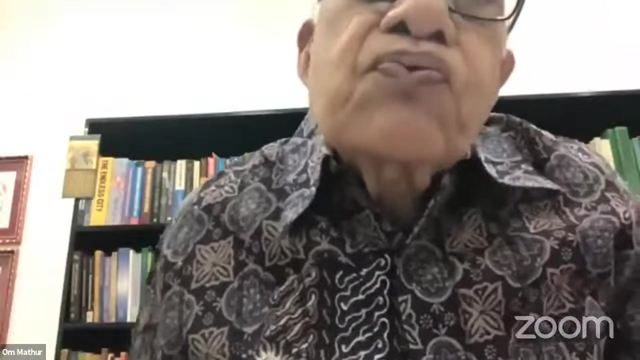 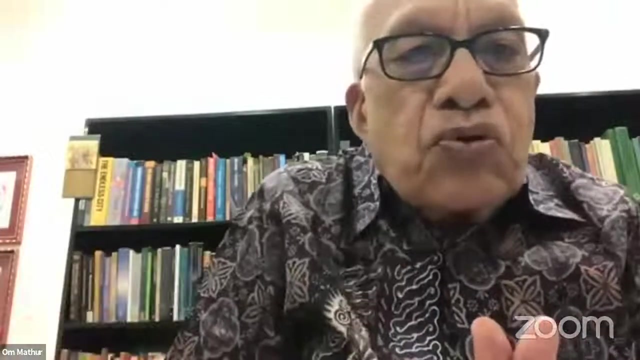 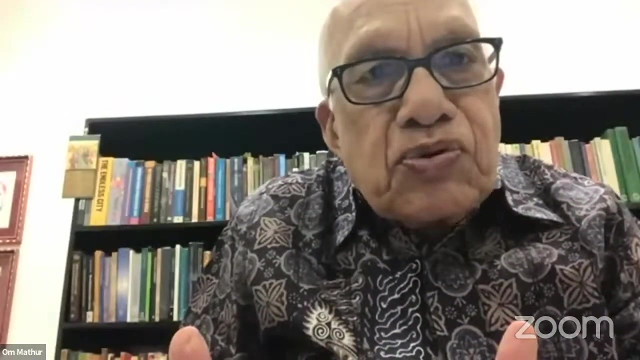 Sir, the question is that you are talking about evidence-based research, which you are saying that it is very critical for policy development, but the existing, yeah, existing institutional structures are more focused towards the, either the education system or either, so how do they focus themselves towards this evidence-based research to contribute towards the policy development? I mean, simply to take one example of digitization and agglomeration economies, if we do not know in what way cloud platform would affect agglomeration economies, how do we proceed? I mean, one alternative is to say, well, all right. 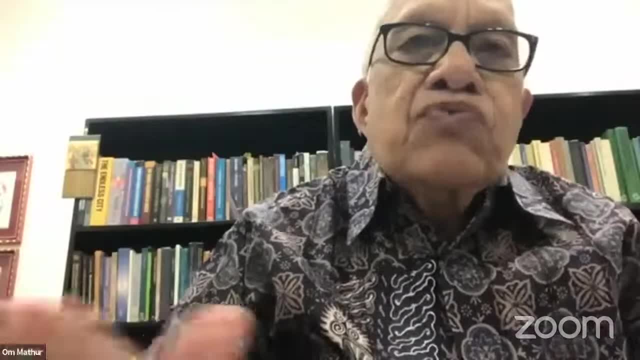 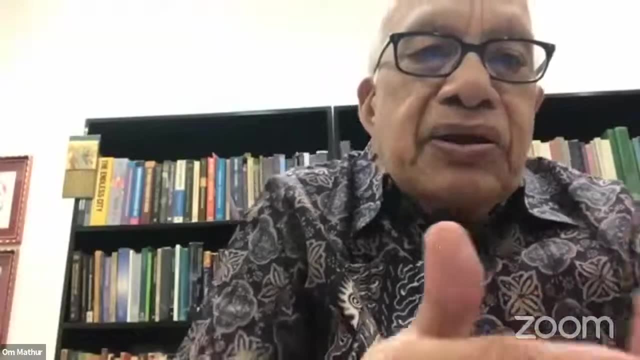 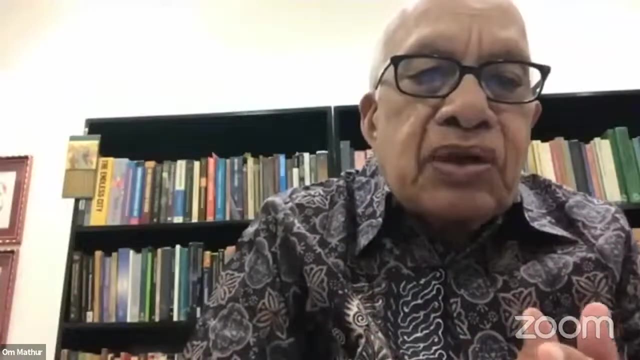 We understand that cloud platform digitization will make some context, some interaction unnecessary. But unless we really know from the field some examples of how it has really affected inter-industry relationships, what kind of a conclusion can we draw? What kind of a conclusion can we draw from this? This is just not possible. So this is just one example. 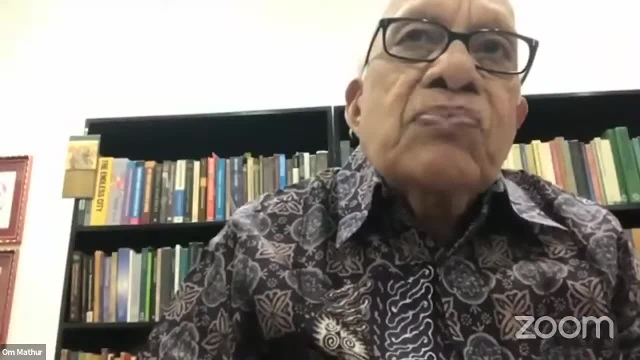 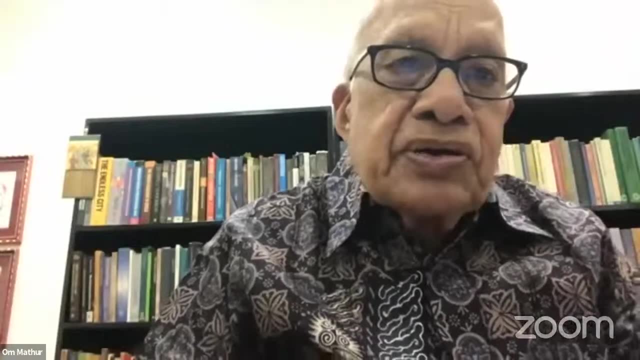 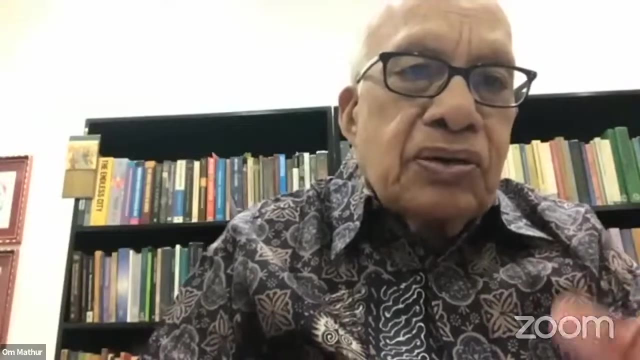 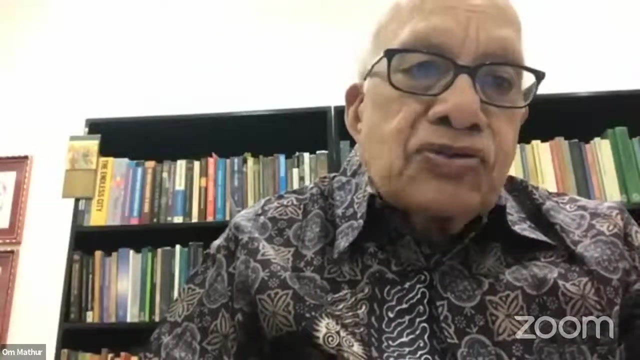 The other example is we have been struggling with the word sustainability for a pretty long time. What does it really mean? In terms of policy making, I mean, using the word is fine, but translating this word into what would be necessary for us to really move forward has not yet been conceptualized or made very clear. 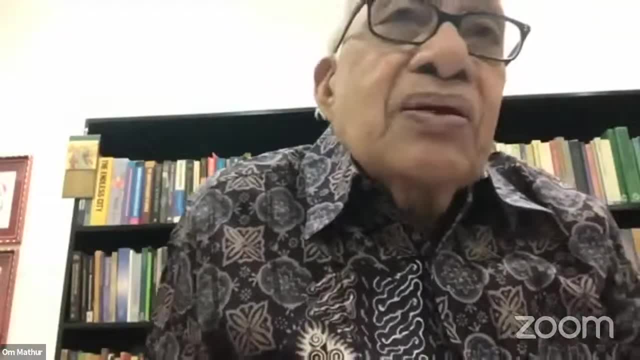 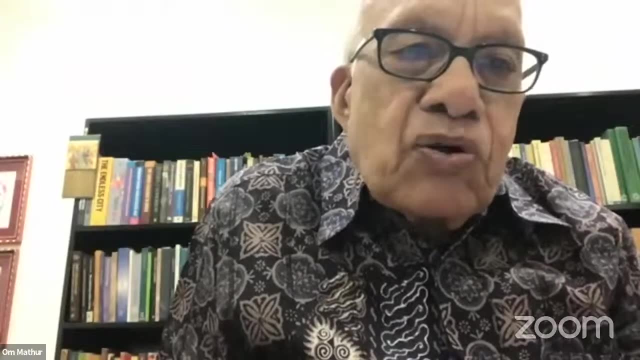 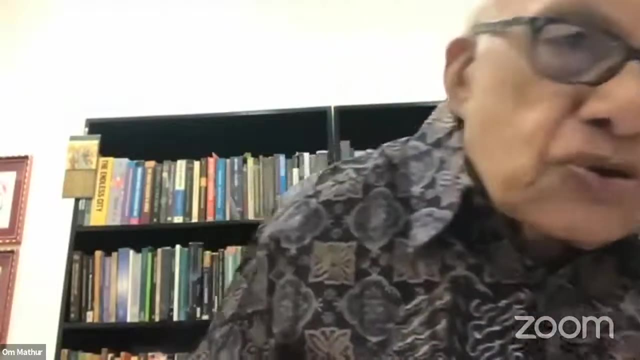 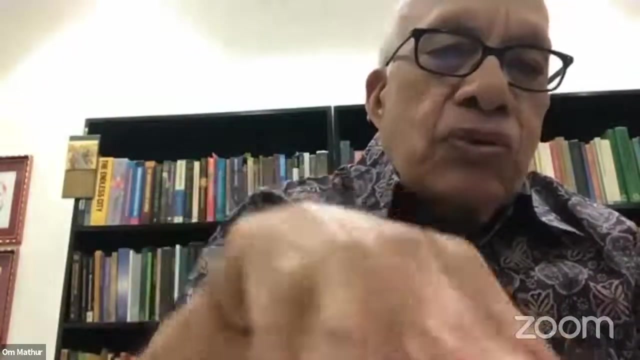 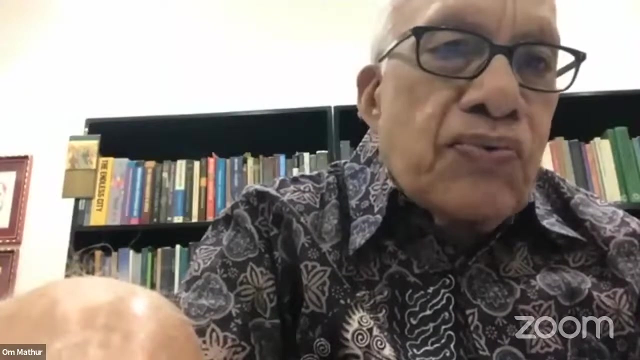 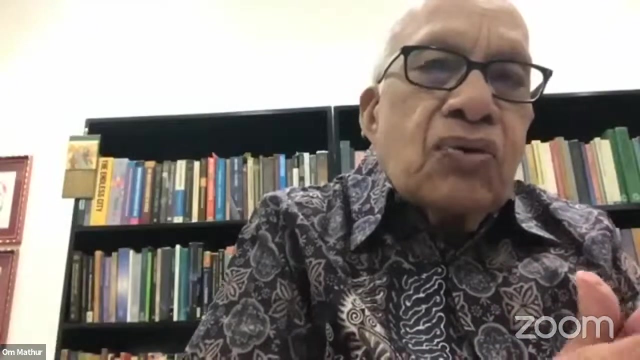 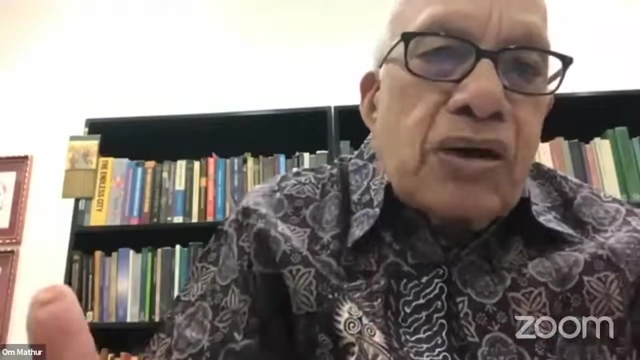 To give you a very practical example. As I mentioned very briefly that Partho, Rokhapadya and myself have been busy with the NITI Aayog, were busy with the NITI Aayog from October of last year until about March of 2020. It is very clear in what way, what should be done for in urban areas to achieve a 5 trillion economy by the year 2022. Now, it can be done in a variety of ways. It can be done in a number of ways. But any further guidance on what is open for us or what is not open for us was never made clear because it was never thought out in the NITI Aayog. 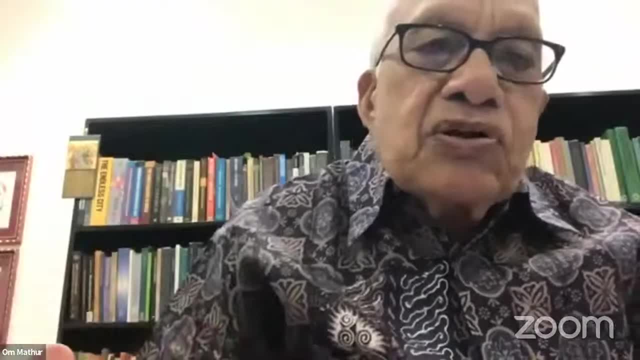 And the moment you ask this question, there is a complete silence. They have not even thought about it. 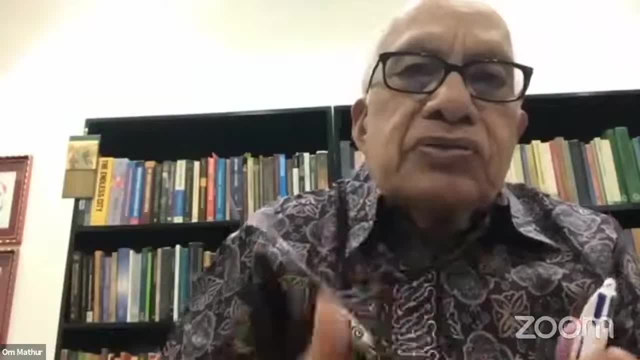 So in what way, what is at limit? What is it that could be done by cities and in cities that could make it possible for the country to do it? 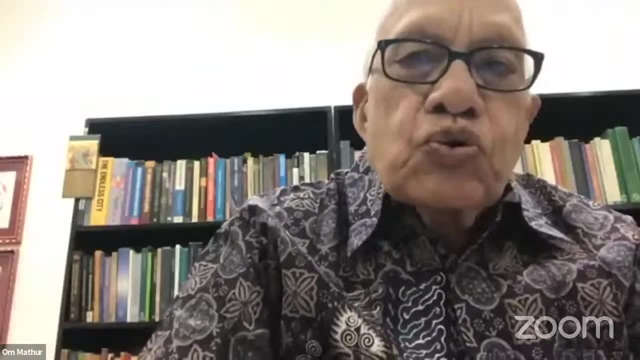 There are so many assumptions. And the moment you throw assumptions on them, the return is a complete silence. 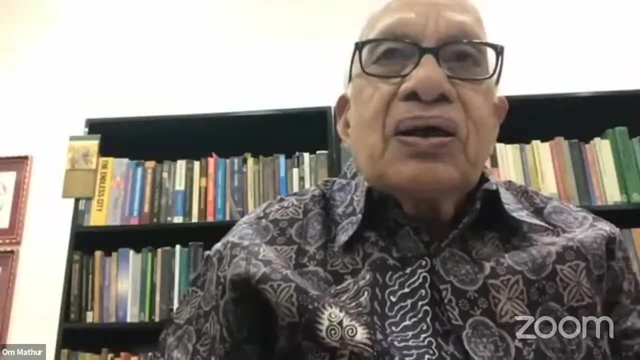 So that is what I really meant. And if we don't know the number of exercises which have been done, the famous one, the 10 principles and sutras and so on and so forth. 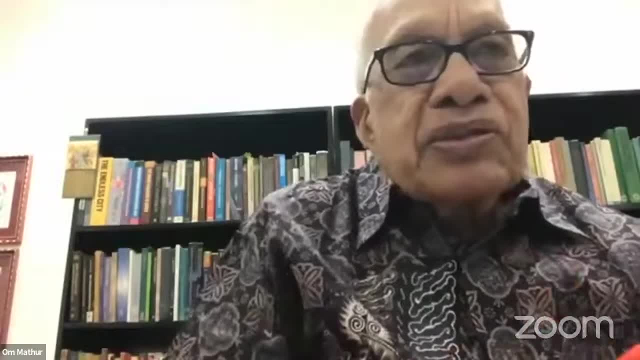 But the whole thing, to give you another example, you read some of the publications on meditation street. 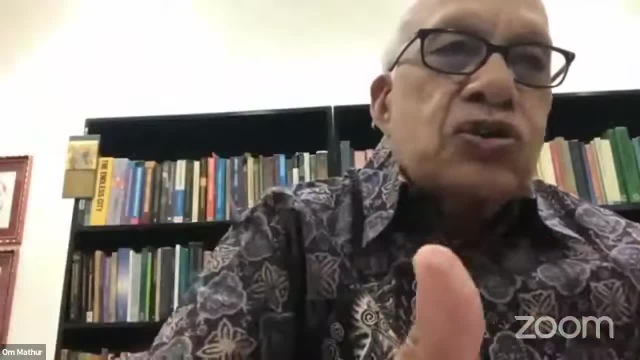 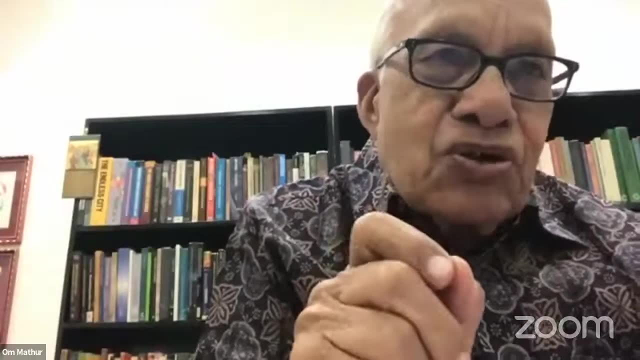 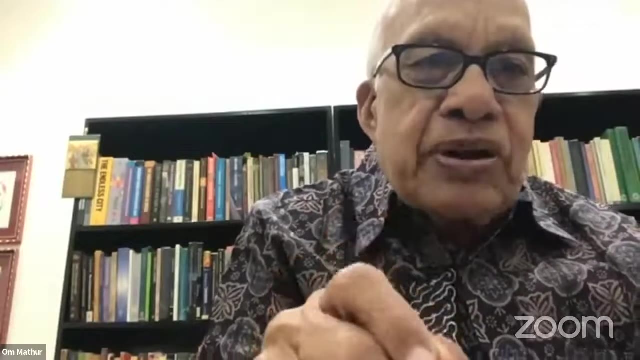 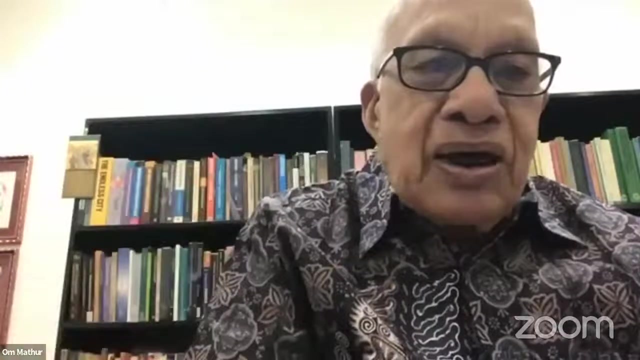 You read some of the publications which have come from the worldwide. I will show you, give you the page numbers, page numbers where urbanization is seen as slow, where urbanization is seen as moderate, where urbanization is seen as rapid, where urbanization is seen as messy, where urbanization is seen as unseen. Okay. 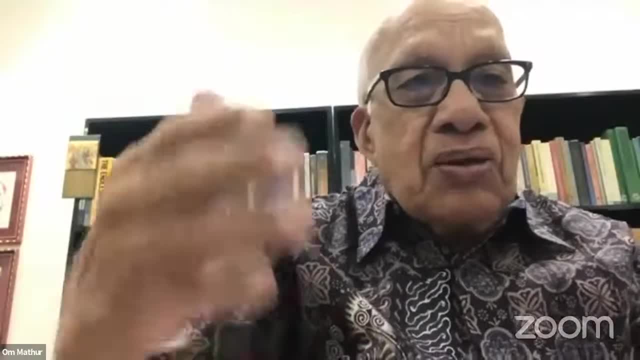 Now there are five different interpretations come, including from the government of India publication. 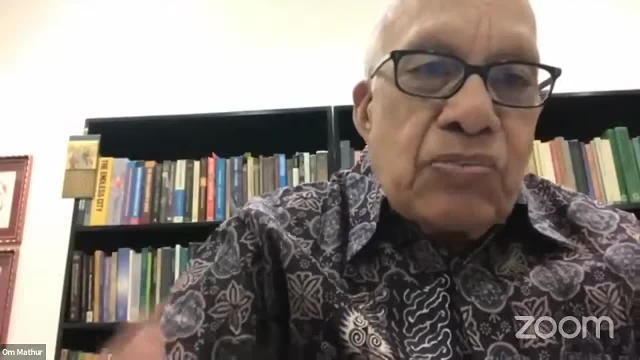 What do you make of it? The response to each one of them will be very different in terms of policy making. 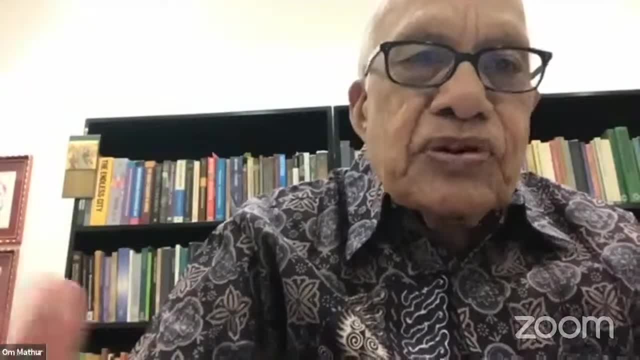 If it is true, the response will be different. If it is rapid, the response is very different. 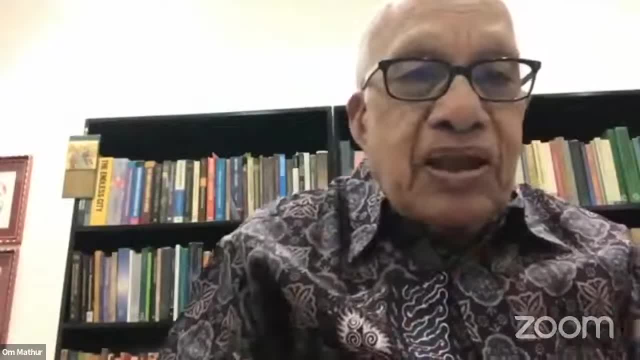 And including in the concept note that you sent, it says urbanization is proceeding very rapidly. 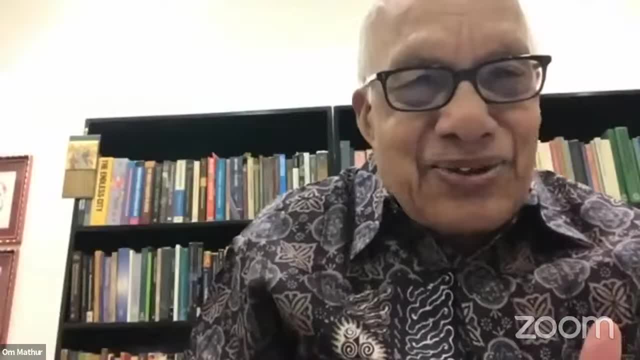 Unfortunately, that is not the case. Unfortunately, that is not the case. 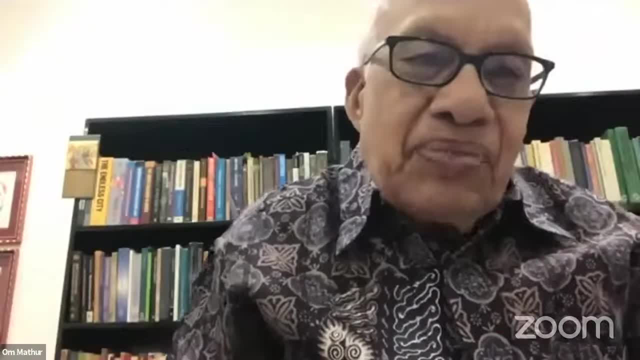 I wish it was a little more rapid. 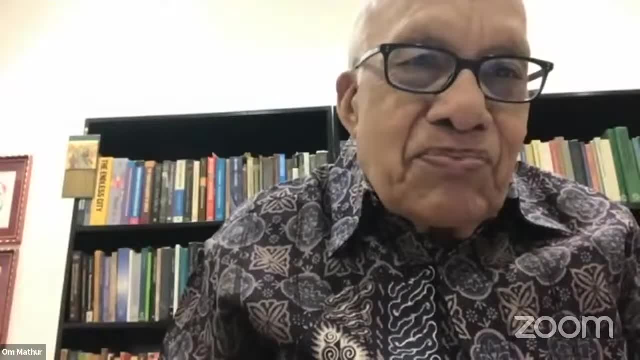 We will make it rapid by changing the definition, but not by the definition that we normally employ. Thank you. Thank you, sir. Thank you. 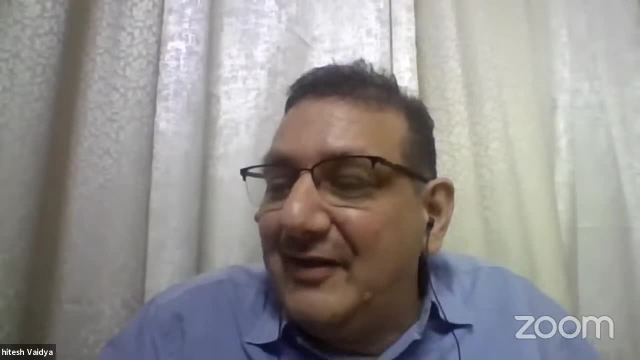 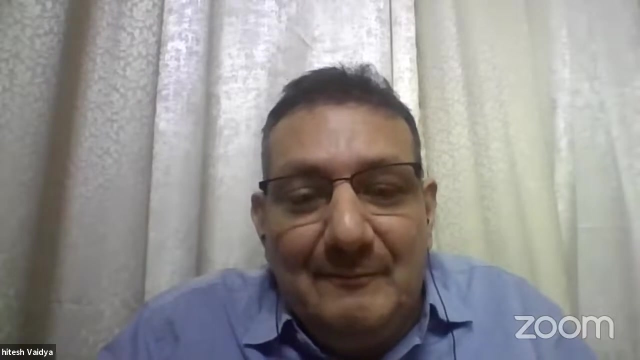 The second question is directed to Professor Ramachandran. Sir, you have talked about public spaces. And the question is, how can reservation of land parcels can be made at a local level so that we incentivize the green public spaces? 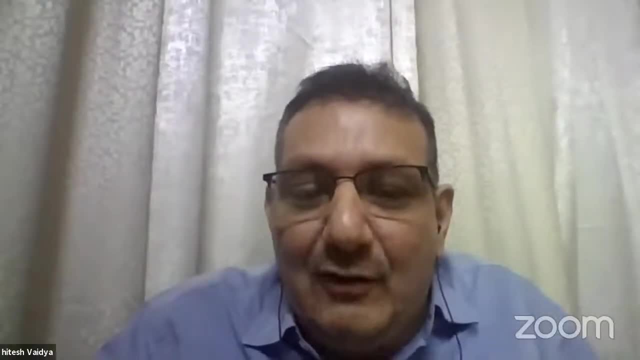 How can it be made at the local level? 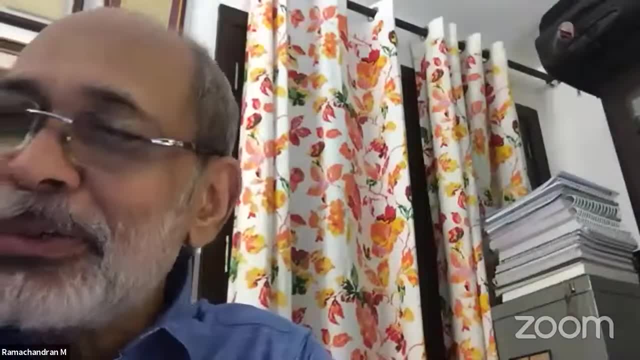 It is for the local bodies and it is for citizens to ask for it. 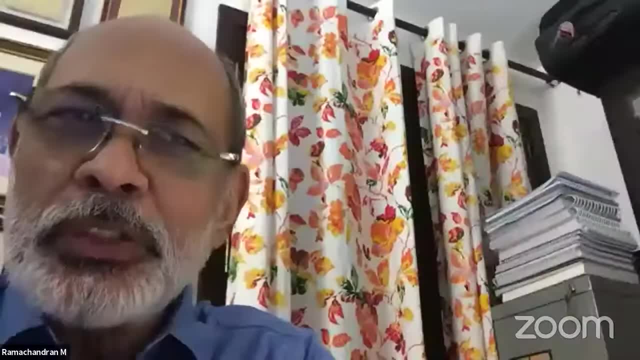 I would think without the citizens sort of asking for it, I would call for agitations and things like that. 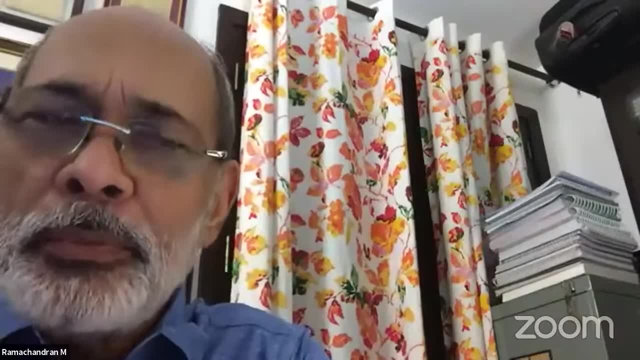 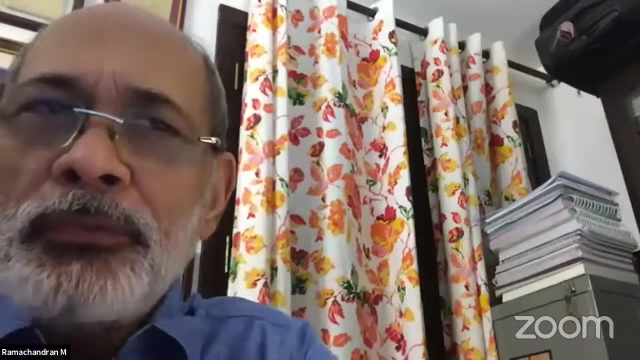 But an enlightened movement to prevail upon the local leadership that these are the chunks of land available, these should be earmarked. And those should get earmarked, notified, and probably there must be a method by which once notified, it cannot be taken back or it cannot be used. 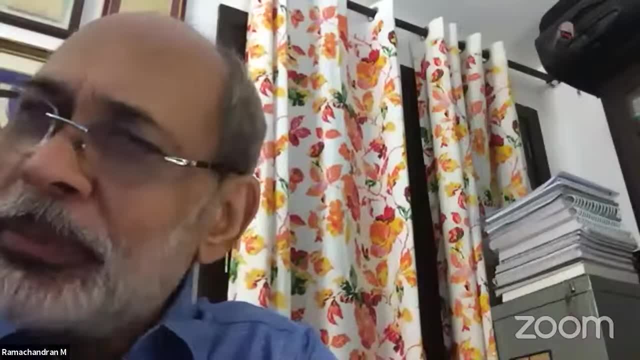 It cannot be taken back or it cannot be converted into any other purpose. Something like that has to happen. 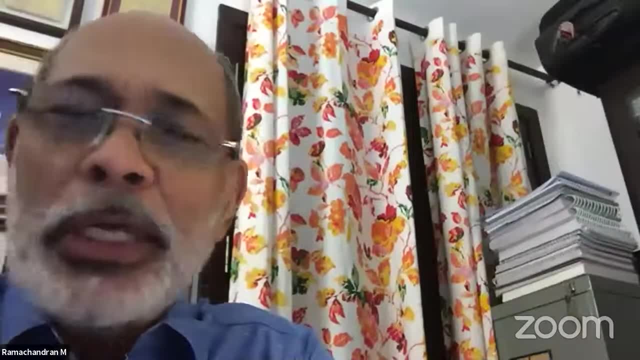 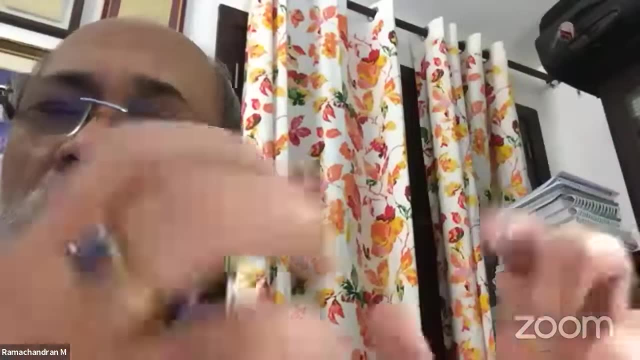 I mean, all these are things which we can dream about and we can advocate if it comes to maybe in half the cities if this happens, nothing like that much more green space gets added. 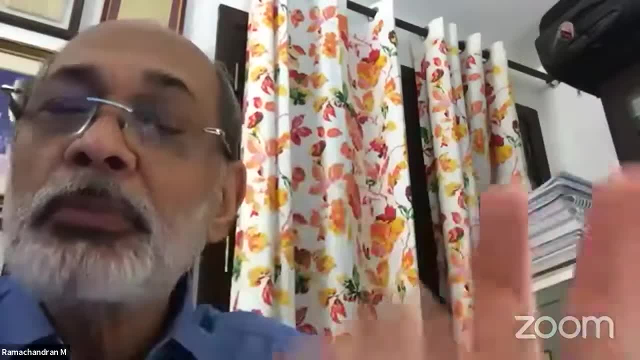 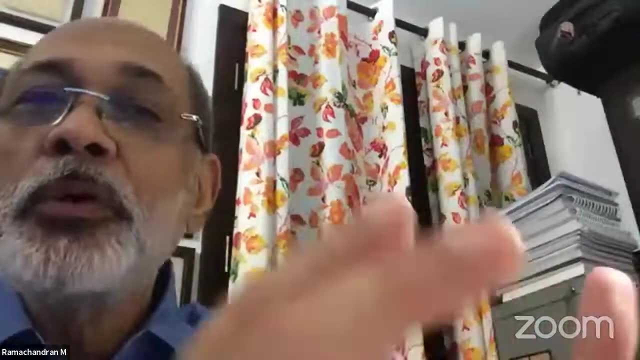 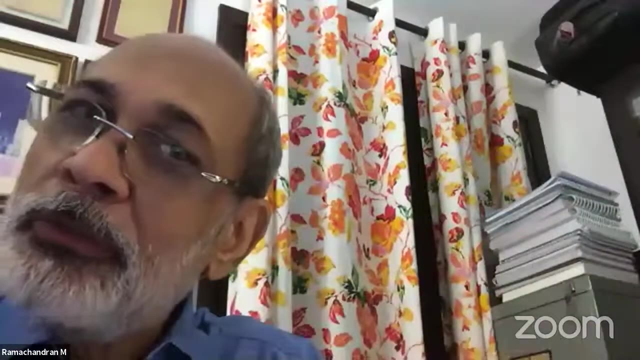 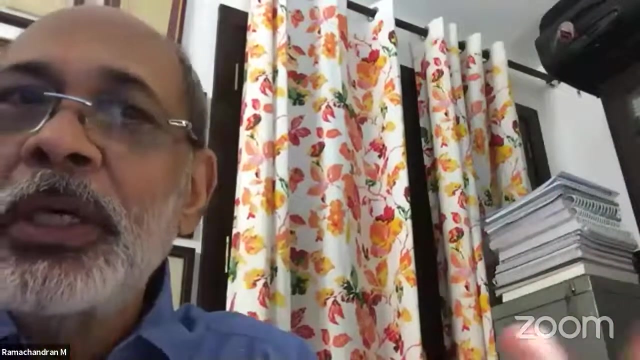 But green space is important. That has to be realized by all of us, more so by the younger generations, because the way construction is going on, the way cities are getting cluttered, I don't think there will be any hope left in the future. So whether there are water bodies, whether there are spaces left, in some places, local bodies would have left some space for some commercial activity. One has to think about it and it has to be well dispersed. I made a reference to the gated communities, probably getting more of the benefits of such parks and things like that. 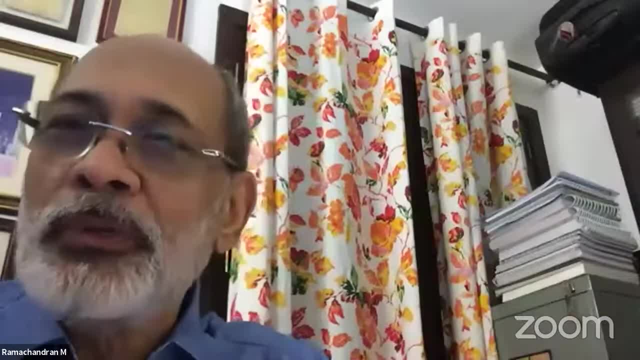 It should be spread out all across the city, all across the town, and it should be available. So, I mean, I don't know why we fight shy of demanding from our local leadership, these are the things which we need. And why should they be? 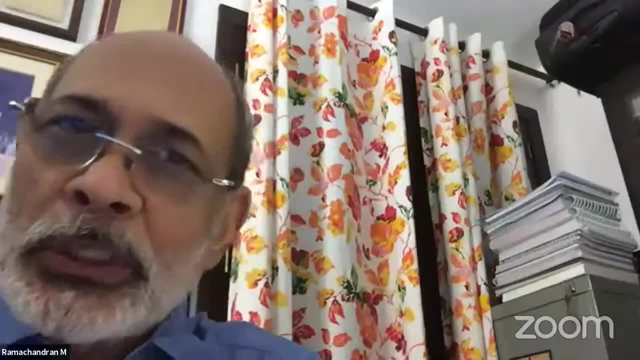 And why should they be on a different plane that, no, I cannot do this because they are meant for us. 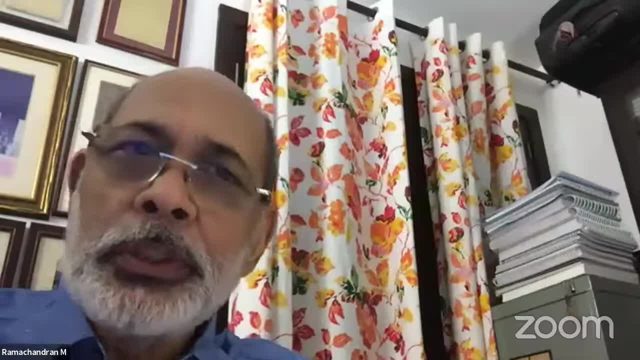 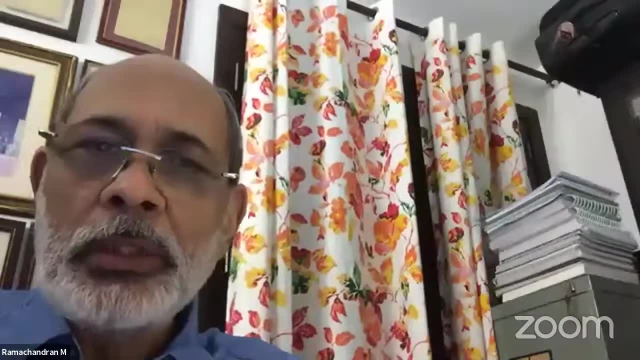 They are supposed to understand and appreciate the city much better. So there should be a dialogue process, an enlightened process of interacting with the city leadership and city authorities that this has to be done. These are the places. There could be excuses. 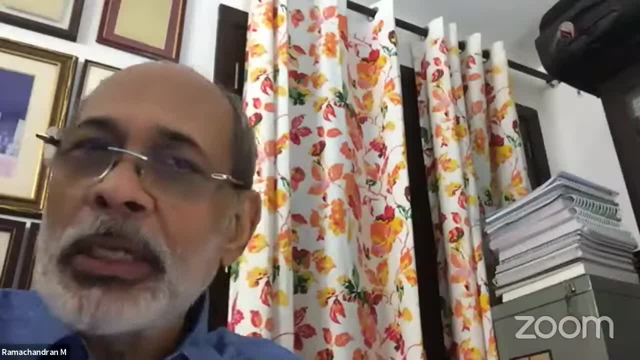 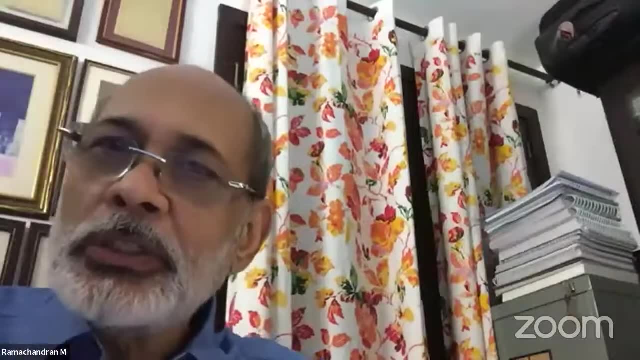 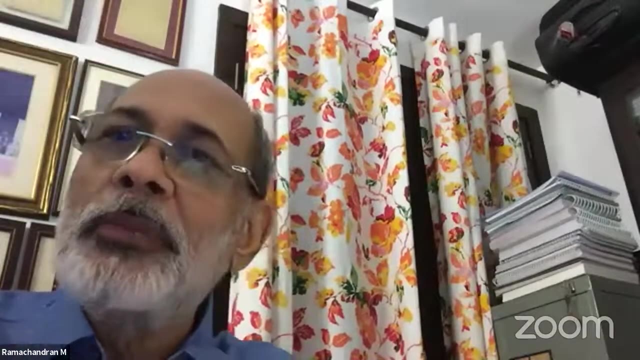 But then there should be a method of, you know, like I always talk about the service level benchmark for other sectors. Similarly, for open spaces, there should be a sort of a benchmark. What is my open space percentage today? To what extent can I take it in adding most of these or whatever is available or including what can be provided for? And we should ask for that and that should become available. That is the necessity. These are the current compulsions of the times. 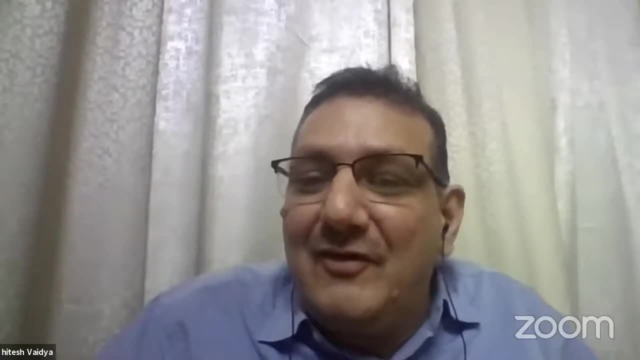 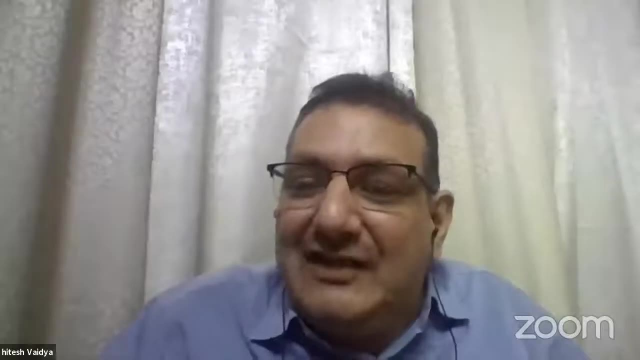 And the question is that you really talking about radical planning, but how do you see the local government institutions be changed or incentivized that they start becoming responsive for the informal settlements within the city? So, you know, it's to you. 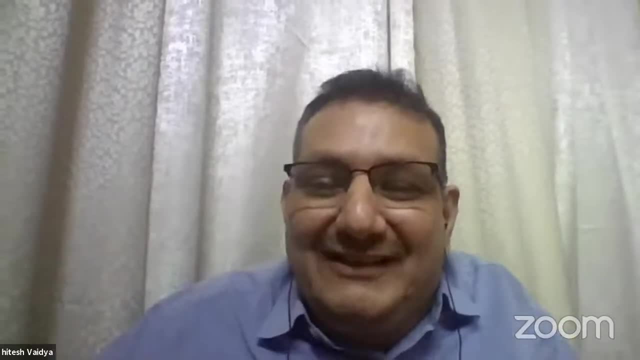 There are a number of questions to you, but I picked up this one because it's more talk about more institutional transformation. 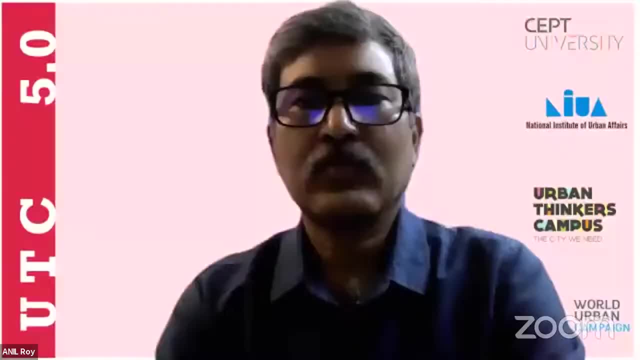 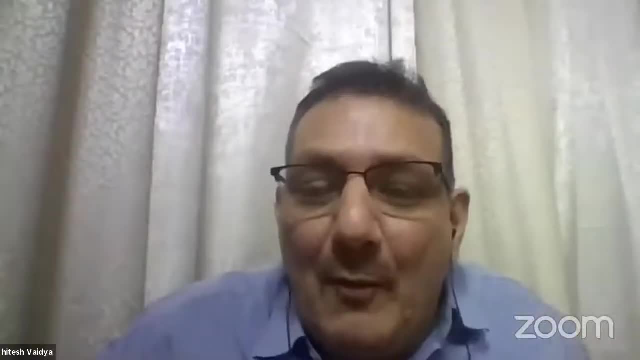 So over to you. You have to open your mic. 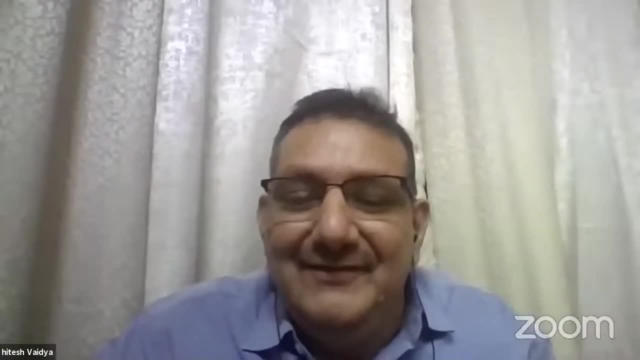 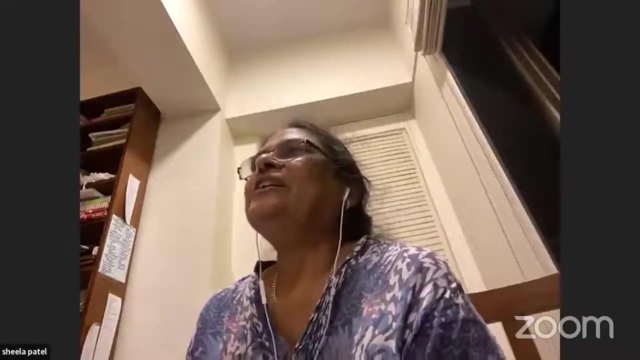 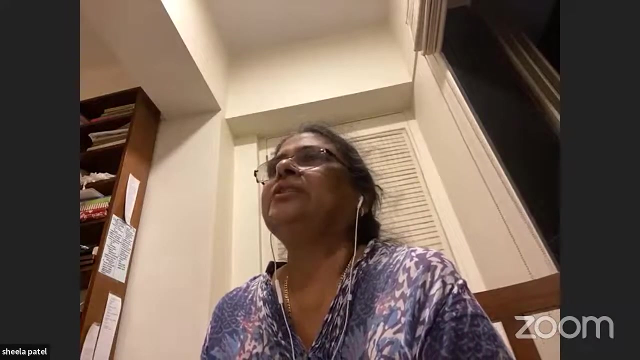 I said something profound and you missed it. See, you know, what Professor Ramchandran said is true, that there should be demand 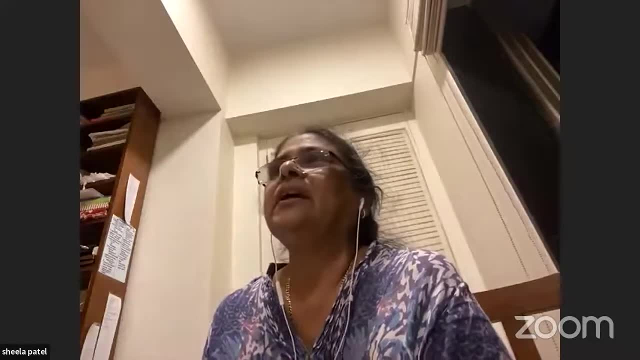 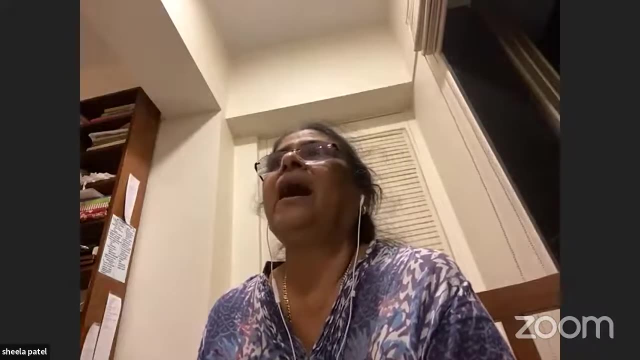 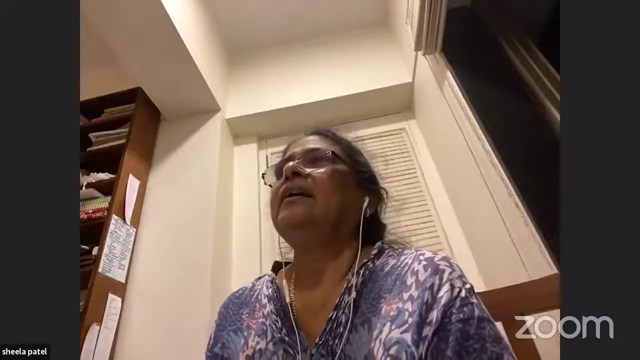 and there should be acceptance. But the reality is that the issues in cities are not decided by cities. They are decided by citizens of the city. We are so embracing the, you know, the fact that the city, you take the smart city mission. Okay. 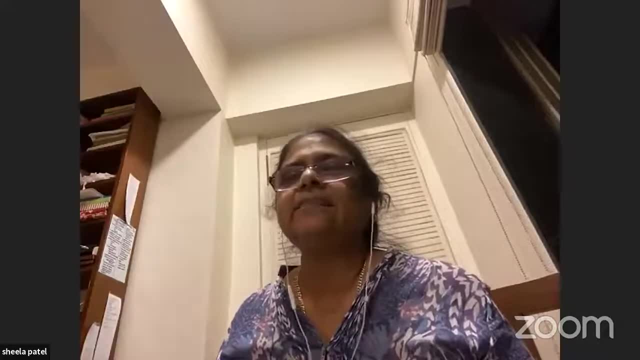 It's not a smart city mission, in my opinion, because the smartest thing to do would be to provide everybody water, sanitation, drainage, sewage, and transport. 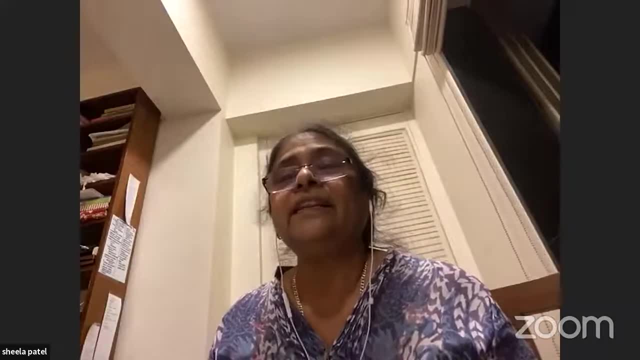 If you did that for everybody in a strategic and good way, it would be a very good thing. It would transform people's lives. 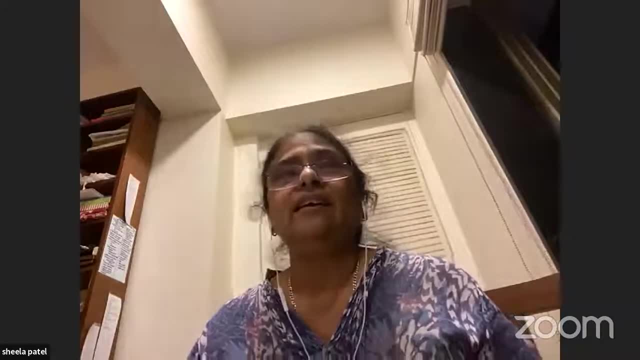 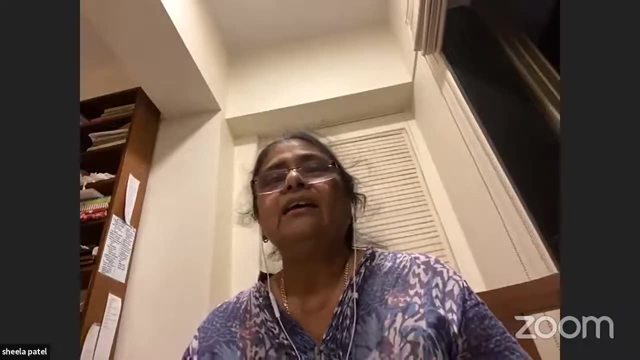 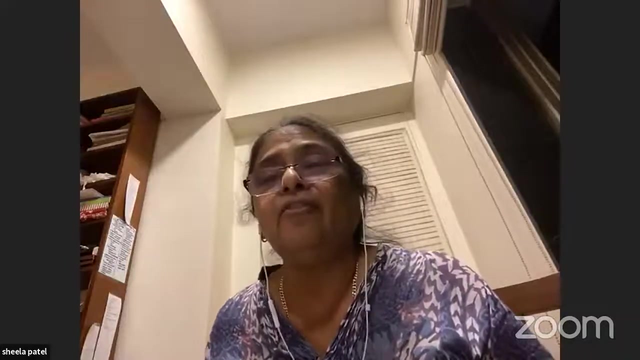 And as our friend from Milan said, you look at schools, you look at health centers, these are all the functions that cities must do. There is nobody in the city, in its design, planning, and execution, nor state governments 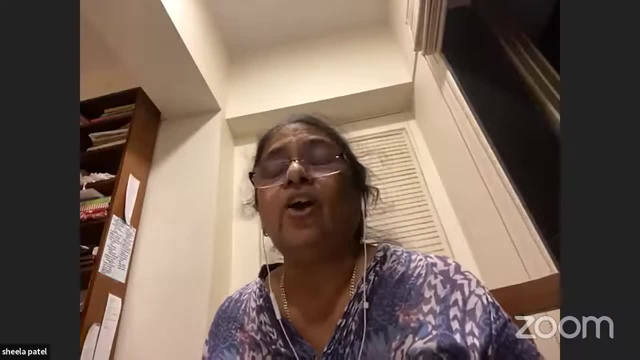 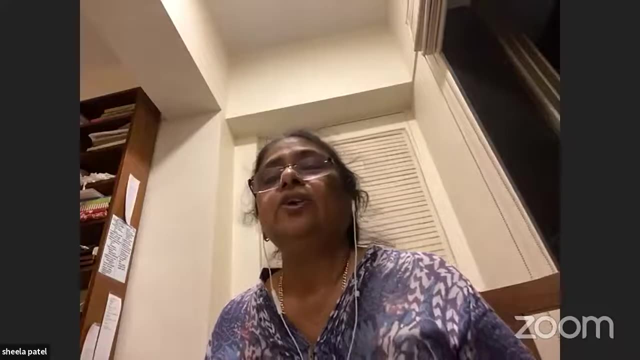 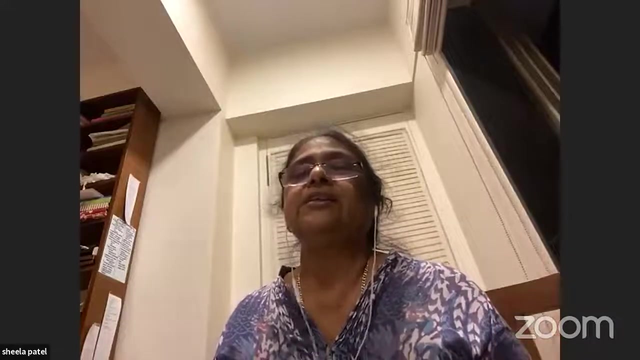 whose business it is to ensure the governance of cities, who care about any of these things. Most of the decisions about gated communities and the obsession of allowing private sector to define the transformations in cities has destroyed or diffused the power of the city. 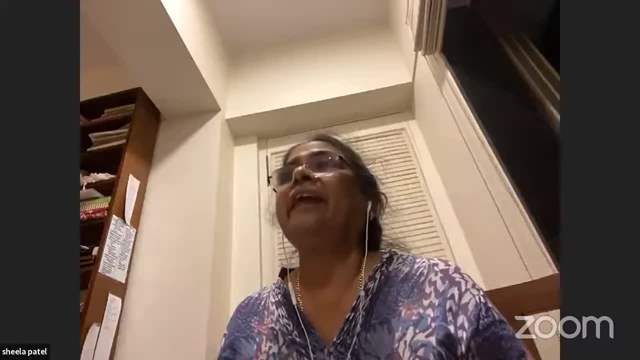 It has destroyed the power of the city. It has destroyed the power of the city. It has reduced or relegated to the side the aspirations of a larger number of people. 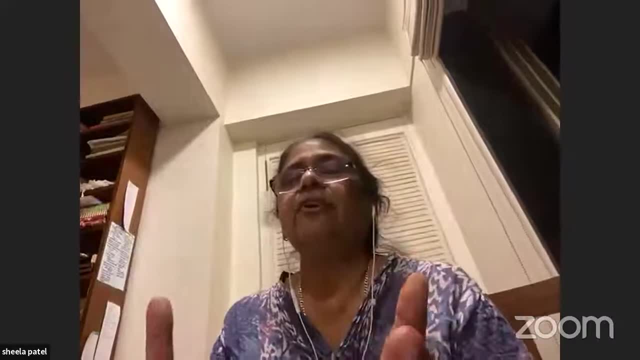 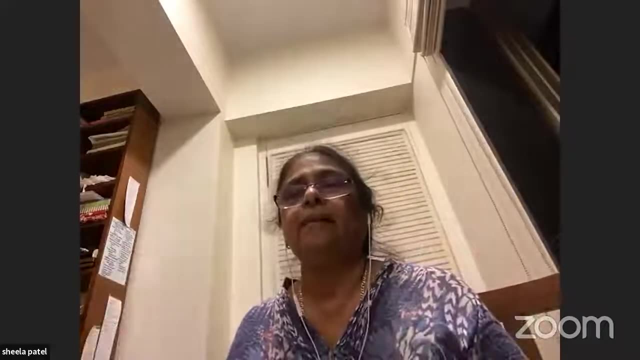 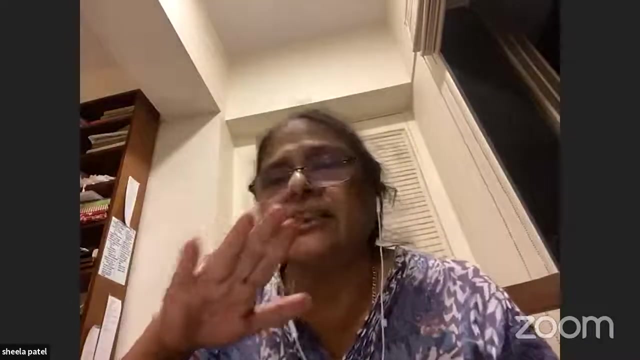 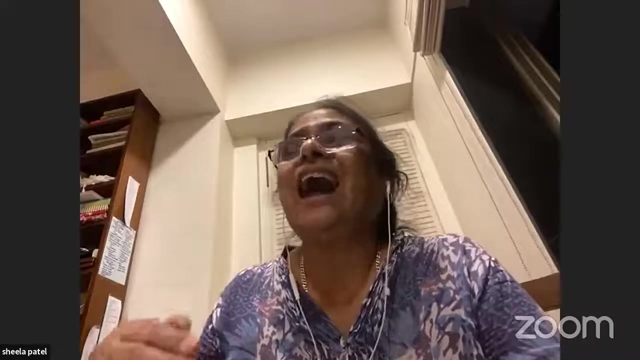 So, in this discussion here, we're not talking about the politics of planning. Who designs cities? Who designs where the open spaces are? I can tell you in the map of Mumbai, there are beautiful allocations. Not one single allocation is in place. So, the question is, who is the guardian of governance for cities? So, I am not being radical. 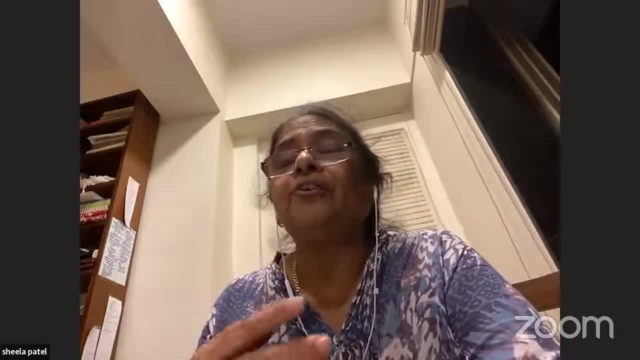 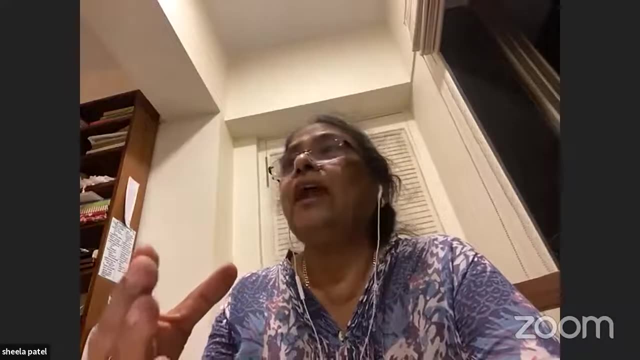 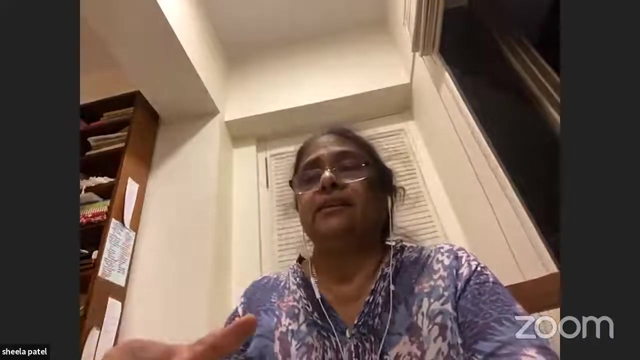 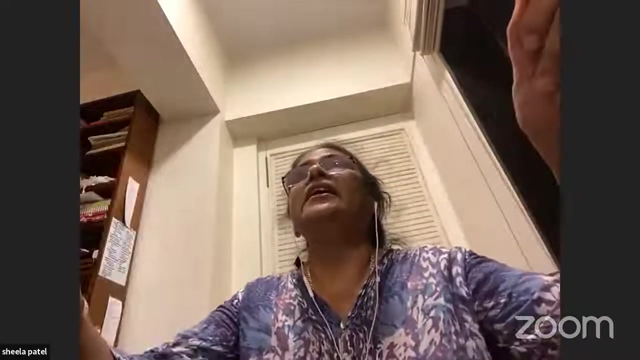 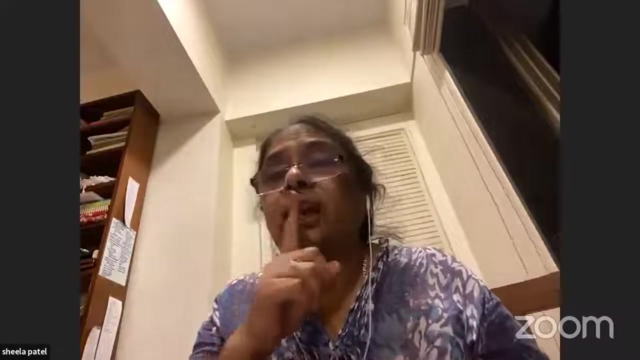 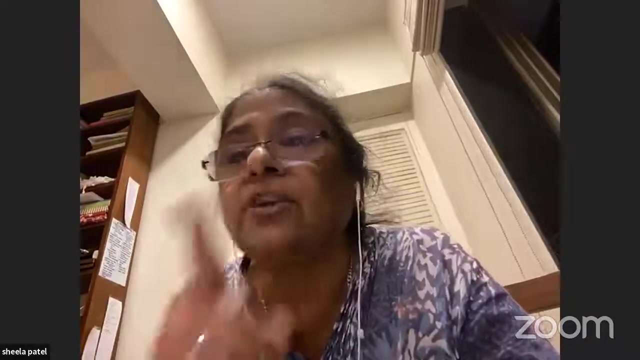 I am being respectful of the right to good governance that allows citizens to do. Today, if a group of people get together and even ask municipal ward offices, we work in 70 cities. Communities who take letters saying, you said our city is open defecation free. In these 17 slums, there is no toilets. They are told, shut up. We have told the state government that this is defecation free. Keep quiet. Don't say anything. 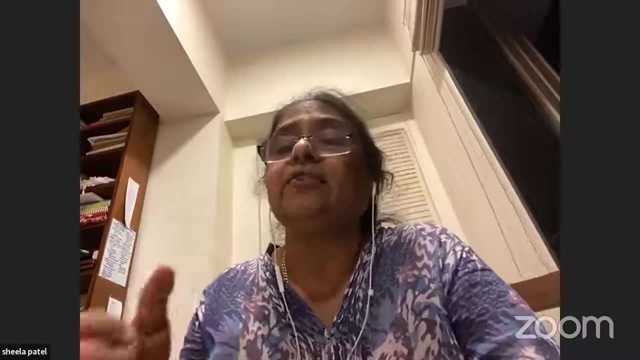 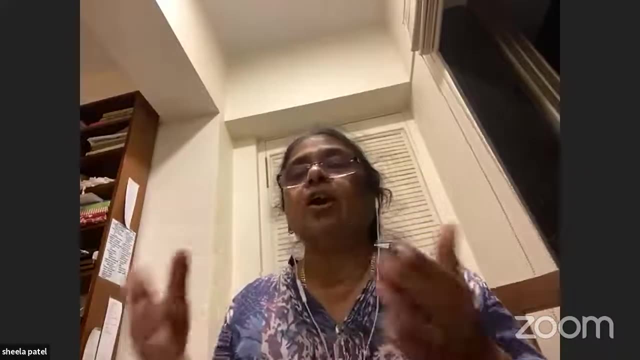 The real sad part of it is that stops those communities from getting sanitation, subsidies. So, you talk about statistics, you talk about data, it's all fudged. 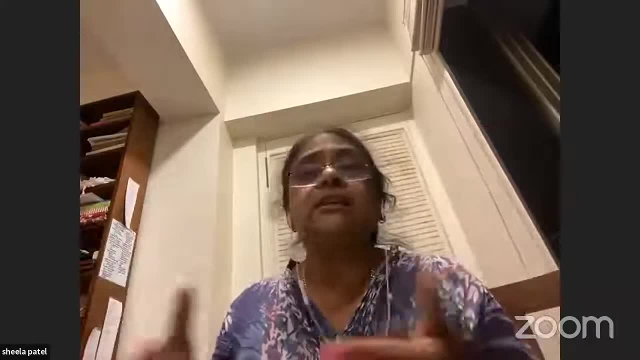 It's fudged in the name of getting prizes for your city and your state. So, what is radical about demanding good governance? 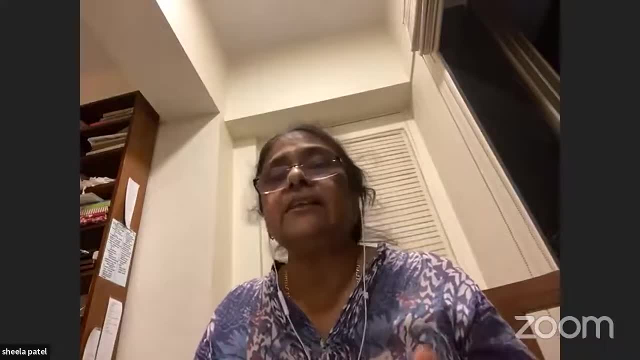 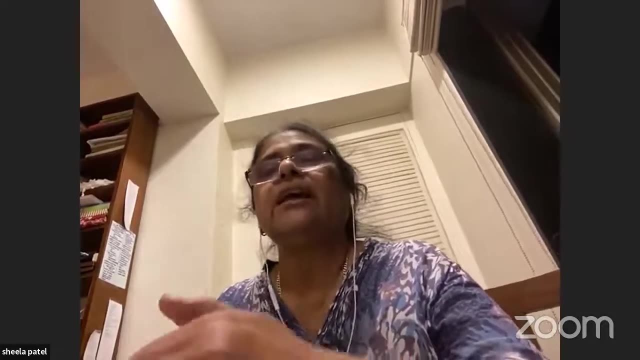 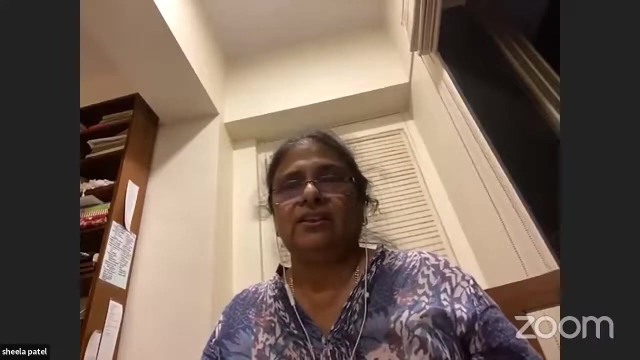 There's nothing radical about that. It's saying that citizen rights is a handshake. It's a handshake between the state institutions, its politicians, and the citizens. The minute that handshake is one-sided. People lose their voice and agency. 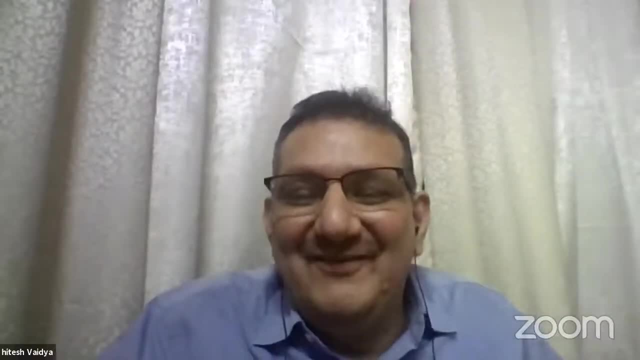 So, I'm not being radical. I'm being sensible. Thank you. 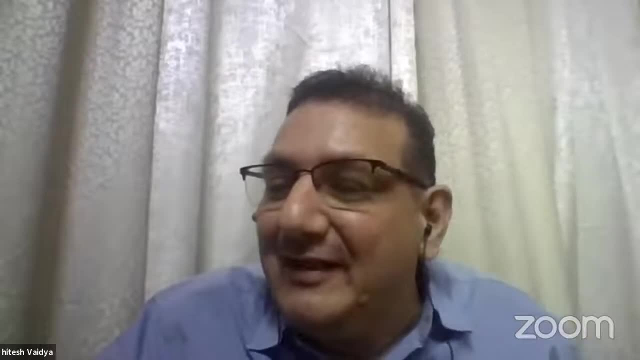 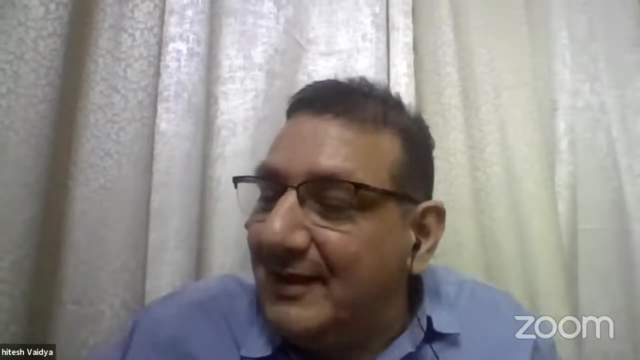 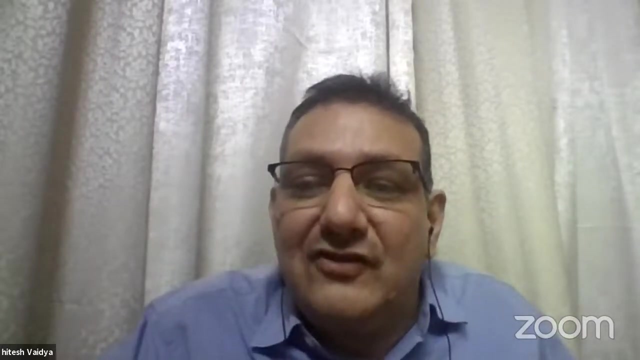 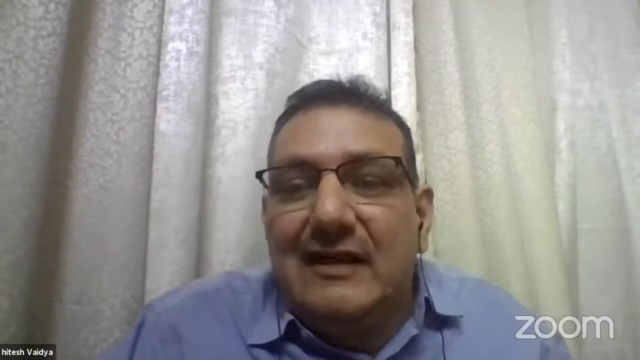 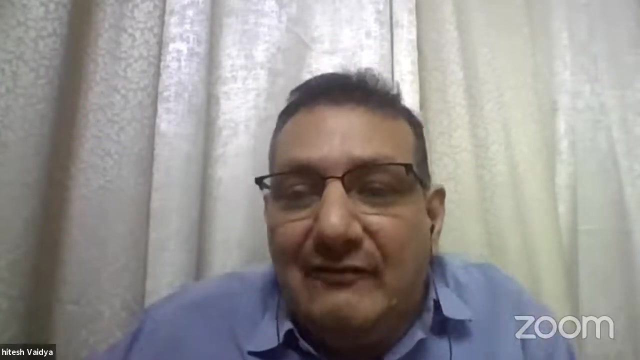 Again, the last question which we had before I close is to Massimo. Massimo, you talked about, you know, the key question is how do you see the relationship between the educational institute? Like yours and the local level planning which you talked about? You know, is it a consultancy-based thing or is it advisory-based? Or how do the institution becomes a think tank for the local body? What type of relationship that should have? Give a good answer. I care a lot for freedom. 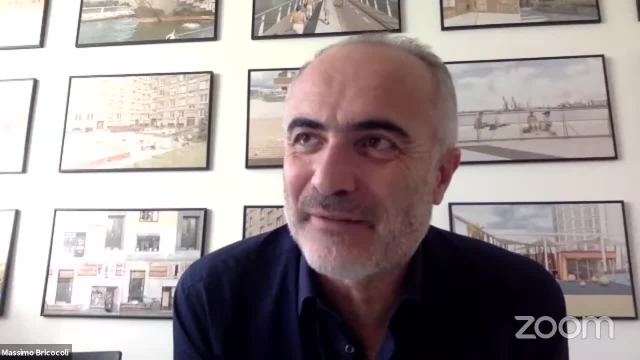 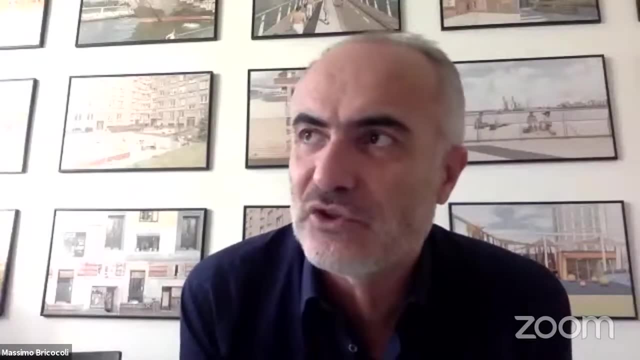 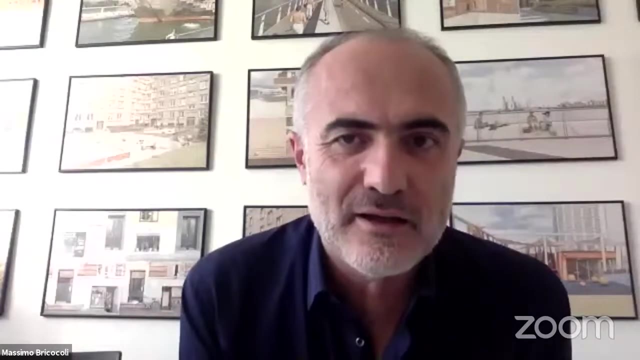 So, I, like, I'm thinking yesterday we were on lockdown. Yes. We were on site with 40 students, international students and Italian students on the site which is owned by the public housing agency. And let's say it took me quite several years to gain the trust of the housing company. 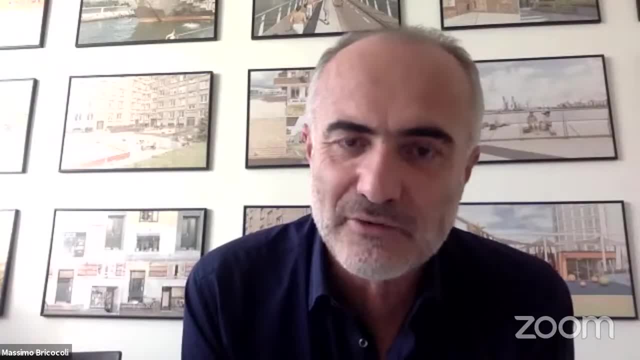 I've always been quite critical in many respects. 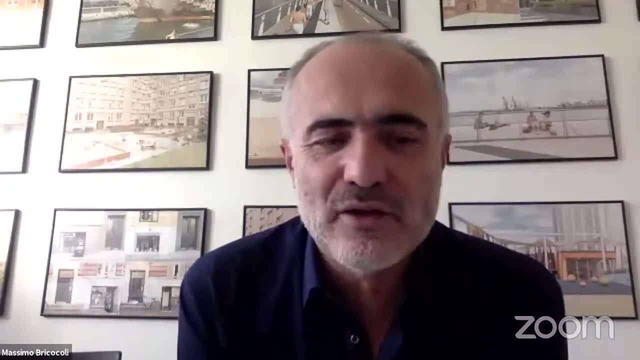 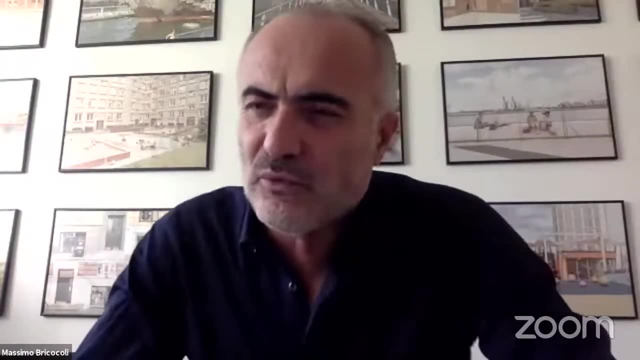 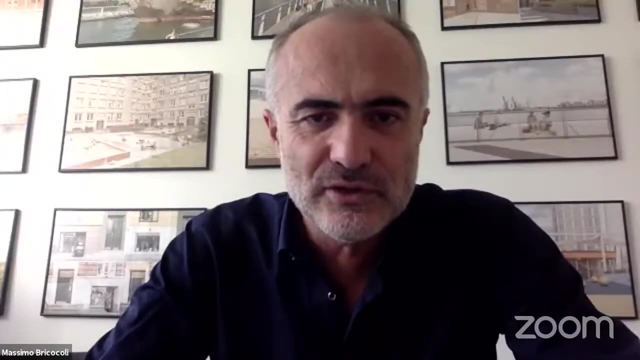 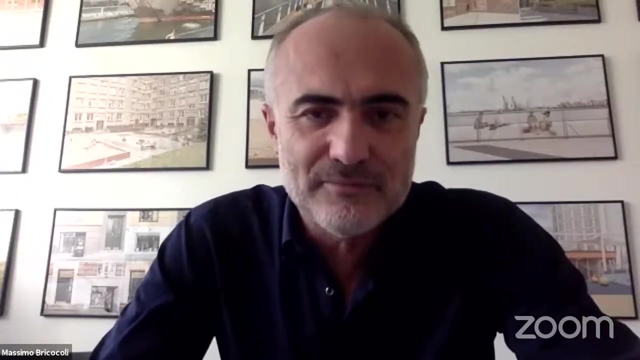 And I think it's a matter of balance. So, I think it's really important as a university that we collaborate. We bring ideas. We bring innovation. But we should also care for having the freedom of keeping our critical attitude in a positive way, in a positive way, but to not to be, to speak out, to always have a voice on things 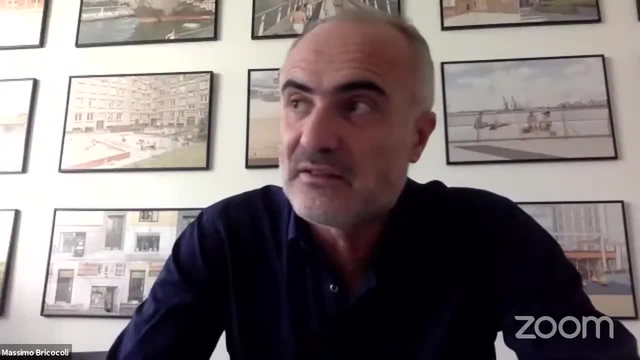 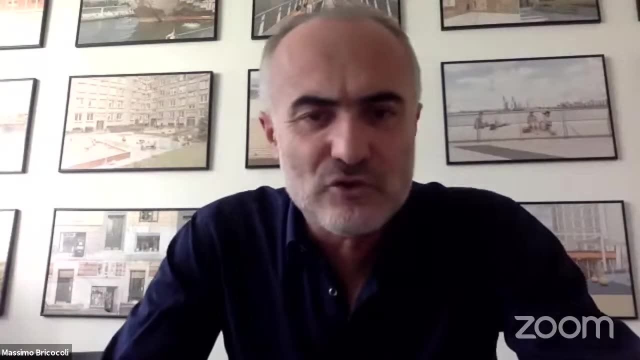 that we study and observe. And I think for the students it's a great chance because something which I realize is that in planning, also in doing research on planning. 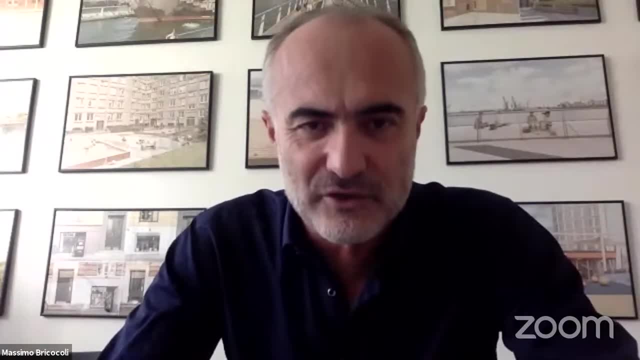 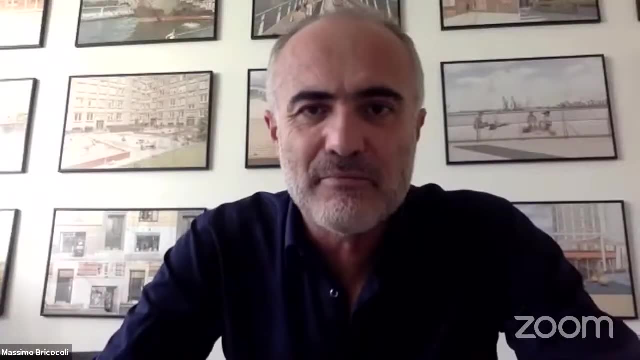 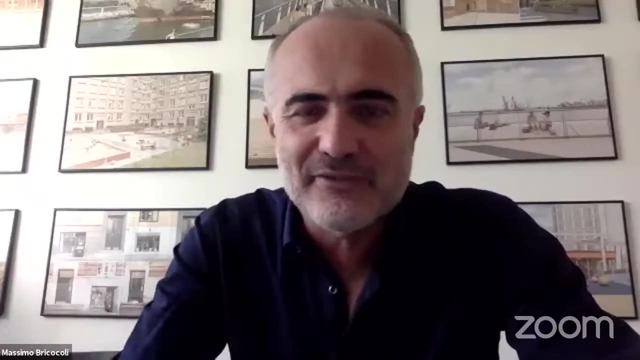 If you are involved, you really have access to information. If you are not involved through interviews, you really remain on the surface. And many of the real processes, the real decision processes, the real interests, you cannot really understand anything. 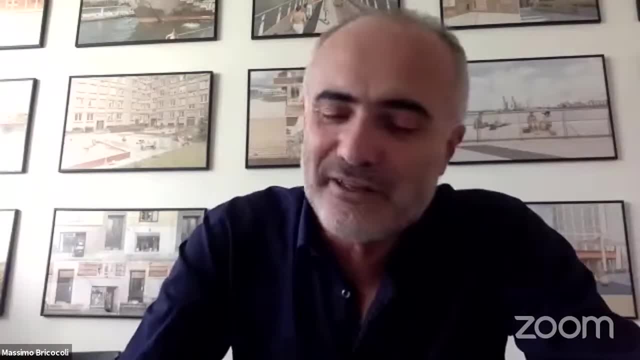 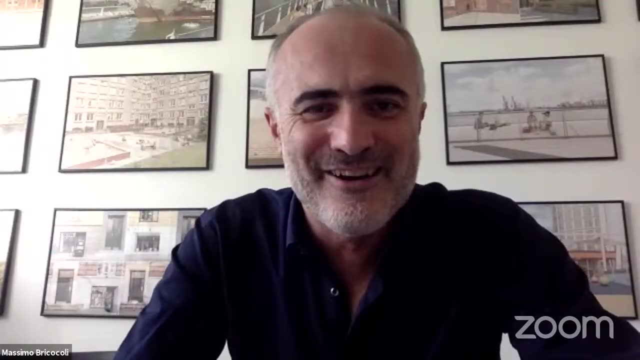 And journalists, at least, I don't know in India, but we cannot rely on journalists being those who really investigate on many issues. 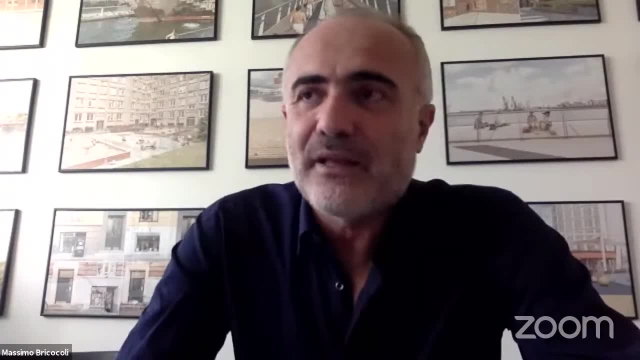 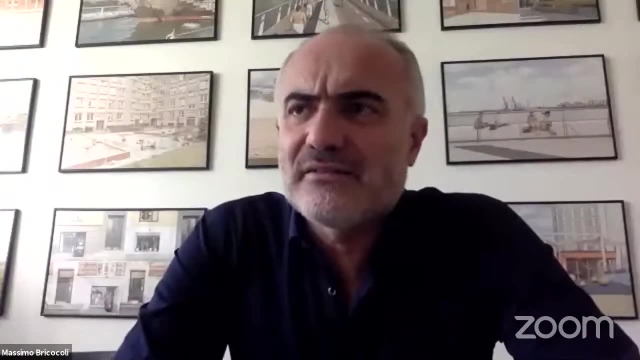 While if you are involved, there is always the risk that you lose your, a bit of freedom. But there are, if you find a good balance, it's the best way to understand how things 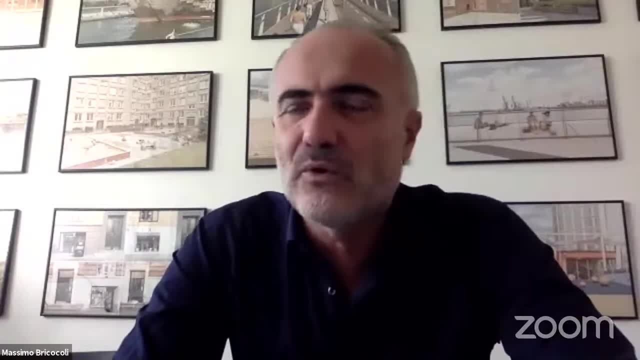 go and how decisions are taken and know who are the different actors involved. 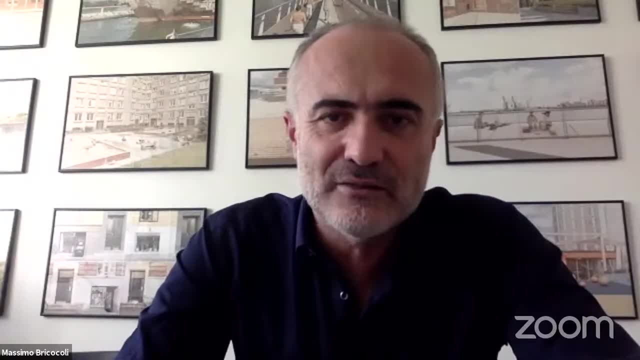 So, we work a lot in this direction. And we involve a lot of students in this kind of work. 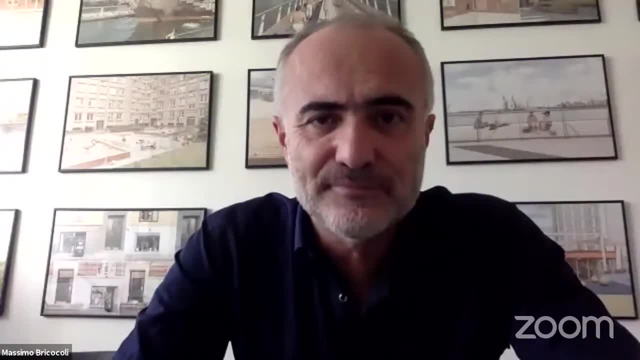 In this kind of on-site work that we do. Thank you, Massimo. 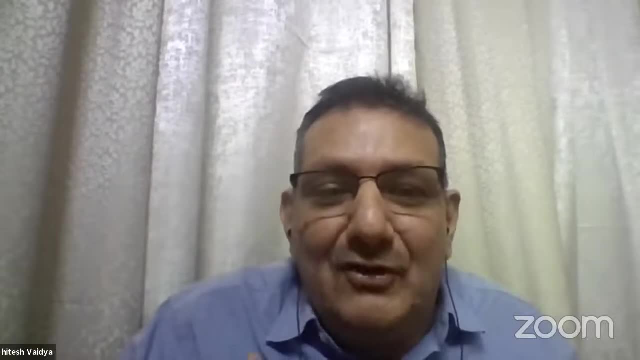 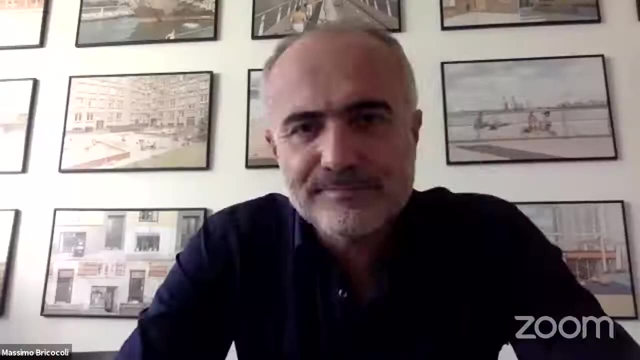 And, you know, I think I just don't have much because after listening to stalwarts, it's like searching for a needle in a haystack and telling that what can be done. 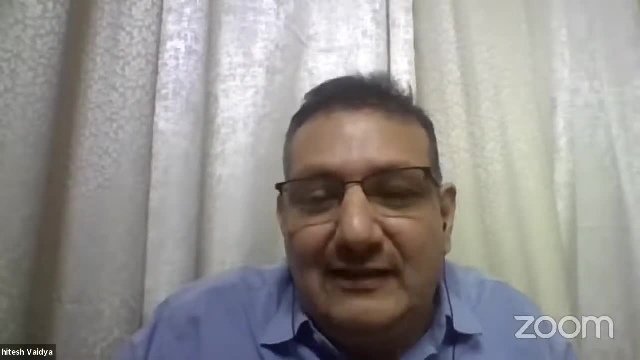 But I think one thing which all of you talked about, and I think which is a common, and I'll take a line from Sheila Ji. 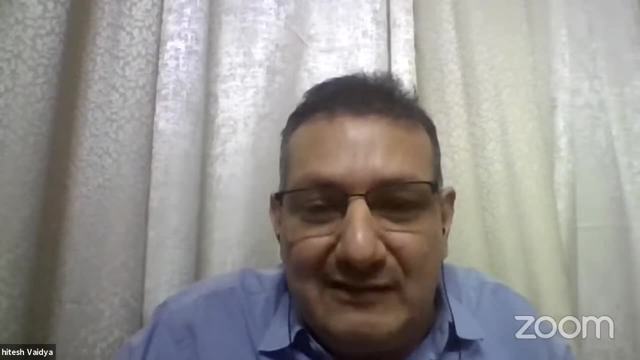 Which she's very clearly said when we are talking about reimagining cities or reimagining urban planning. 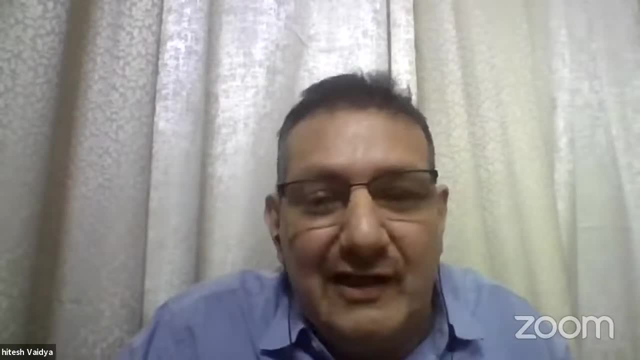 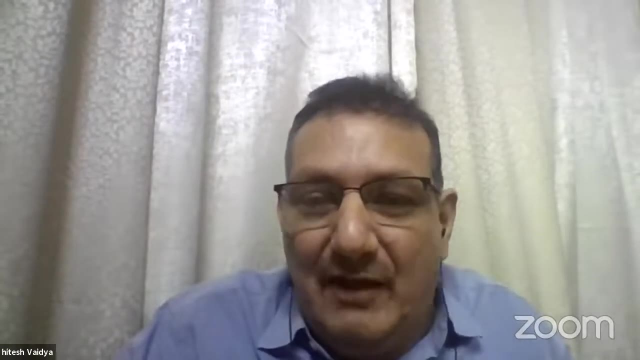 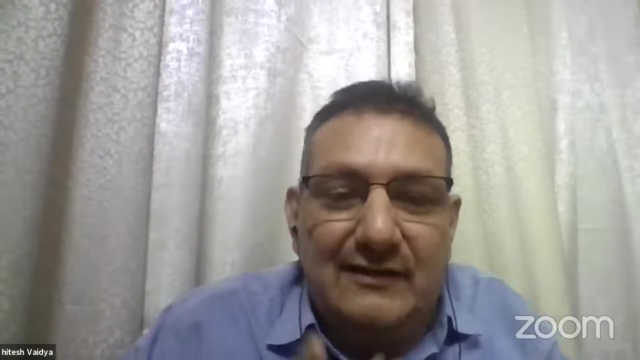 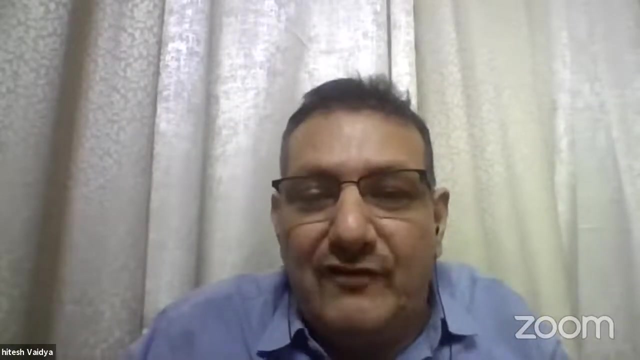 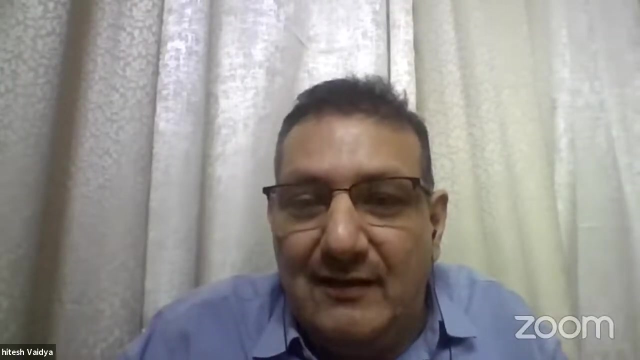 And I think she said it very nicely that local realities will produce local solutions. And these need to be scaled up at a city level. But we need to focus, and I think Massimo, Professor Ramachandran talked about ward level areas and local sabhas. And Professor O.P. Mathur talked about evidence-based research. But all of them. I think four of them, one common factor which four of you really talked about is go back to your neighborhood planning. Forget about, you know, start talking to people at the local, local level. 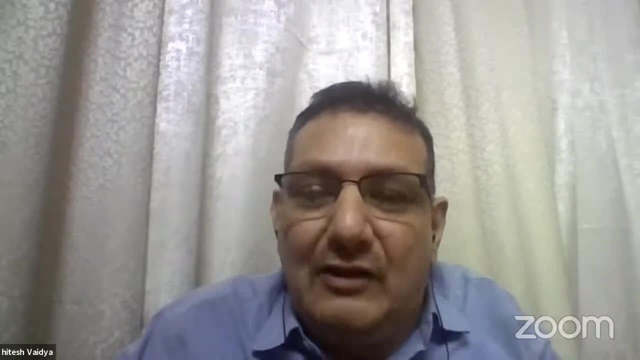 Come up with a granular work at the local level and create that data, that evidence, which can then be scaled up at a city level. 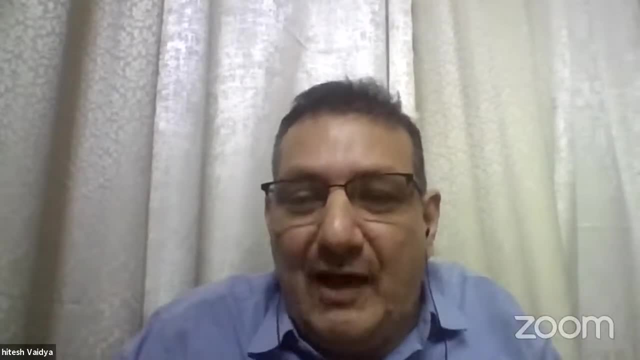 And just don't bog down with the master plan of a city and make a very colorful, beautiful plan. Be more realistic and more citizen-oriented. 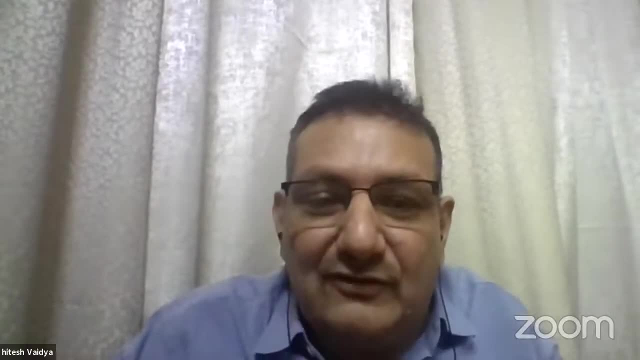 And I think that's the way I will try to sum up. 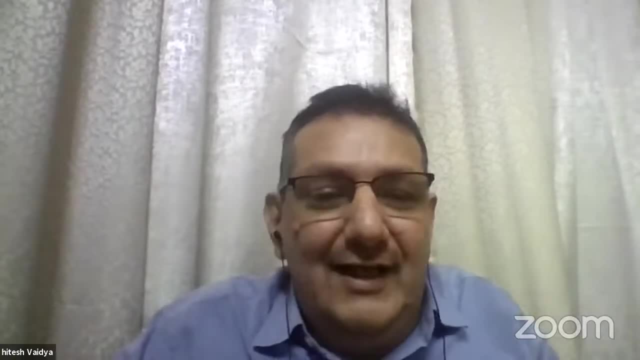 And I just wanted to, again, thank you all for joining us, spending time, sharing with your thoughts with us. 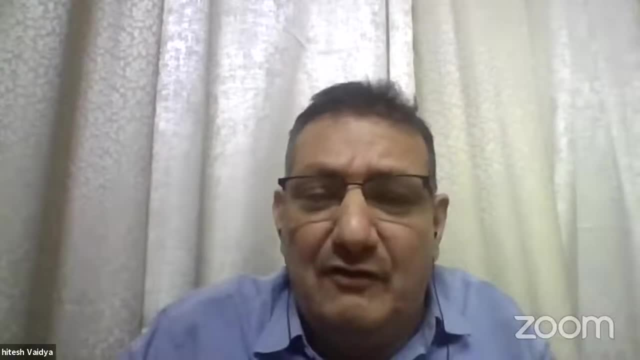 They were very enriching and really gave a lot of hope for way forward. 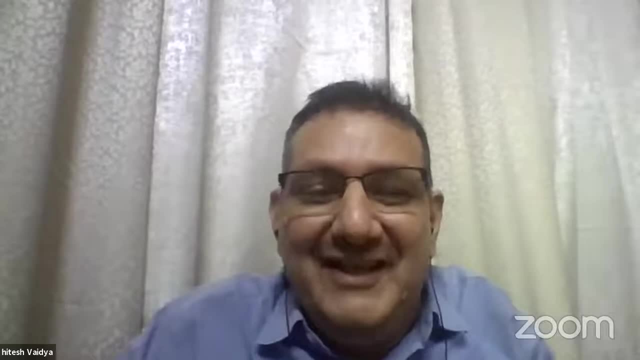 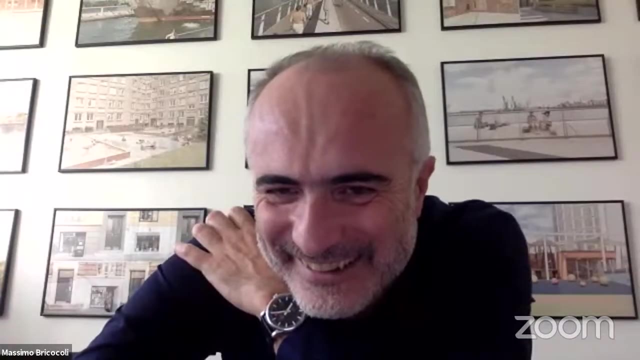 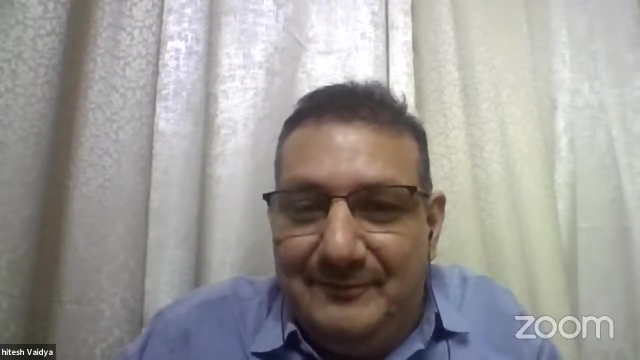 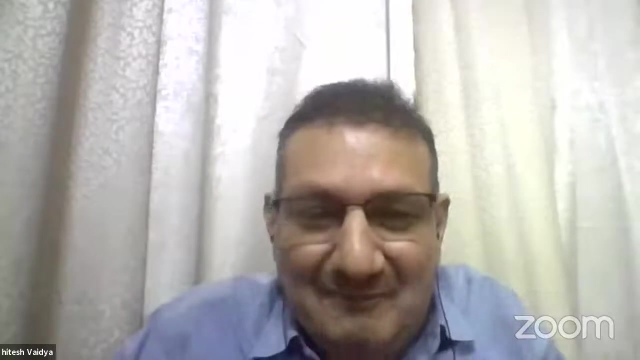 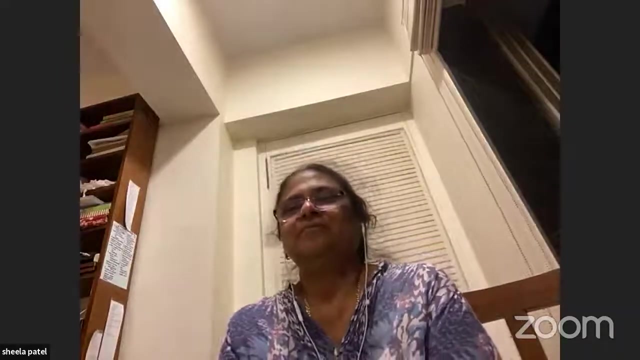 Sheelaji, don't be so pessimistic. We'll definitely take things step by incremental. But we are taking baby steps forward. And we will definitely, you know, take it forward. You know, I won't, you know, I think that this generation which is there right now will not disappoint you that we will take that. So with that, I will request Ravi to give concluding remarks and move forward. Ravi, over to you, please. Yes. 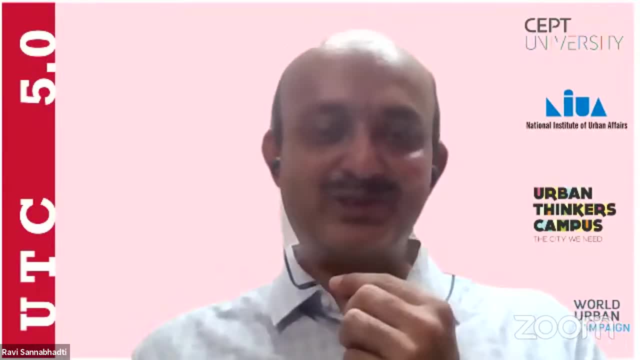 Yes, sir. I would just say thanks to all of you. And some of you have really kind of thrown up questions that will need a lot of thought from us, especially for, as Sheelaji says, for a light institution should not become ivory top, ivory top institutions. So it is, it is certainly kind of, it's food for thought as to how does pedagogy kind of influence some of these practices and policies. Because today's, today's students are tomorrow's planners. And whether, how do we deal or how do we kind of make them realize this is, is something that we have often debated amongst ourselves. 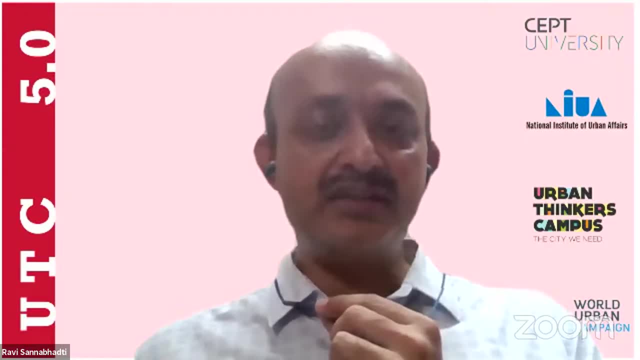 But this COVID situation kind of makes it, makes it much more starker, as Professor Massimo has said. 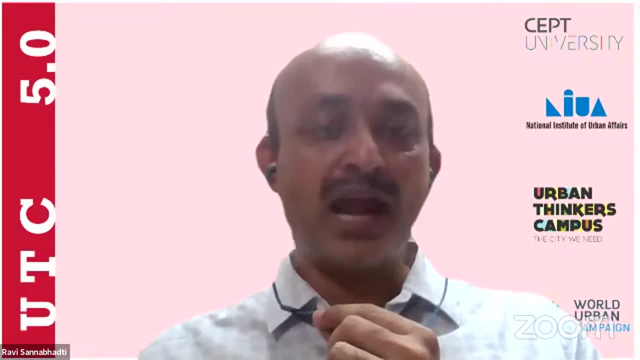 Or rather, can evidence-based planning go hand in hand with community-based planning? The community-based planning is something that, when we listen to Professor Optima Thor 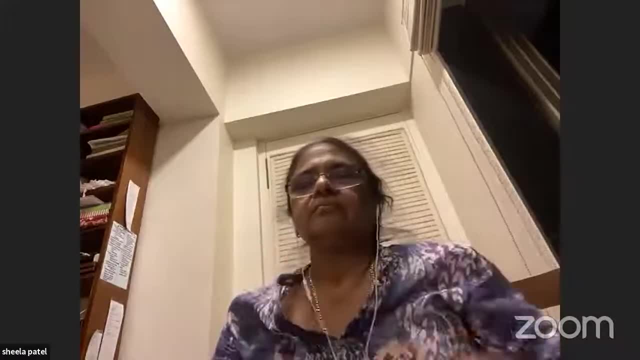 and Sheelaji simultaneously, it makes us wonder about that. Okay. 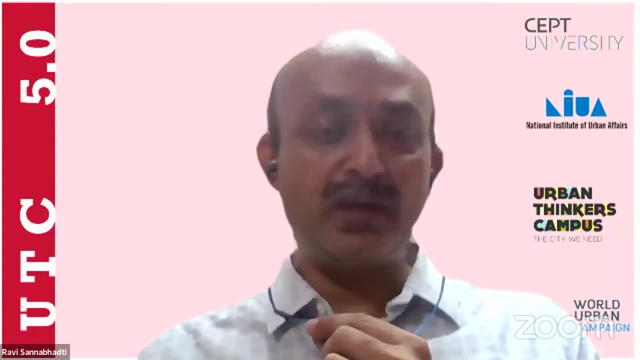 Can, can communities themselves become propagators of evidence-based planning? So, and which evidences are we talking about? 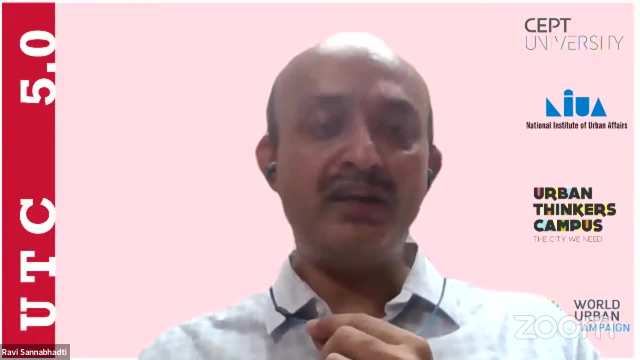 Whether evidence is coming from just data or lived experiences of people as evidences? It makes us wonder about some of that. 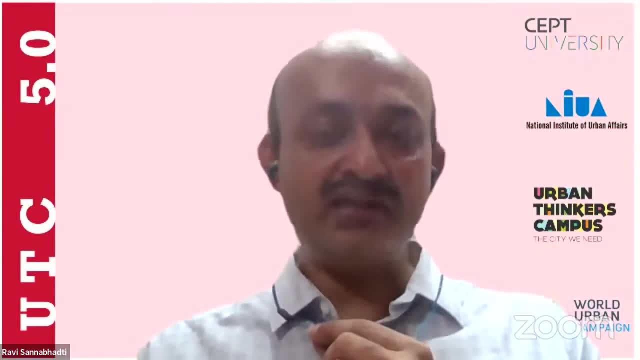 It makes us wonder about some of these things. So, it has been, it has been, for me at least, and all those people who are still remaining as a part of this, a thought-provoking kind of exercise. 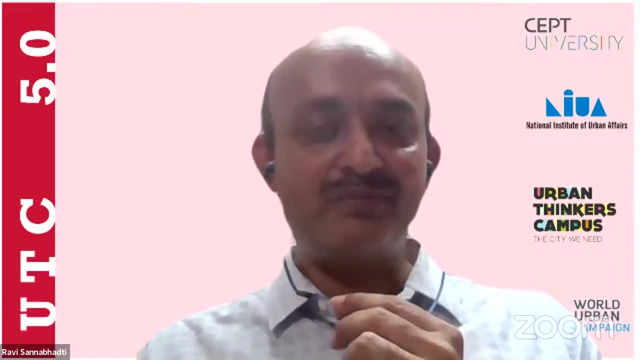 So, I would, I would really thank you for, for provoking these thoughts. And I would, I would second Hitesh's, this kind of, what he has been arguing. 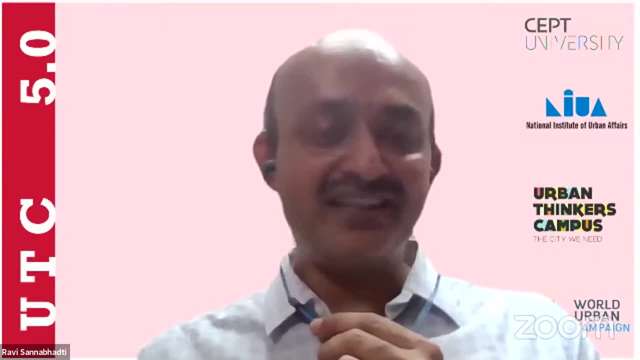 And it's really not so pessimistic. If after this, from about 160 or 170 people, if about 80 people have stayed back, that is still glass half full. So, that is, that is, there is hope. 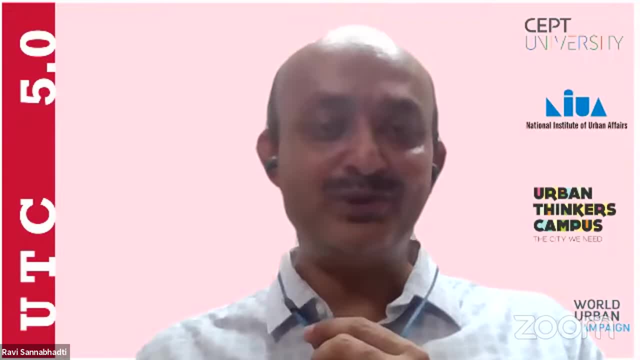 So, I would just request all of you to stay back for five minutes in this same room. So, the students want to kind of, as a token of our gratitude, the students have kind of created a small digital memento for all of you. Oh. 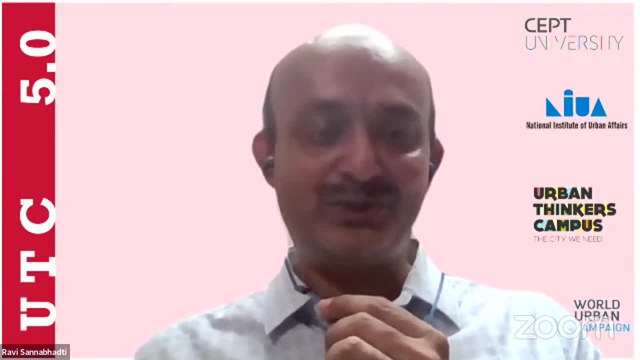 And they would want to take this, they would want to present it to you. 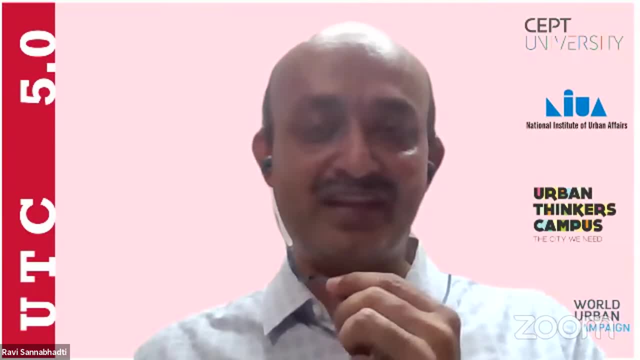 So, I would just request all of you to stay back for five minutes. 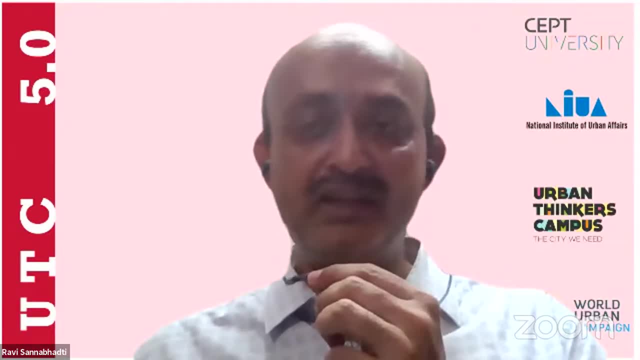 Can I, can I request Manoj to come? Yes, sir. 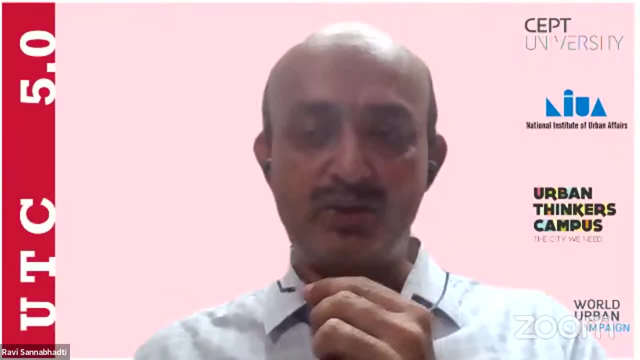 We do it here itself instead of taking them to the breakout room. Sure, sir. Yes. Yeah. 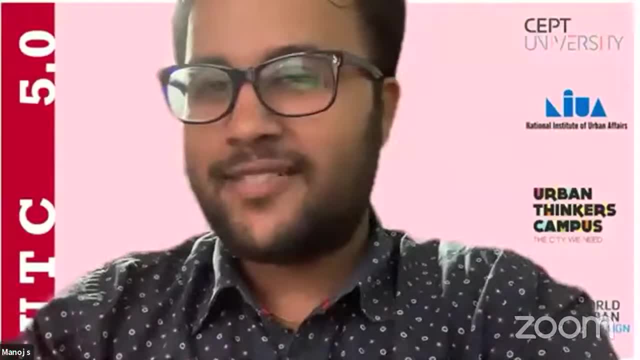 Before presenting the memento, I would like to introduce myself. Myself, Manoj. I'm doing postgraduate course in urban design, SEPT University. So, it's my pleasure. Can we also look at your video? Can you also be brought into the focus? We don't see Manoj. 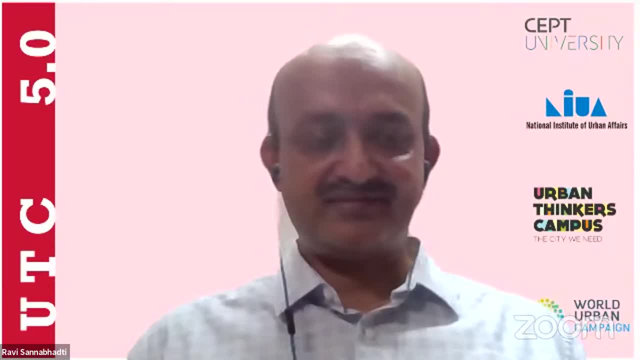 Satvik, can you hear? Yeah, we can see him. We can see him now. Yeah. 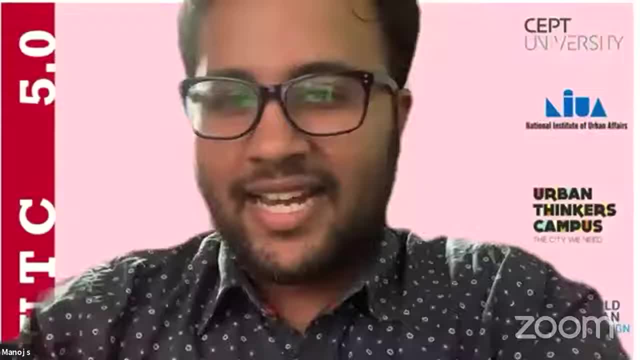 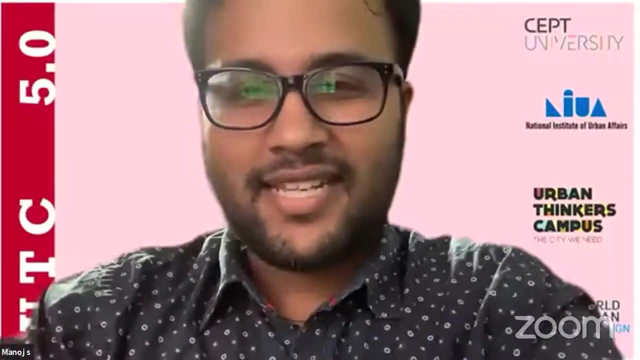 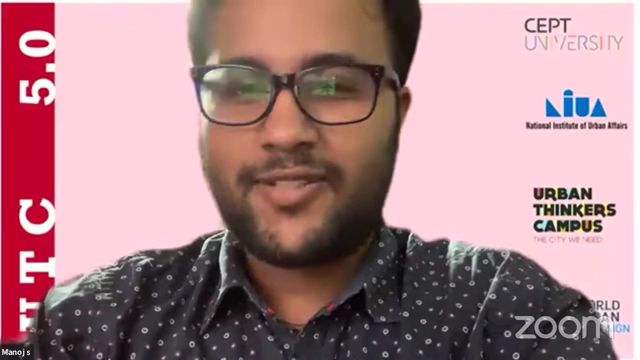 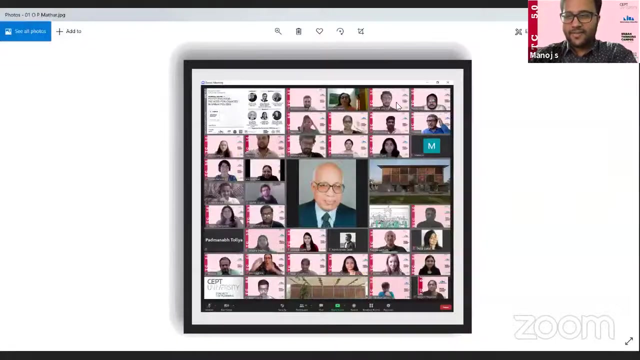 It is my very much pleasure and extremely honored in the meantime to provide a virtual memento to the esteemed guest for the UTC event, technical session one. So, I'd like to ask Niveda to present the screen. Please accept this with our sincere thanks. We'll start with Professor Hopi Mathur. Thank you, sir. 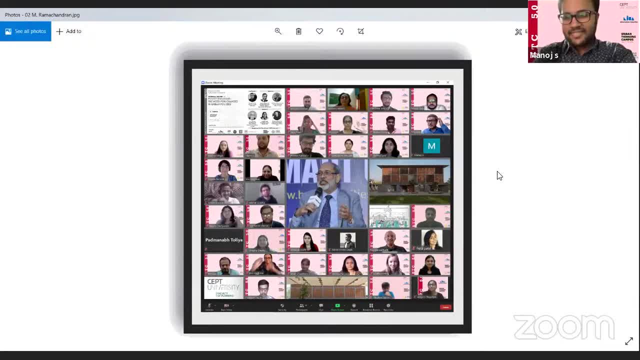 Moving ahead, Professor M. Ramachandran, IAS. 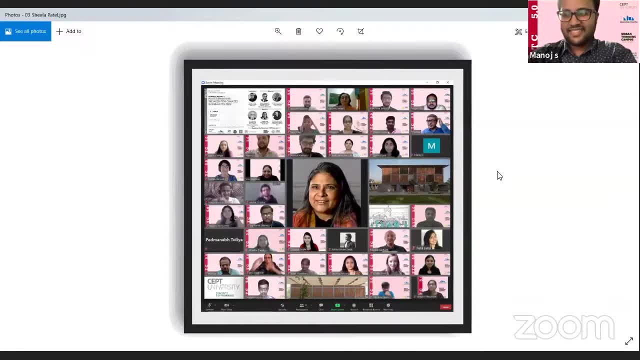 Thanks for joining us today, sir. For the next, Professor Sheila Patel. Thank you, ma'am. And Professor Masinu. 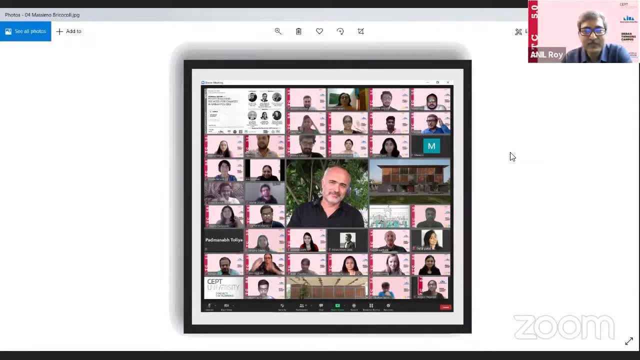 Thank you very much, sir. 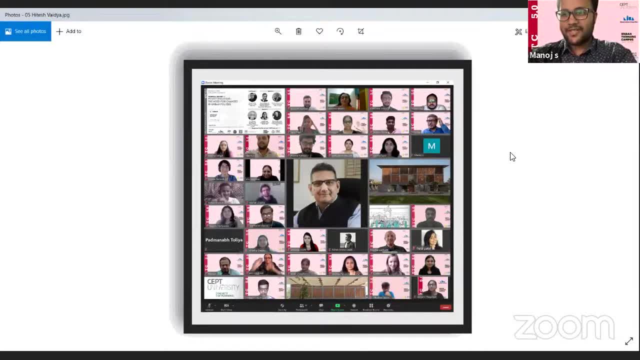 And in the last, I would like to present a memento to our moderator, NEUA Director Hitesh Vaidya. Thank you for joining us today, sir. 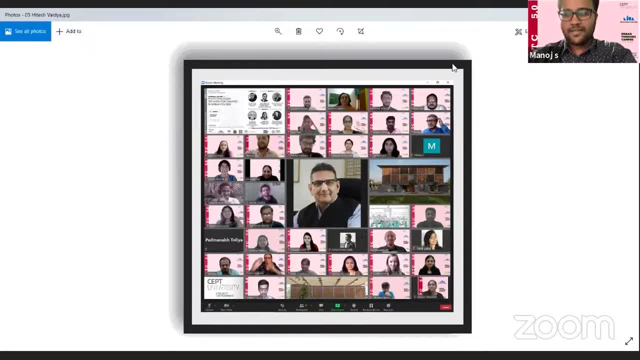 Once again, thank you, everyone. For. Presenting your thoughts and your experience with us. Thank you very much. 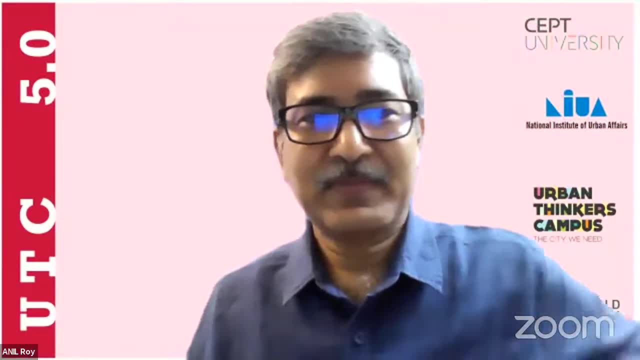 Bye-bye. Thank you, sir. Bye. Thank you. 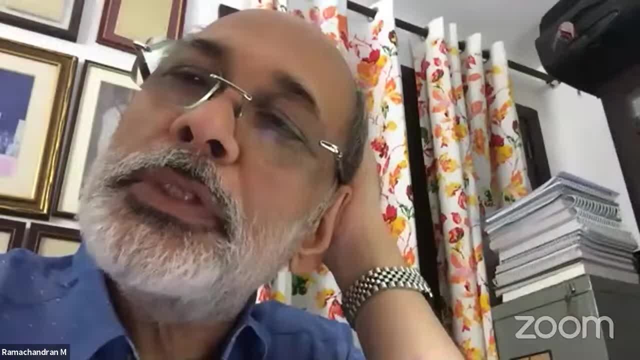 Thank you for that thoughtful, thoughtful digital. Thank you for that thoughtful, thoughtful digital memento. Maybe you can mail it to us so that we have it. Sure, sir. Sure, sir. That's a great idea. We'll do that. We'll do that, Amit. And, and, and. 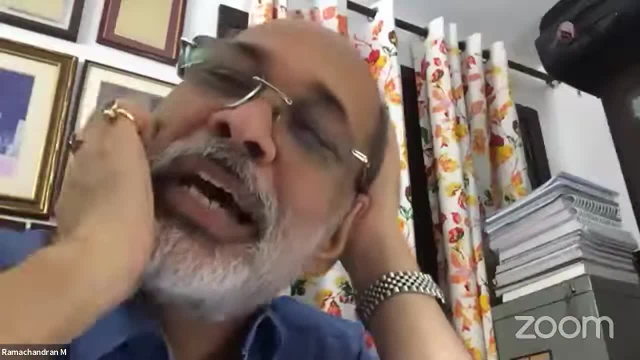 Hitesh ji. The existence of a happy change has been in this sector for any number of years. 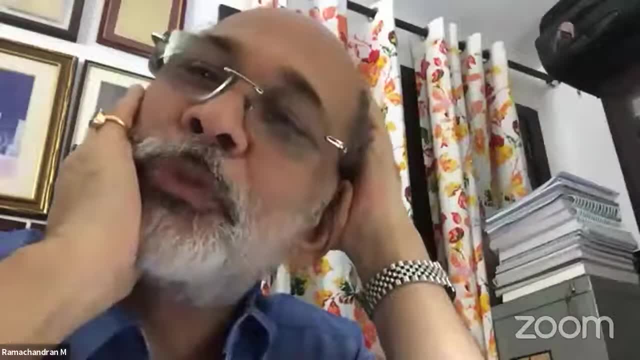 I can understand and appreciate Sheila. But I suppose what you stated would have slightly consoled her that. 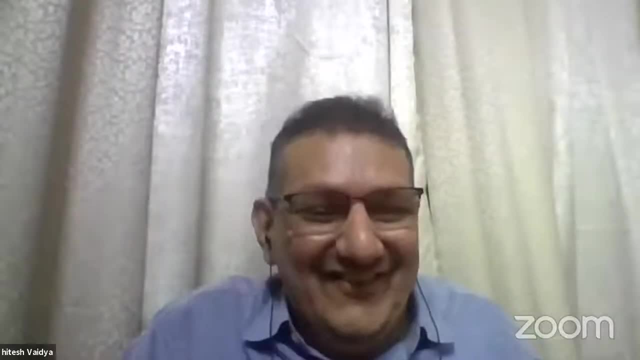 Yes. Changes are happening though. Not to the extent desired. 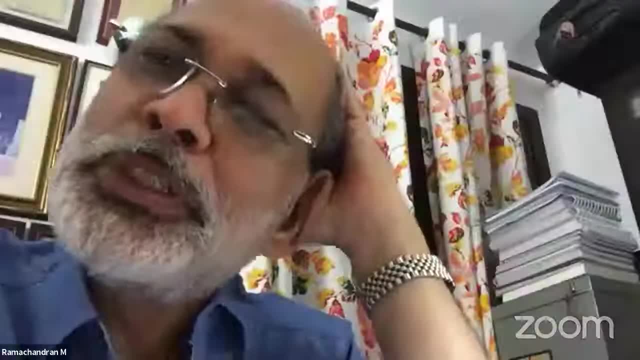 Also responded to the. Possible questions. 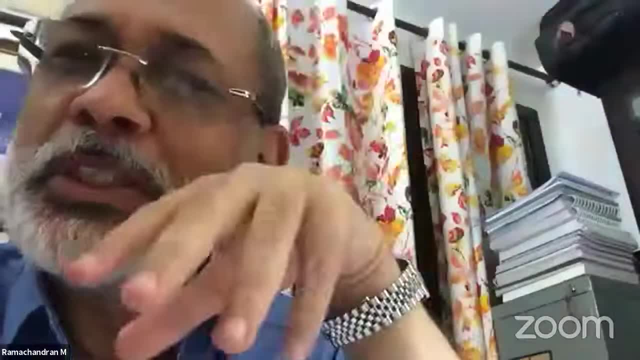 Who is to bring about the change. She has covered the politicians. 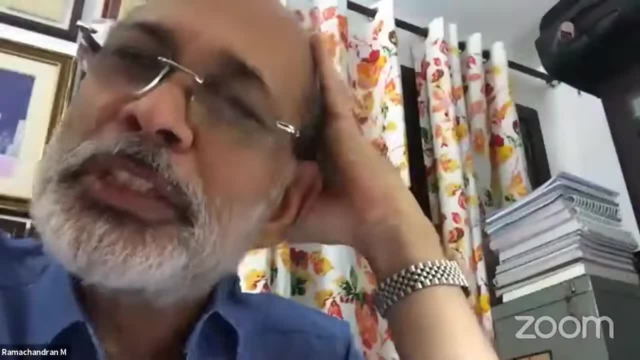 She has covered the civil service. She has covered the civil society. the youngsters probably should think of 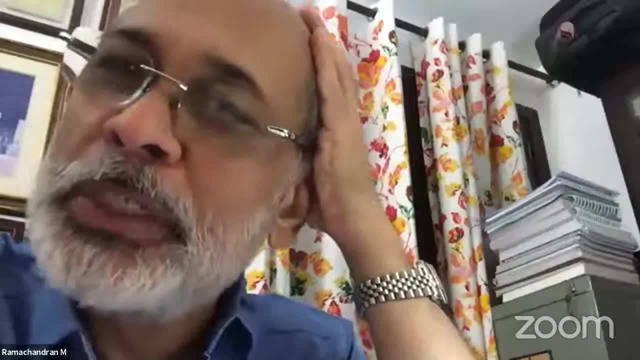 what could be a workable alternative. I always repeat this point that she also emphasized. It's not collusion which will deliver results. 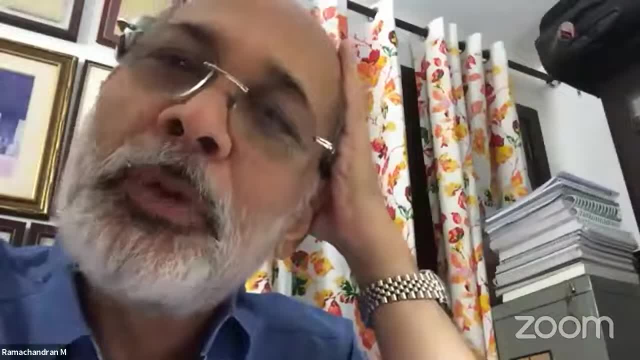 We have to think of methods of getting things done in a more positive, collaborative way. 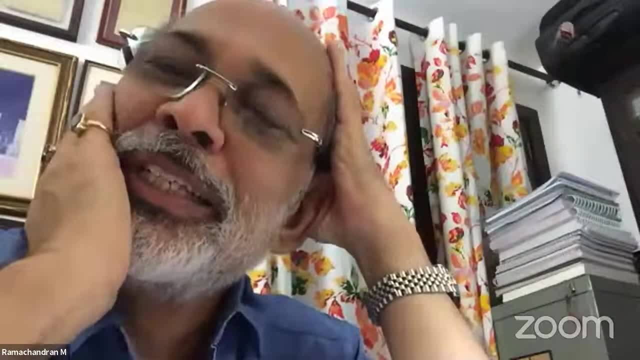 I appreciate, Sheila, seeing you once again on this platform. Thank you. Thank you, sir. Thank you. Bye-bye. Thank you. Bye. Thank you, Massimo. Thank you. Thanks. Massimo.